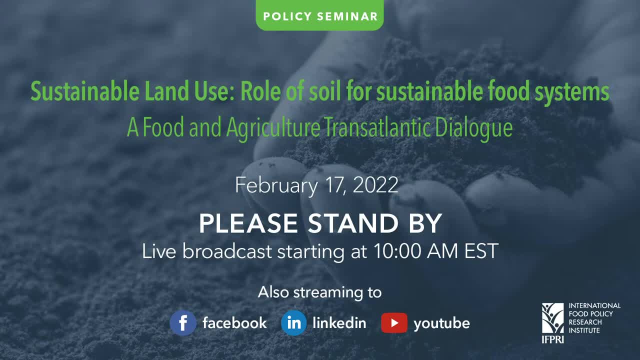 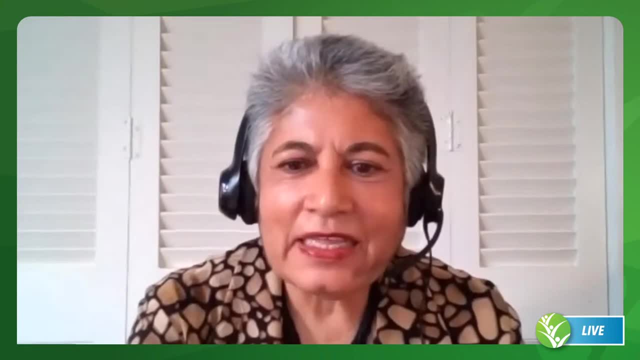 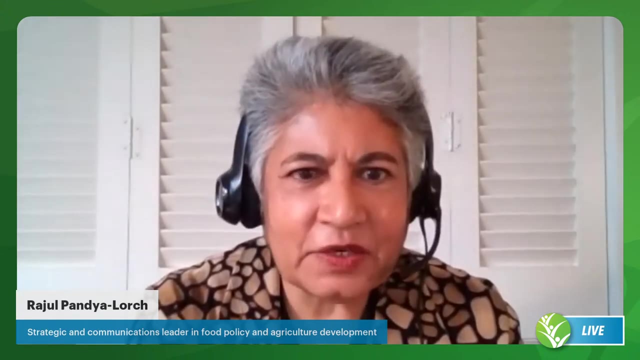 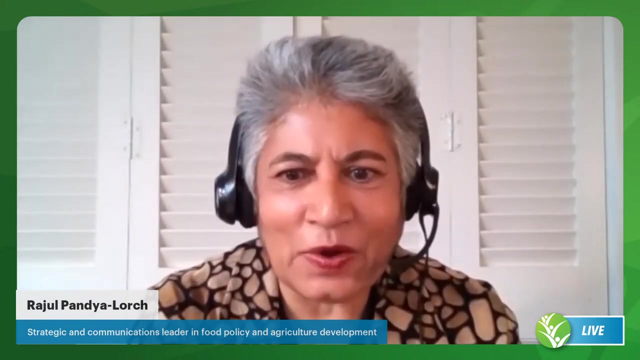 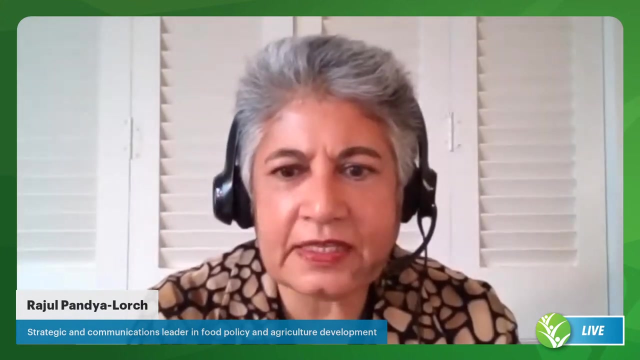 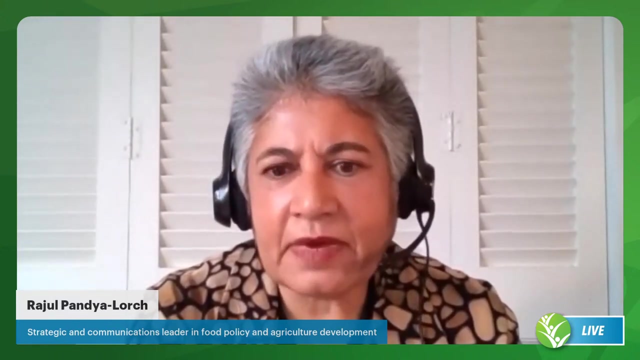 Hello everyone, Welcome to this Policy Seminar co-organized by IFPRI and the Embassy of the Federal Republic of Germany in Washington, on Sustainable Land Use: the Role of Soil for Sustainable Food Systems- a Food and Agriculture Transatlantic Dialogue. We will have the opportunity today to hear and discuss the key outcomes of the 14th Global Forum for Food and Agriculture, the GFFA, that took place last month, January 24 to 28.. 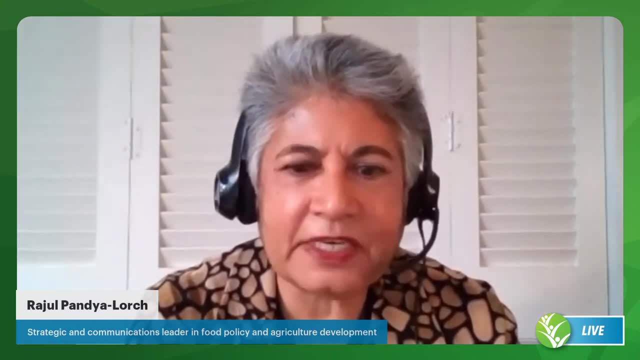 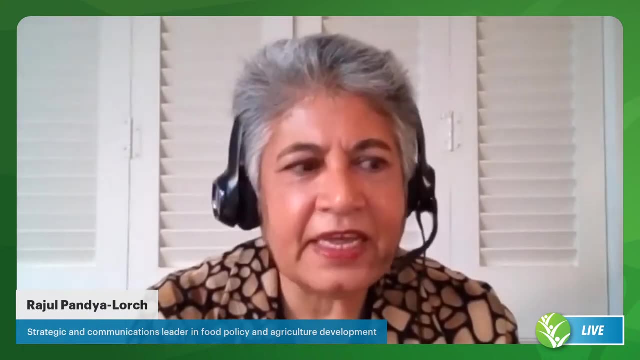 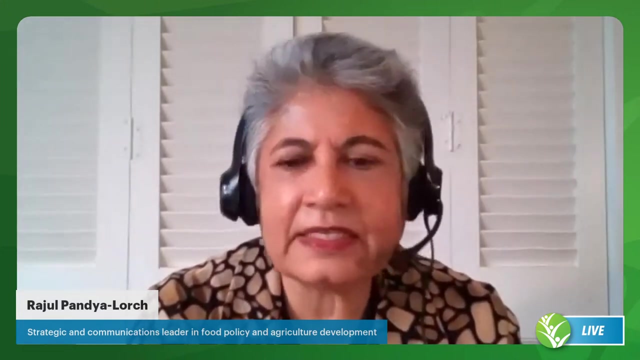 The GFFA is an important annual event organized by Germany's Federal Ministry for Food and Agriculture. In a few moments we will hear more about the GFFA and what it is about, And we will discuss the policies and the partnerships essential to move forward to the key topic it addressed: sustainable land use and sustainable soil management. 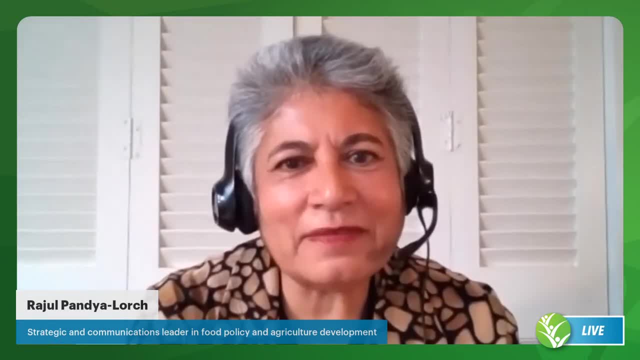 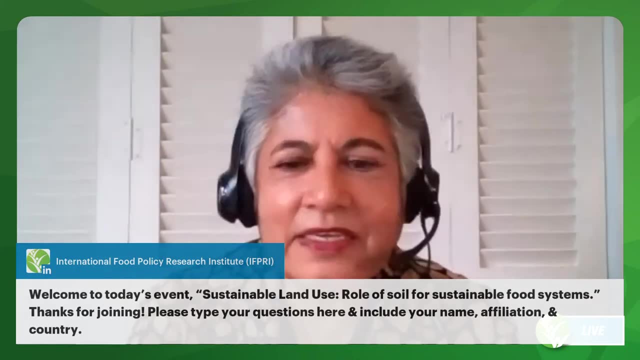 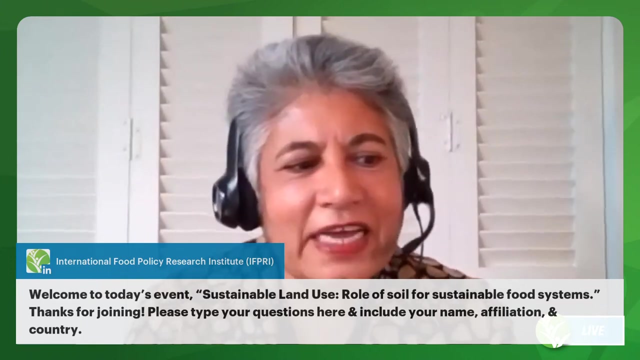 Thank you for joining this event. We would like to hear from as many of you as we can, So to participate in our Q&A session that will follow the speaker's remarks. please submit your brief questions on ifpriorg, Facebook, LinkedIn, YouTube or by using the hashtag. 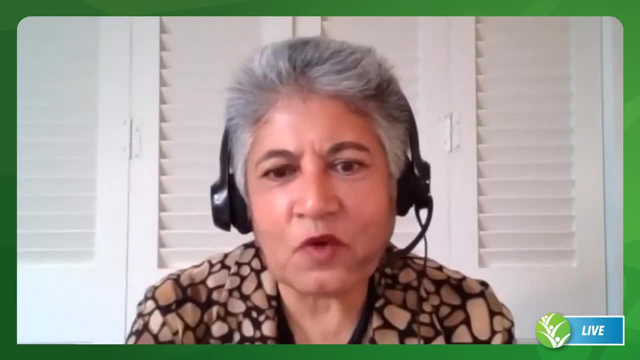 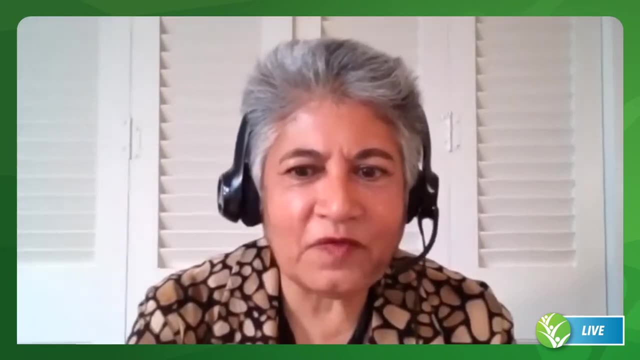 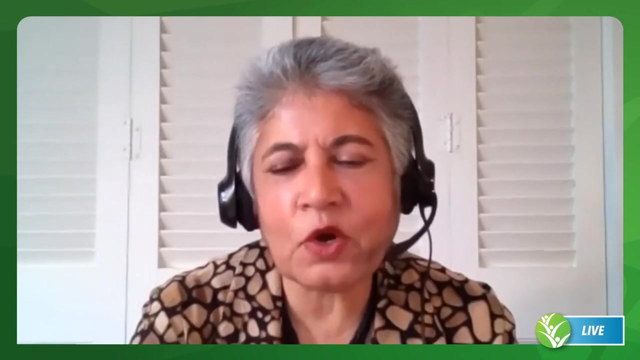 We have a rich and informative program lined up for you. so, without further ado, I'd like to call upon Johan Swinnen, the Director General of IFPRI and the Global Director of Systems Transformation of the CGIR, for his introductory remarks. Over to you, Jo. 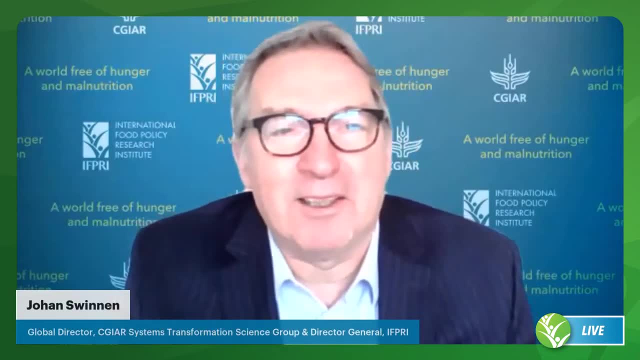 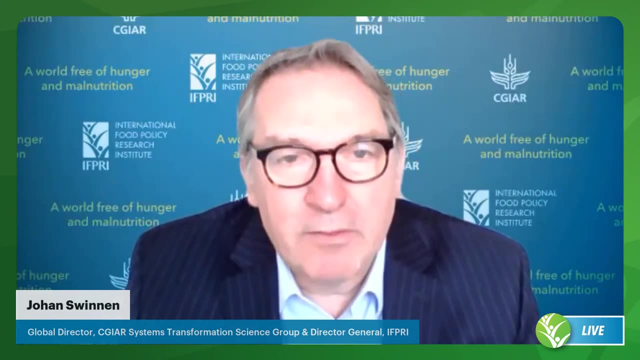 Thank you so much, Rajul. It's great to see you chairing this panel today, to have you back with us. Good morning, good afternoon and good evening, everybody. I would like to welcome everyone to the panel. I would like to welcome everybody to this policy seminar on sustainable land use and healthy soils which, as Rajul already explained, is co-organized by IFPRI and the embassies of the Federal Republic of Germany. 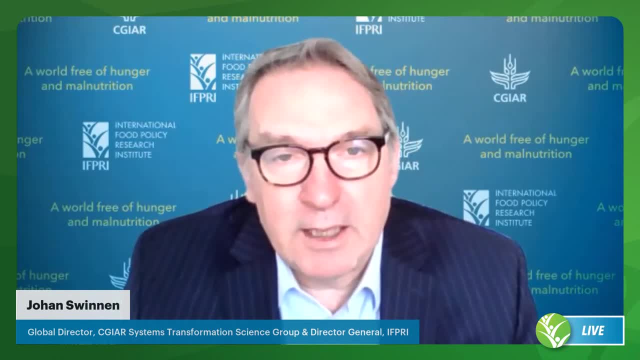 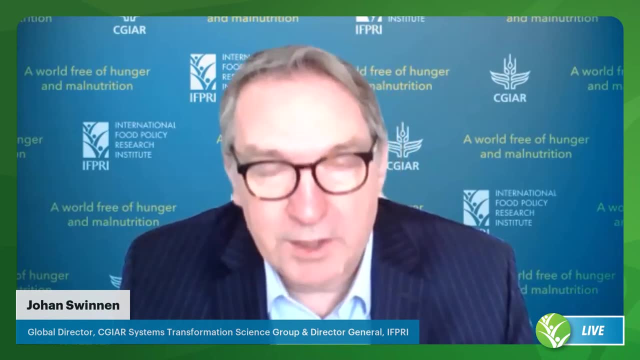 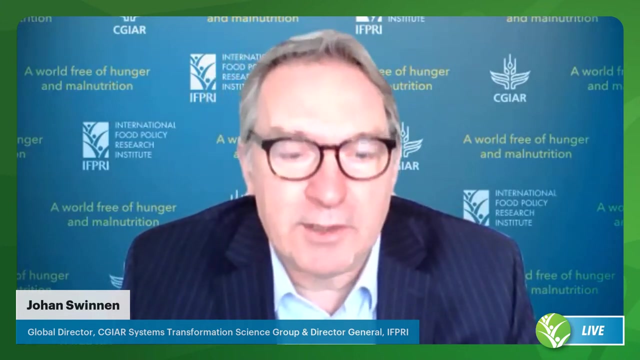 The event today is now an annual event which we host each time together with the embassy, following the GFFA which has been hosted in January, again in Berlin. So let me start by thanking our panelists. My pleasure, Thank you. 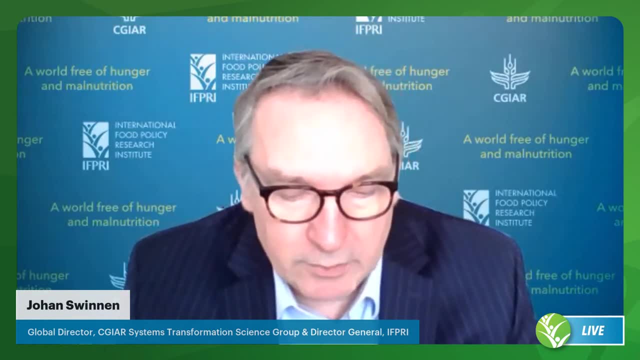 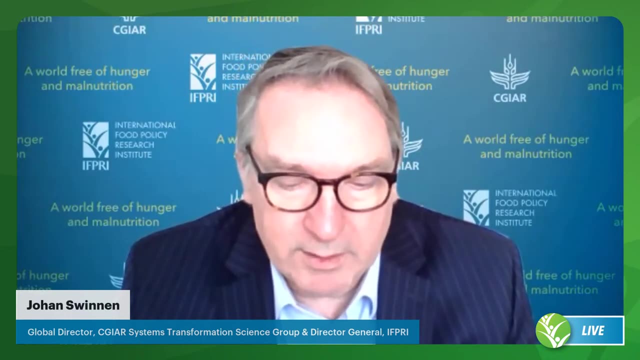 And thank you to all our co-organizers and the participation here today of them. I'm very glad to see Miss Cornelia Burns here with us. She's from the German Federal Ministry for Food and Agriculture and she will present the key results of the GFFA. 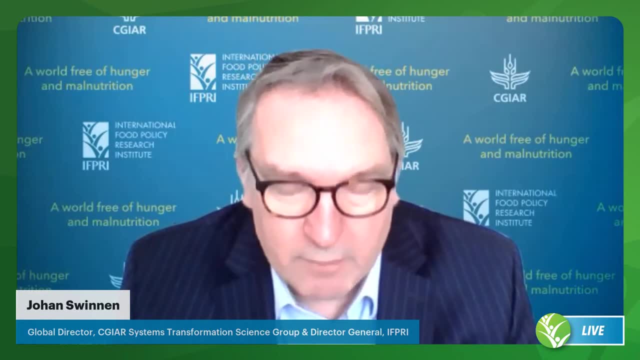 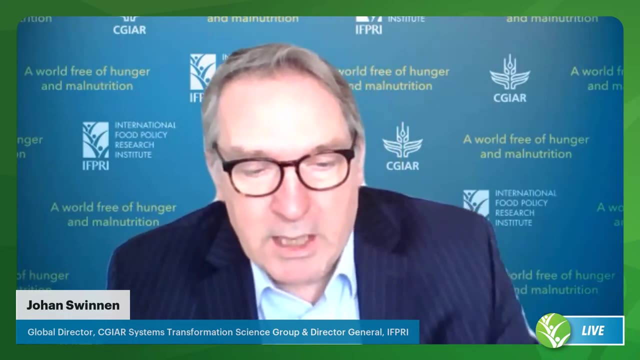 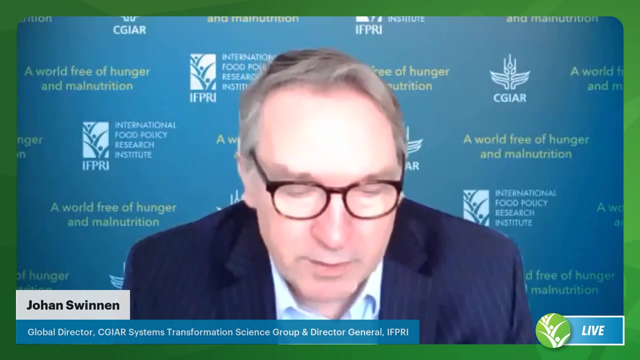 I also want to thank very much Astrid Astrid Jakobs, who we have collaborated with in the preparation of this event and also another cooperation for the Berlin event, The 14th Global Forum for Food and Agriculture. a very successful event, again as it was the previous years, and the topic was extremely 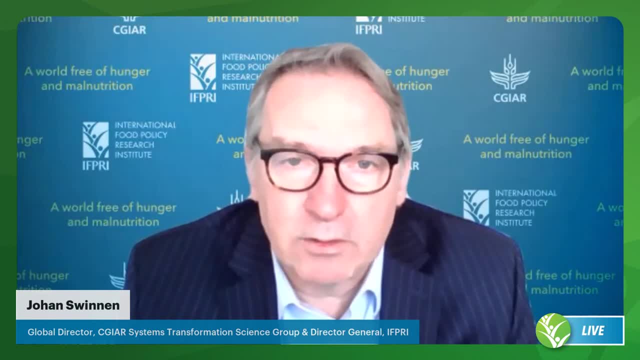 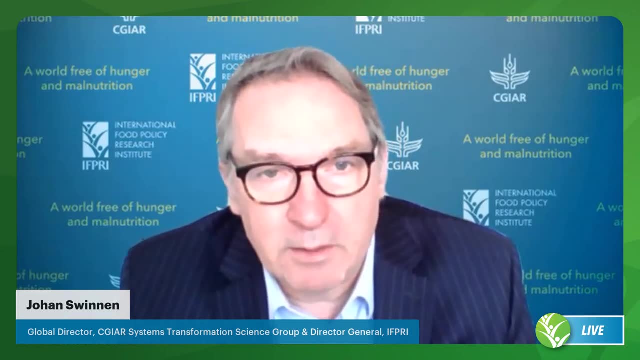 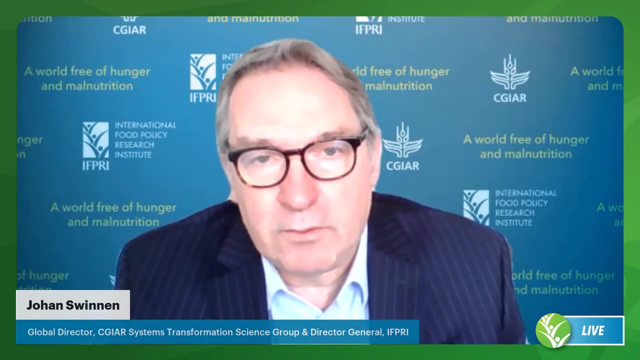 timely. i think we know that land and healthy soils are central to the transformation of our global food systems, and this transformation is really essential to deal with food security, sustainability and a number of other challenges going forward. so it was the focus of the of the conference of. 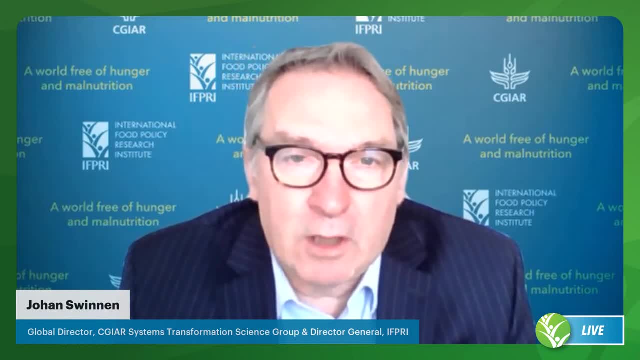 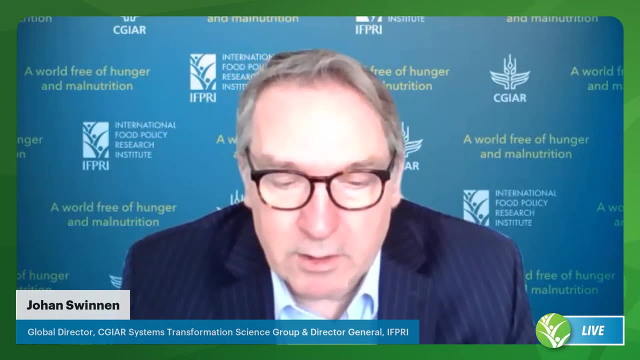 the event was both timely and crucial. we know now that there are no long-run trade-offs between sustainable land use and global food security. if we want to increase our food supply in the long term, this requires that challenges addressed to climate change and biodiversity, for example, are addressed as well. sustainability and productivity of existing production systems. 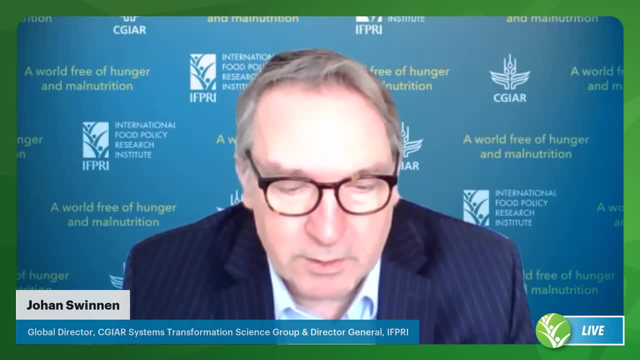 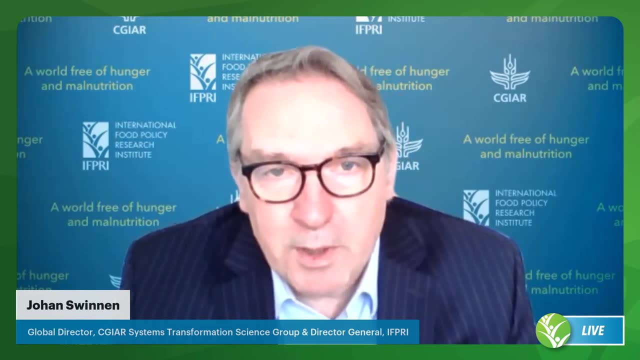 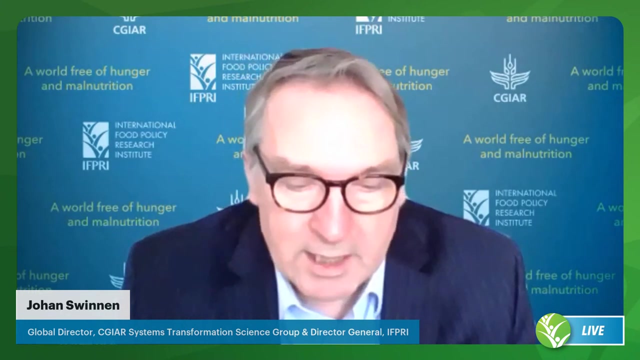 must be increased and, at the same time, degraded lands must be restored. there are actually quite a lot of things that we know how to do better, and this uh knowledge comes from experience. it comes from research, both in practice and in the policy side, or in the policy uh making area. for example, we know that farmers are the stewards of 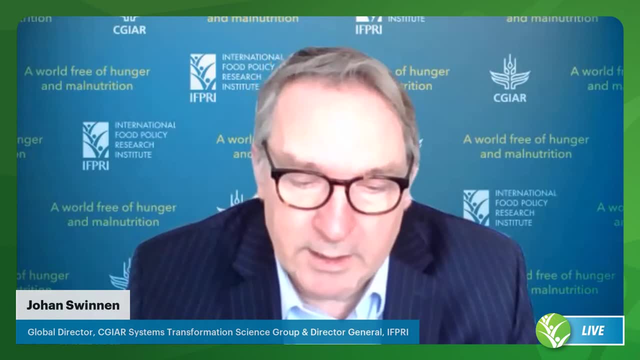 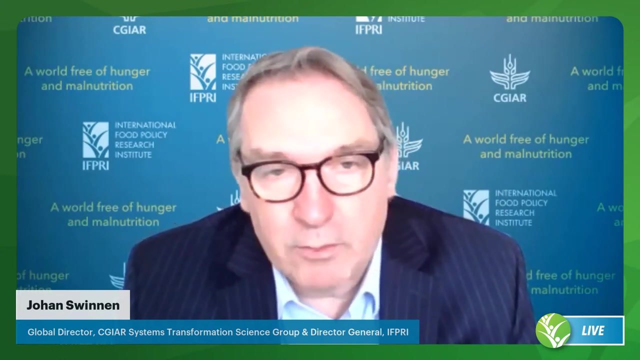 much of the soils on the earth, so they must have an incentive investing in healthier soil, and for this we need policies that support the rural economy and that offer incentives for improved soil management practices. a soil management is a long-term investment. therefore, the policies and the regulations should 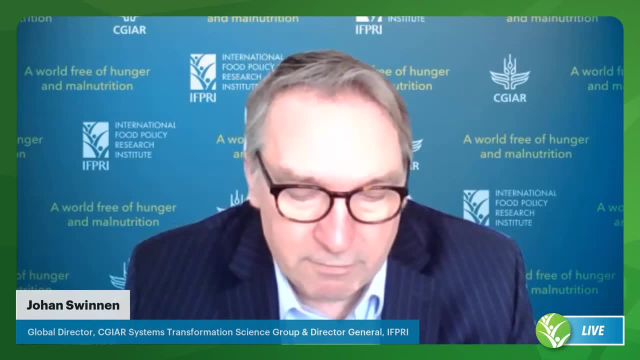 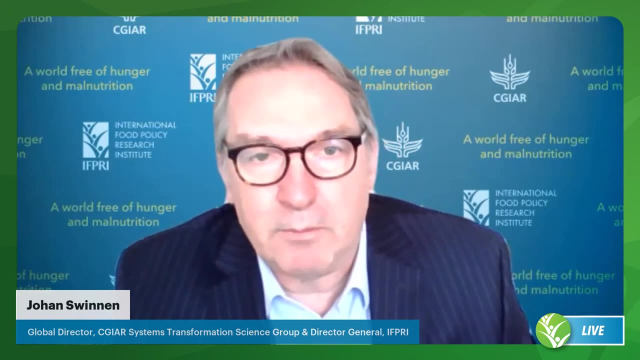 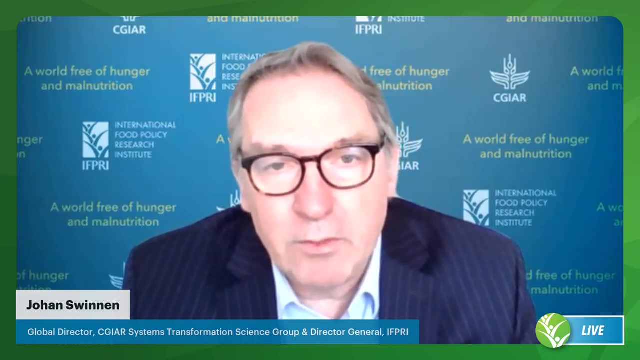 be there to ensure secure tenure and land rights, to give farmers the incentives for better soil management of also to give communities incentives for proper land use management in abroad and common lands. we have to rethink our policy systems for that and i'm really pleased to see a martin. 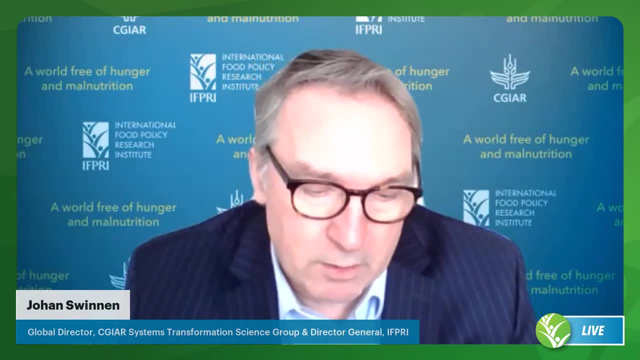 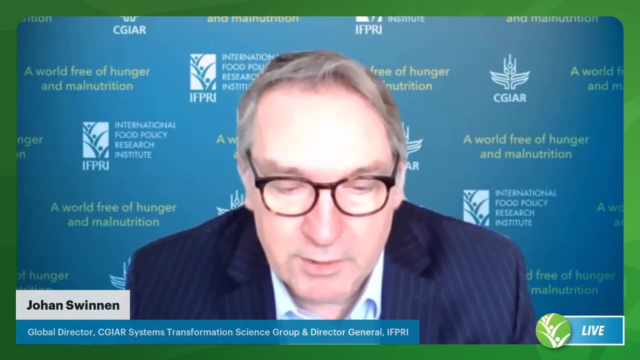 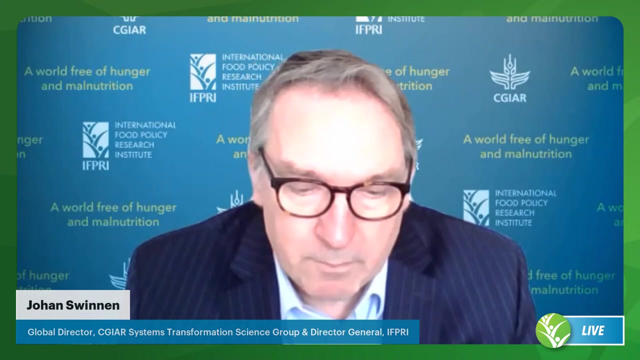 new cop here on the program today. we have worked very closely with martin and the world bank on our rethinking of policy system, particularly the work on repurposing agricultural subsidies, which should help to target investments towards better land management, better soil management, etc. and so in. 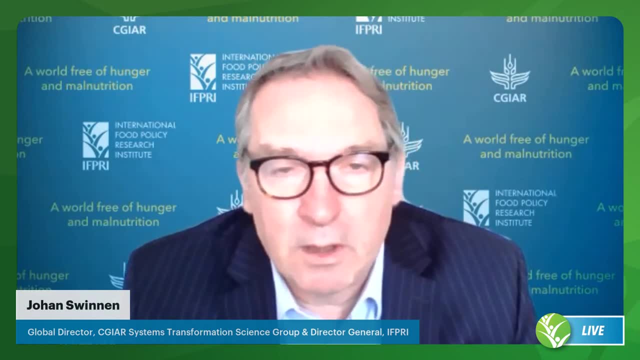 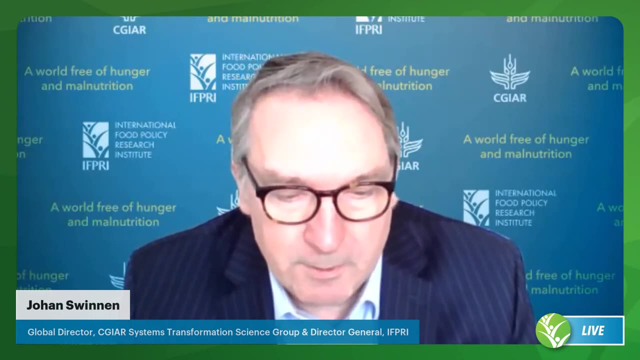 this way we have shown, and we have a report out just now, a few weeks ago, which shows that it is possible to achieve both environmental and economic benefits by repurposing subsidies in many regions of the world. there are large difference between the potential and the actual. 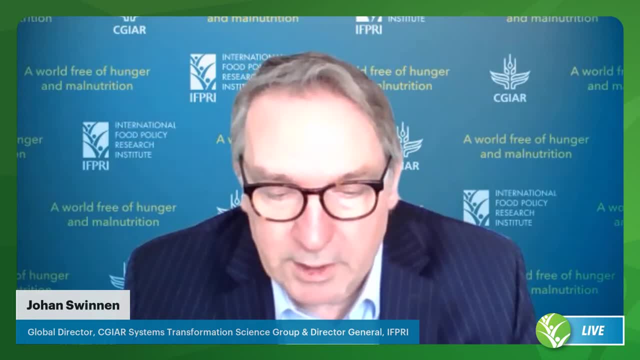 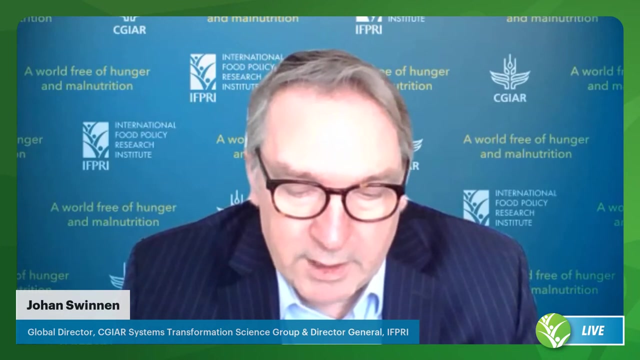 agriculture productivity, promoting sustainable land use, intensification- incredible noch lighted technologies, better practices can improve both crop yields without expanding crop land and while also promoting sustainable land use. but there are also many things that we do not know or do not know well enough, and for this i think we should. 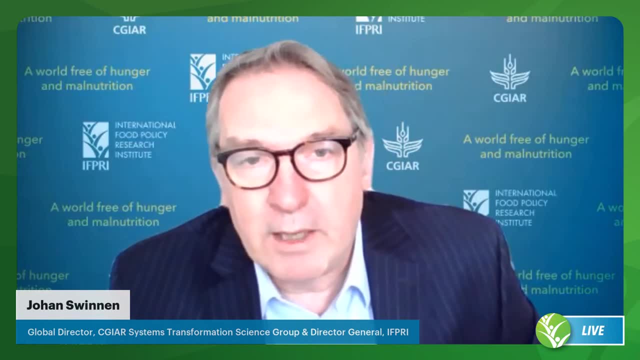 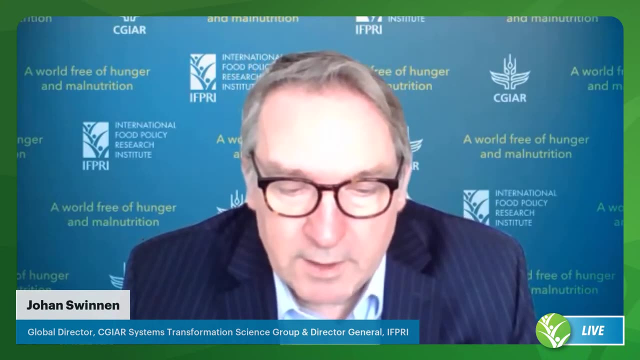 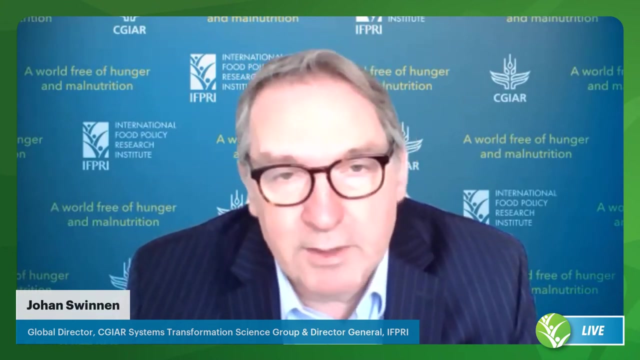 keep until they continue to invest in further research and innovation. to go forward, my organizations- if pre and once eg, ir more broadly, have a mission to deliver science and innovation that advances the transformation of food, land and water systems. we have a new strategy, the strategy. it's an ambitious strategy to provide knowledge and innovation in this field. so we are. 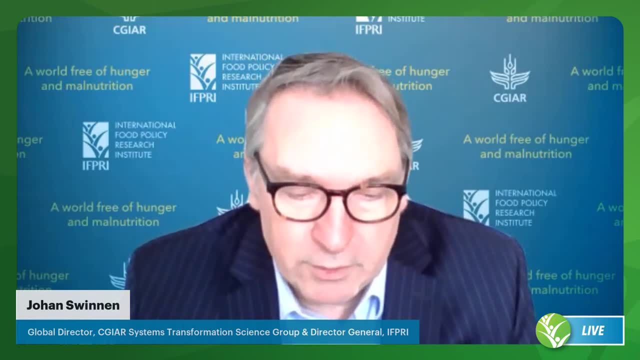 ready to deliver in-depth research to elite to deliver, sorry. we are ready to deliver in-depth research to achieve ecological, economic and social sustainability. in conclusion, let me again congratulate the organizers of the gffa. i think it was an important and timely platform for international discussions with various stakeholders. it provided a great opportunity for all the 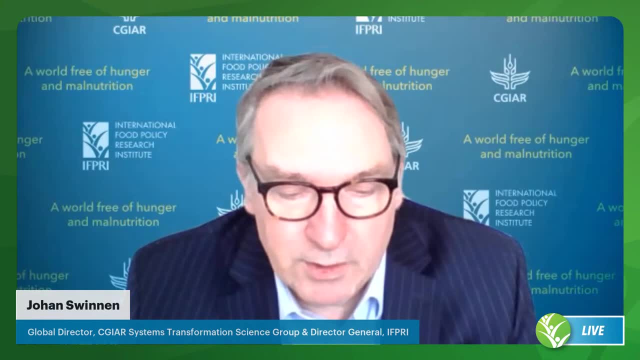 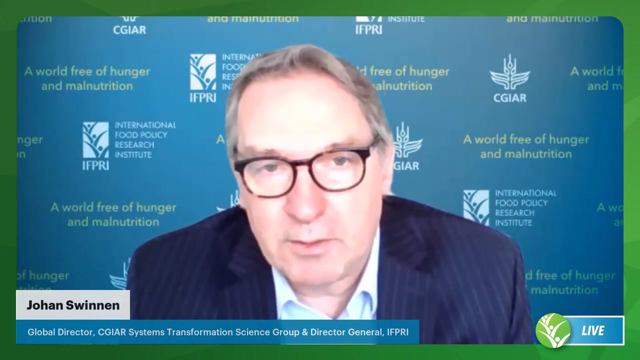 participants to share findings on best practices and lessons, to raise awareness on the urgency and the importance of sustainable soil use and to provide evidence-based advice to the policy decision-making process. so congratulations again. i really look forward to the summary that mrs burns will give on the findings, the key conclusions of the gffa, and also to the panel discussion we 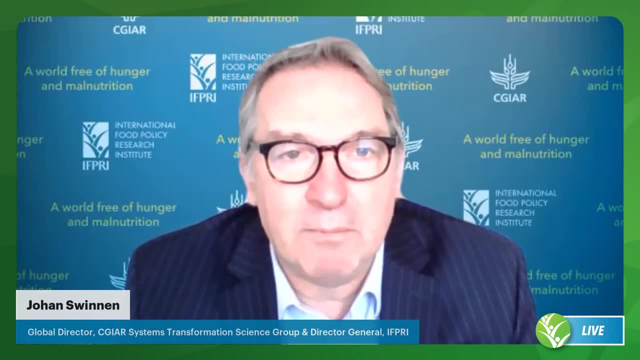 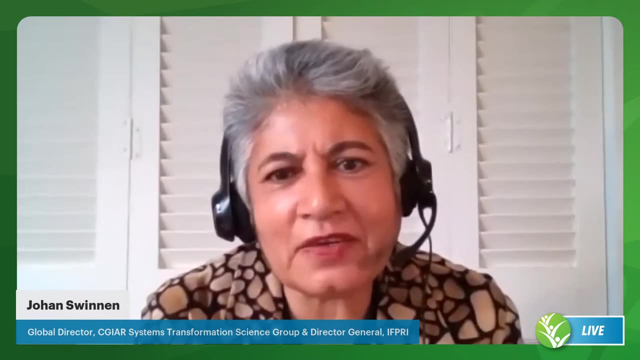 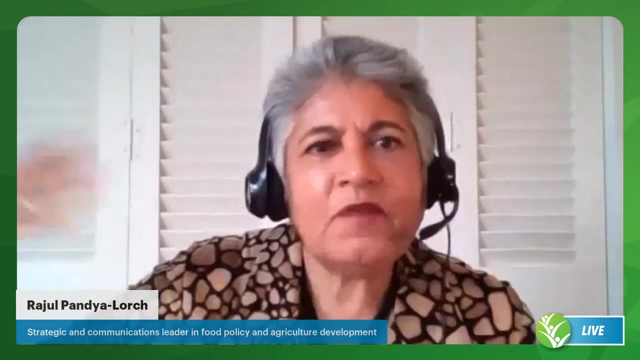 have excellent speakers on the panel, so i really look forward to hearing with that back to you. excellent. thank you so much for your remarks here and setting the context and, like you, i'm absolutely delighted we are continuing this annual tradition of co-hosting an event at the embassy in washington to further. 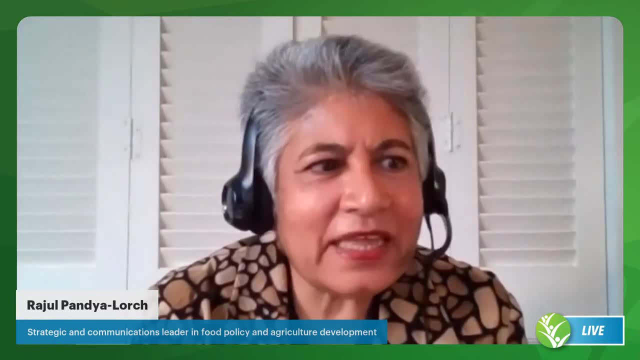 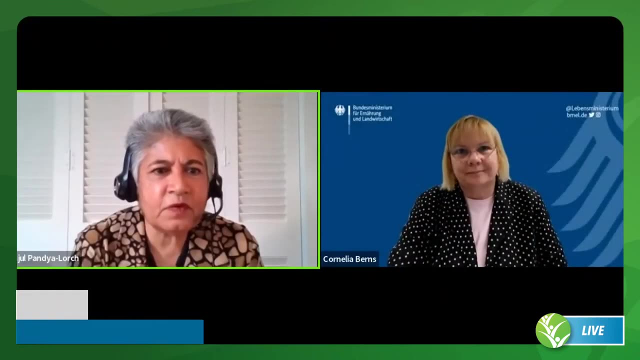 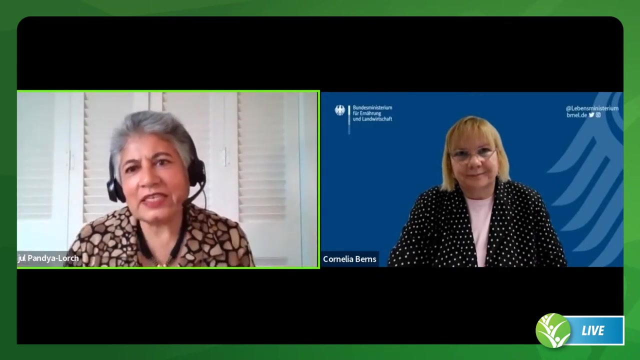 follow up on the findings of the gffa. with that, let me now call upon miss cornelia burns, the deputy director general of the german federal ministry for food and agriculture. cornelia, we're eager to hear more from you. what is the gffa and what are the results it has achieved? 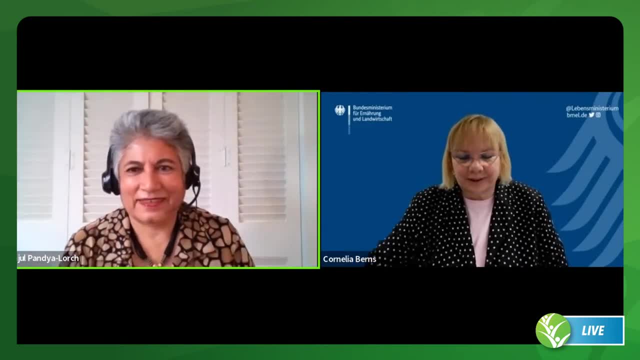 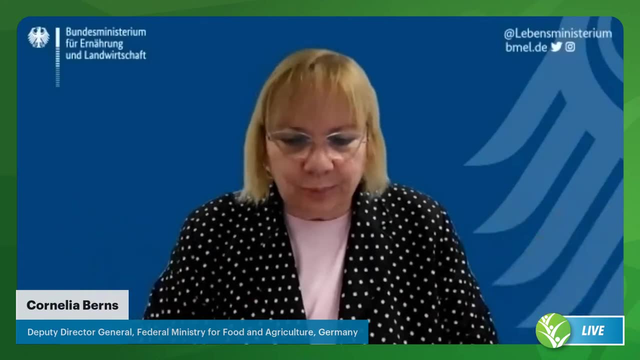 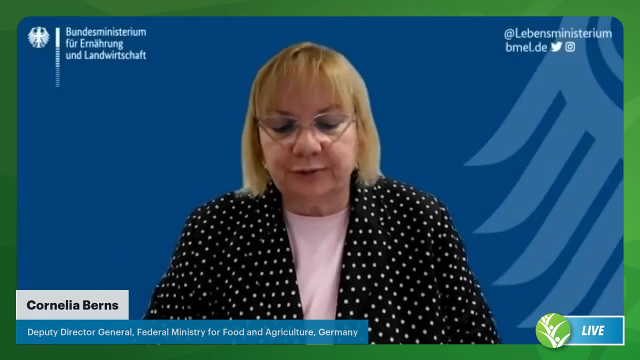 so i'm going to turn it over to you, cornelia. thank you very much for your nice introduction and thank you very much for inviting me to this event. yeah, the, the global forum for food and agriculture, the gffa, was hosted by the german federal ministry of food and agriculture for the 14th time in 2022. 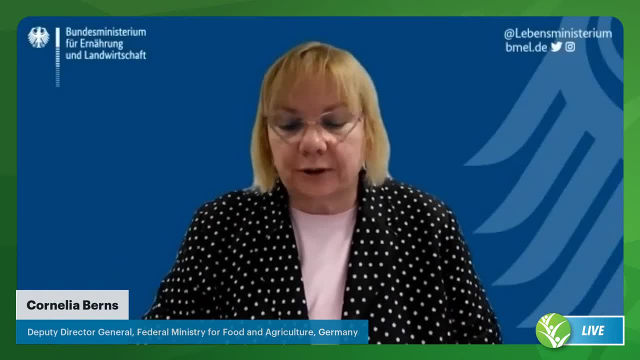 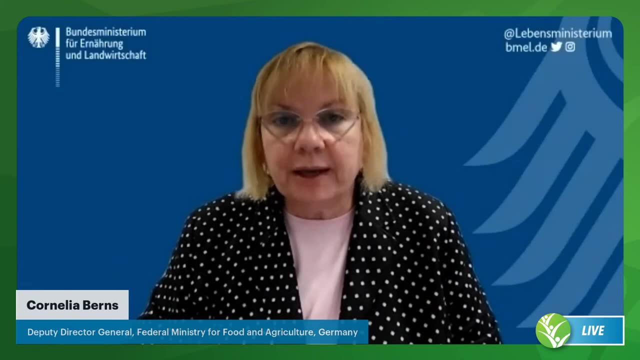 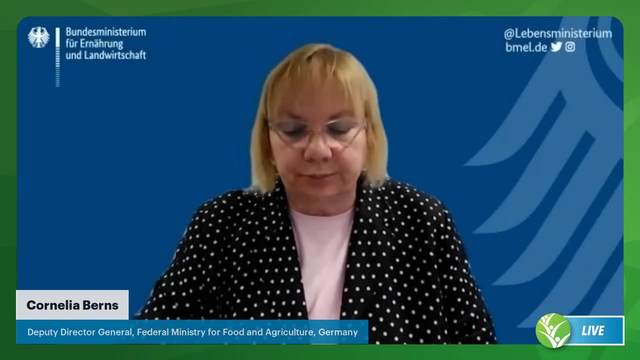 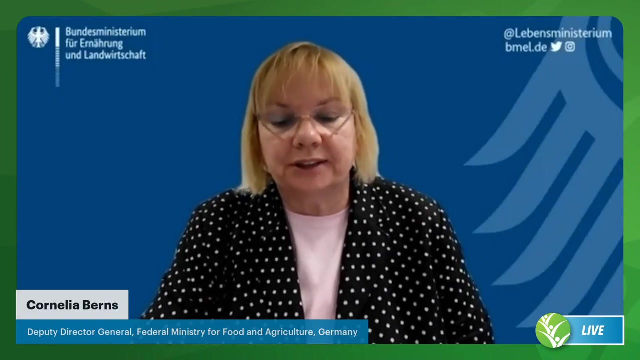 it has evolved into the, the international conference on key issues regarding the fusion of food and agriculture and the future of the global agri-food sector. its climax is the agricultural ministers conference, the world's largest informal conference of agricultural ministers. this year, 68 ministers and 11 international organizations participated. live streams were accessed more than 10 000 times. 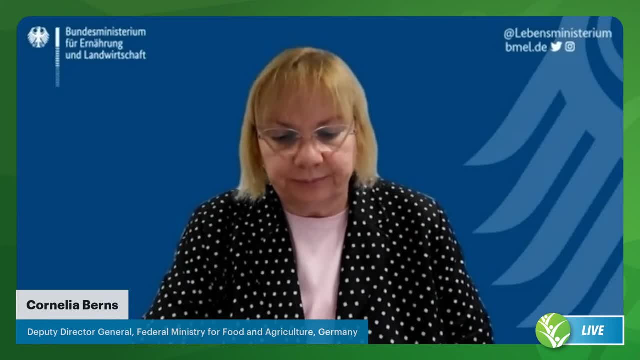 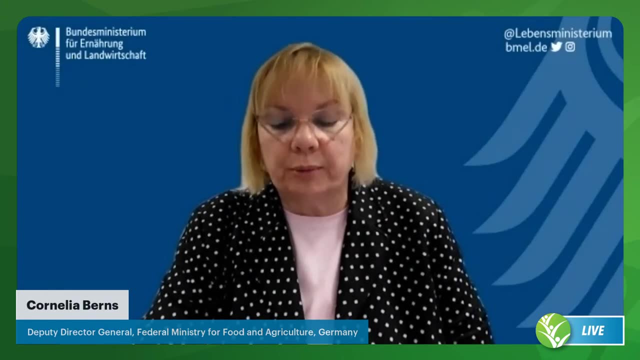 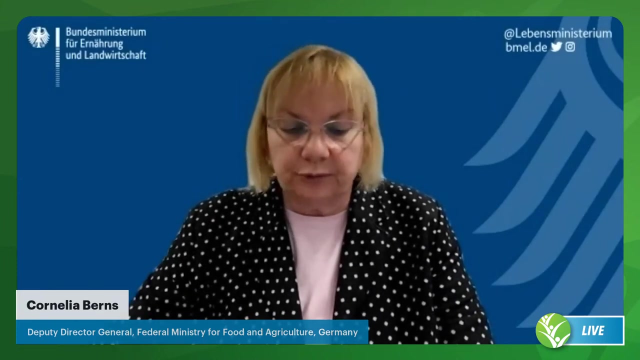 from 125 countries and the gffa. we are driven by the fact that around 800 million people around the globe are still afflicted by hunger and over 2 billion people lack access to adequate food. in order to solve this problem, we need global responses for sustainable food systems of the future. the question of global 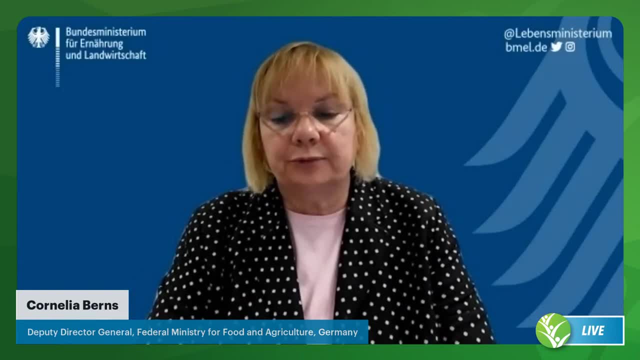 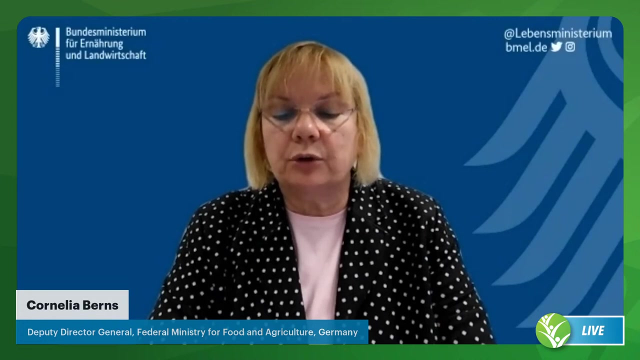 food security is therefore at the private of agri-food sector. every gffa. every year, we dedicate the gffa to a priority topic that must make a key contribution to global food security. in recent years, these topics have included international agricultural trade or climate issues and their contribution to global food security. 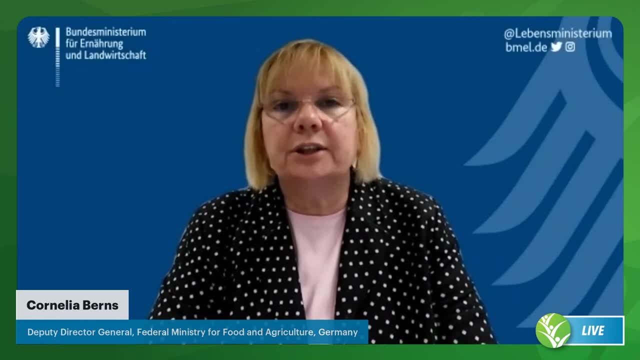 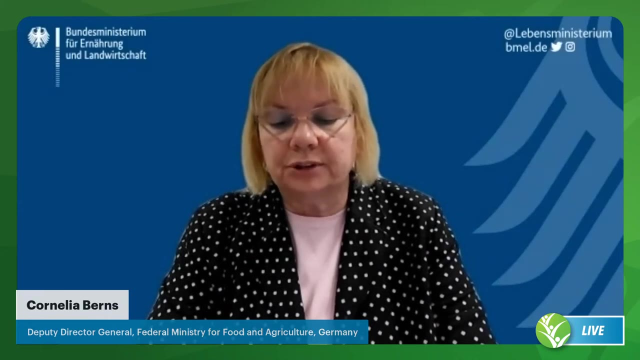 this year, we choose the topic of sustainable land use. food security starts with the soil. more than 90 percent of global food production depends on soil. soils provide habitats for soil organisms, purify and store water, filter pollutants, and they are the earth's most important to terrestrial carbon sink. however, soil quality 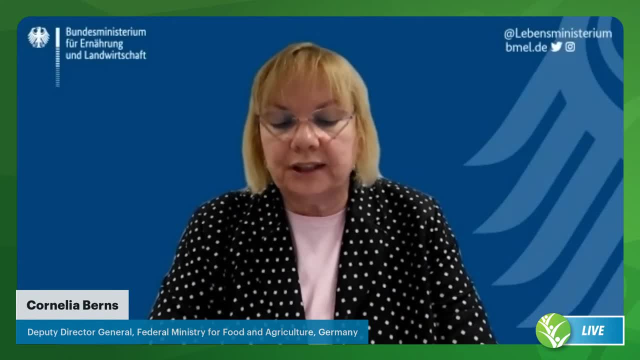 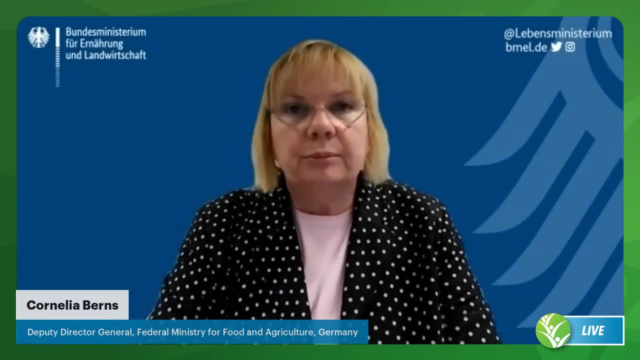 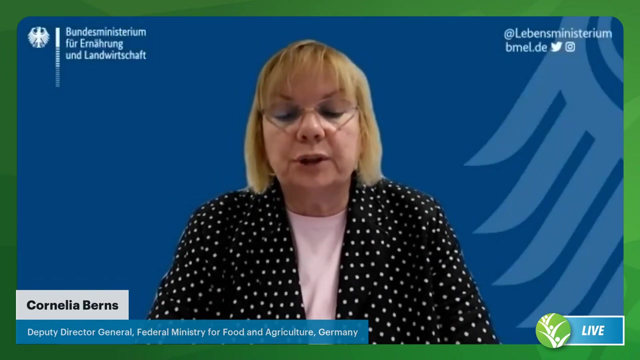 is increasingly deteriorating and fertile land is becoming more scarce. the causes for this include soil sealing, but also the loss of land due to the sea level rise and desertification. meeting the united nations goal of achieving a world without hunger by 2030 will only be possible if we succeed in protecting our soils, only if we utilize land resources sustainably and preserve existing agricultural land, we will be able to feed the growing, growing global population, keep global warming below two degrees and reduce the loss of biodiversity. the ministers and the 2022 gffa therefore discussed the following questions: how can we improve soil protection? how can we restore degraded soils? how can we reduce? 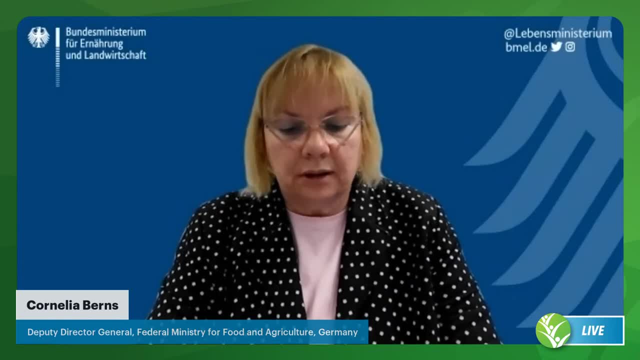 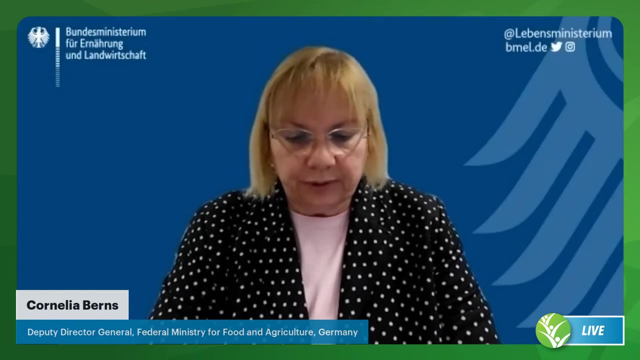 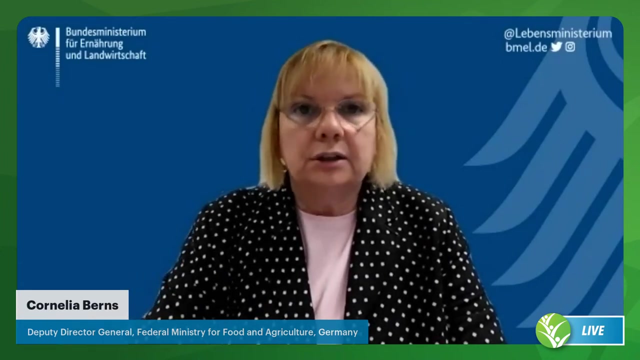 the natural environment. we can preserve the natural environment. we can preserve the natural environment, make the use of finite land resources more sustainable, and how can farmers worldwide get fair access to land? which results have been achieved? the most important conclusions of the final communique can be summarized as follows: soil as a scarce resource and the 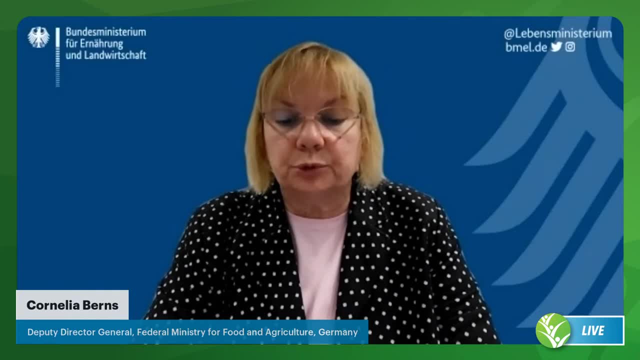 foundation for terrestrial ecosystems and agricultural production must be protected. climate change mitigation and adaptation must be advanced, soil being a valuable instrument for both. soils can store significant amounts of carbon, and soil that is rich in organic matter can store more water. for dry periods, it is particularly crucial to reduce the cost. 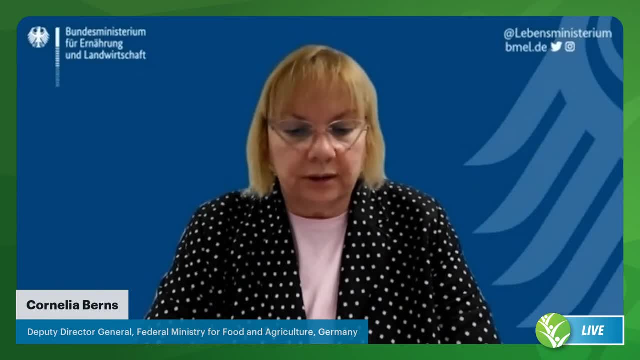 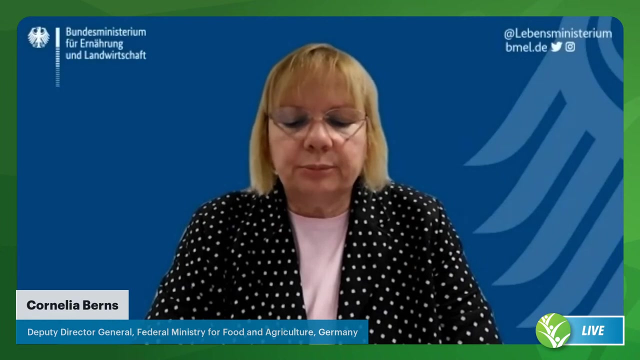 of carbon dioxide emissions of drained moorland soil. biodiversity is a prerequisite for healthy soils. in turn, healthy soils are also rich in biodiversity. the ministers therefore want to promote agricultural practices that serve this purpose. examples include an adapted nutrient supply and the responsible use of organic matter, and the use of organic matter as a source of plant protection products. another important contribution to protecting and improving soil biodiversity is organic farming. as global land resources are limited, they need to be managed sustainably. this entails minimizing land take and restoring degraded land for agricultural use. the progression of decertification is alarming in this situation. 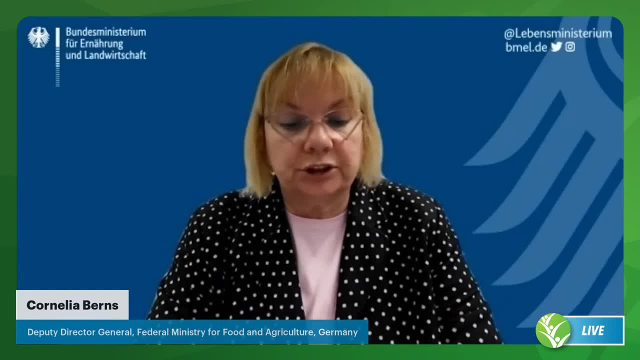 in this regard, site adapted measures, such as the restoration of productive and biologically diverse landscapes, are necessary. one example is africa's great green wall. the ministers also underline the great significance of ground cover through forest and grassland as protection of soils against erosion. their protection should also be supported by responsible agricultural. 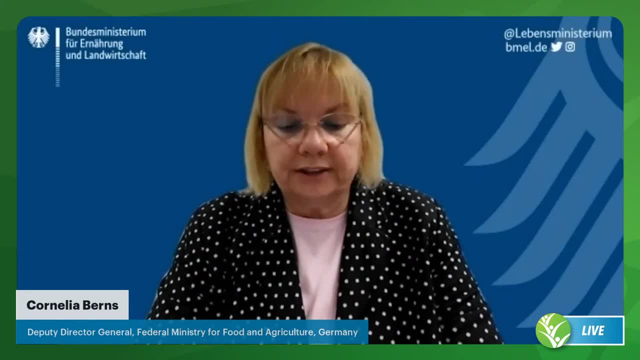 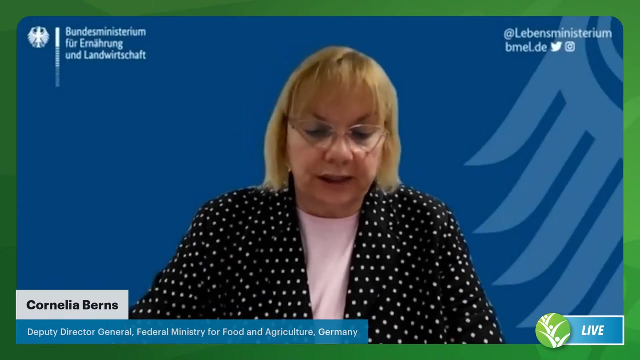 supply chains. long-term and secure tenure rights promote a careful handling of soils. they are a central contribution to food security. farmers must be able to gain access to land which is necessary for farming. all people should have non-discriminatory access to agricultural land. the ministers underlined the importance of the 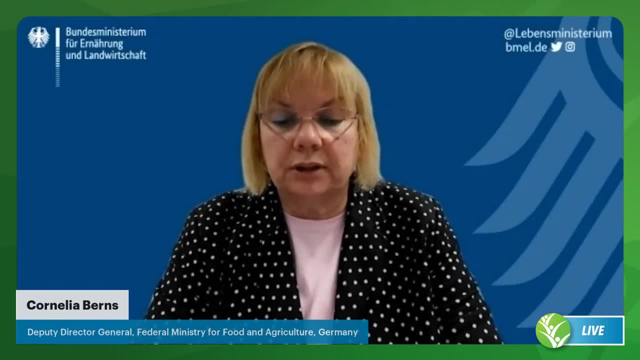 land on both sides of the aquifer, and the person is a good example of the great land users must be able to obtain the land, which is the most important resource for ability for growth and storage of land. thesequently, we must have the right to preserve and protect. 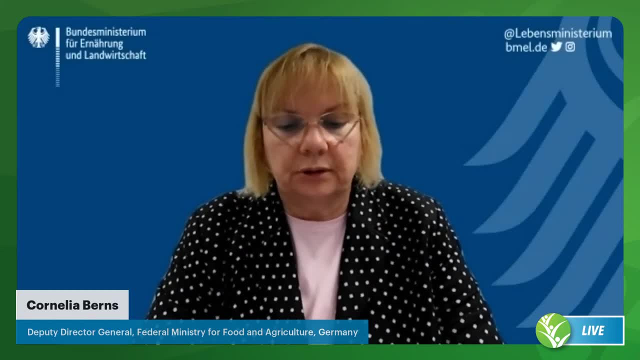 the land and protect it in the best possible and the best possible time for the development of new food. Until the end of last year, we have not been American farmers by the way of the 20th century. for the first time, the European Union for the participation of 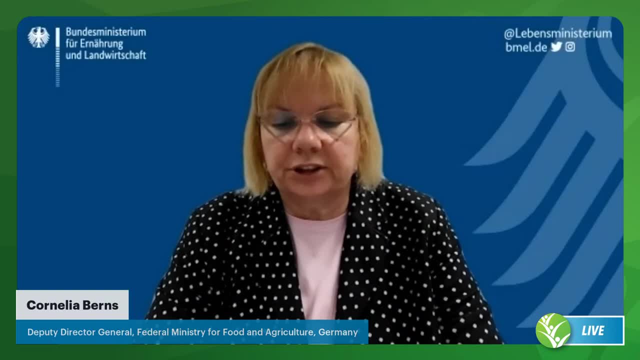 the European Union, were a major factor in the climate change of the world, and the climate change of the world has been a major issue for our country and we need to continue to do this. we must not forget that we also need to address the problems in the climate change. 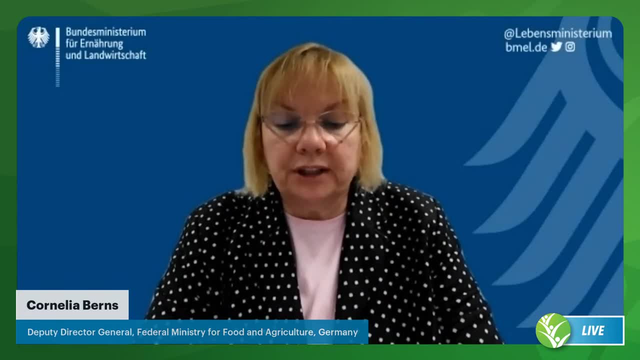 of this very muchuel and what the climate does is to implement new economic rights, and we must ensure that all the issues that we create are not Halal decisions. resilient and sustainable food systems must be supported on a global scale. we do not have much time left if you want to meet the united nations goal of achieving a world. 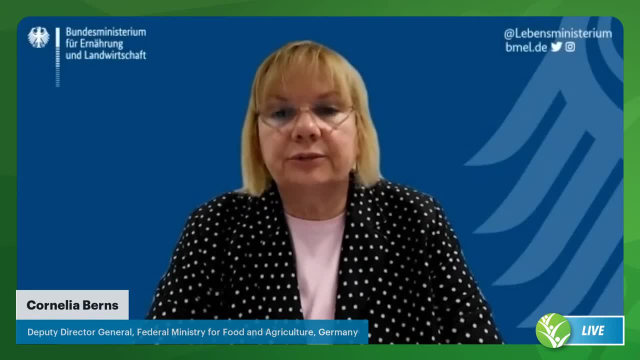 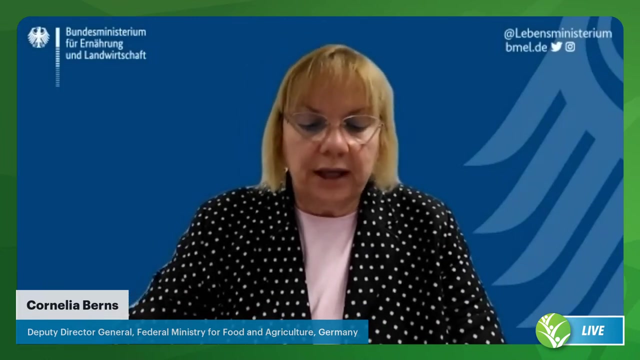 without hunger by 2030.. this is a difficult pathway, also because we must achieve the other sustainable development goals at the same time. the international community now needs to put the constructive suggestions of the final communique into practice, each country for itself, but also united fao, the global soil partnership, the secretariat of the united nations. 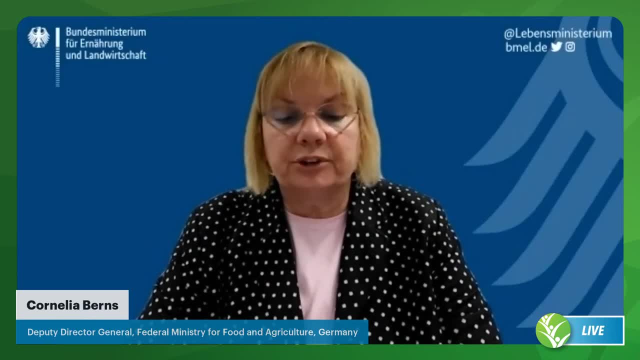 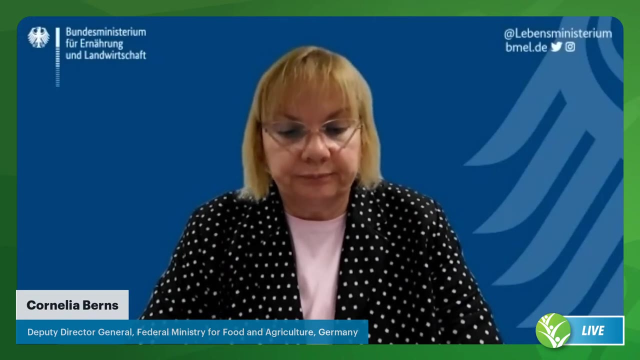 convention to combat desertification and the committee on world food security have taken the mission to the day-to-day business. The UNCCD is planning to include the communique in their conference of the parties in Abidjan, Cote d'Ivoire, in May. Last year's UN Food System Summit has 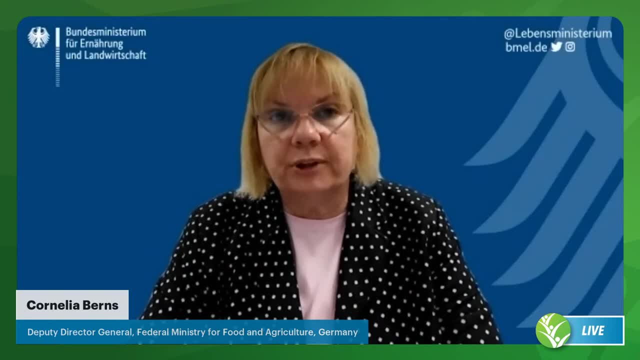 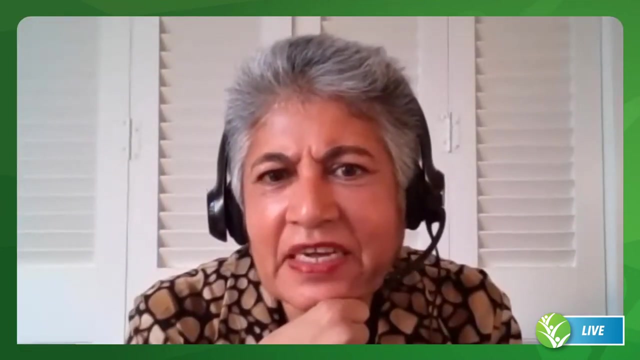 given us no less than the impetus to transform the entire food system, a goal we were supposed to achieve by 2020.. Let's finally make a start. Thank you very much. Thank you very much, Cornelia, for that comprehensive and compelling overview of the GFFA, and what 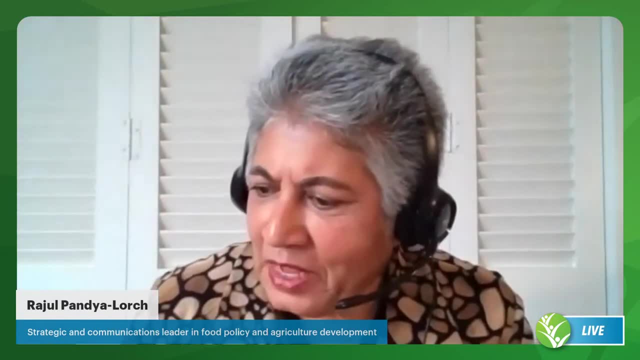 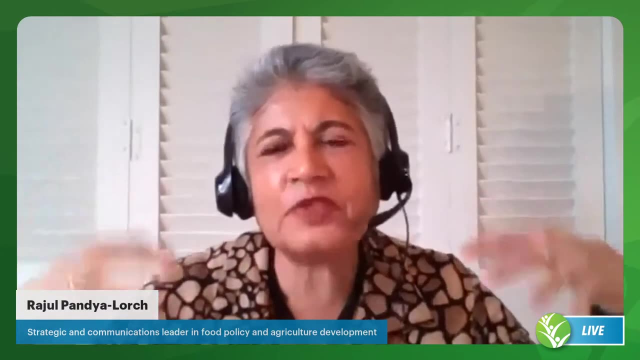 it focused on and what it sought to achieve. We are, of course, all eager to know what will be next year's topic, because this is such an important spotlight that the GFFA puts on a topic, as you say, of a priority for global food security, And it's important. 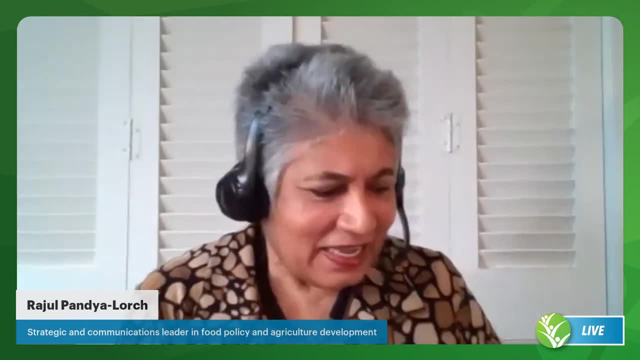 that you do that, So we'll come back later in the Q&A on that. Colleagues, before I move us to the presentation, I'd like to thank all of you for joining us today. Thank you very much, Cornelia, for that comprehensive and compelling overview of the GFFA, and what it focused on and what it sought to achieve. We are, of course, all eager to know what will be next year's topic. We are, of course, all eager to know what will be next year's topic, And it's important that you do that, So we'll come back later in the Q&A on that. 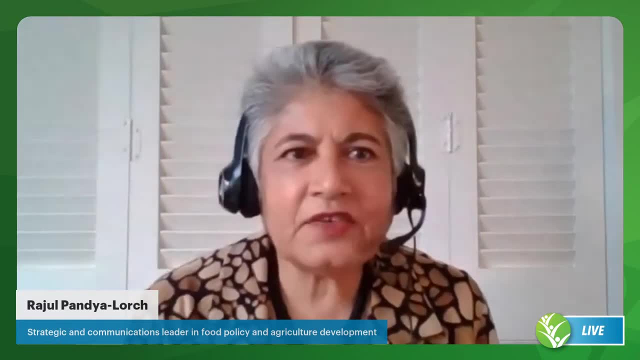 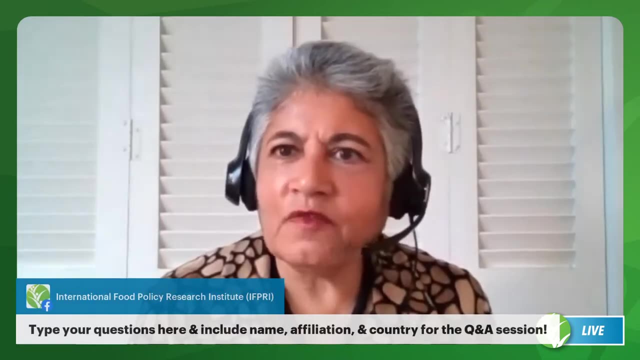 Colleagues, before I move us to the presentation, I'd like to thank all of you for joining us today, And we have an incredible panel discussion ahead of us. I'd like to remind all of you joining in that you can submit your brief questions in various platforms: on iffreeorg, on Facebook. 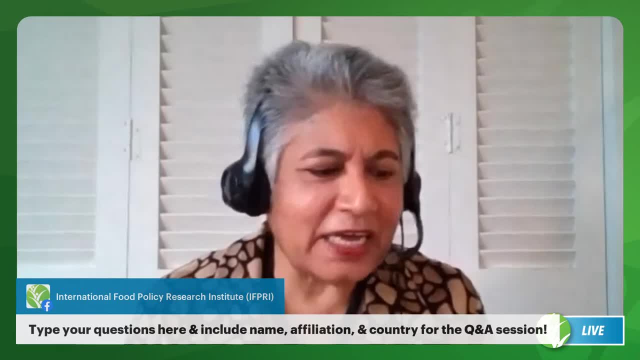 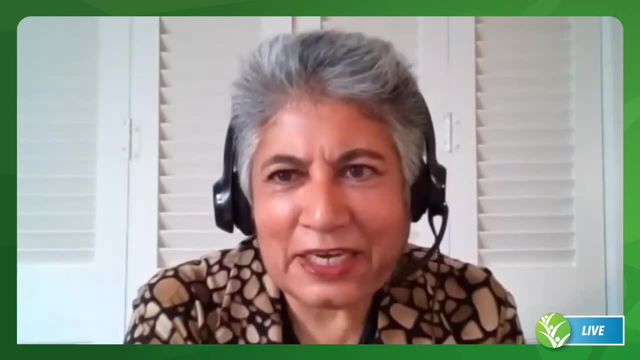 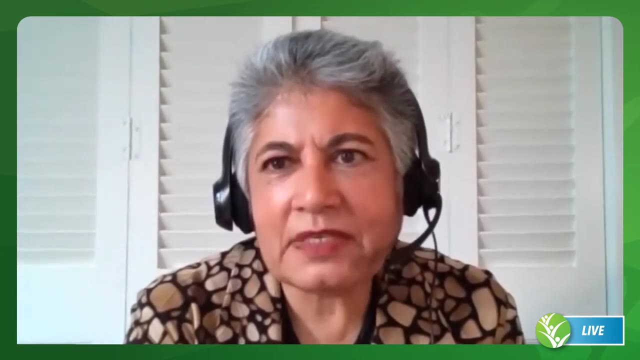 on LinkedIn, on YouTube or on Twitter through the hashtag AskIFFree. So do not be shy, Go ahead and do that. So we do have a fabulous panel discussion lined up, And we will begin with scientific perspectives and then move on to national policy perspectives. So thank you very. 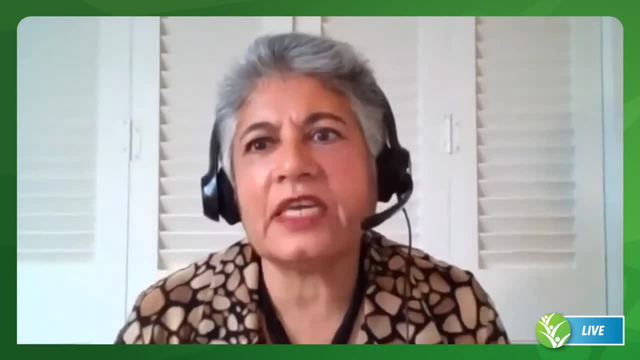 much, Colleagues, for your active input And I'd like to turn it over to you, Colleagues, to give you some perspectives- and international organization perspectives- on how we can move this agenda forward. I would like to call on our first panelist, and that is Professor Ratan. 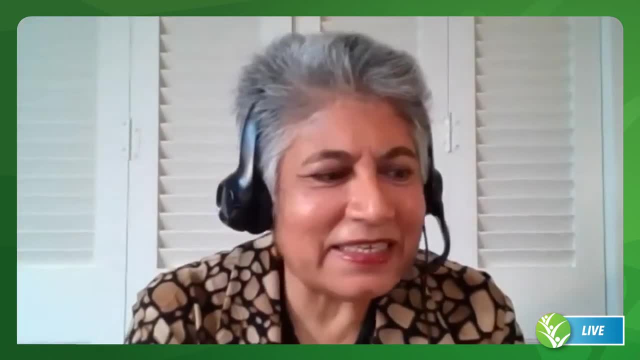 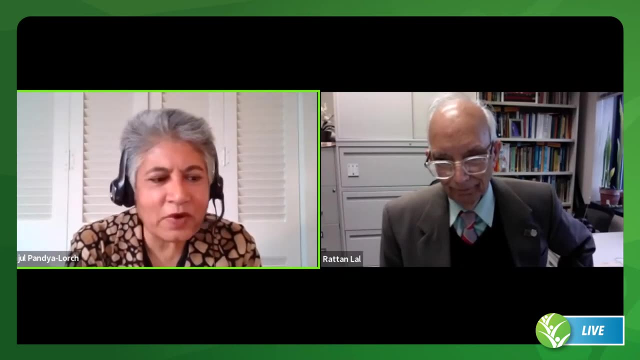 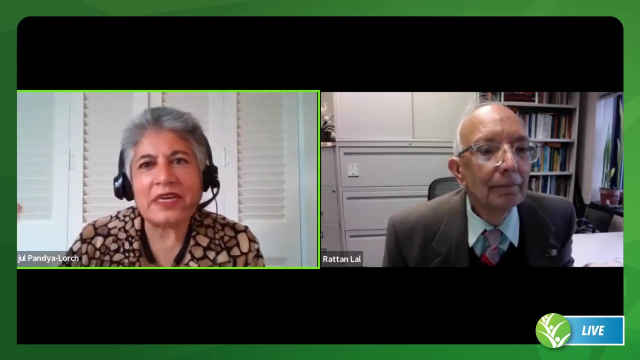 Lau, who is well known to all of us. He is the Distinguished University Professor of Soil Science at Ohio State University. He's also the 2020 World Food Prize Laureate, And if I was to continue and give all the various stories of his bios, our event would be over, So forgive me. 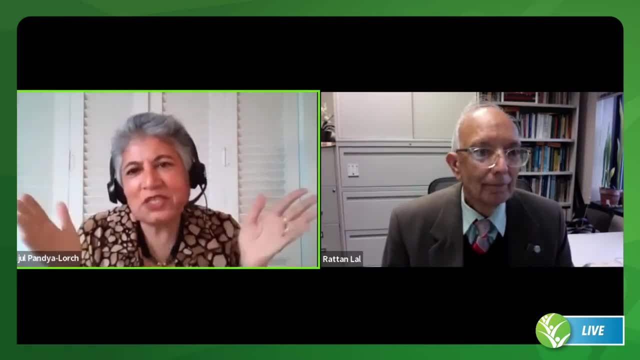 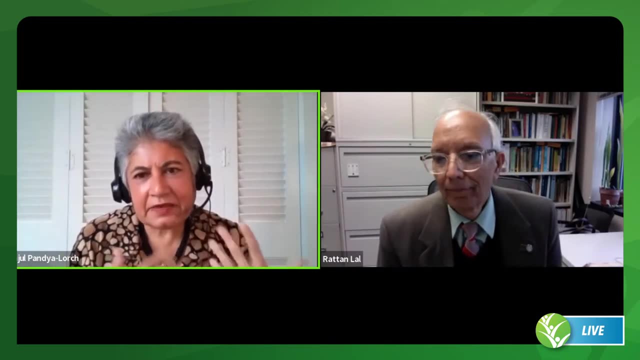 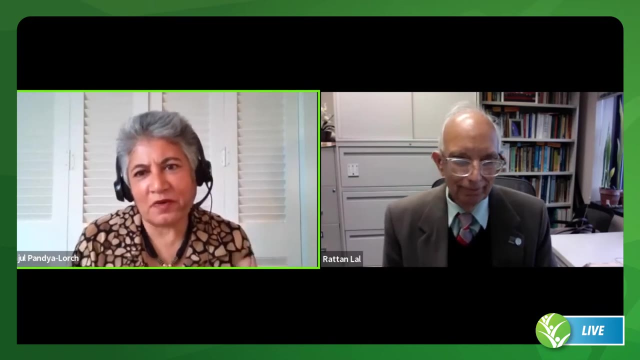 Dr Lal, that I will give you the chance to tell us more about why are soils so important and what are some key, scientifically proven best practices for sustainable soil management. What is it that we know Over to you, Professor Lal? Thank you so much for inviting me, and I'm really grateful. 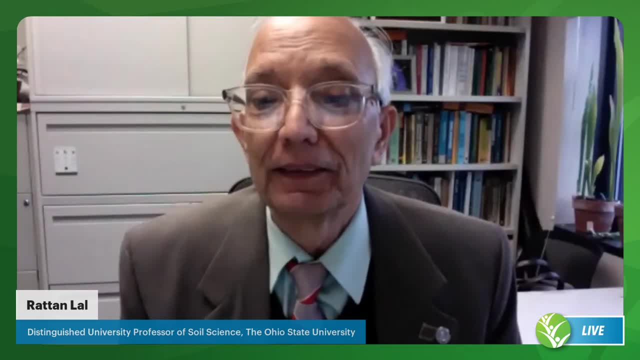 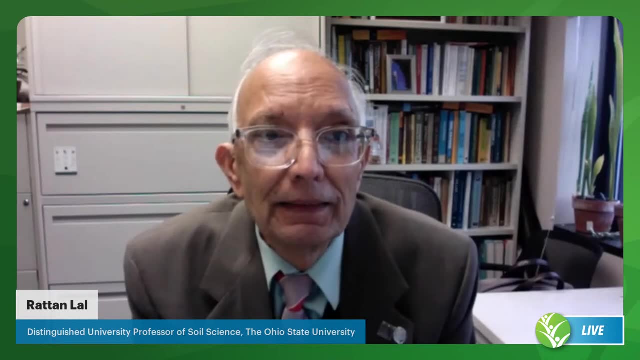 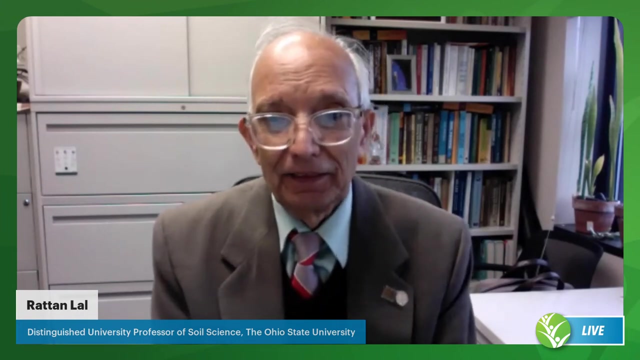 to IFPRI and the German embassy for organizing this program. Soil is the essence of all terrestrial life. There's no life without soil and no soil without life. They have evolved together, So soil is the basic component of our life. If I may go step further and indicate that at the soil root here. 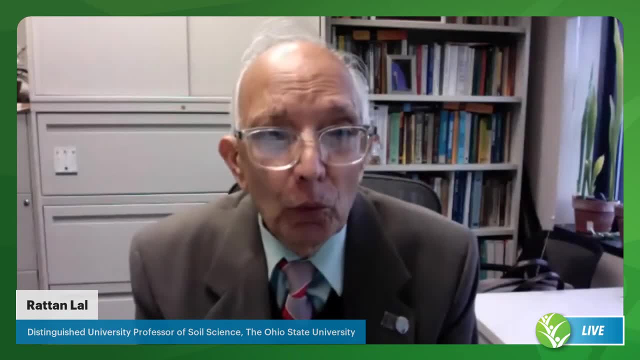 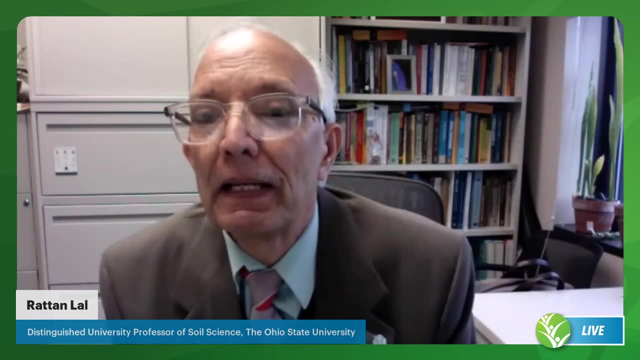 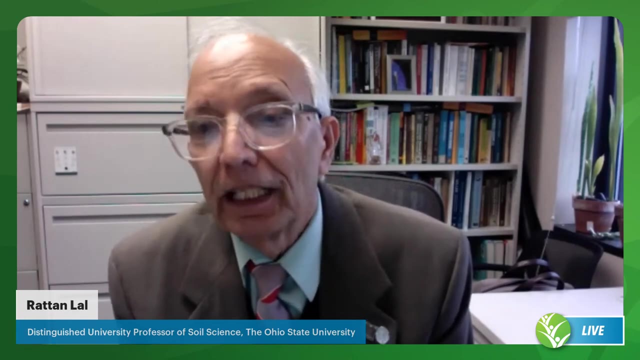 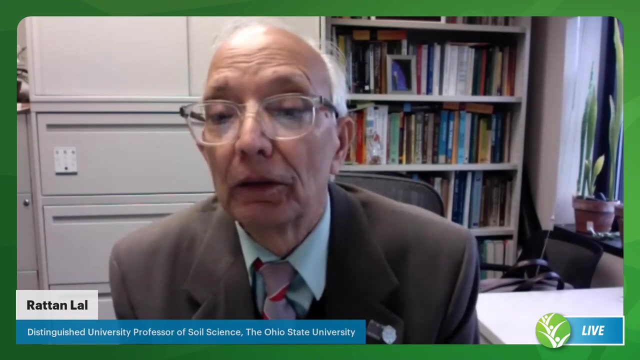 interface at a nano scale is that soil is the only proven entity where death is resurrected into life. so it is that essential. soil is also essential to climate change. Before agriculture began, the carbon stock in the atmosphere was 360 gigaton. Since agriculture to pre-industrial revolution, the carbon stock 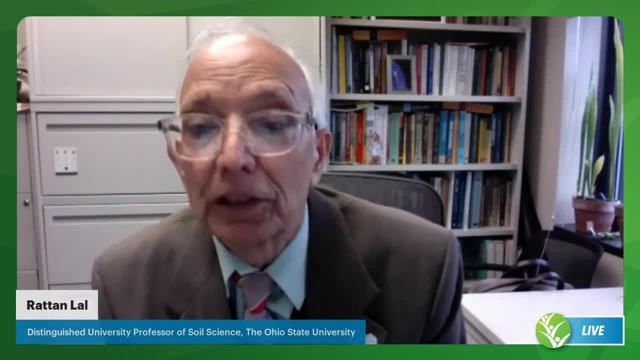 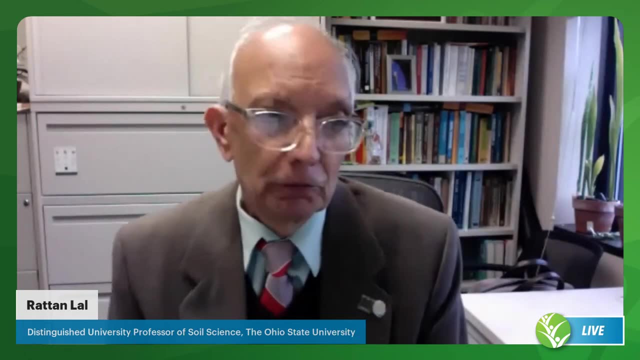 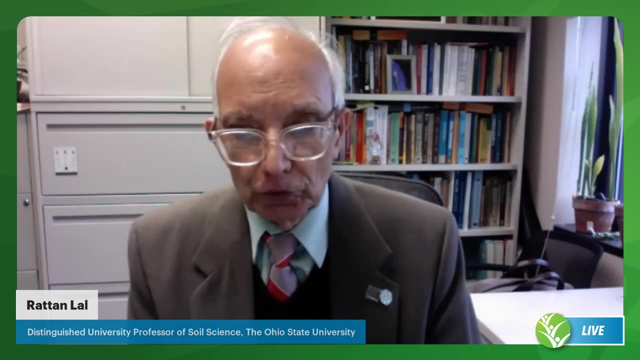 increased to 560 gigaton. 200 came from land use conversion and at present it is around 560. gigaton is 880 gigaton and quite a lot of it's coming from soil and we can put back into the soil. that's another reason why soil is important. the question of food security was mentioned. 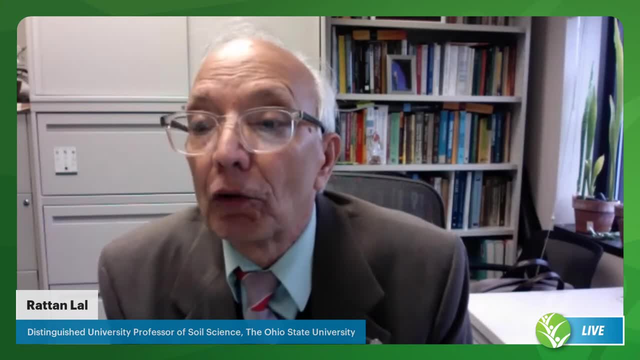 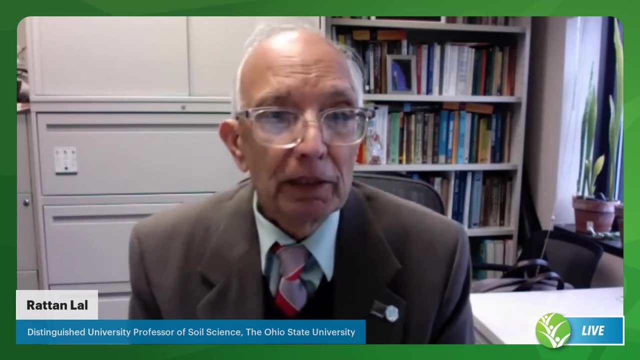 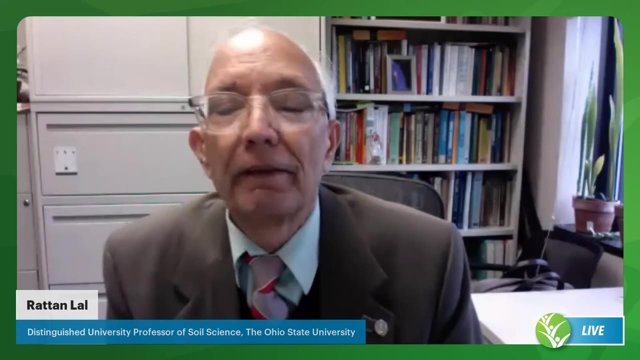 the way food is produced and consumed affects the health of soil, plants, animal, people, ecosystem and the planet. above all, the sustainable development goals for next eight or nine years, i think, are in jeopardy if the soils are not properly addressed. the question of under nutrition was brought up this morning. i would like to state an old saying. 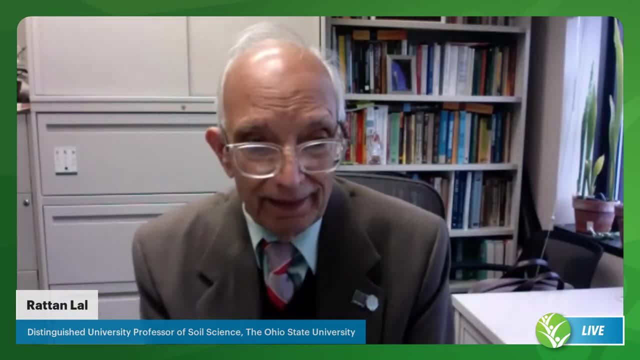 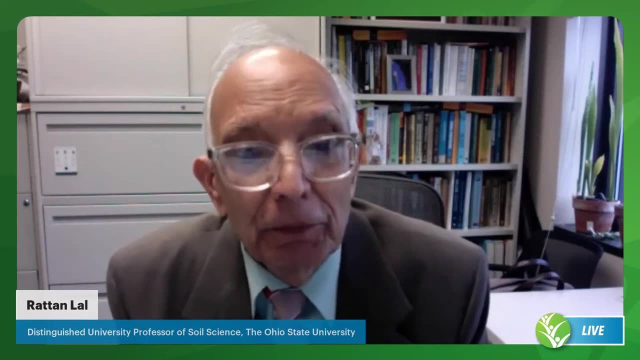 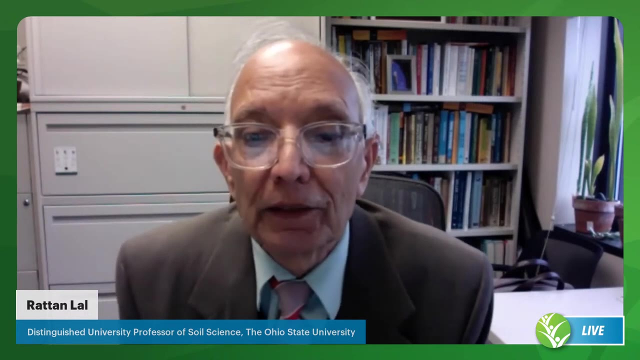 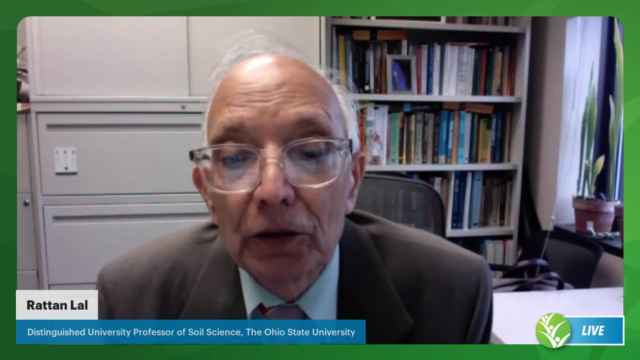 when diet is correct, medicine is of no need, and when diet is wrong, medicine is of no use. and correct diet come from healthy soil. we must never forget it. the question is asked: what are the better agricultural practices? i will first like to indicate better agriculture processes. for example, we are degrading soil because we are depleting nutrients. we are 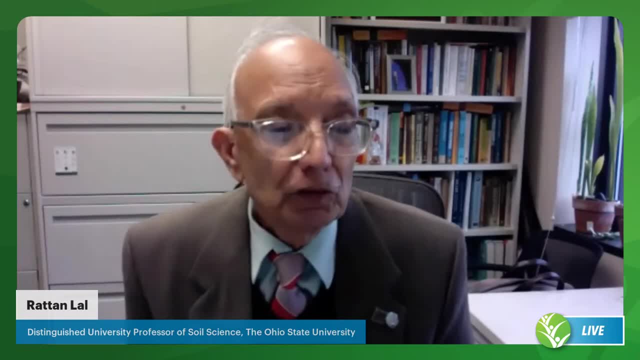 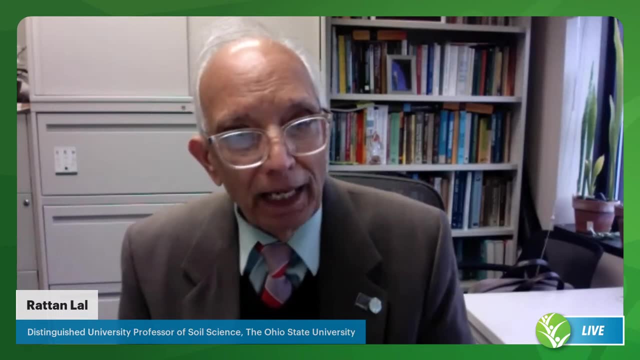 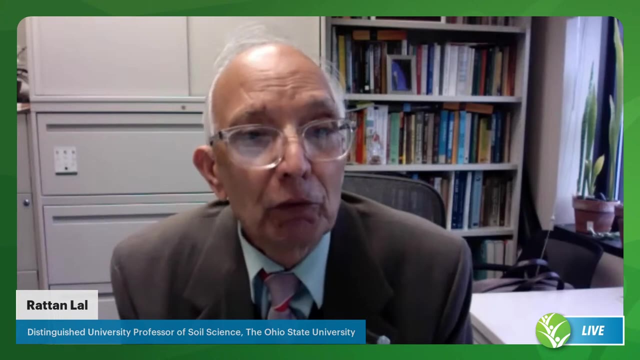 removing the soil from nature. we must return some soil back to nature rather than bringing another 500 million hectare of natural system to agriculture. if we do agriculture properly, by 2050 we should return some land back to nature, but 2100, i think as much as a billion hectare or more could. 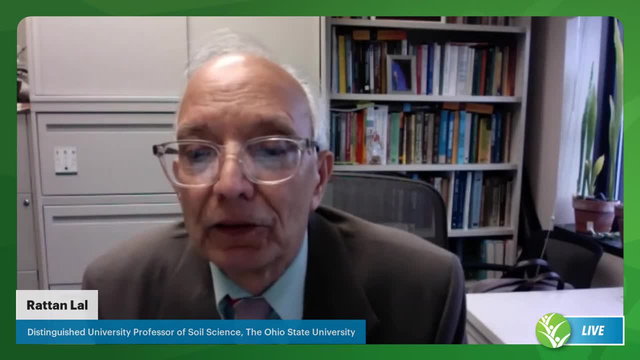 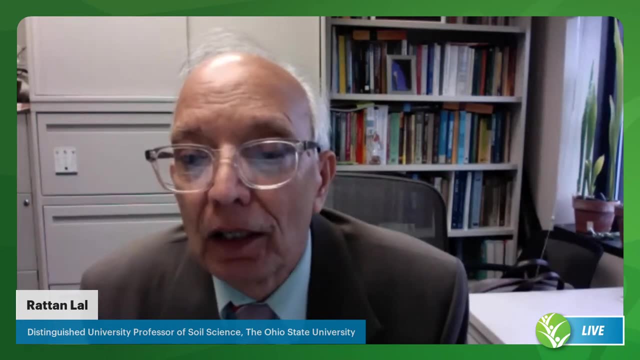 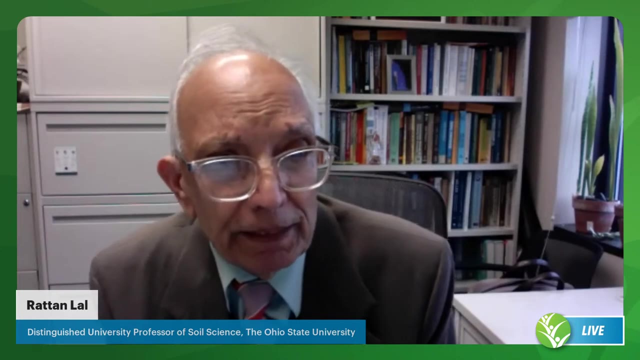 go back. so what are the practices? conservation agriculture, regenerative agriculture, agroecology, agroforestry, integration of crops with trees and livestock, practices which create a positive soil ecosystem. carbon budget: a slogan of cnpk- c for carbon rather than npk if we focus on c. the need for 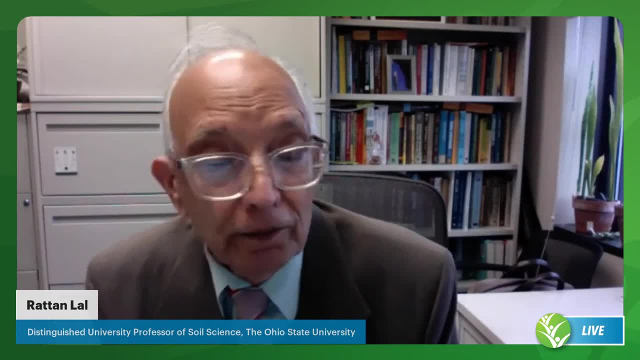 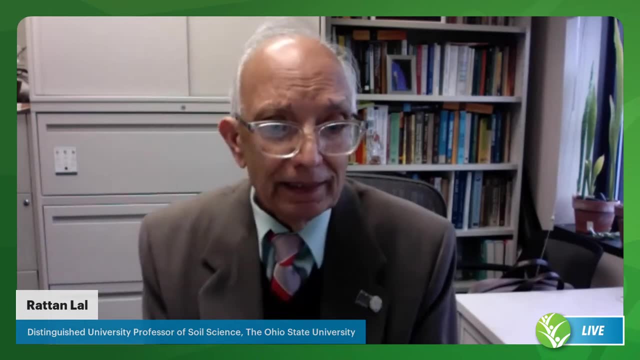 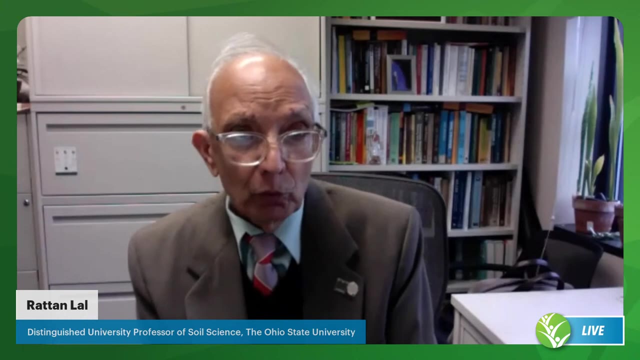 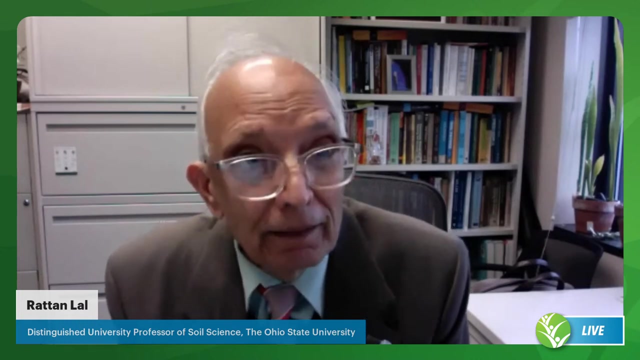 npk and pesticide will decrease balance. use of plant nutrients rather than flood irrigation, drip, digital agriculture, artificial intelligence, so that you can remove drudgery. i know the time is running short. i would simply mention that the farmer should be properly motivated. and how much? i would suggest 125 to 130 dollars per ton of carbon. that translate into per credit. 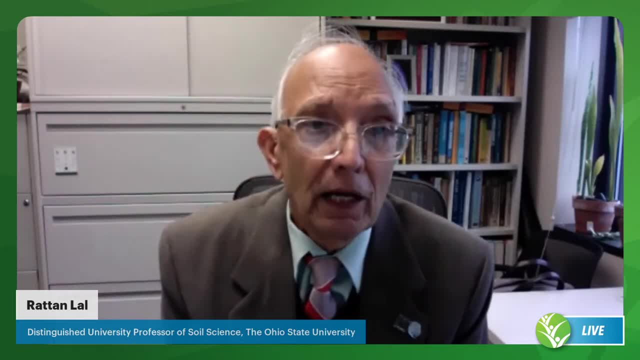 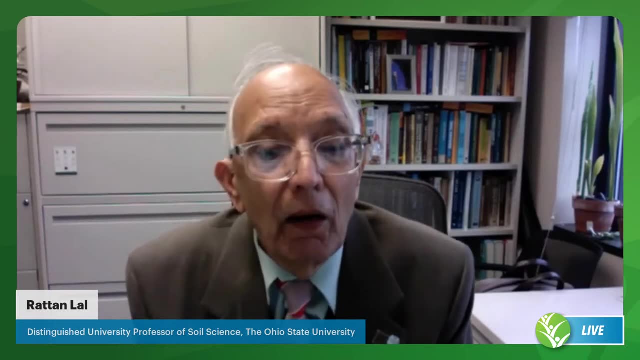 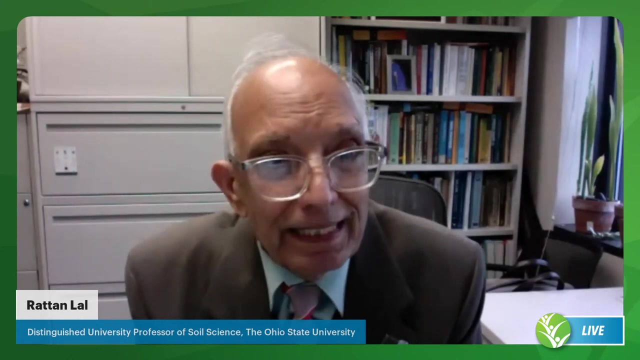 it will be about 30 to 35 dollars per carbon credit. that the price that the farmer should be compensated. why is carbon compensated by carbon? the science does not know that how to make carbon. because on degraded soil, if they persist, the global peace and stability and tranquility. 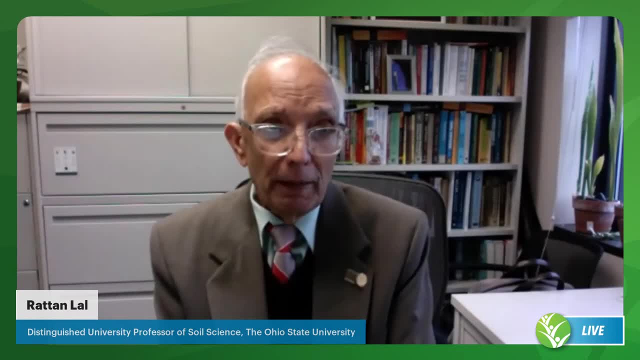 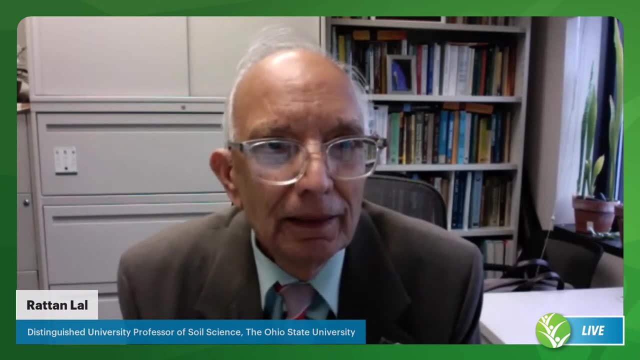 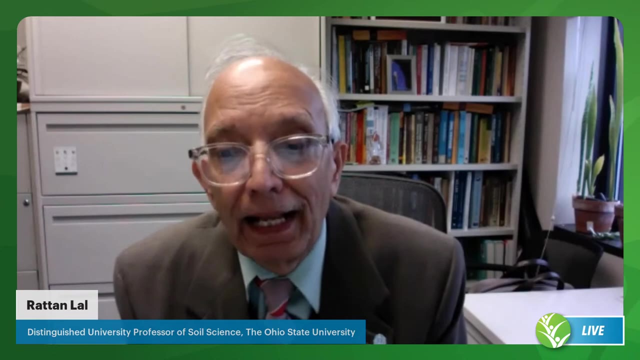 is in danger. in fact, the only mass of weapon of mass destruction that we know by now is hunger and malnutrition, killing 16 to 17 people a minute. therefore, solution lies in a mantra: healthy soil equal to healthy diet, equal to healthy people equal to healthy ecosystem. 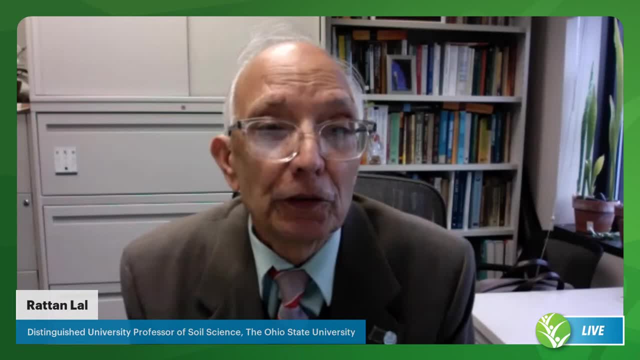 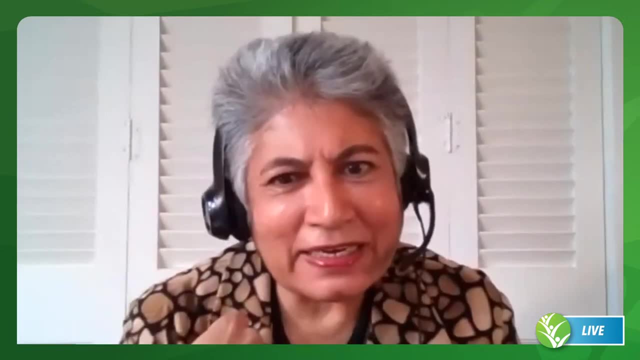 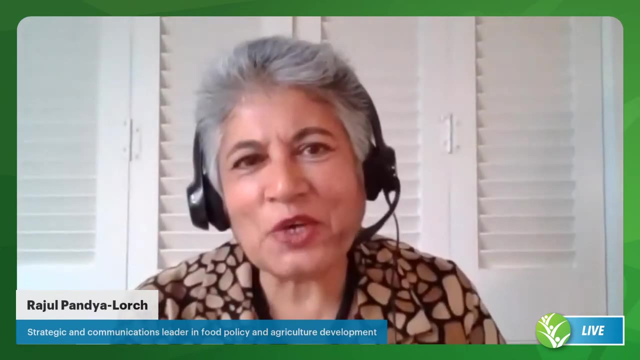 equal to healthy planetary presses, equal to world peace and stability. it is that important. thank you, professor. that was a master class in five minutes or less why soils are so important and what we can do. truly, i applaud you for that. i'm sure we will come back in the q a for further elaboration. 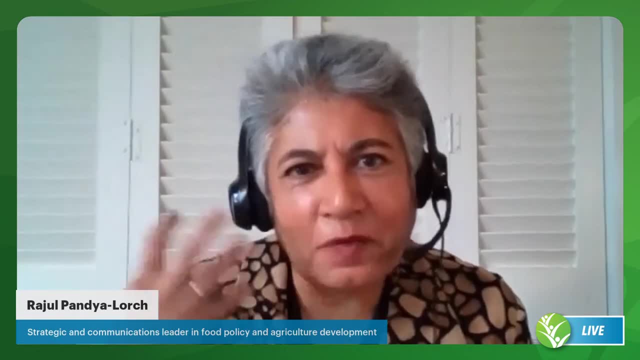 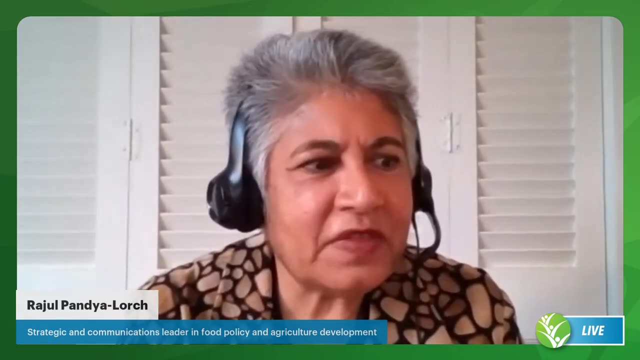 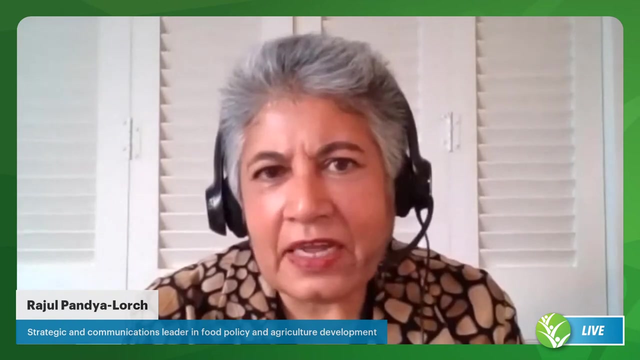 but i would like to turn to the next speaker, and that is javu ku, senior research fellow at ifri, javu uh. professor lal also talked about the importance of digital agriculture and the communicates of, also emphasizes high quality soil data and advocates for new technologies. 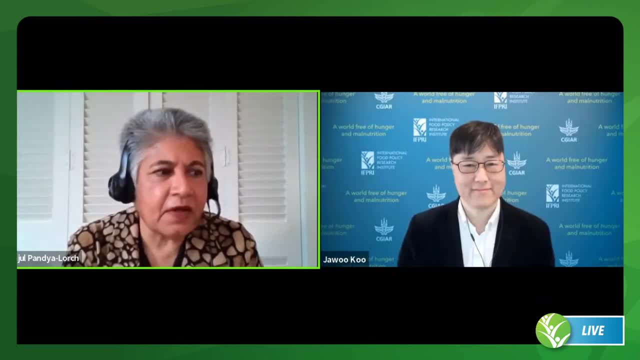 and digital solutions. so thank you, professor, for sharing that, and i would like to thank our next speaker, and that is javu ku, senior research fellow at ifri. Can you tell us a little bit about how digital technologies can contribute to improving data and to otherwise achieving healthy soils? 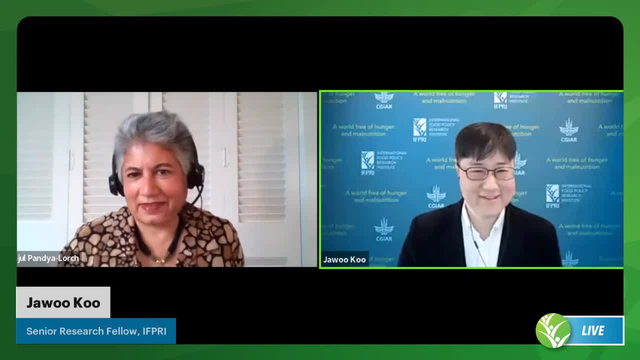 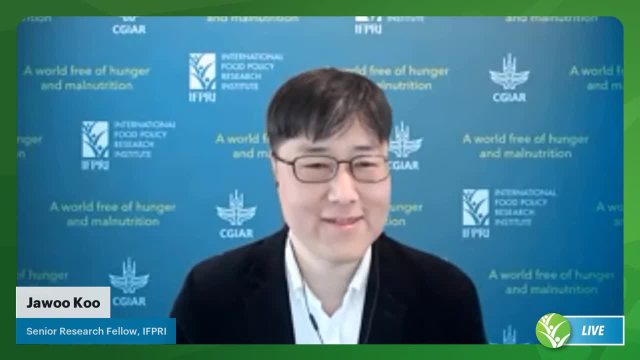 Over to you Absolutely. Thanks so much for this opportunity. It's a great honor to follow Professor Lal's presentation. Despite the importance of soils, however, it has been always challenging to find quality soil data, no matter where you farm or conduct research. 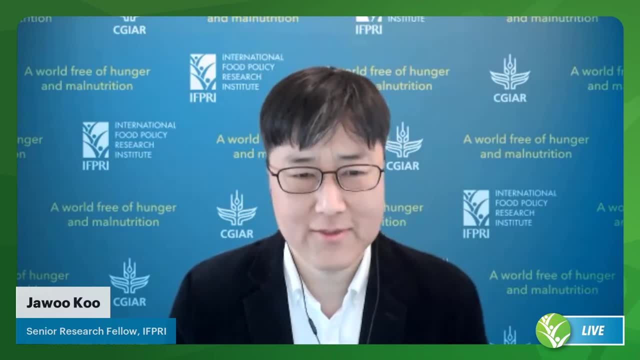 I'd like to briefly describe a couple of fundamental challenges in why it's so difficult to generate quality soil data and how digital technologies are addressing them. The first reason is somewhat obvious: Unlike weather and climate, we cannot see what soils look like on the ground. 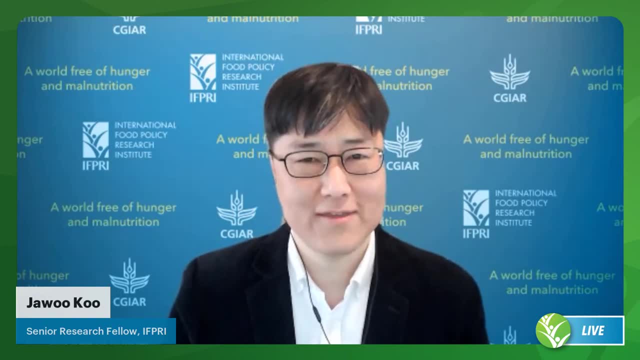 There are only a limited number of soil pits where soil scientists dug up the ground, collected soil samples at different depths and analyzed them in the lab to generate site-specific soil reports. This soil profile data is crucial to understand what kind of soil nutrients there are. 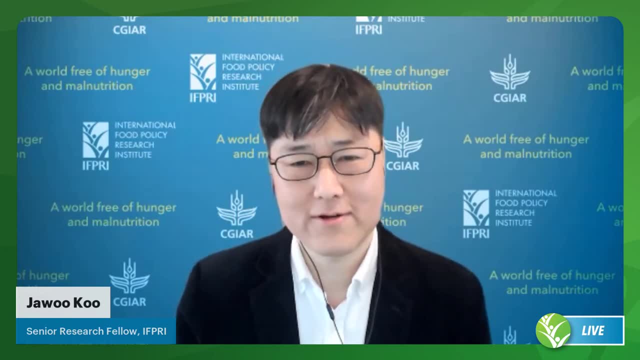 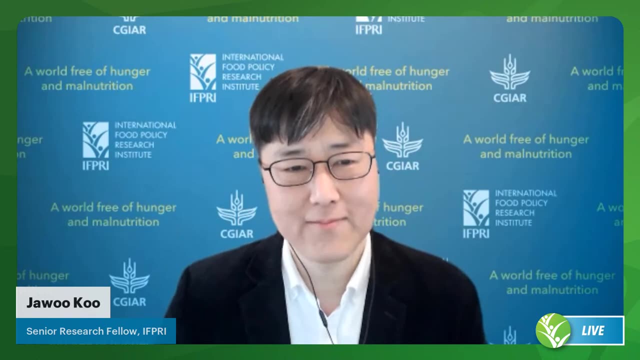 and help farmers to decide how to manage them. Because of the logistical challenges of collecting and analyzing soil samples at scale, recent advances in digital soil mapping approaches are playing an important role. Soil scientists correlate soil properties with other information we can collect or observe. 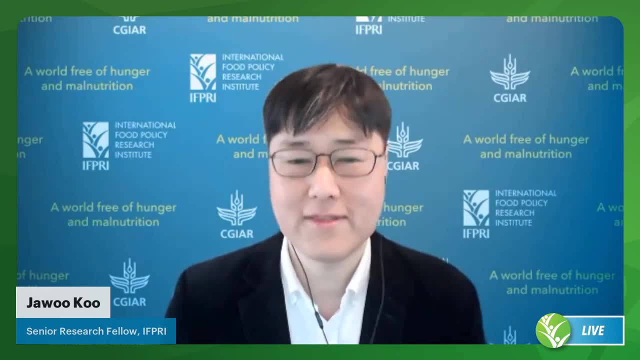 such as farm management practices and land cover data, and predict soil properties in other locations, For example taking advantage of AI and machine learning techniques. the Latest Soil Maps from ISDA initiative provides high-resolution soil property data across Africa at 30-meter resolution. 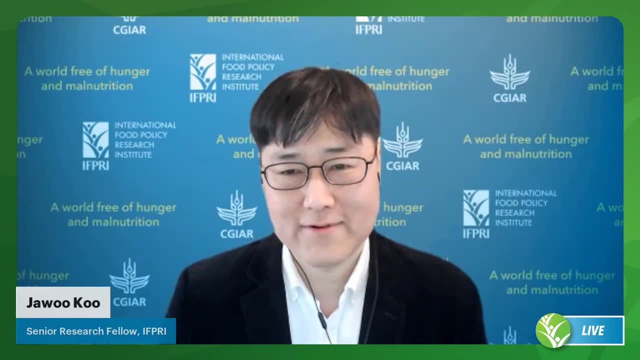 The second reason is the dynamic nature of soil properties. Some soil properties, like texture, are rather stable over a long period of time. You can use data measured in the past. On the other hand, soil nitrogen and soil moisture content, for example, are highly sensitive to high-density soil and are also highly sensitive to high-density soil. 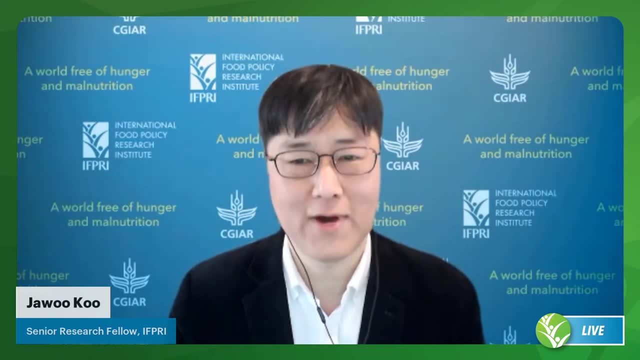 are highly sensitive to high-density soil and are also highly sensitive to high-density soil. The third reason is how farmers manage the field, under what weather and climate conditions. There is already a global shortage of soil samples and tracking the dynamics of soil properties over time. 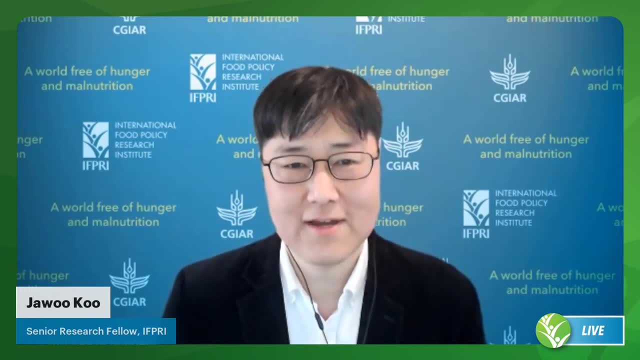 is even more challenging. Here, data from remote sensing technologies, either from satellites, drones or in-field sensor devices, are particularly useful to fill the gaps. There are statistical relationships between the reflectance of light on soils and their properties. These relationships can be applied to remote sensing data. 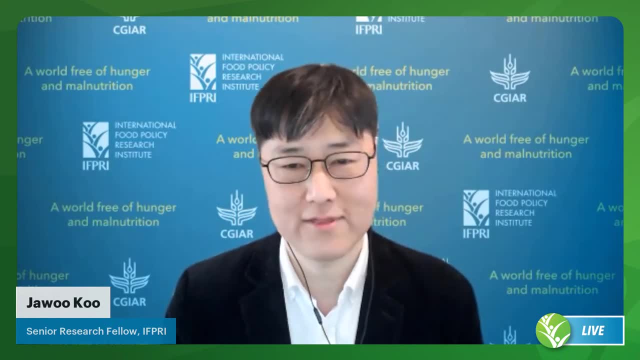 and used to monitor changes in soil moisture and carbon stock, for example, across large area when mushroom changes happen. These data are already being used in practice to more vorneal soil quality and promote healthy soils. The Ethiopian government's effort to develop a high-quality soil database called ETOCis. 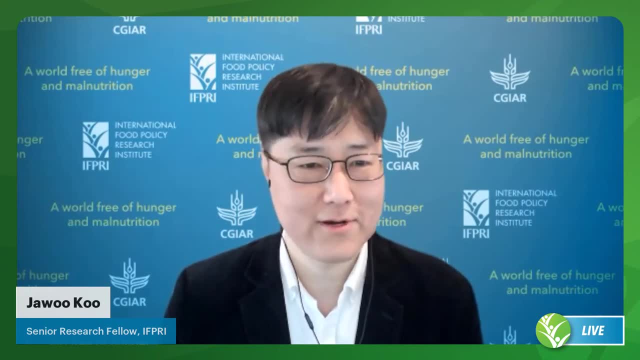 is used to prescribe the most optimal blend of fertilizers locally. Digital technologies also connect soil scientists, businesses, integrity researchers, communities, etc. connect soil scientists with farmers by streamlining soil sampling and lab analysis- Indian government soil health card system, for example. 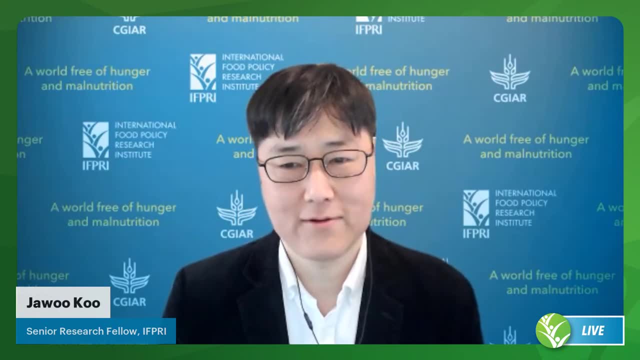 collect soil samples from all across the India, analyze them at low cost- about $3 per sample- and, once analyzed, farmers receive a soil health card digitally and they learn how best to manage their own soils. An impact evaluation study found that soil health card scheme. 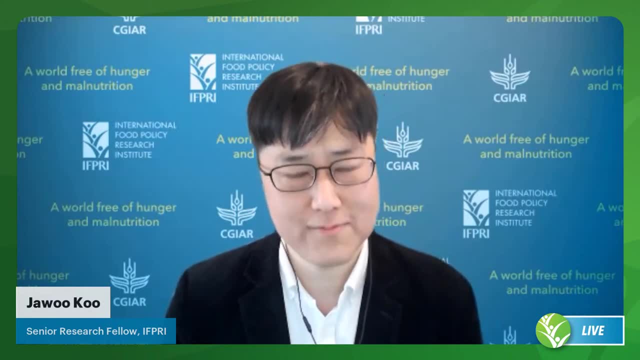 reduced fertilizer use and reduced management costs, and increased the use of gypsum and other micronutrients that otherwise might not have been managed. And these are just small subset of examples, and there are many other innovative digital applications that contribute to making quality soil data more available, accessible and relevant. 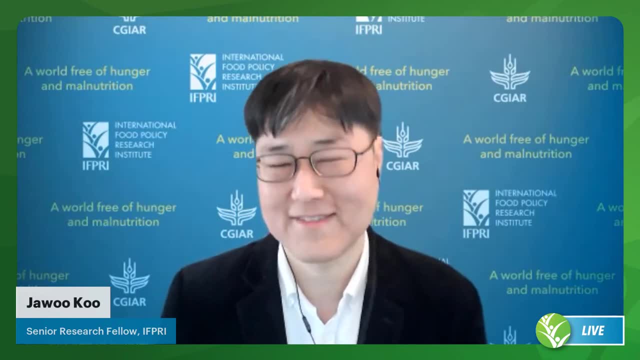 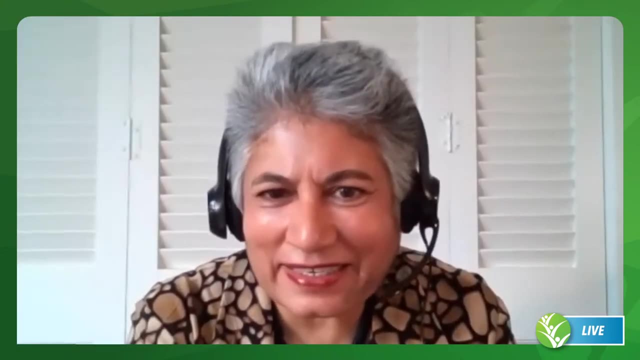 In a way, it's an exciting time to be a soil scientist, Thanks. Thank you very much, Jao. It is an exciting time to be a soil scientist. It is an exciting time to be in science. Thank you for sharing with us some of these examples. 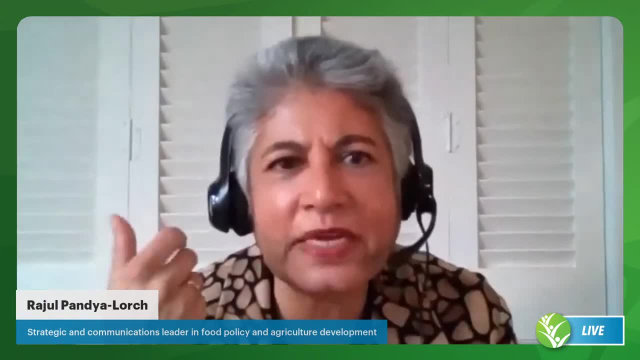 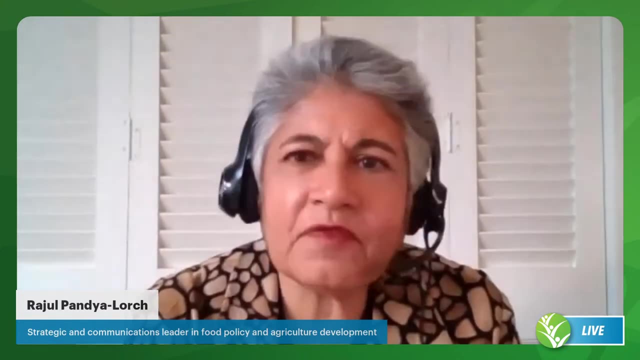 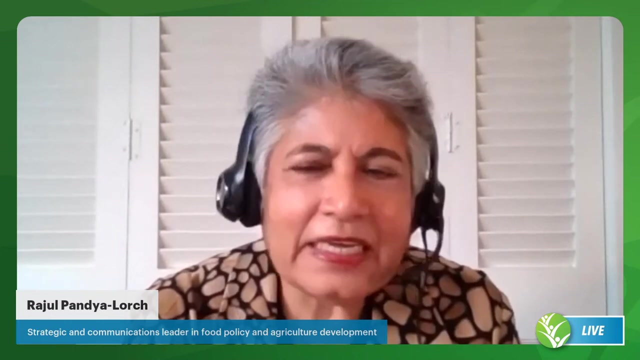 and for sharing the real on the ground examples, with story from Ethiopia and India. Hopefully we can delve further into that in the Q&A session. So we switch gears now to hear from national activities and national perspectives, And our next speaker comes to us from Malawi. 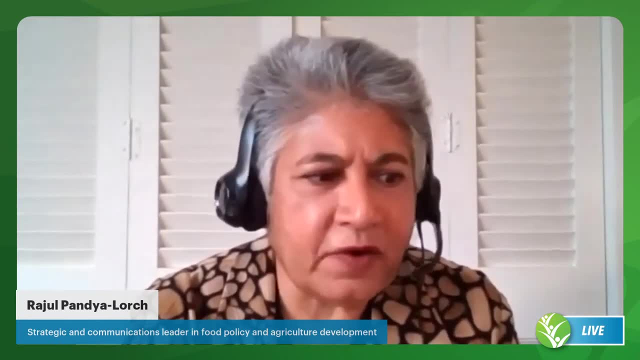 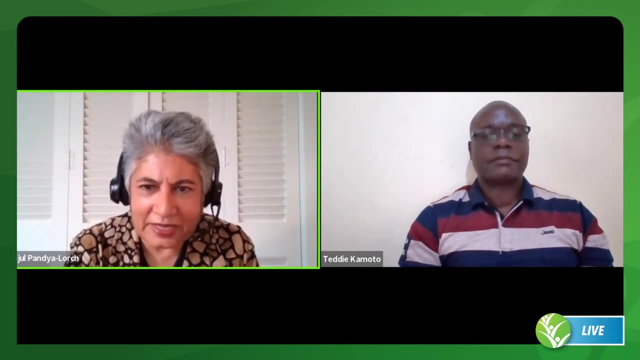 He is Teddy Kamoto, the deputy director of forestry in the Department of Forestry with the Ministry of Natural Resources, Energy and Mining in the Republic of Malawi. Teddy, long term, Thank you for your time. I'm glad to be here. 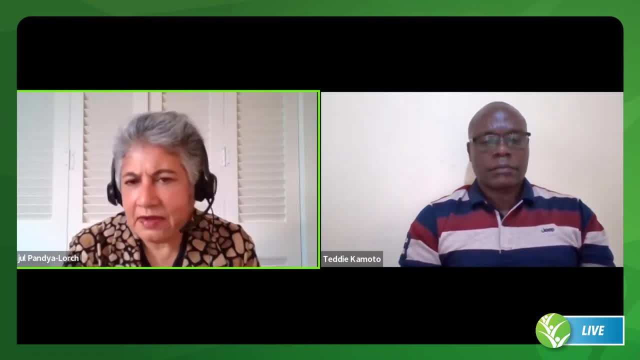 And I look forward to seeing you in the next session, But for now, I just also want to thank our speakers on the panel who are here, So I can't wait to hear from you. I'm so happy to hear what's you have to say. 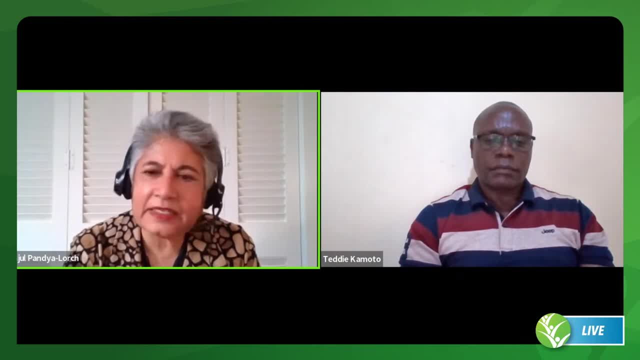 Yeah, sure, Thank you to everyone for attending. This is only my first time here, but I'm sure there will be a variety of things that we can try to address, But I would like to acknowledge our panelists who have spoken with us today. 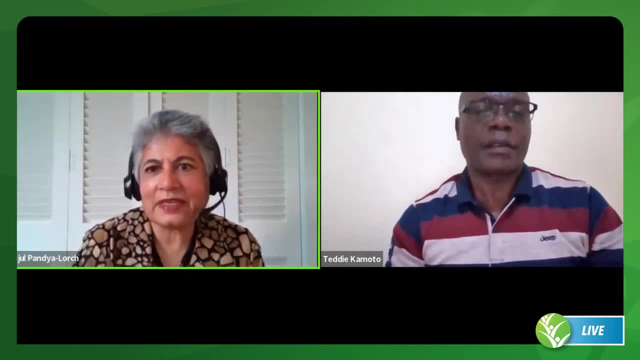 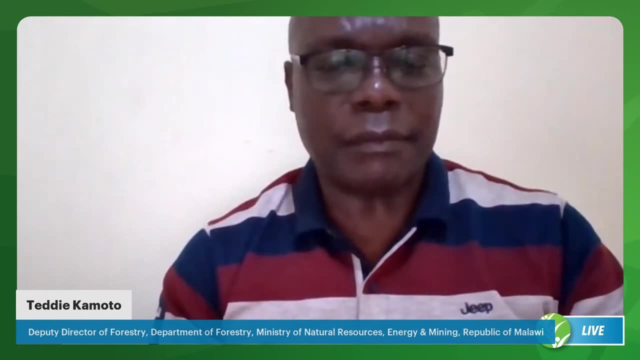 And thank you very much, everyone, for coming. I hope you will have a good afternoon And thank you very much. I'm so happy to continue, no matter what. So thank you to everyone who's brought in today. Thank you to congratulate the organizers of this function. 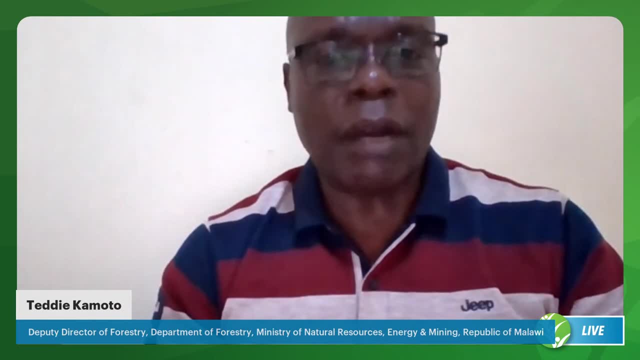 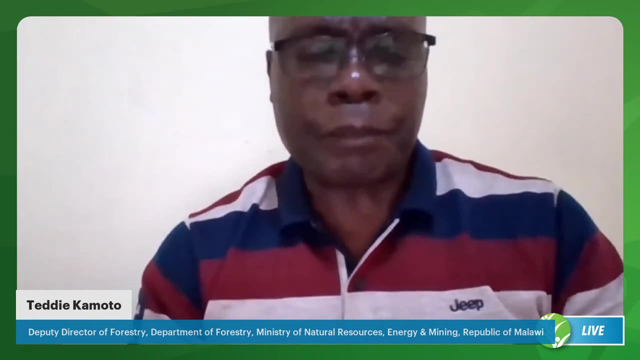 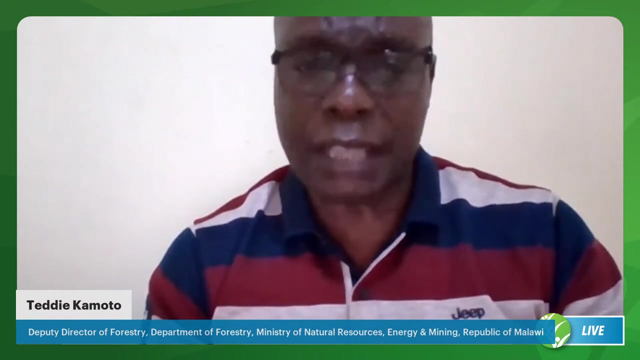 and, at the same time, our appreciation for bringing Malawi on the table, allowing Malawi to be part of this conversation. Maybe I should start by saying that, when you look at Malawi, Malawi, basically the economy is agro-based, and what it means is we depend more on agriculture. 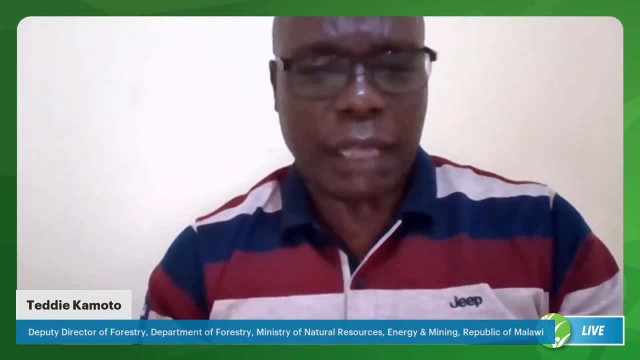 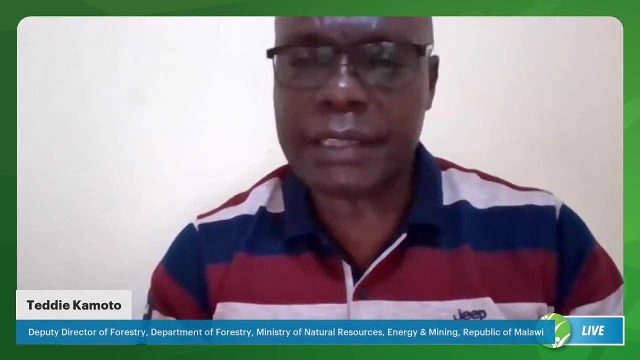 and therefore land is very critical And when you look at the landholding sizes, for the local Malawian farmer in Malawi is less than half an acre And that brings a challenge in terms of making sure that we have enough food. Of course, government has put a number of efforts. 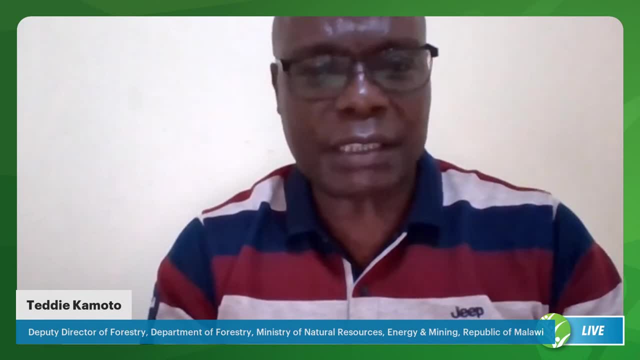 You may wish to know that we are one of those countries that provide subsidies to local farmers in form of fertilizers and seed. This is because the soils have been degraded so much so that productivity is very low. Now, when we look at these small landholding sizes, 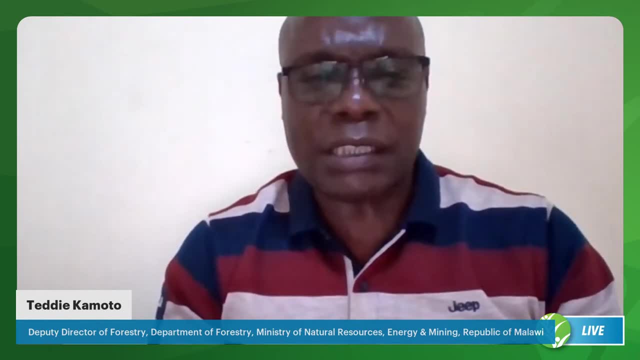 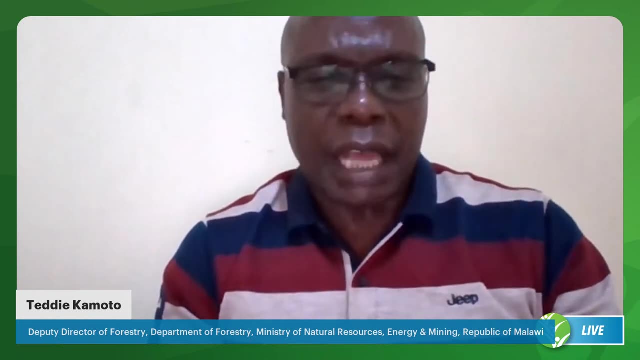 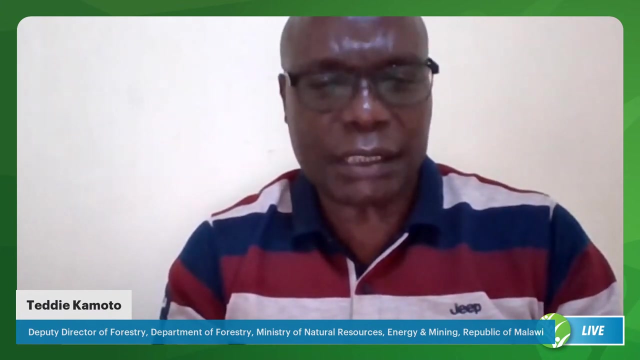 obviously you need to make sure that each piece of land that a farmer has is put to good use. And now when you look at the governing laws that are there on customised land, you will note that in the past, obviously all the land at customised level. 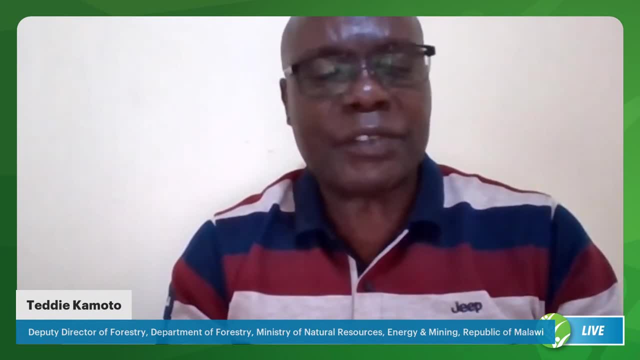 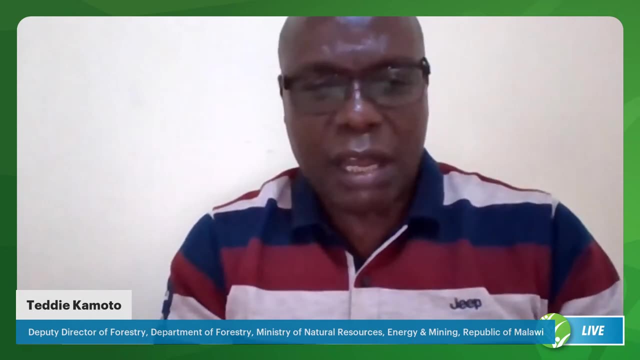 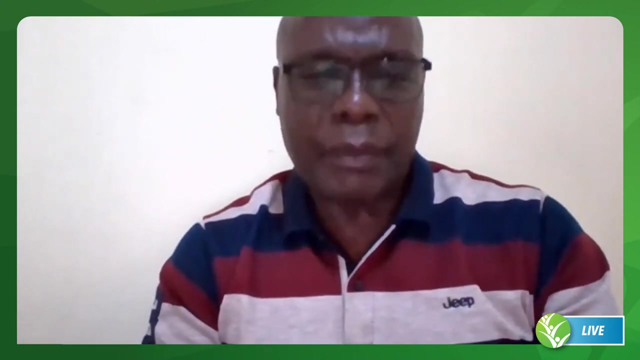 was being managed by the chiefs and therefore the chiefs could have the right to allocate land to anybody that he feels like. But now I think government has moved on and what it has done is one work on the legislation, making sure that the 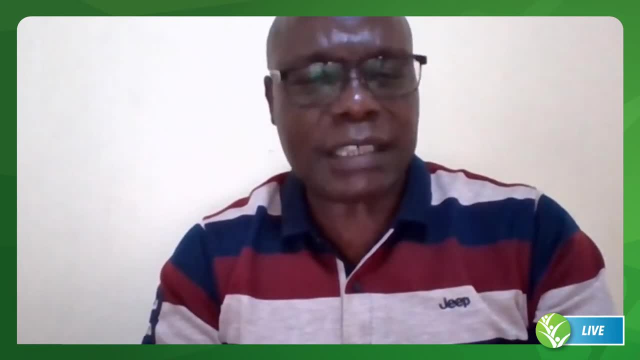 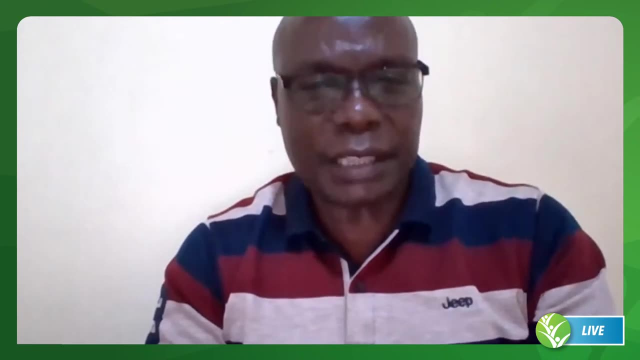 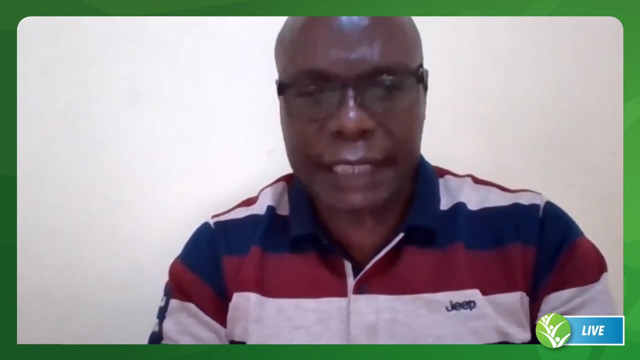 we put in place the governance structure at local level that manages the land other than the chief, the traditional leader himself. So that brings in the issue of fairness and that issue brings in the issue of assurance that when you have a piece of land that you are working on, 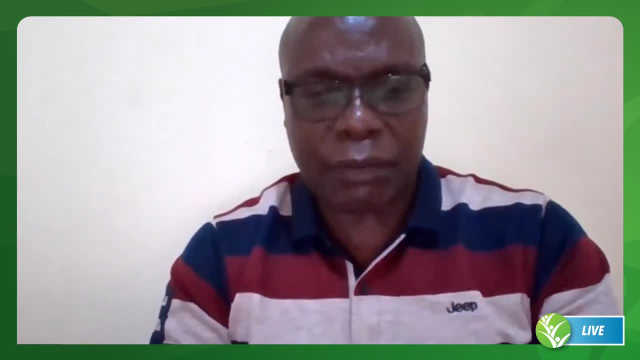 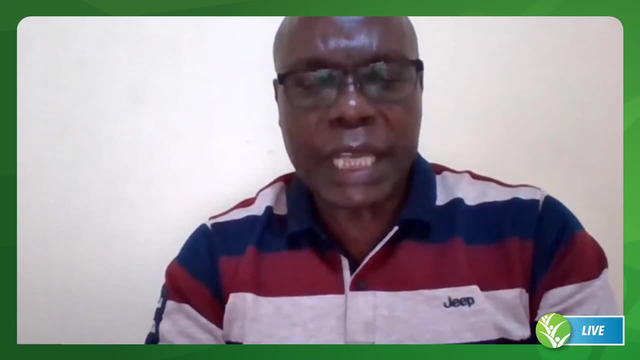 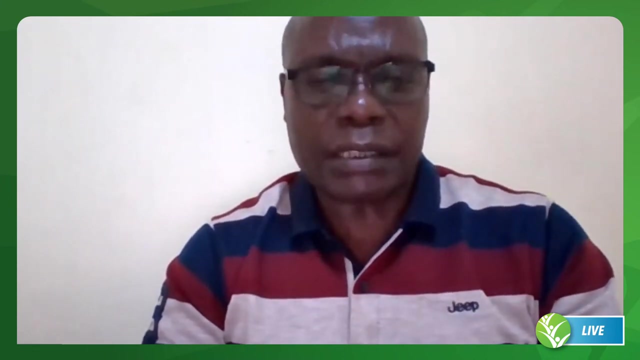 will not be grabbed from you and then, therefore, you can invest on that piece of land. But on top of that, what we're doing is to make sure that we, we, we, we are doing what we call participatory land use mapping, so that we are able to 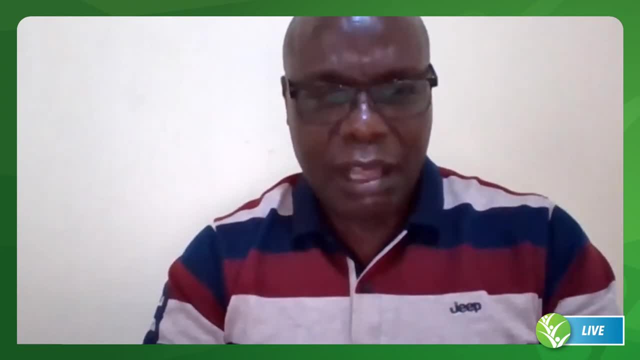 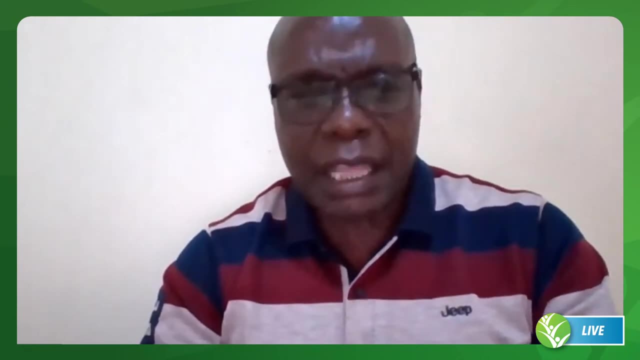 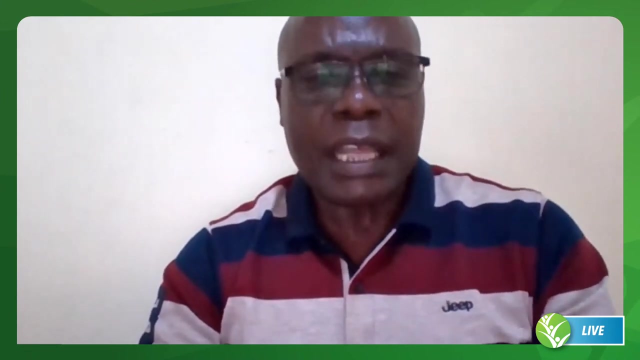 categorize the degradation in terms of the kind of interventions that can be done. So this participatory land use planning in all the districts we've done that- and therefore the distance of what we call participatory land use maps and these maps they are able to show the kind. 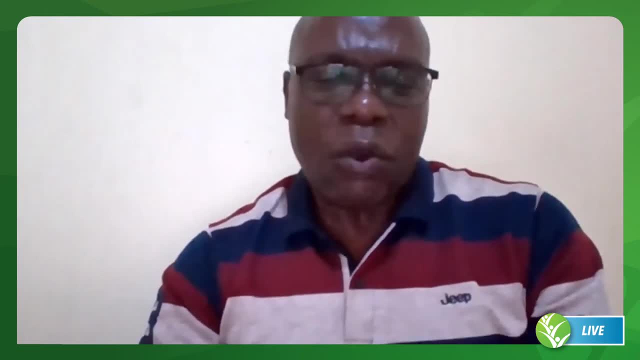 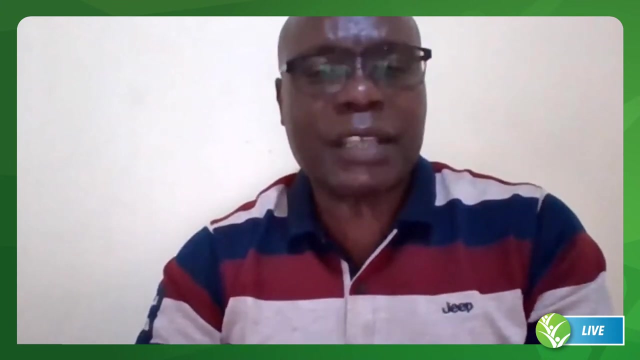 of degradation that has taken place and therefore, using what we call the national forest landscape strategy, we are able to use the interventions that are in there and, based on the assessment that we've done in the country, almost 70 to 80 percent of the country is degraded and that is very 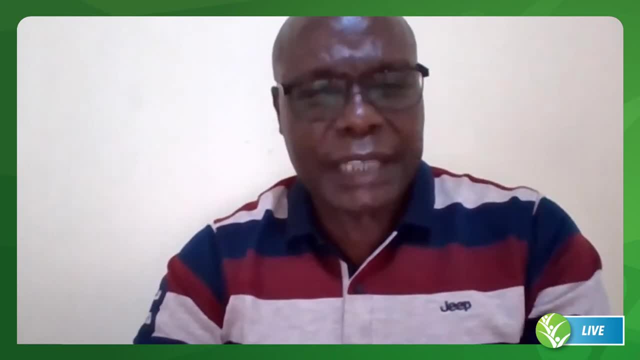 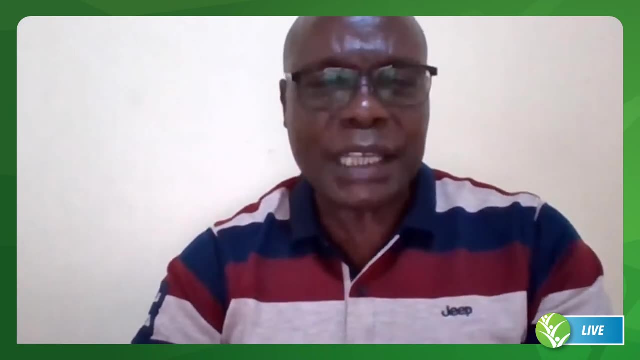 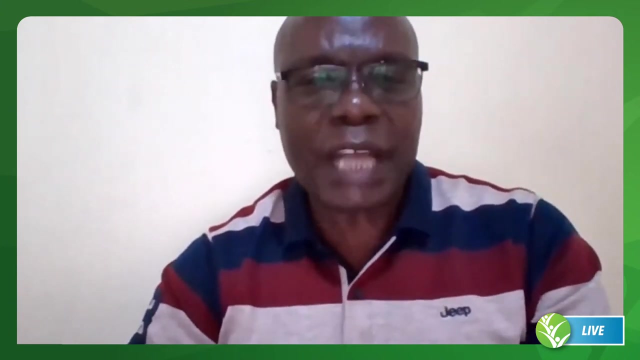 very scary situation and, based on that assessment, we were able to establish that 40 percent of that- 80 percent. for it to be rehabilitated, we need to use what we call improved agriculture technologies, because the soils are so much degraded. things like conservation, agriculture, climate smart. 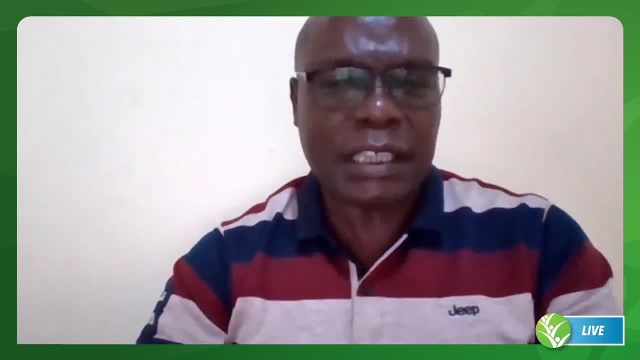 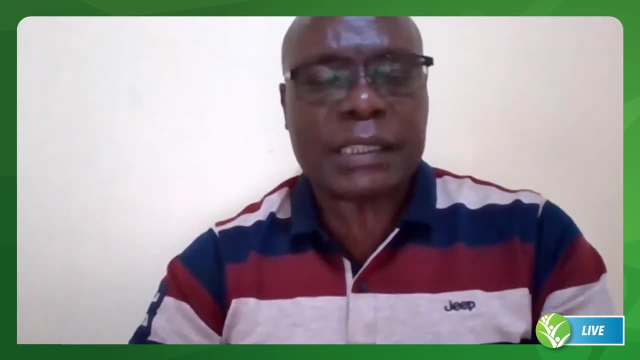 agriculture, agroforestry, farmer, managed regeneration because we have to do that, otherwise productivity will be very low. and when you look at the soil erosion and soil control, the interventions that we have in the strategy based on the assessment, shows that 11 percent of 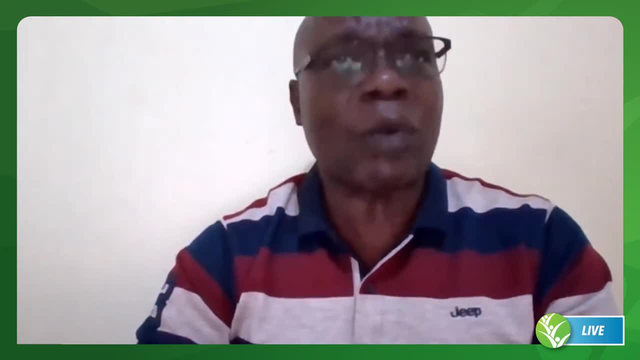 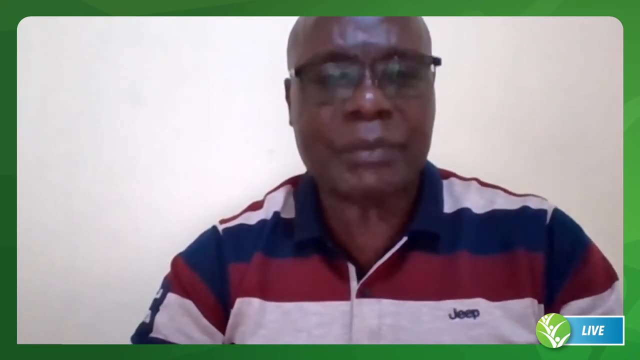 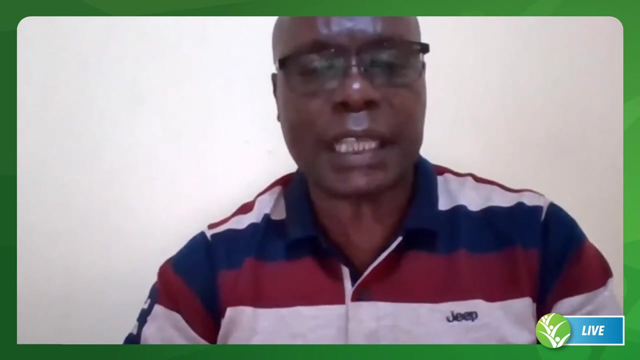 that 70 percent of the degraded land would require soil and water conservation type of technologies for us to be able to restore it, like the, the check dams, like the, the contours, and all that to reduce the flow of of water, and even water harvesting techniques. so these are some of 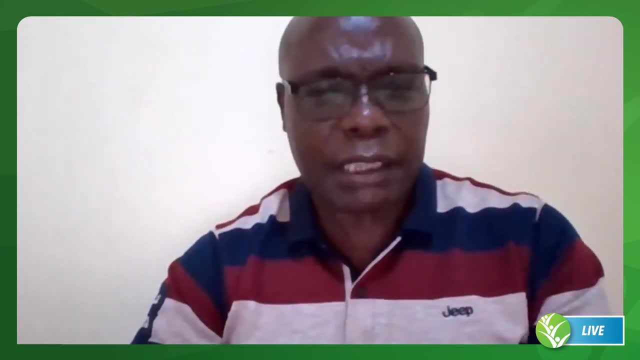 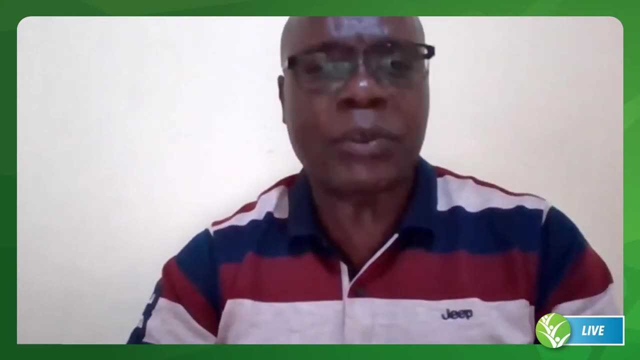 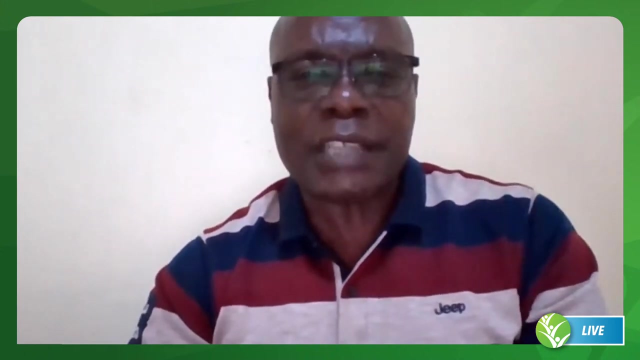 the things that we are doing and on top of that, we have platforms like the forest landscape restoration platform, where practitioners are able to share experiences in terms of what they are able to do in order to restore the degraded areas. so this this has helped, because now many farmers are 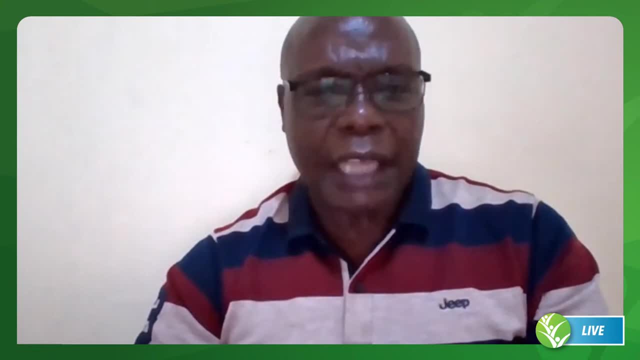 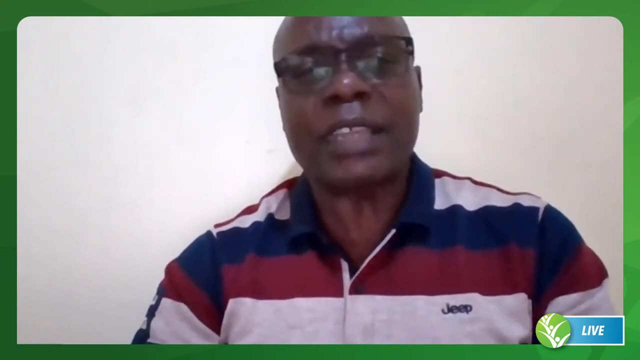 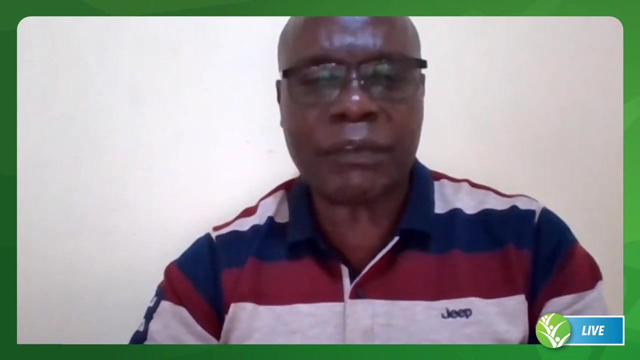 aware and they're able to access in terms of how to restore the degraded areas. So these are some of the things that, as a country, we believe that will help us to restore the degraded areas, Because if we don't, obviously it means even the number of farmers that have to depend on some aggregated substance will. 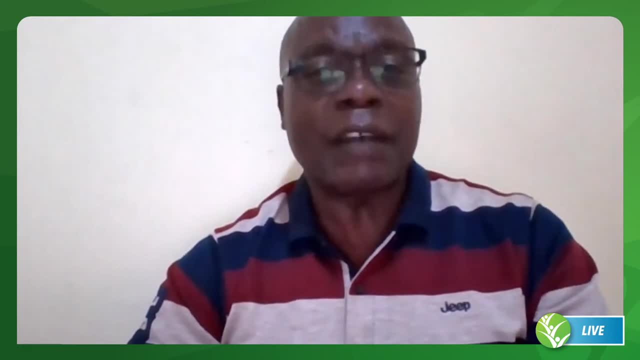 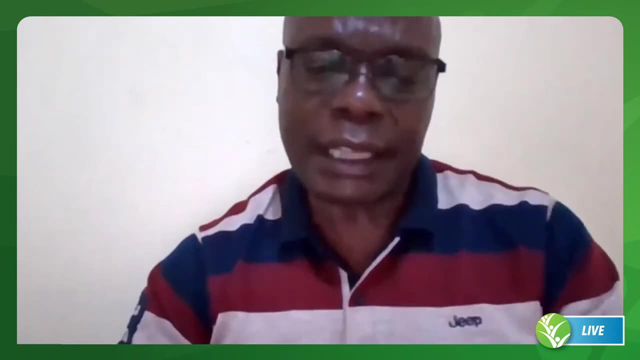 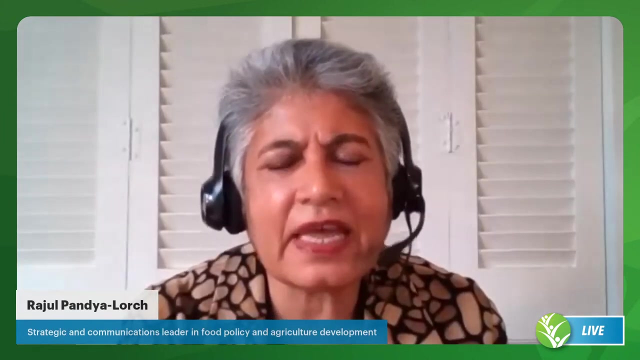 have to increase And I don't think government will have enough resources to do that. So the best way is to actually restore these degraded areas. So maybe if I can stop there for the time being, thank you. Thank you very much, Teddy. Thank you for sharing it as Malawi's. 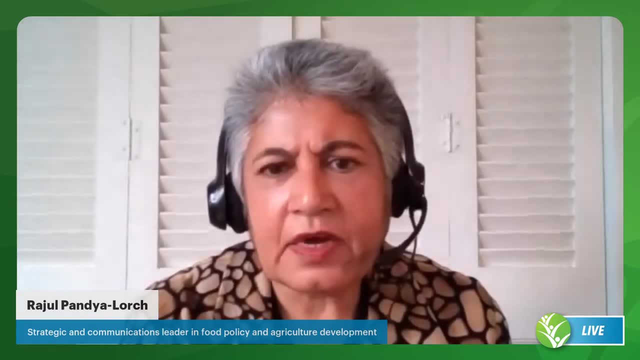 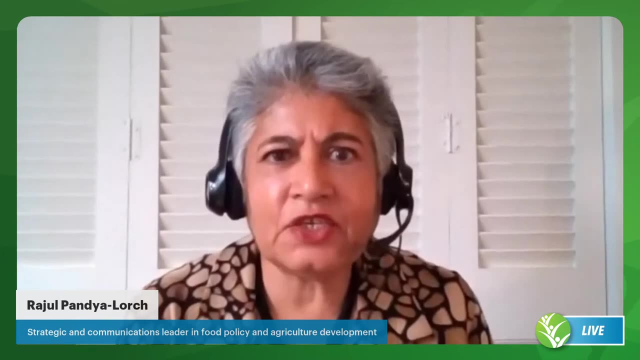 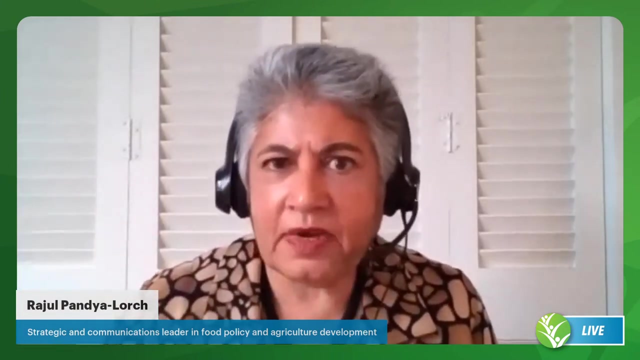 efforts, Malawi's investments and efforts to restore degraded lands, also to understand the extent of degradation and what actions can be taken. I was also happy that you talked about water, the water management. You were talking about the water management. you mentioned that, the water management. you were talking about the water management. 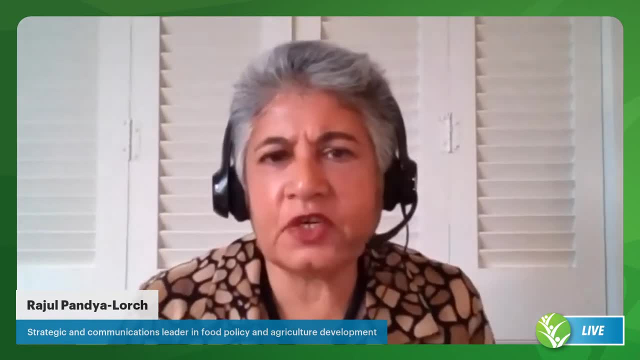 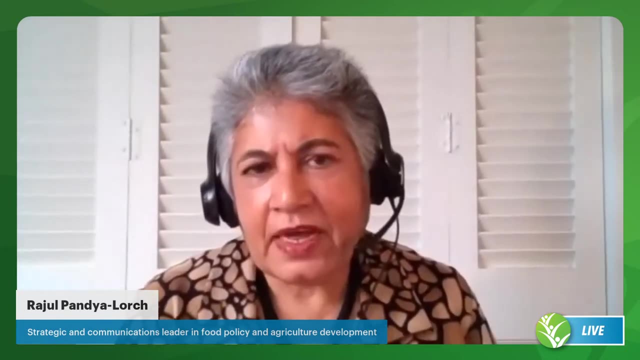 you mentioned that the water management. you mentioned that the water management you mentioned You talked about forestry and reforestation, so you kind of brought the whole family together of how to improve soil management. We'll come back to that in the Q&A, but thank you. 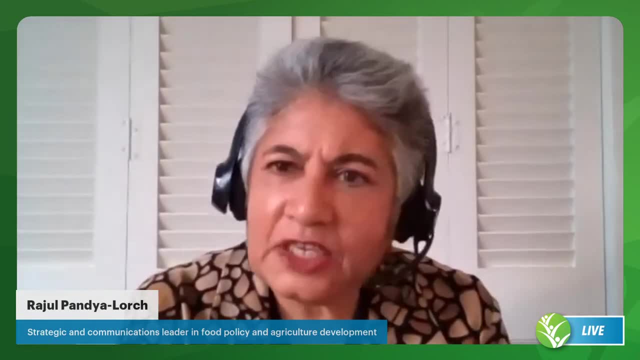 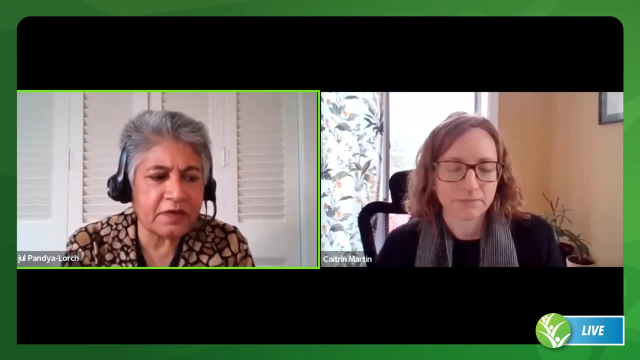 I'd like to move to our next speaker, then, and she is Katrin Martin. She is Agricultural Scientific Analyst in the Foreign Agricultural Service of the United States Department of Agriculture, USDA. Katrin, how are the existing and planned efforts in the US? 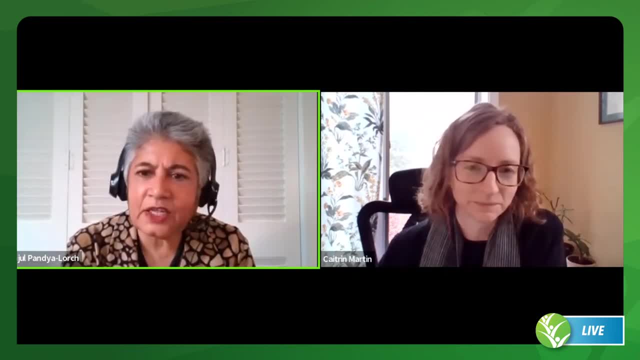 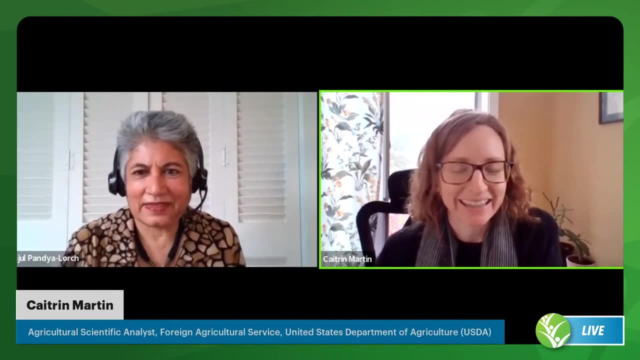 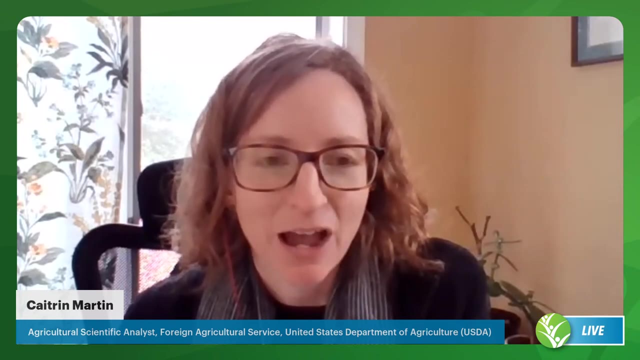 contributing to sustainable land use, climate-smart agriculture and healthy soils. Could you give us a quick flavor? Sure, thanks a lot, Rajul, And thanks to the organizers, Ifri and Astrid and other colleagues at the German Embassy for this opportunity to participate today. 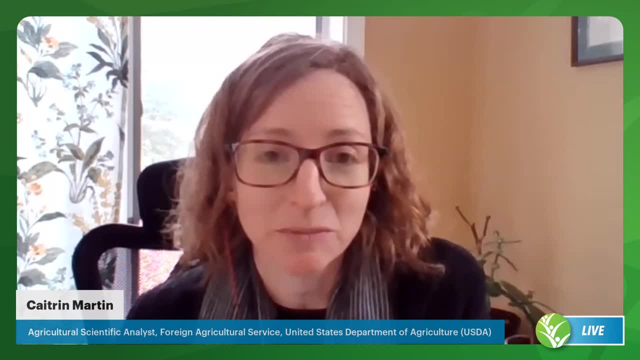 These are all topics that are priorities to USDA, so it's gonna be a challenge to distill all the relevant info into five minutes, but I'll start by saying that this year's GFFA communique essentially summarizes USDA's vision, which is to provide economic opportunity. 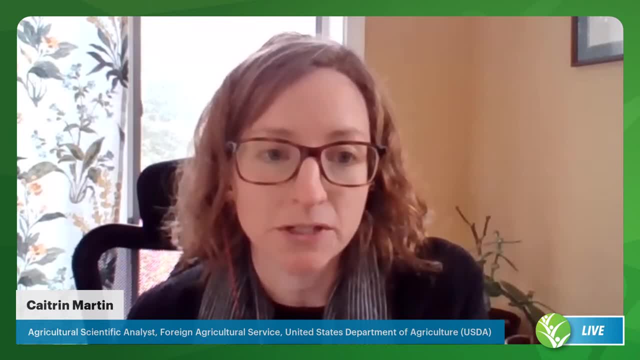 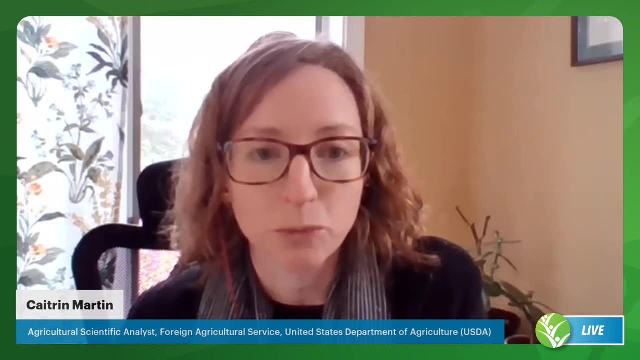 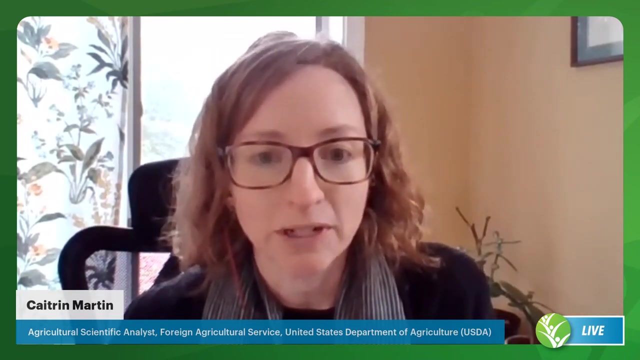 and promote agricultural production that better nourishes the world, while preserving our natural resources through conservation, restored forests, improved watersheds and healthy working lands. And I'll say, early in this administration, USDA conducted broad consultations with diverse stakeholders to inform our climate-smart agriculture and forestry strategy. 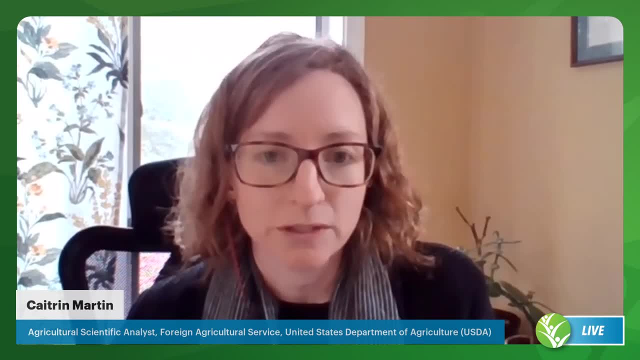 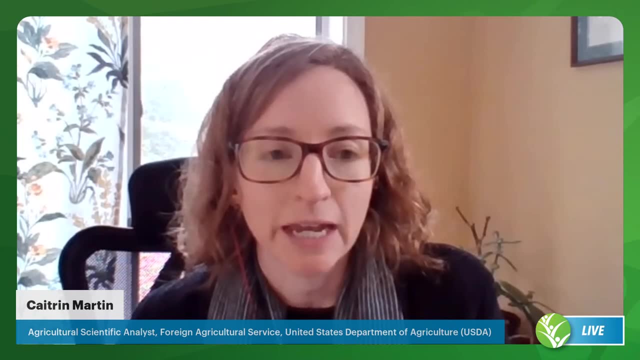 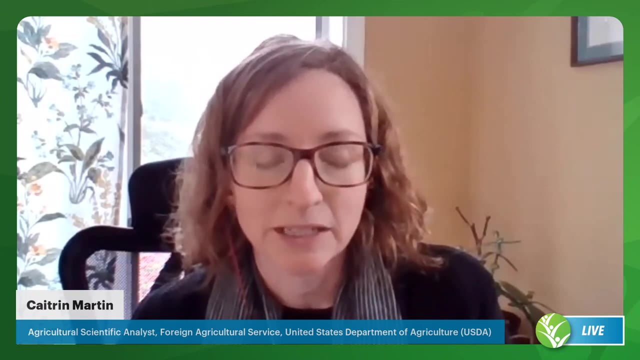 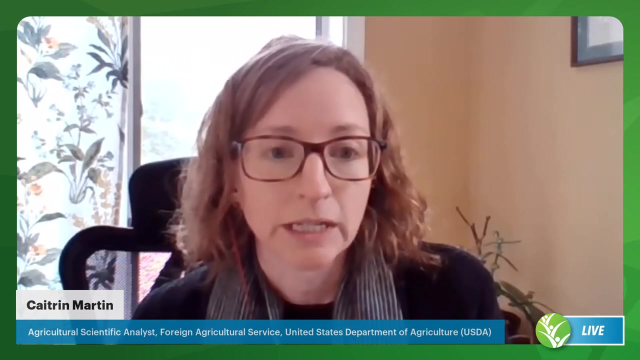 Input from these consultations reaffirmed our focus on innovation and partnerships. USDA's efforts are voluntary and incentive-based and farmer-led. These efforts include, among others, sustainable forest management and landscape-level planning, growing the biodiversity, of course, food loss and waste measurement and reduction efforts. 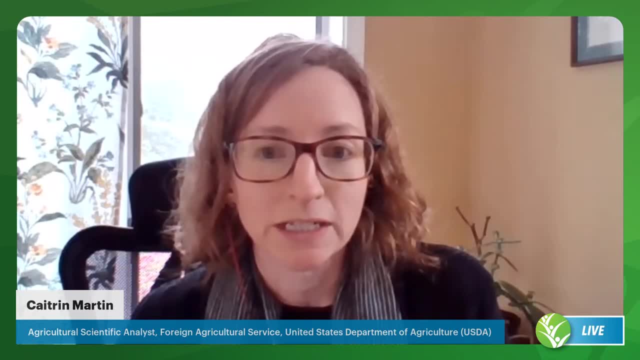 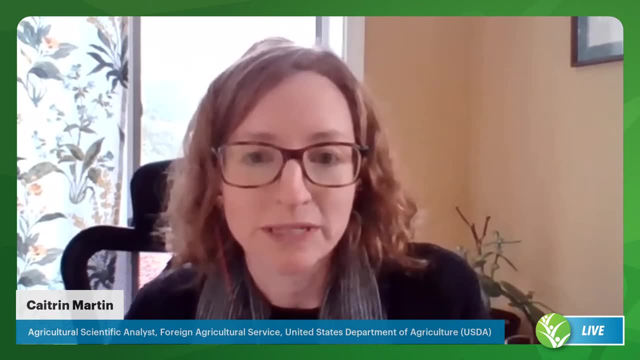 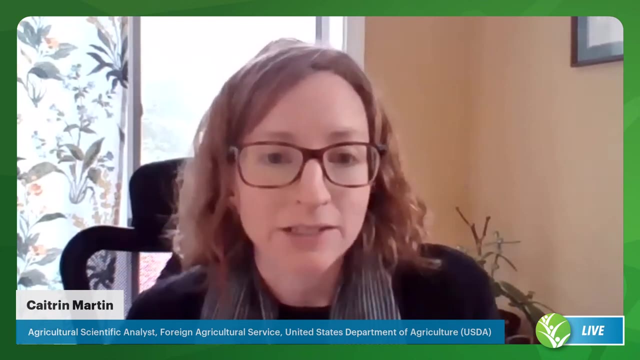 including research, data collection, MRV, and investing in the science and quantification of carbon sequestration. On trade and markets: we know we need to improve the business case for farmers to adopt and scale more sustainable practices by working to expand access to markets to meet the demand. 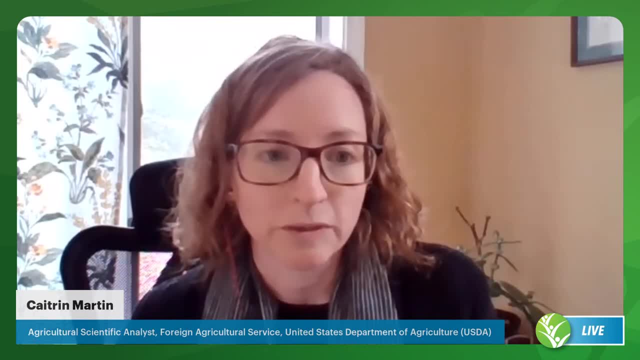 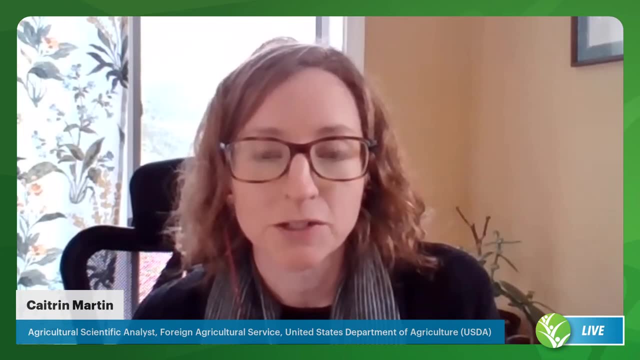 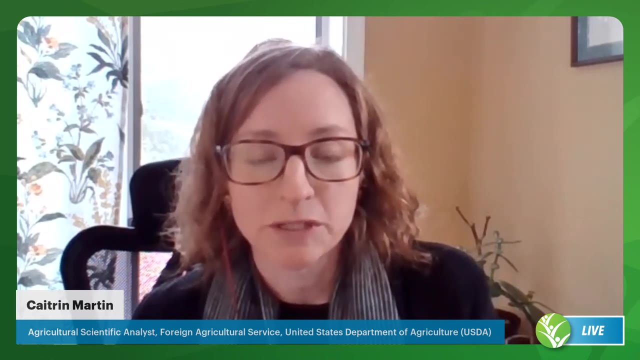 for sustainably produced foods, both domestically and globally. USDA is providing technical and financial assistance to help producers and landowners make conservation improvements that enhance biodiversity and ecosystem services, build resilience and contribute to the nation's broader efforts to tackle the climate crisis. 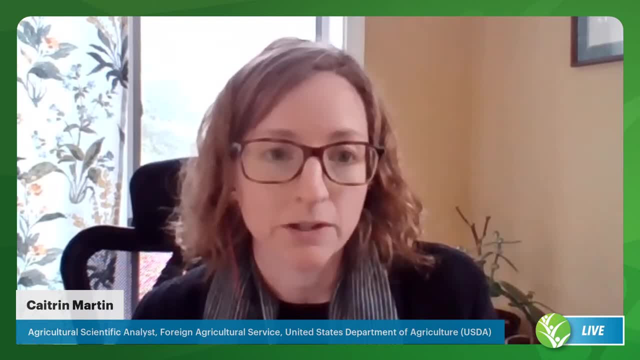 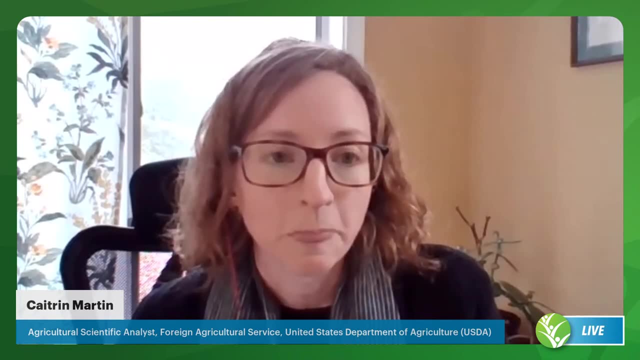 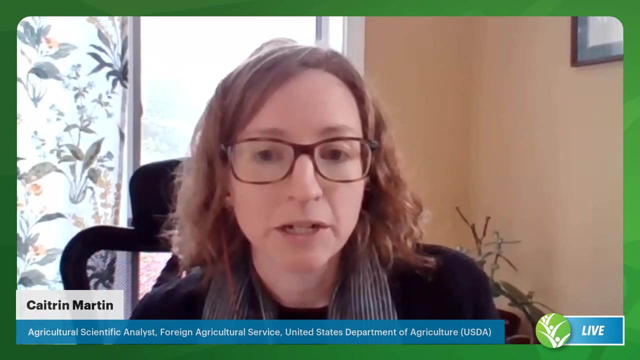 And I'll mention just a few of the Department's efforts since January. We've expanded investments in existing conservation programs, like the Conservation Reserve Program. We're continuing the Pandemic Cover Crop Program, which offers farmers who plant cover crops a discount. Thank you. 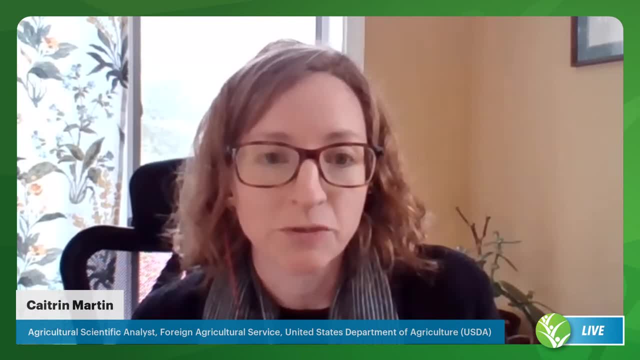 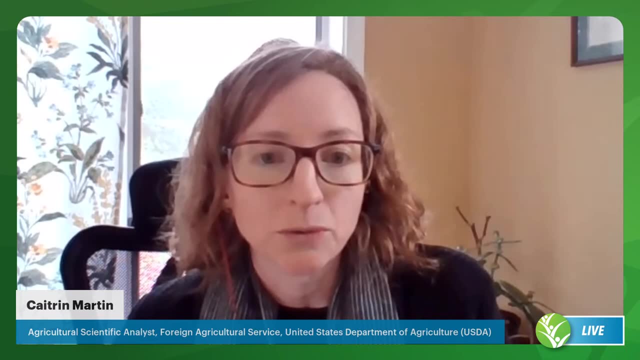 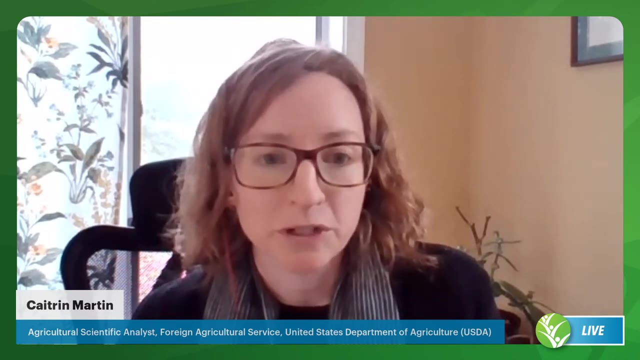 Thank you. This has been successful in retrieving". We have missed you. this program gave farmers a new discount on their insurance premiums and this program incentive covered over 12 million acres last year. There's a $9 million investment in new cooperative extension and USDA Regional Climate Hubs Partnership. 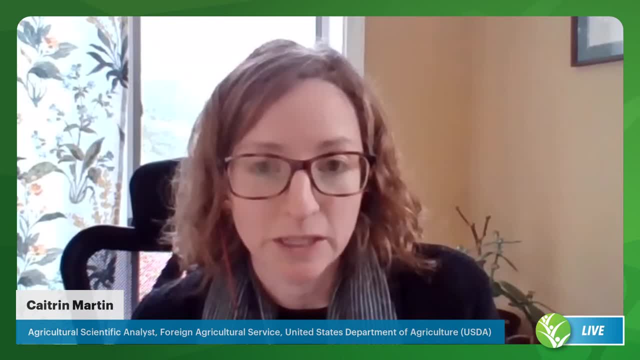 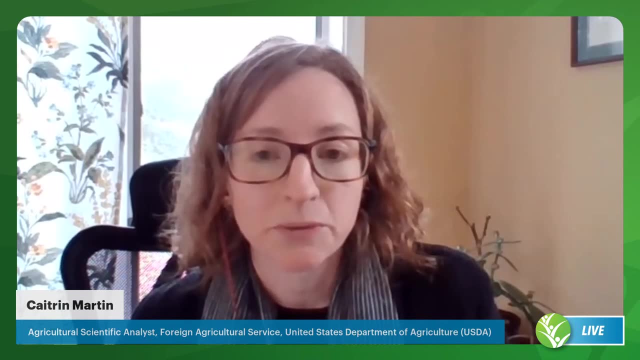 to bolster climate-change research and share climate-smart solutions directly with the agricultural community. that will support the production of climate smart commodities through through a series of large scale pilots and demonstration projects. A key component of these partnerships will be in financing the steps. 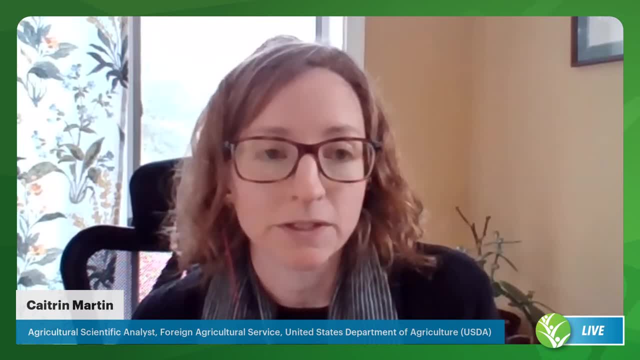 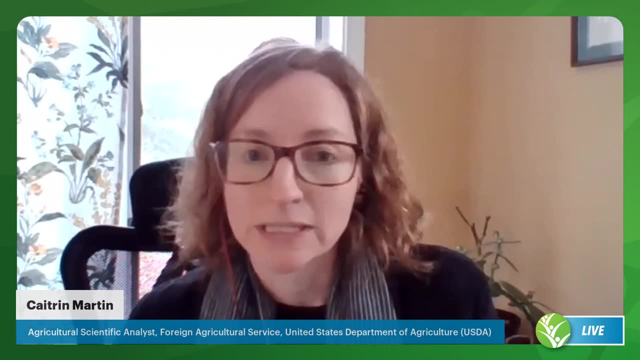 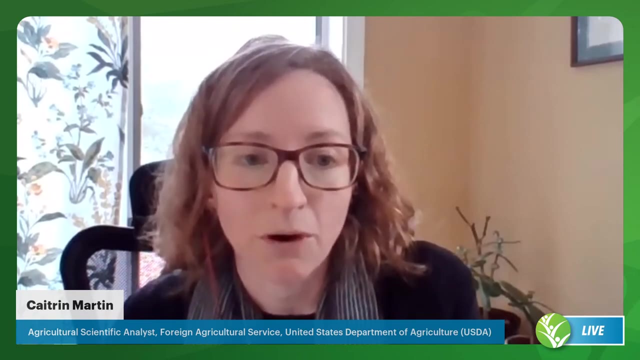 necessary to measure and validate the greenhouse gas benefits of those practices. Another key aspect of the partnerships will be equity and inclusion. USD or US agriculture includes a wide range of farm systems and sizes, and the program is accessible to all. So you can check out the website. 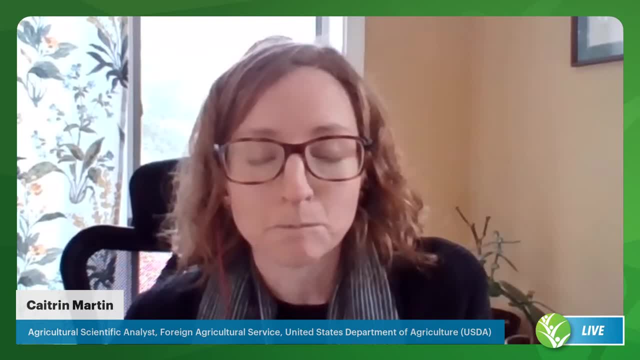 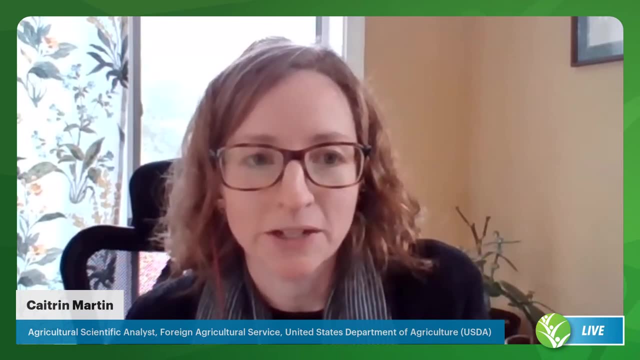 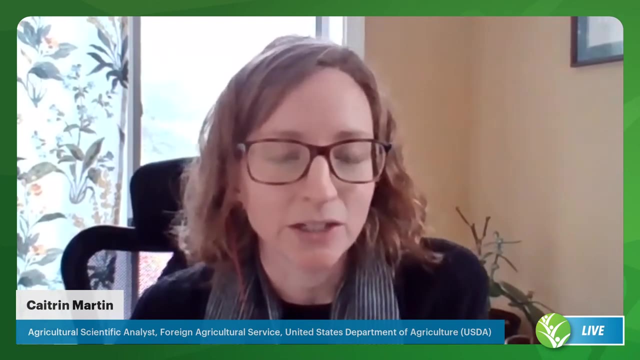 We're accepting project applications now. So in preparing for this discussion, I was talking with some of my USDA colleagues, and in chatting with a colleague from the National Natural Resources Conservation Service He picked up a copy of the the 1938 Yearbook of Agriculture that he had sitting in his office. 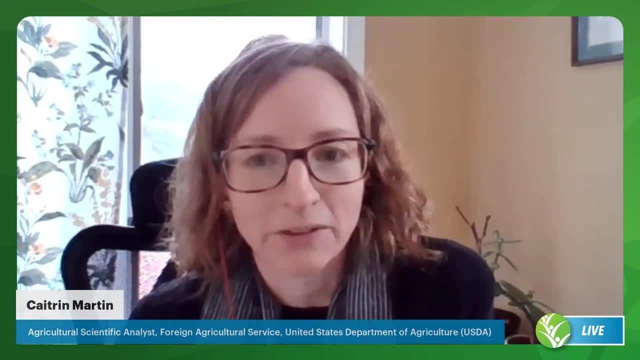 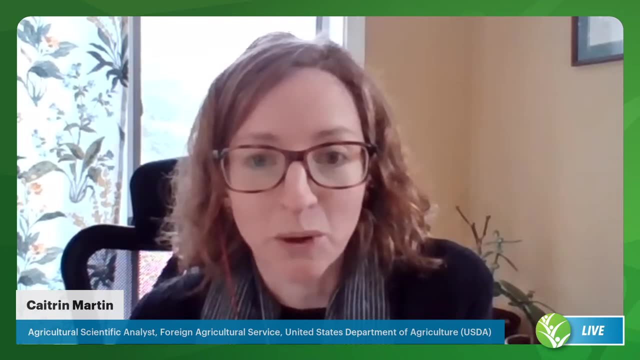 and he highlighted a few chapters to offer a sense of some of the challenges that had been identified over 80 years ago that we continue to work to address and many of the proposed solutions, like restoration of soil, organic matter with cover crops, use of manures. 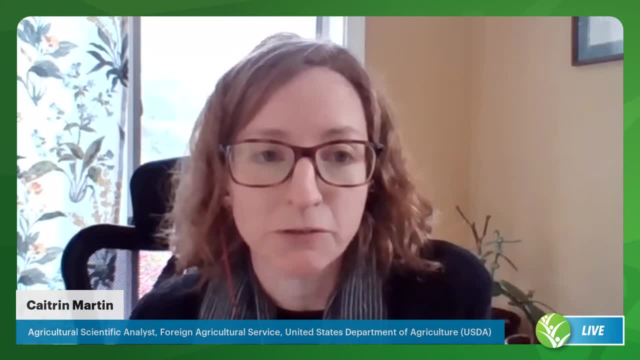 and organic amendments. reforestation and revegetation of marginal lands for erosion control: These solutions are not new, but that doesn't make them any less effective or less necessary And, if anything, in light of the climate impacts and the needs of the growing global population, they may be even more necessary. 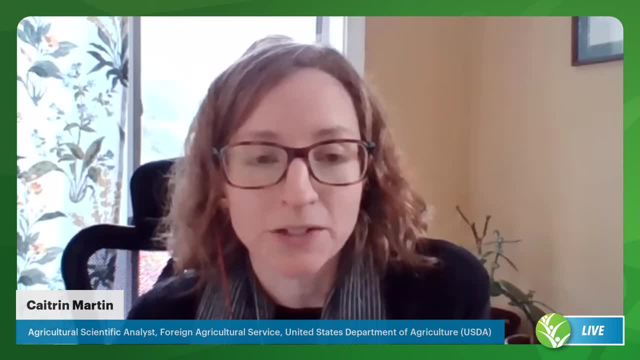 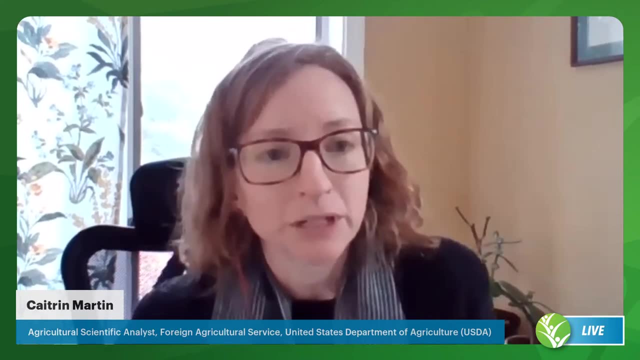 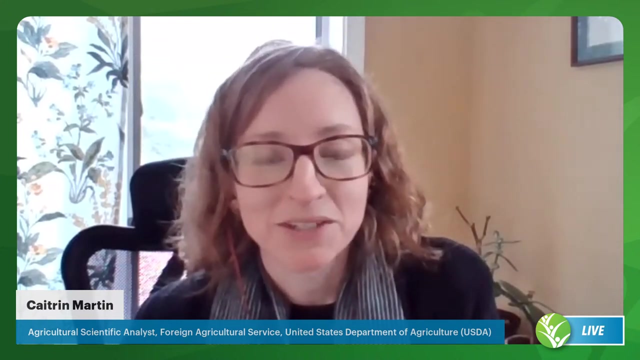 now, and by pairing those tried and true conservation practices with cutting edge new tools and technologies, we can really see improvements in soil health, nutrient use efficiency and sustainable productivity growth that enhance livelihoods. And there are so many potential exciting new game changers on the horizon. 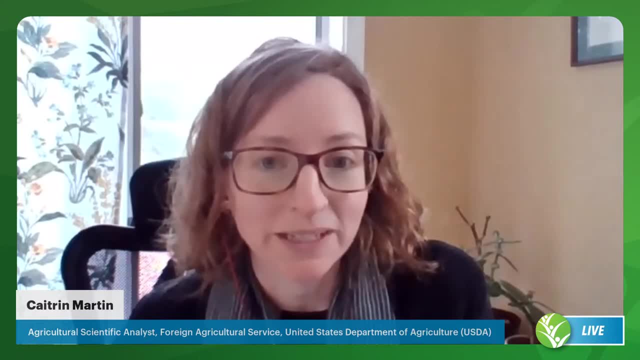 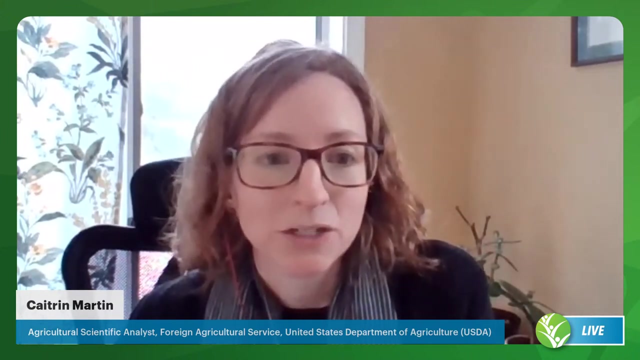 So an example is research on new perennial grain crops that can enhance agrobiodiversity, improve soil structure and nutrient and water retention. A recent grant of $10 million was awarded through USDA's Sustainable Agricultural Systems Program to a coalition of researchers and farmers and educators and industry leaders to scale the research production. 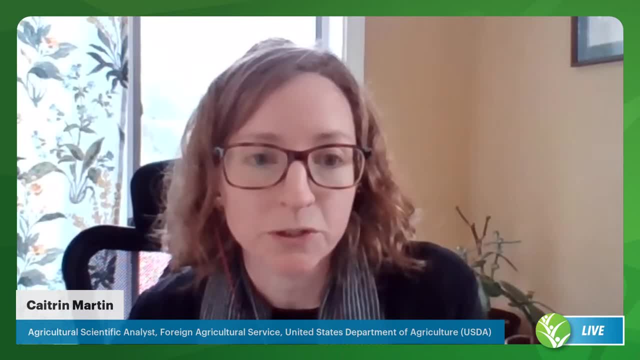 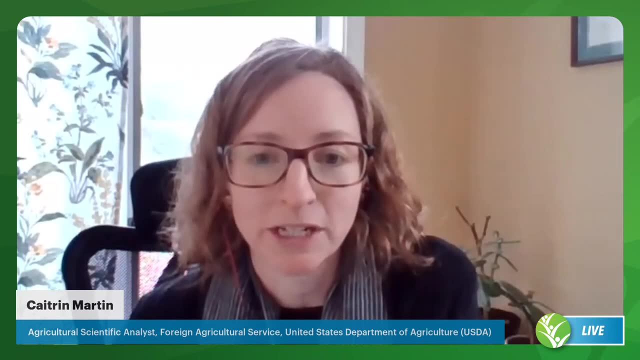 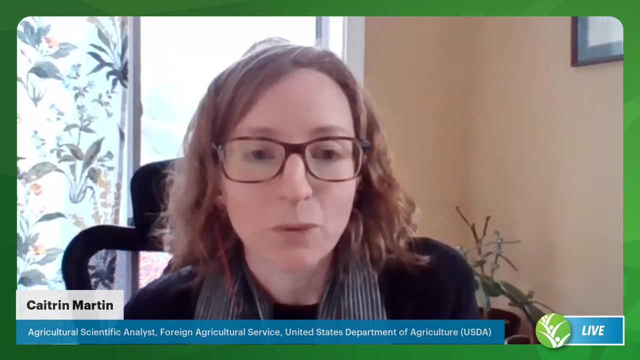 and commercialization of Kernza grain, which is the first commercial perennial grain in the United States. These solutions and innovative partnerships are vital to more sustainable land use and global food and nutrition security And, like all global challenges, we need global solutions And, of course, international collaboration cooperation. 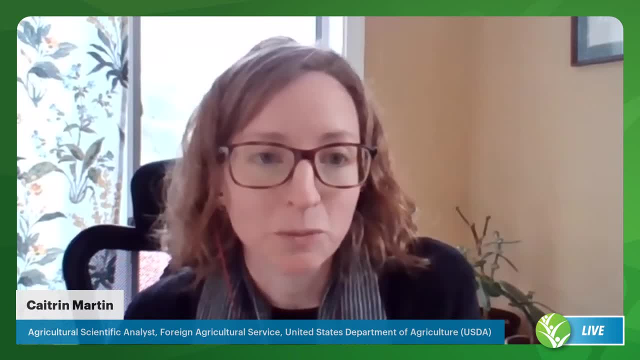 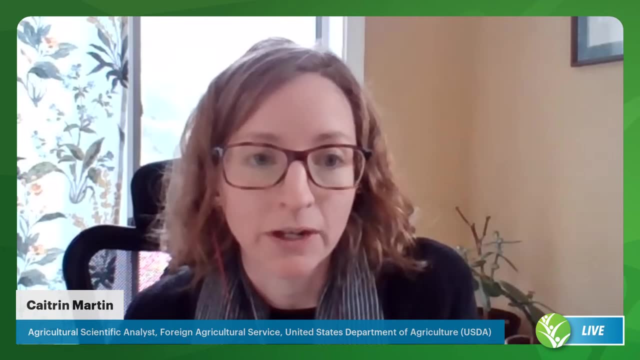 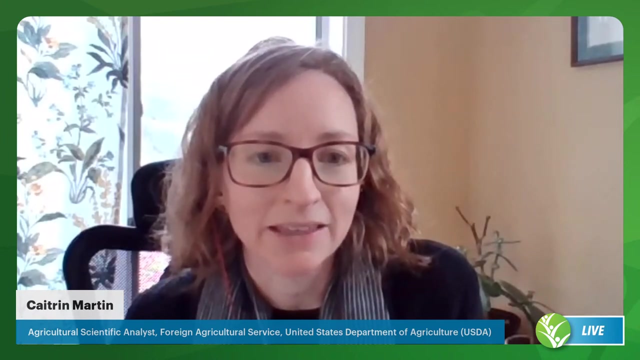 USDA is committed to working with all partners and we truly value multi-stakeholder dialogues like these, where we can advance shared goals through research, collaboration and knowledge sharing and policy dialogue, And I'll stop by mentioning that next week, USDA is holding its 98th Agricultural Outlook Forum. 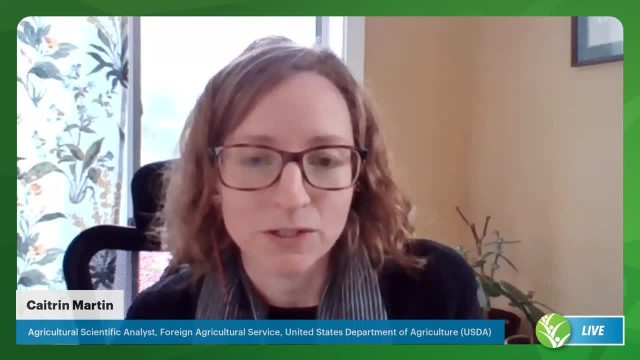 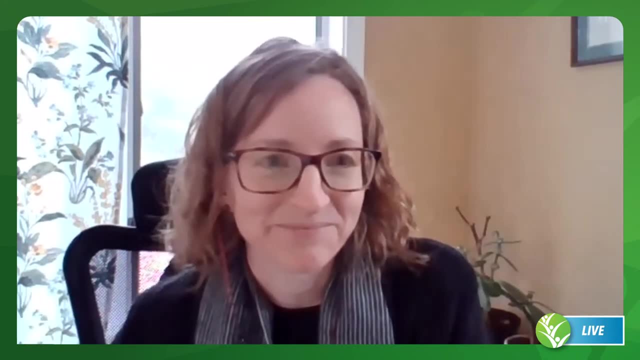 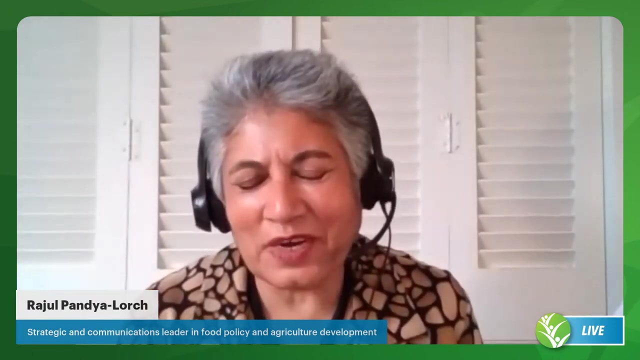 and there are some relevant topics. The theme of this year's forum is New Paths to Sustainability and Productivity Growth, So I'll stop there. Thank you so much for the question, Thank you. Thank you so much, Katrin. This is a heroic overview, in five minutes or less, of all the many, of some of the highlights. 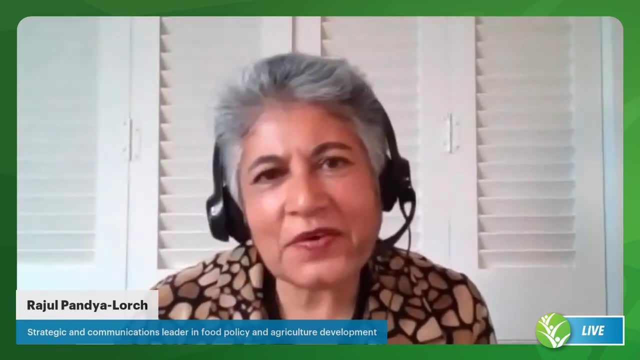 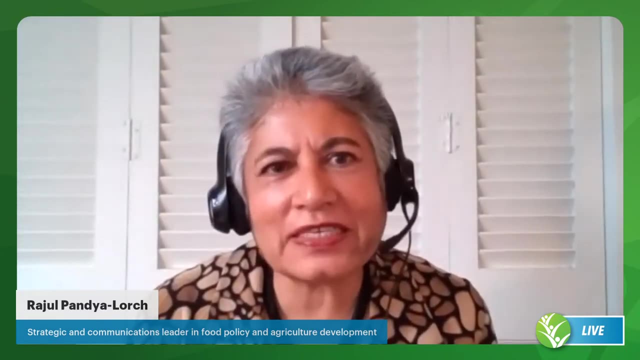 of what USDA is undertaking or supporting, And in the Q&A we'll come back to something you mentioned at the end, which is global solutions, international cooperation. So I hope we'll have a chance to discuss that And I hope that we can all come back to that at that time and come back and delve into some of these other efforts. 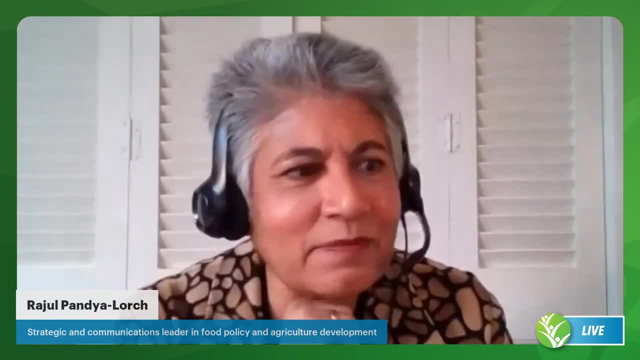 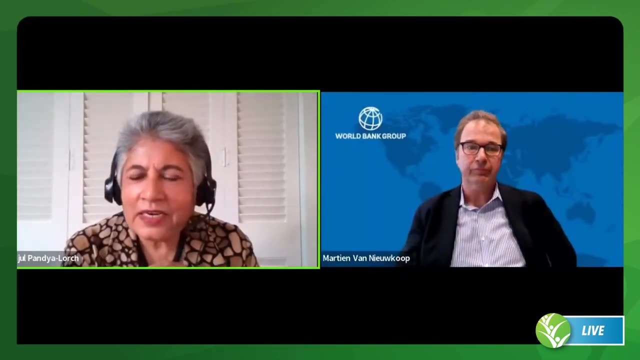 But thank you for that, Katrin. So let's move to our next panelist, and that is Martin van Nieuwkoef, Global Director for the Agriculture and Food Global Practice at the World Bank. Martin, you have heard the different scientific perspectives. 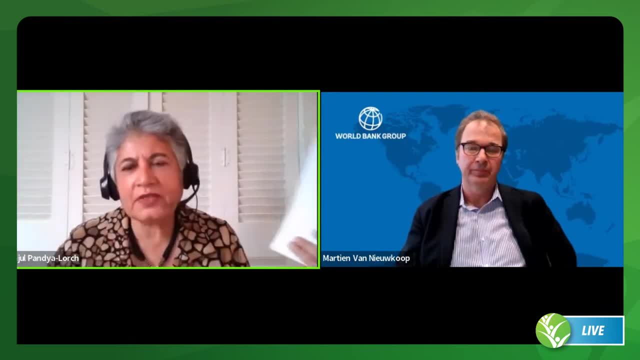 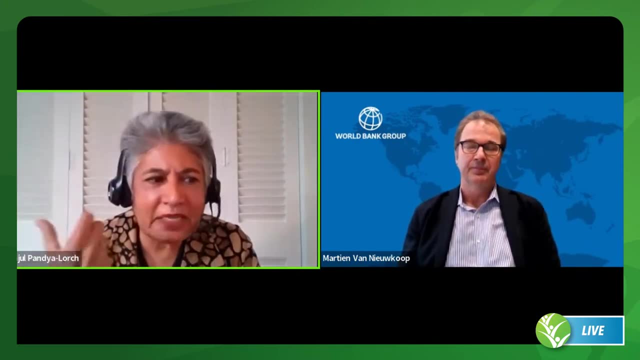 You've heard of the experiences in Malawi and the United States And I'm sure you've heard also from many different partners. What can the World Bank do to help move forward For improving soil management, saving of deforestation and land degradation? 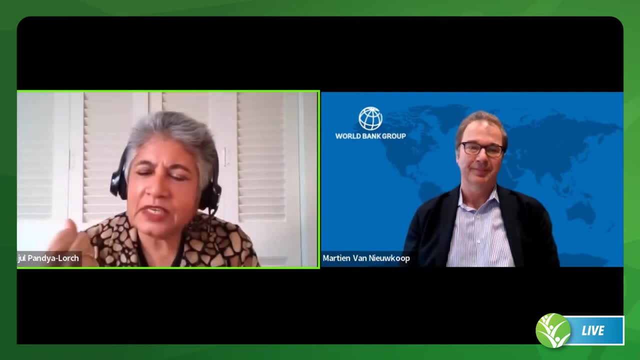 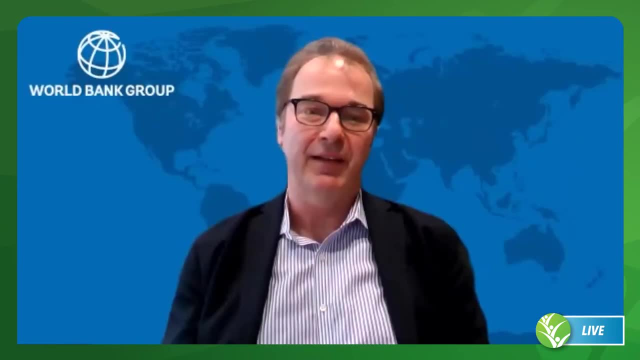 protecting carbon sinks and so forth. How can it help to move this agenda forward in a decisive way? Over to you, Martin. Well, very good. Thank you very much, Ranjula. It's a great question. Greetings to all and I'm very pleased to be part of this panel today. 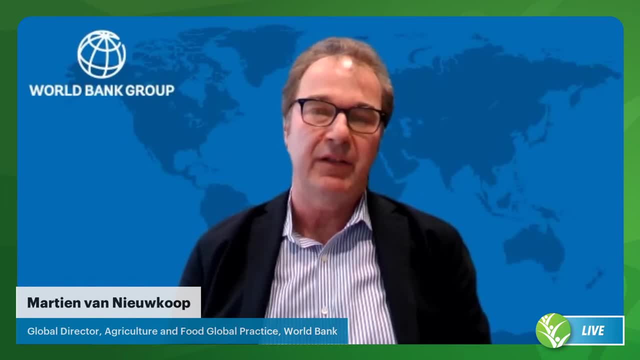 You know, let me start. you know Cornelia mentioned in the opening remarks. I mean that in 2022, the World Bank is going to be the world's largest producer of food and agriculture. I mean positioned healthy soils as a key starting point for food security. 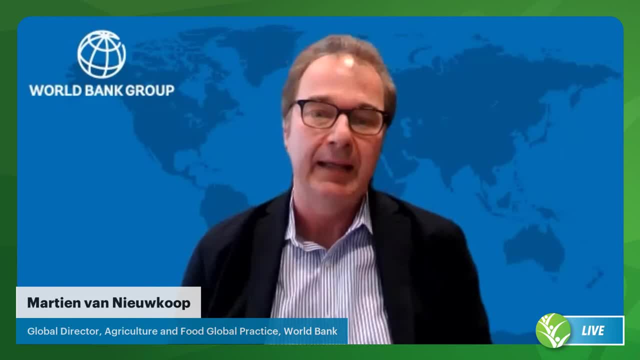 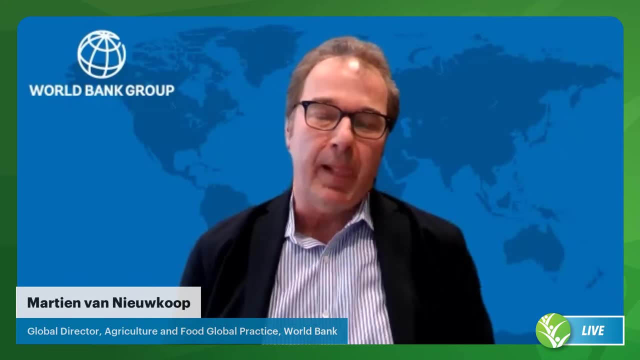 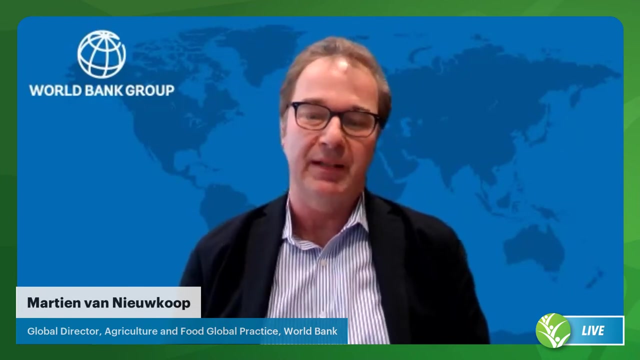 which requires global cooperation and action- This was also just mentioned- And the World Bank- let me start by saying this- and the World Bank fully agrees, I mean, with this proposition. Of course, you know that proposition is also a reminder of what Franklin D Roosevelt. 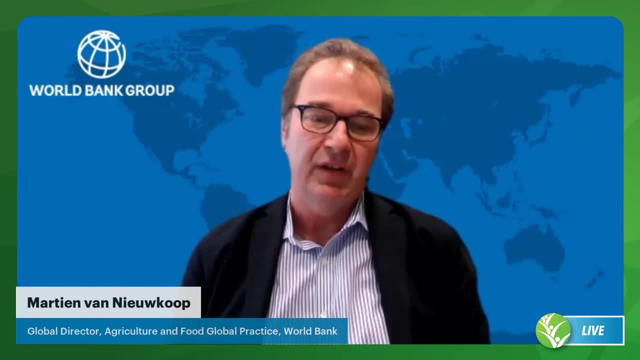 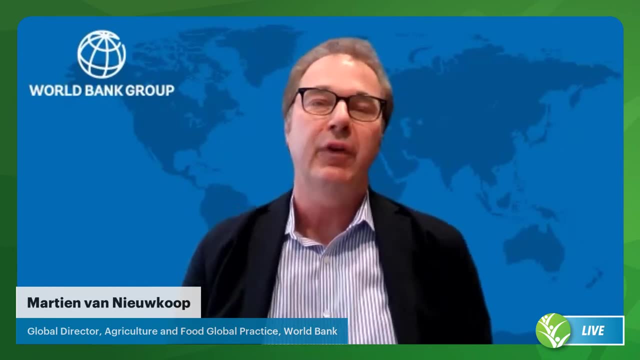 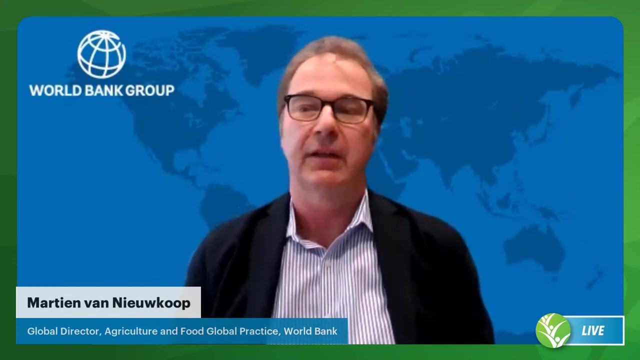 I mean the 22nd US president. the nation that destroyed soils, I mean, destroys itself. And, of course, we need urgently to reverse soil degradation and capture the opportunities that healthy soils offer, as mentioned by Professor Lal, in terms of building resilience and mitigating greenhouse gas emissions to carbon sequestration. 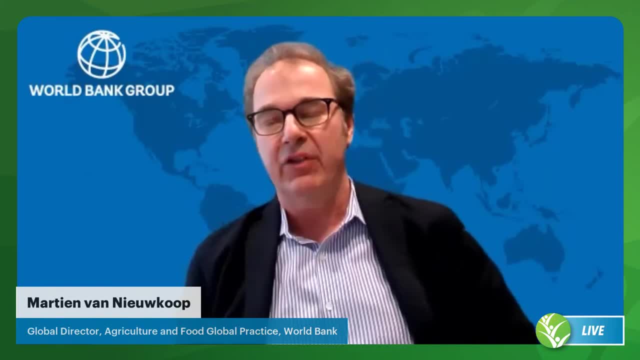 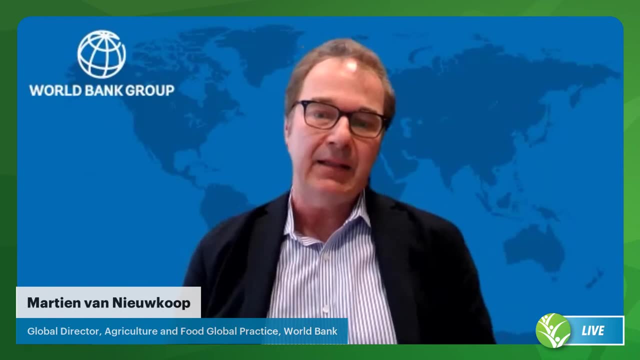 Now the World Bank, if you look at the final communique that was issued three weeks ago at the DFFA. we are supporting many elements of that communique And I can actually put them in three buckets. I mean incentives, innovations and investments. 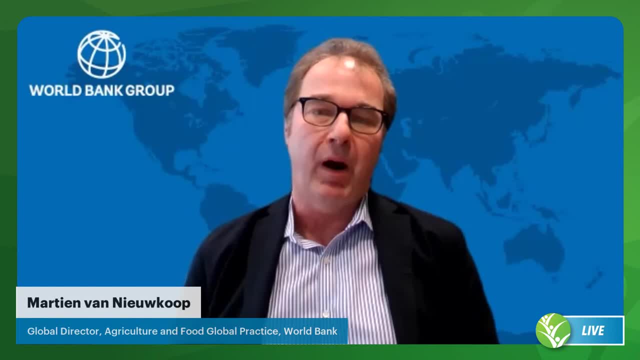 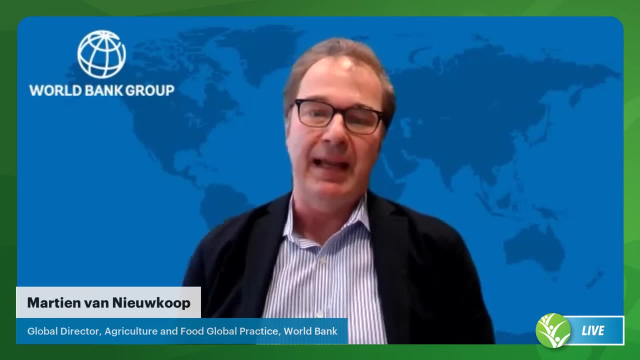 Now, when it comes to incentives, now we are working with key partners. I mean, like the UK government, to get the incentives right. I mean for farmers to invest in healthy soils and make agriculture more sustainable. Also, Joe Sweenan was talking about incentives. 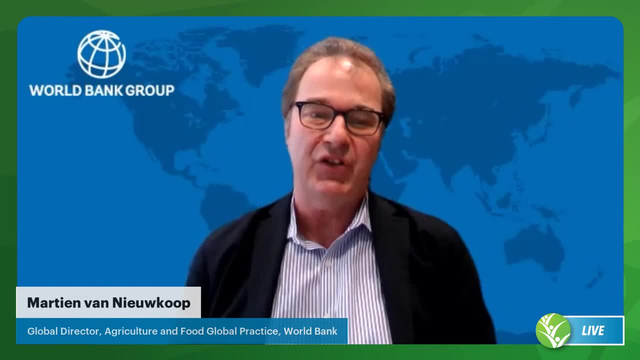 And I also like very much, I mean Professor Lal's suggestion. I mean that farmers should be compensated for sequestering carbon. Now, in our work with the UK government, we had a series of global policy dialogues, over 30 countries identified and shared experiences. 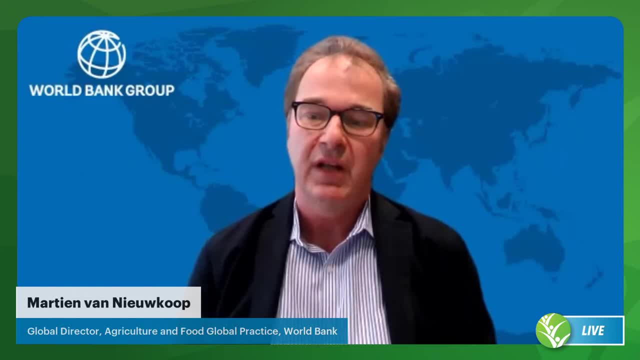 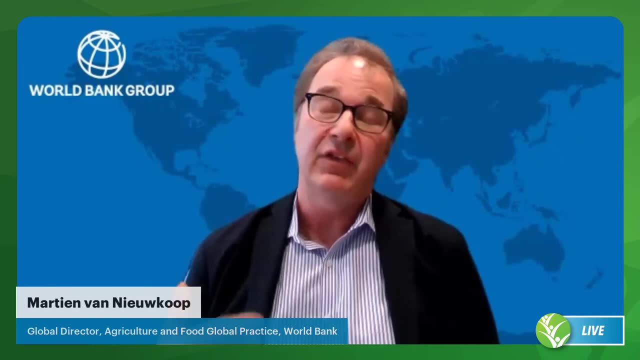 that they have taken to redirect their policies to transition to sustainable agricultural practices. And the final results of these dialogues is a policy action agenda which was launched at the COP26.. And this aims to repurpose global public support to agriculture, and this exceeds $700 billion per year. 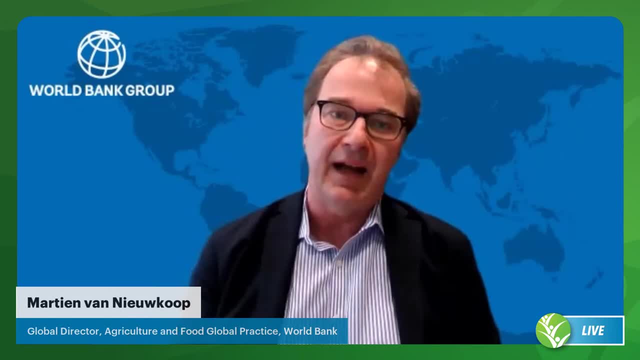 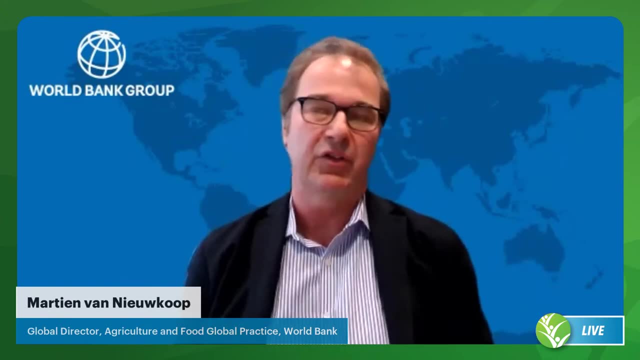 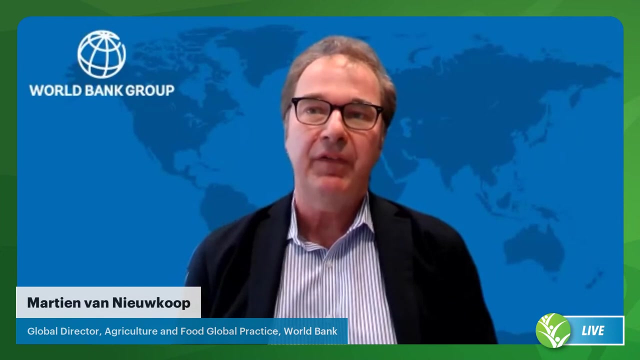 and is mostly ineffective. I mean towards better environmental, health and social outcomes. I mean through our Food Systems 2030 initiative, which is supported by Germany, the UK, the Bill and Melinda Gates Foundation and the Netherlands. we are working right now in 15 countries. 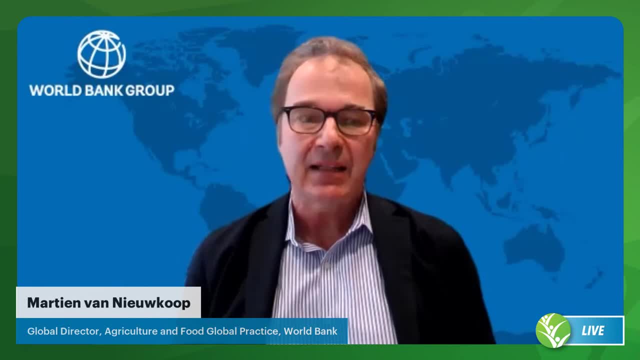 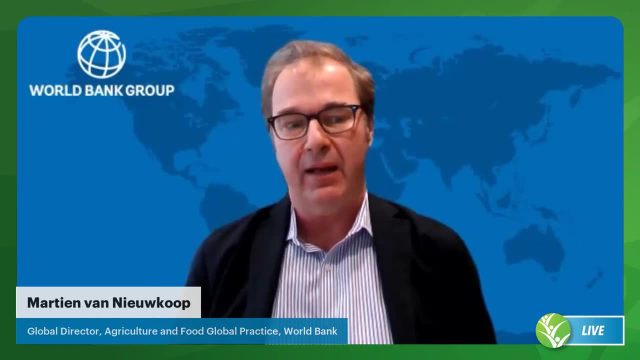 to identify repurposing options and assess- I mean- the specific trade-offs and synergies of their existing agricultural policies and public spending. And a key part of this is equipping the countries- and the farmers I mean- with the critical data that they need on soil health. 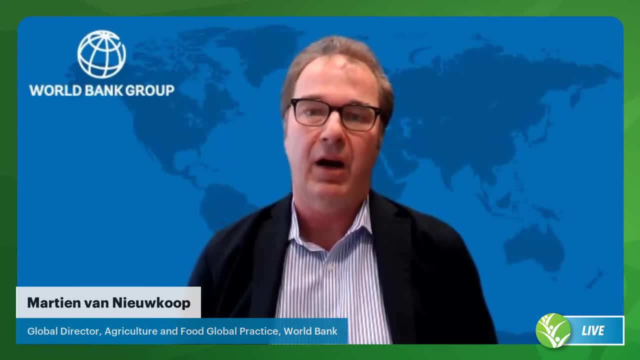 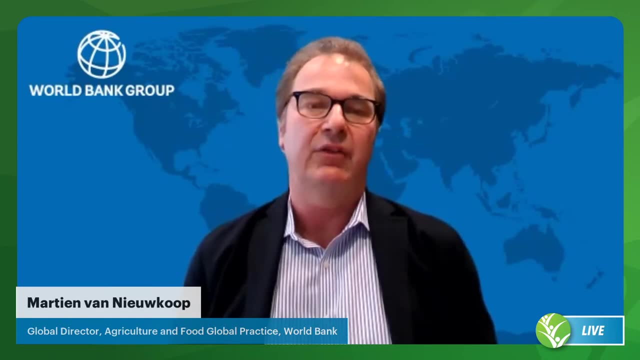 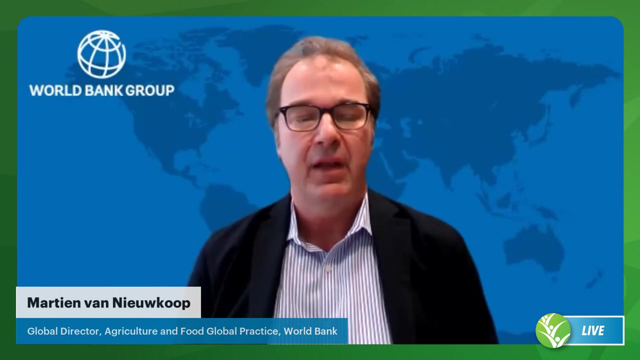 Accurately accounting for soil organic carbon changes. you know, accounting for those changes is a very important lever, we think, to unlock climate financing for soils, which is currently lacking. We recently identified innovative approaches and public guidance in a source book on soil organic carbon measurement reporting. 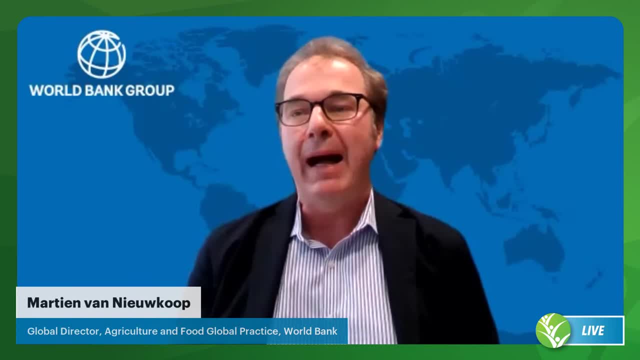 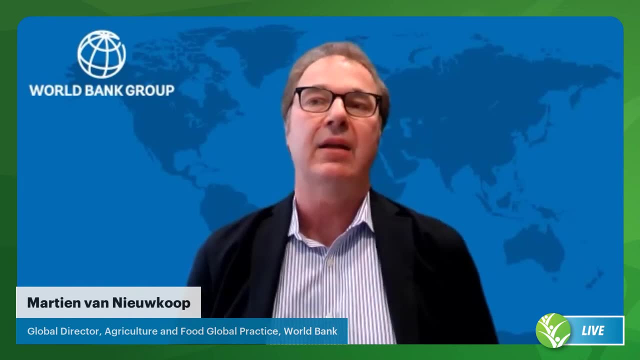 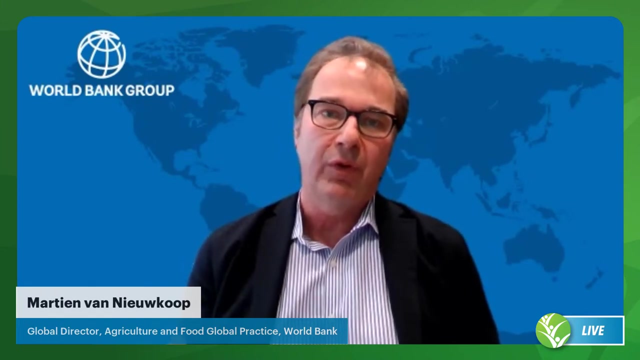 and verification and we are looking- I mean to pilot- such approaches in our client countries. Now the second bucket in the areas of innovations. so we are working with public and private partners to build foundational global data and analytics and we are supporting the development of digital agricultural ecosystems. 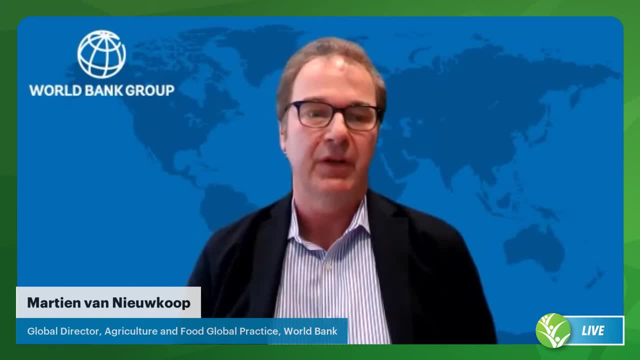 for smallholder farmers. I mean to increase their incomes and their livelihoods through transformation of the food system. An example is the Accelerating Impacts of CJR Climate Research for Africa project, in which we are working to deliver climate-smart African future, developing the first soil carbon monitoring. 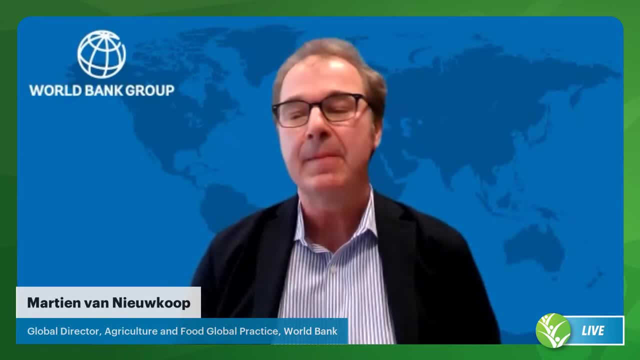 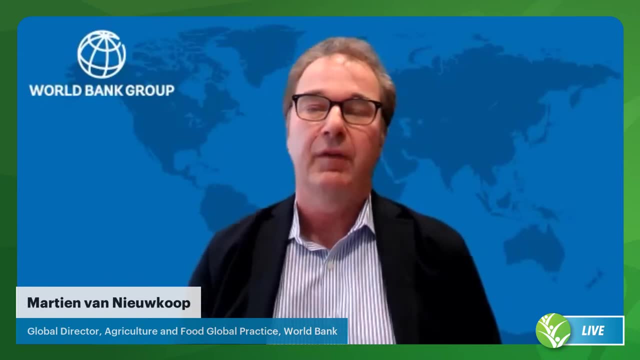 prototype and soil carbon maps of Eastern Africa as well. as you know, we are working on digital solutions to optimize, I mean, the location-specific fertilizer recommendations, Also through our flagship report that came out last year on digital transformation of the agro-food system. 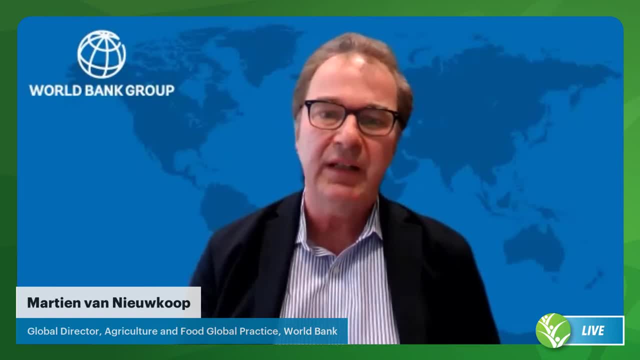 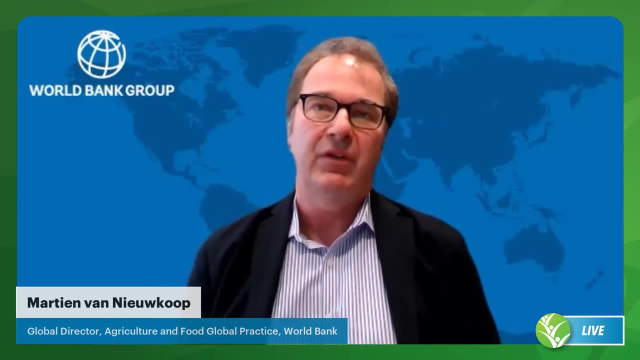 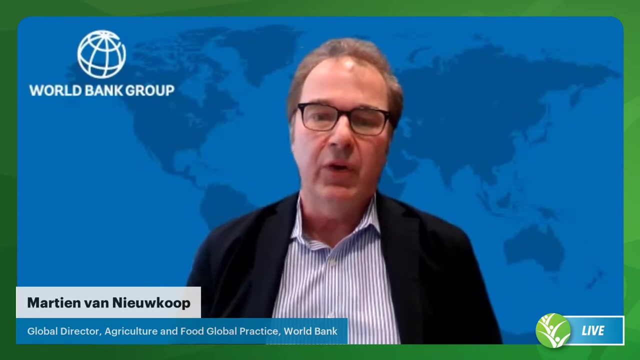 I mean we are exploring, you know, how digital technologies are improving the food system and providing, by doing so, a roadmap for countries. I mean to scale up their own digital agriculture. Now, finally, on investments, You know these are urgently needed. I mean to scale up the solutions. 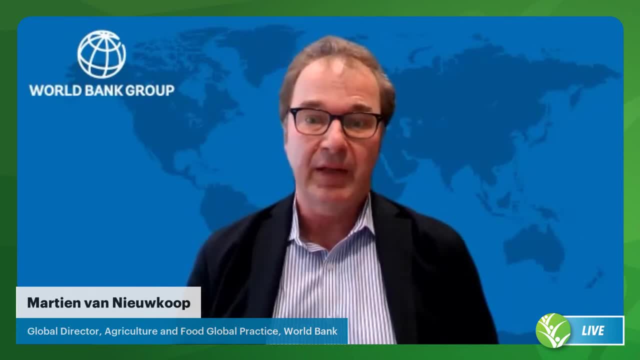 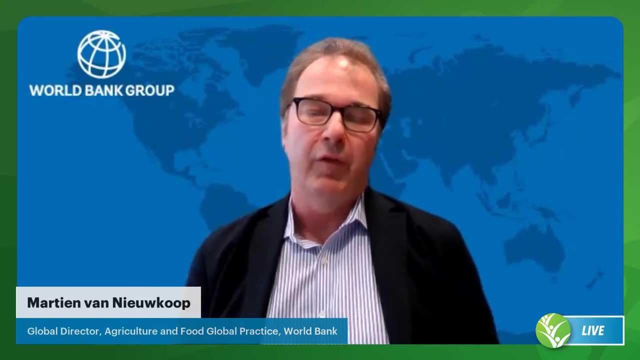 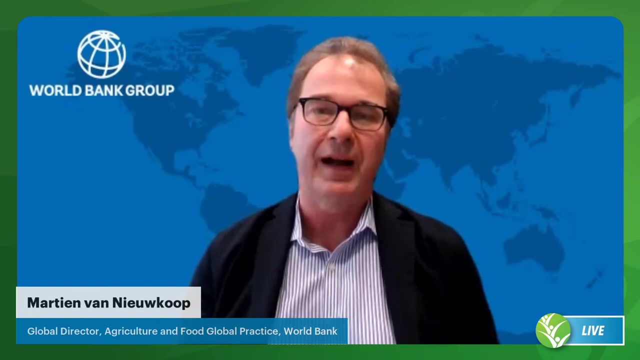 that work for farmers and build climate resilience. I mean. the World Bank is the biggest provider of development financing for agriculture and food. We have a portfolio of about $20 billion in financing for agriculture and food-related projects and we do about $4 to $5 billion new lending for agriculture. 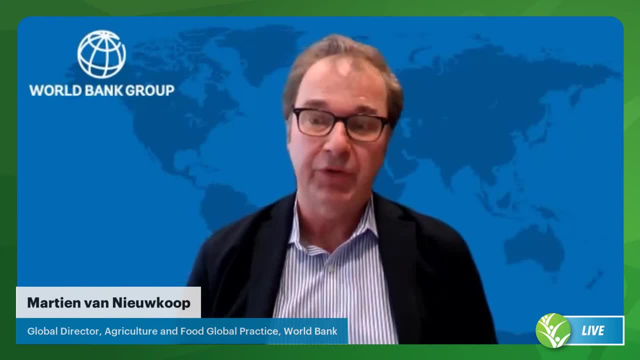 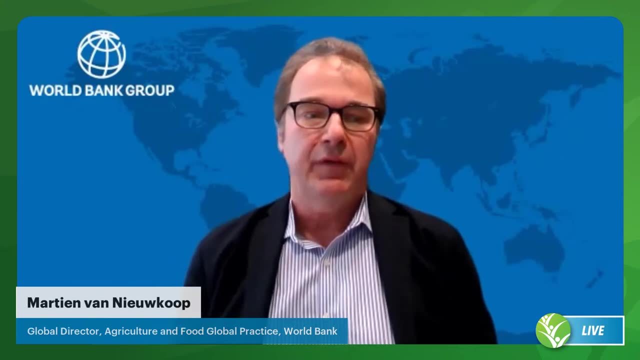 and food annually for agriculture and food. And we have increased, We have increased our annual financing for climate action in agriculture and food by seven times, I mean since the Paris Agreement, I mean, and last year we provided nearly $3 billion. 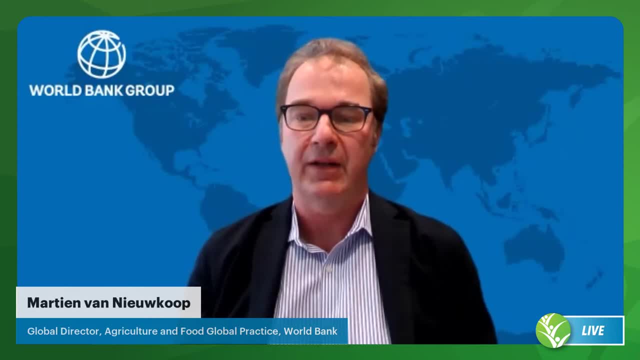 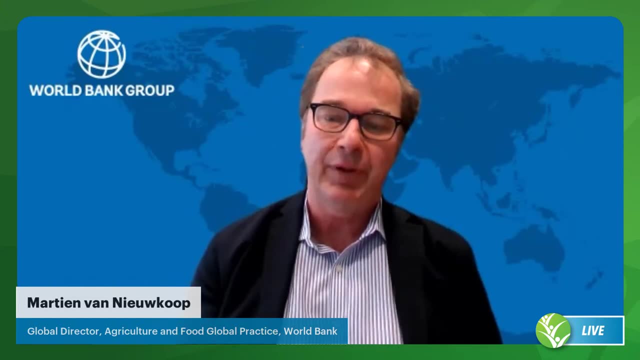 in climate-related financing for agriculture and food in the last financial year, And also on the private sector side. we think that's very important. We are working to translate- I mean voluntary principles, CSR- into mandatory ESG environment, social and governance standards. 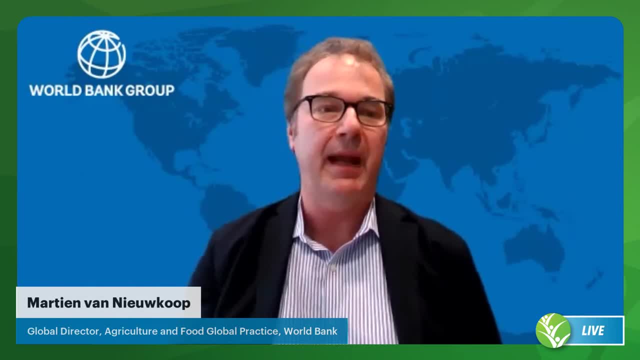 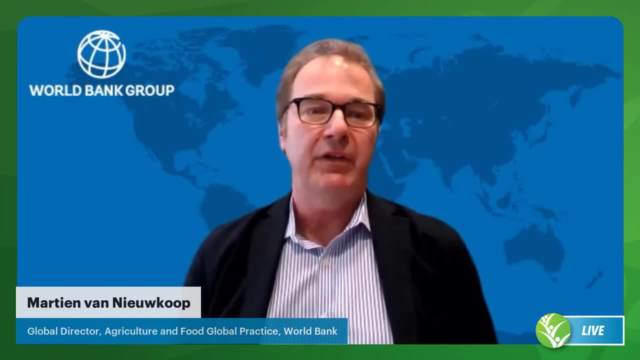 I mean working with the World Benchmarking Alliance. in this respect And as part of our investments, we are very much engaged on the great green wall, which was mentioned in the GFFA communique and was also mentioned by Cornelia in her opening remarks. 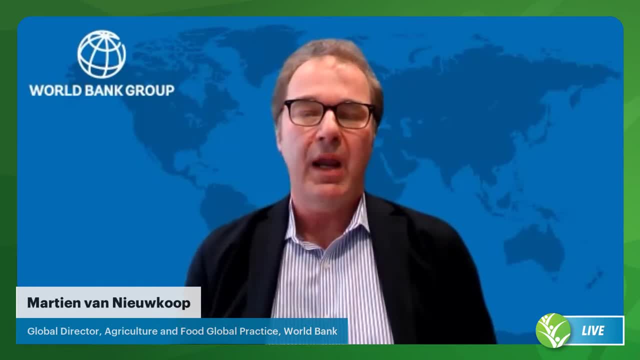 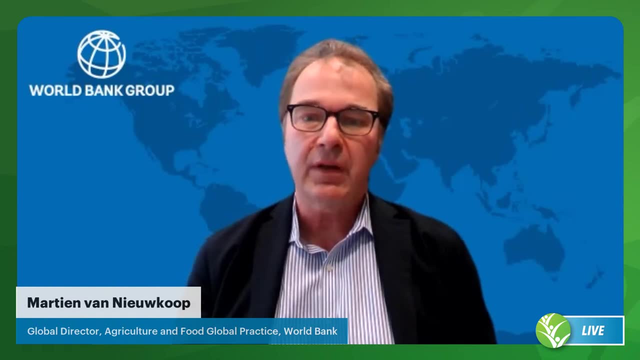 where we have about $5 billion. I mean to ongoing and newly planned projects in 11 countries. in support of that, We're also investing in the protection of forests and the restoration of landscapes. I mean to two To two, Two impactful programs. 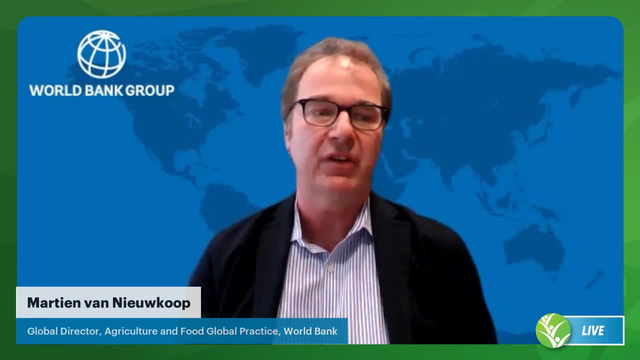 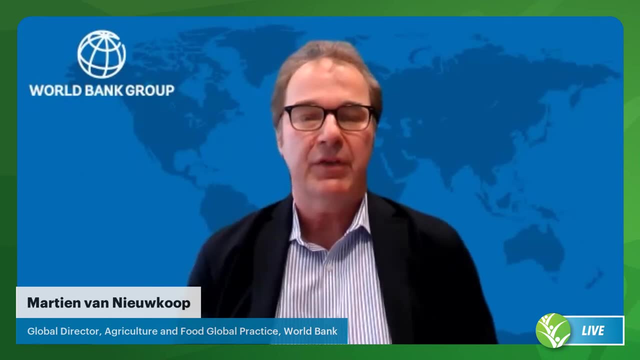 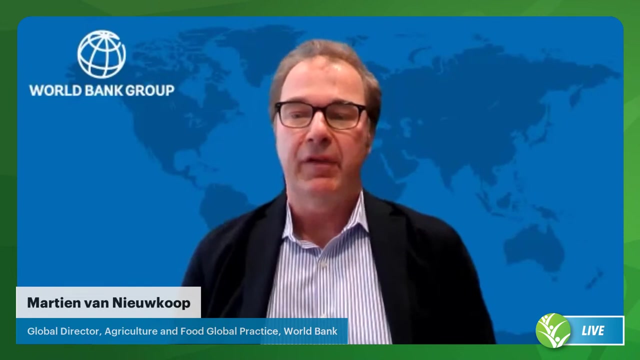 I mean FOLUR, or the Food Systems, Land Use and Restoration Impact Program, which is funded by the Global Environmental Facility, and PROGREEN, or the Global Partnership for Sustainable and Resilient Landscapes, So we can push the envelope there and do frontier innovations. 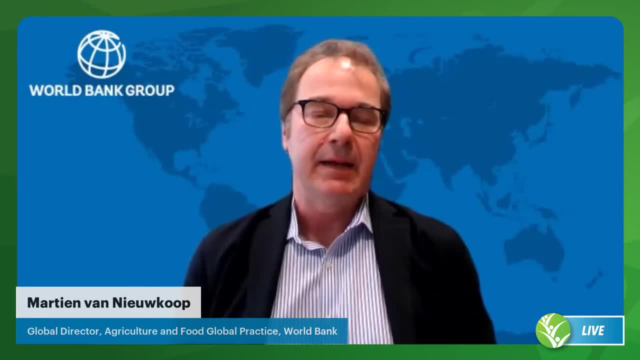 and activities And these programs recognize, which was also mentioned by previous speakers. I mean that it requires all of us to make this change And that new ways of working together- Rajul- are essential. I mean to create better food systems. 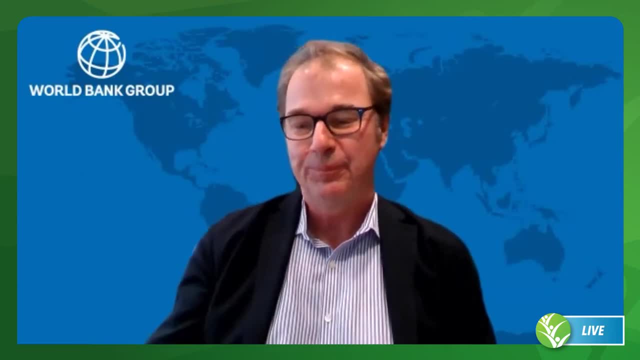 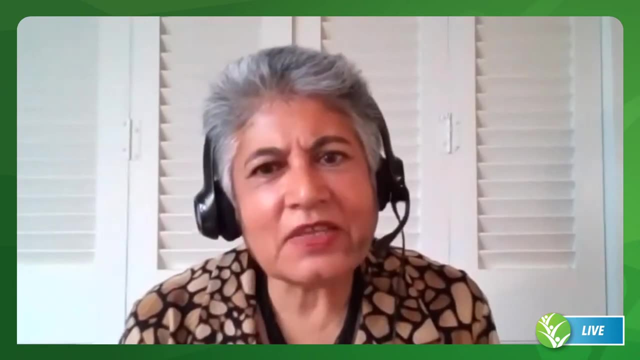 So that's from my side, Thank you, And back to you, Rajul. Thank you, Martin. That was another masterful summary overview of all the different World Bank efforts And I really like the three buckets that you put together: the incentives, the innovations and investments. the three I's. 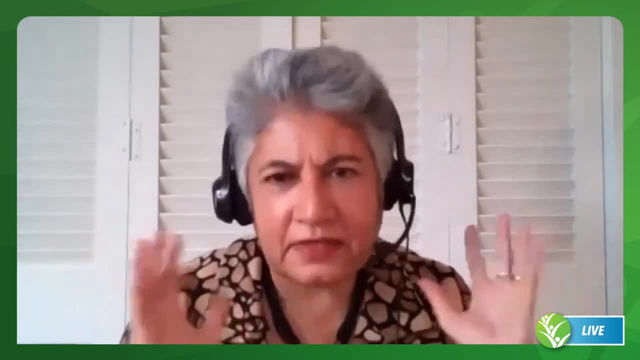 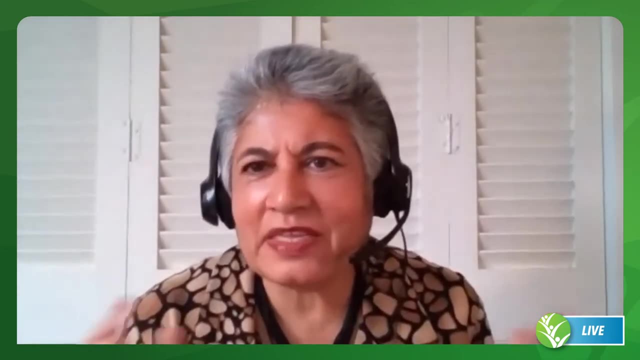 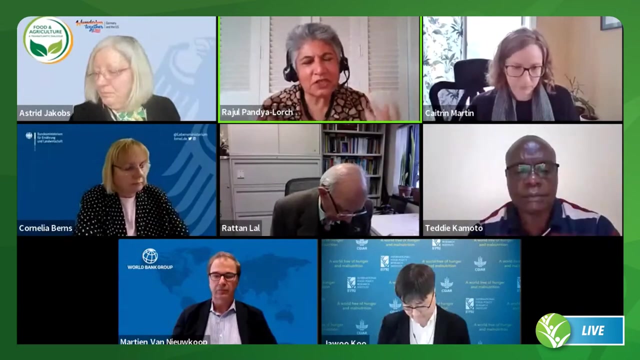 Very powerful way to think about how we can support this agenda moving forward. So colleagues are watching this event from around the world. I'm sure you will agree with me that we had an incredible panel here: a very deliberate, very insightful and a very rich set of ideas. 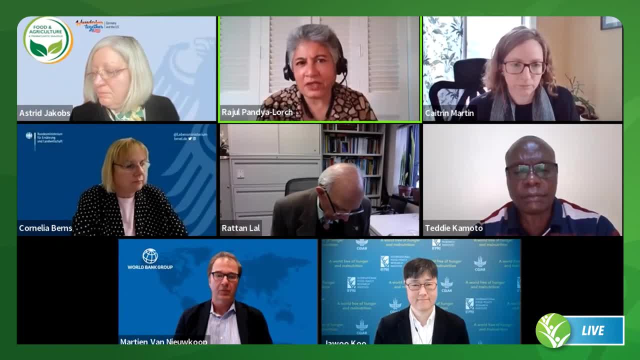 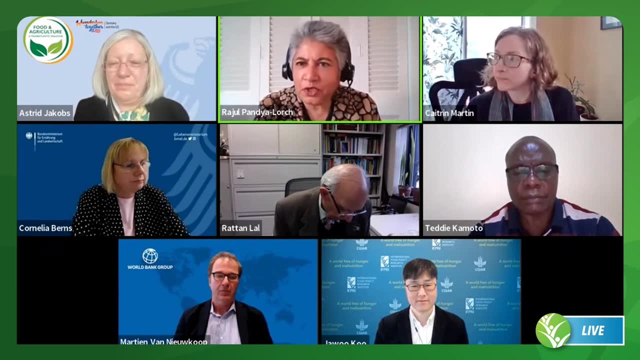 put on the table, from our scientists, from our national policymakers, from the international organizations and so forth. I would like us to move forward to the Q&A portion. And a reminder again: please feel welcome to submit your questions and comments in the different platforms I've mentioned. 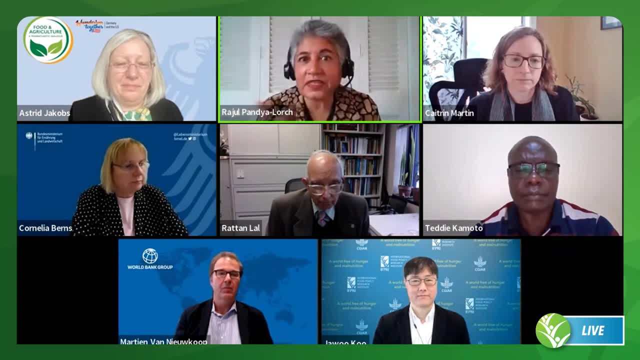 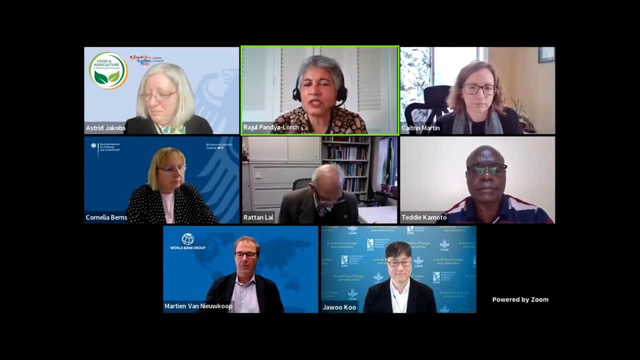 I also ask the panelists if they wish to also ask each other any questions. give me a signal. Let's have a dialogue between us. also, you know, in terms of things that you heard from each other that you want to do. 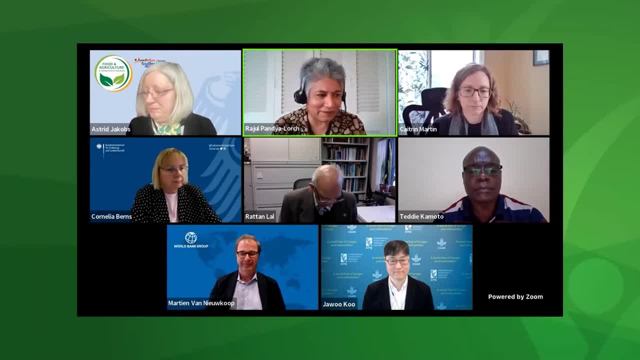 Follow up and probe, Give me a signal That will make it interesting. So I will read a question at a time and I will indicate the person to whom that question is directed, And I will ask our panelists: be brief but be insightful, so that we can have 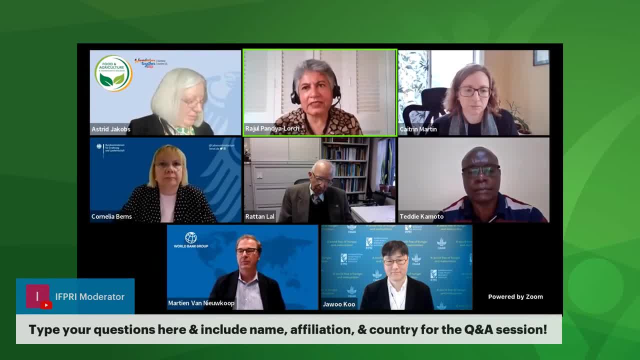 as much conversation as possible. Thank you, Thank you. Thank you very much, Dr Chandra. I'm sure there are a lot of questions that we have from the audience as well, So I will try to answer as many as we can with the audience and among. 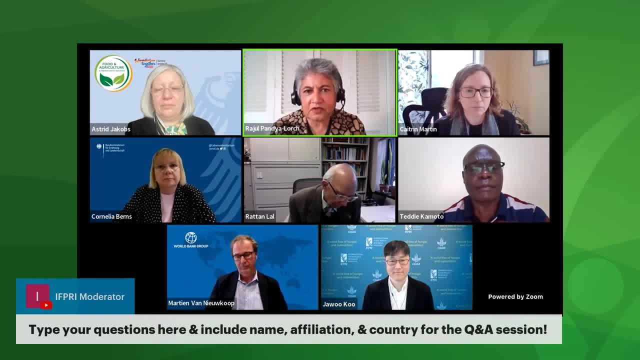 ourselves, And I notice we have several questions that have come in, So let me pick up on those questions that are coming in and go from there, as well as other questions from other platforms. The first question I would like to direct is to Professor Lal. 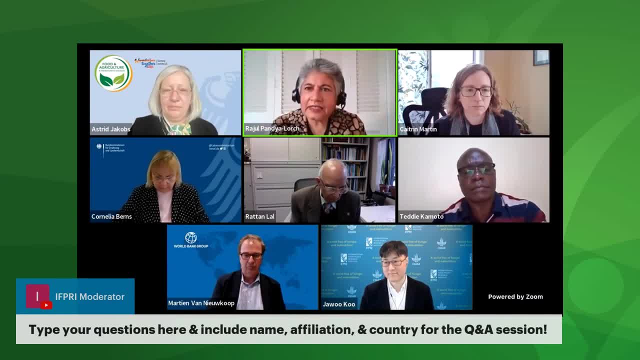 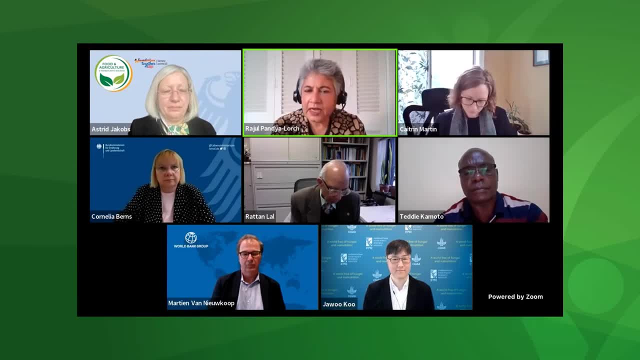 Professor Lal, one of the questions- and this has been raised several times- is about soil carbon stocks. what is the scientific evidence about the permanence or non-permanence of soil carbon stocks, and what, then, should we be thinking about in the future? over to you, professor lal. 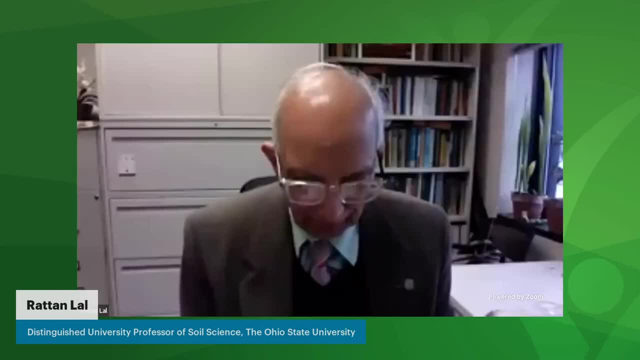 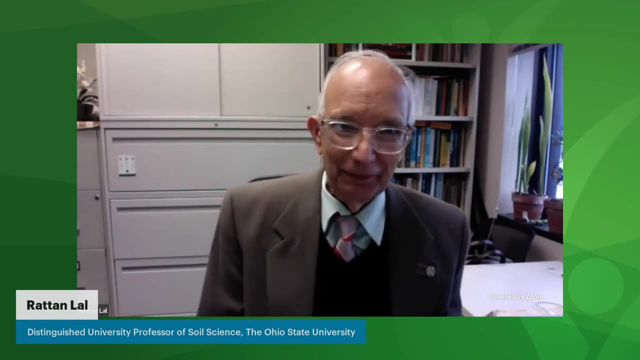 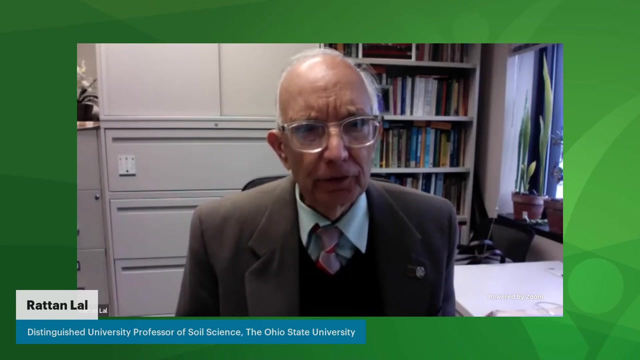 thank you. that's a very good question and people are discussing this in many meetings. if carbon put in soil and land, is it permanent? nothing is permanent in this universe. everything is changing. the question is how long it can stay. let's take the case of conservation agriculture. if you adopt conservation agriculture and the soil is kept covered all the time with 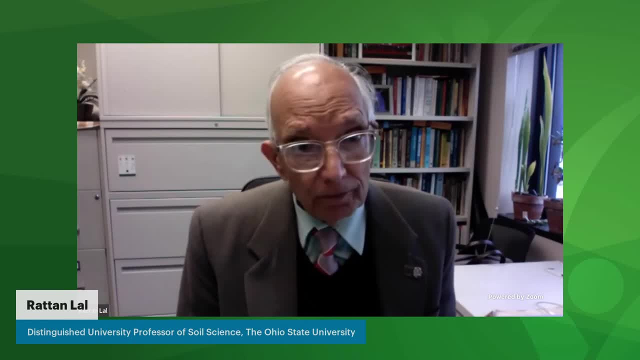 cover crops and crop residue mulch and it's not plowed, that carbon will not go anywhere. but if that soil is disturbed, of course the carbon will go back into atmosphere. and so the question is when you reward farmers, just like in the case of crp and wrp. 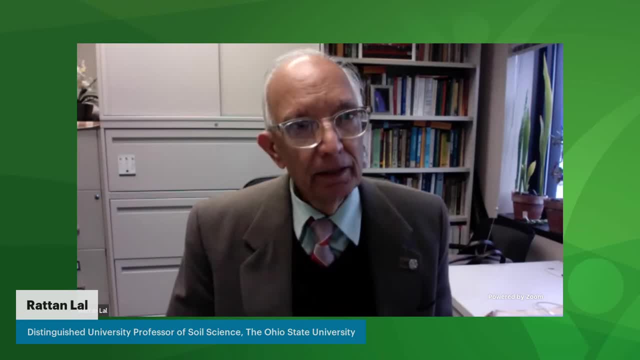 we are avoiding them. if they do not disturb the land, the crop residue back on the soil and grow a cover crop in the off season, and that is the reward, for they will be rewarded if they practice that. they will not be rewarded if they don't. if they practice it, soil carbon will be permanent. this is the organic carbon, inorganic carbon, which 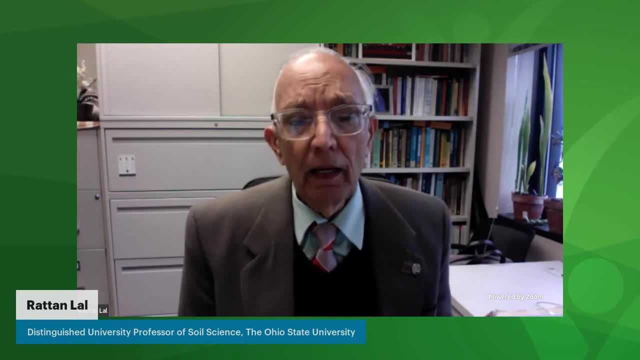 has not received much attention. it must is very stable. so formation of secondary carbonates, formation of bicarbonates, and they're leaching into the ground water and then precipitation there as a caliche many times you see, and the drier climate, which are about 42 percent now. 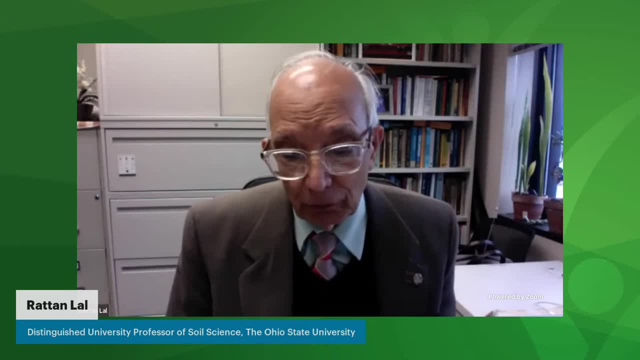 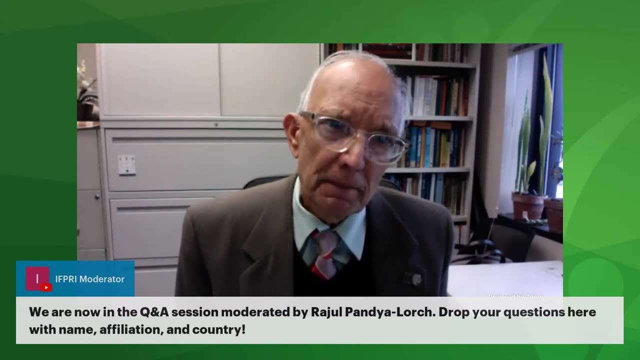 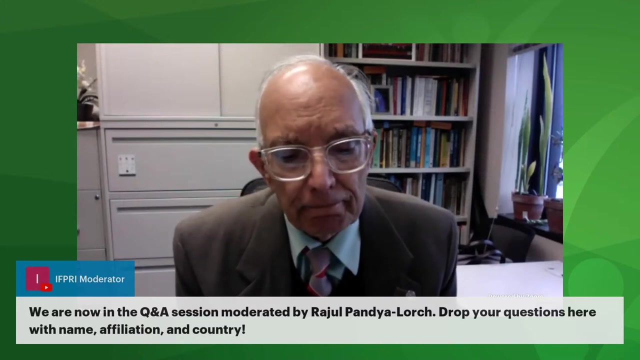 of the world. they may become 50 percent uh by 2050 or so. secondary carbonates: carbon sequestration is very critical and they are very stable. uh, very briefly, i think i shouldn't take too much time. uh, the question of measurement, monitoring and verification. i think it's very nice. we should. 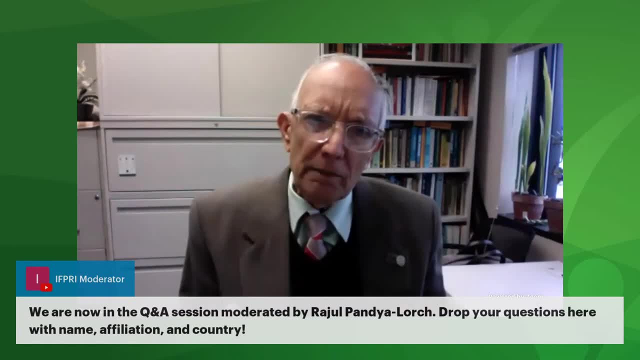 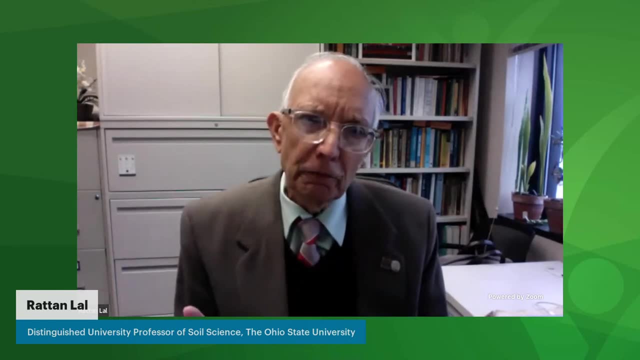 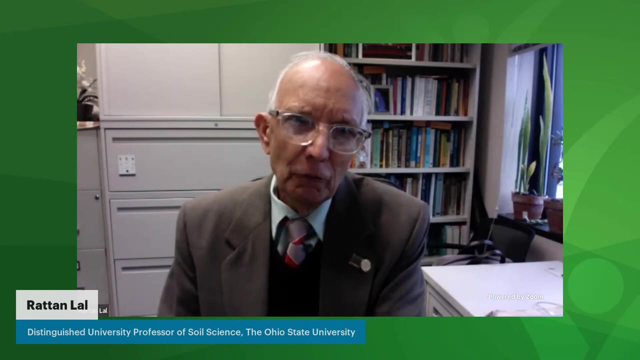 uh, promote that. but please remember, crp was not based on monitoring runoff and erosion from each acre of land, it was based on satellite imagery. if the farmers were not cultivating the land, they were paid. so let's not go too far on that. mrv which apply to geologic sequestration. 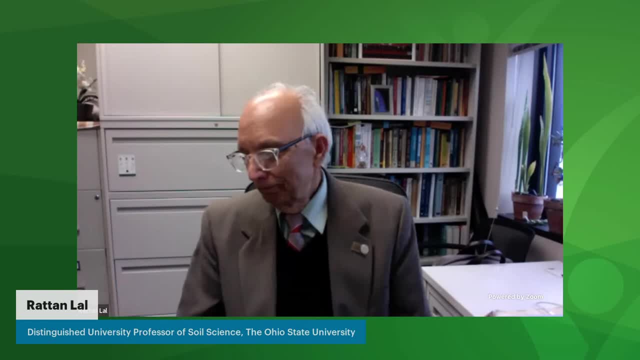 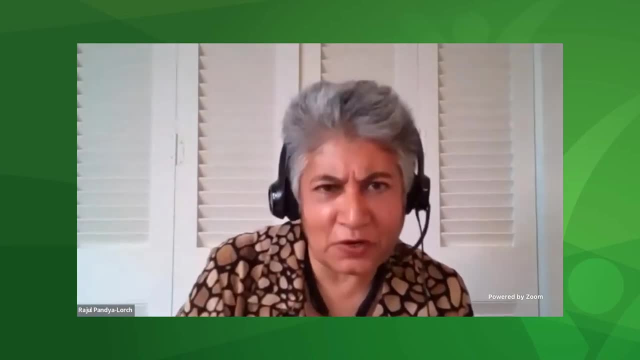 do not try to push that onto agricultural part, thank you. thank you, professor lal i. if any of the panelists wish to come in and also further comment, give me a signal, otherwise i will move us on. okay, and i'm pretty sure they'll come back to this later and as we 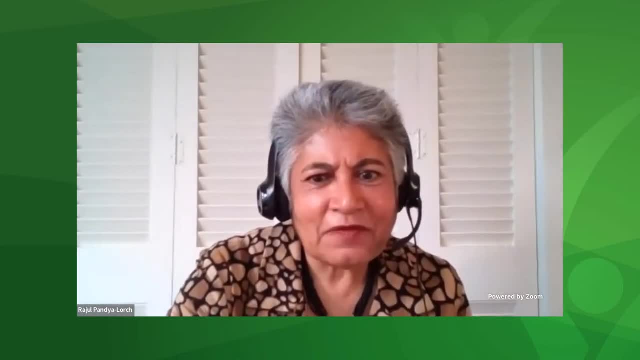 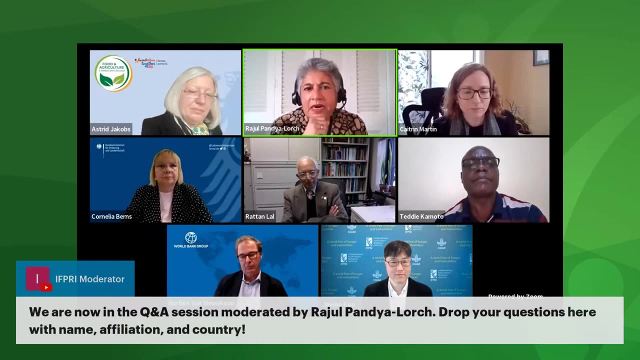 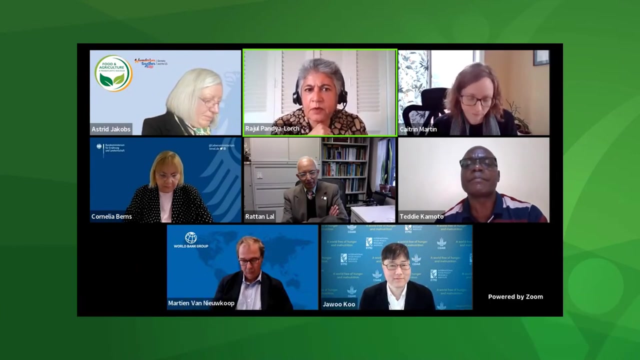 vote to you as i see questions coming in. the next question is for java and java. this question has come in from uh, from around the world, and uh, and perhaps also martin, may wish to also reflect on this question. the first, java: how cost effective will digital technology be for small, far small? 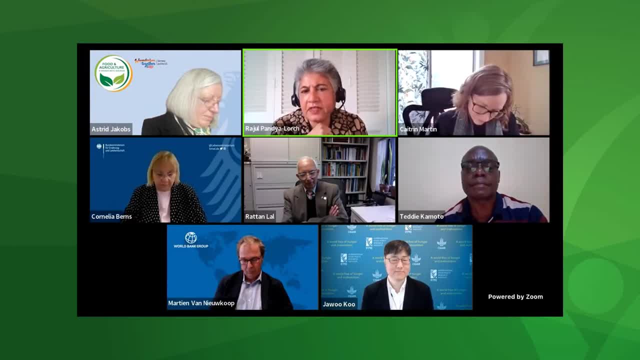 scale farmers in the world, and africa in particular, given the few commercial farmers in africa. so, java, would you like to comment on that and if martin also wishes to do that first job? yes, and that's a really good question, and that's where we really need to be careful. 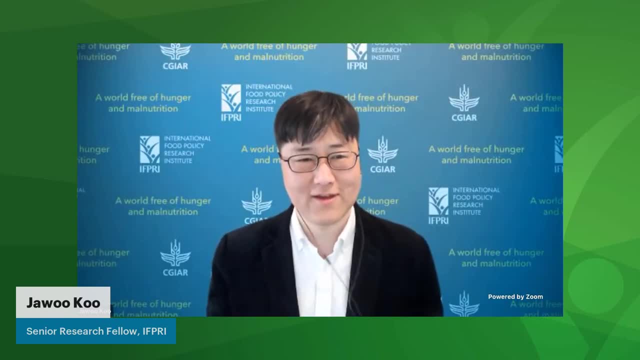 when we introduce new digital technologies and innovation. um, the adoption is totally different side of the story. so the technology should be accessible and easily understandable and there should be a continuous dialogue and communication channel between scientists and researchers who develop and provide content. and we use the farmers who use the technology and use the digital tool in the field. uh, and giving. 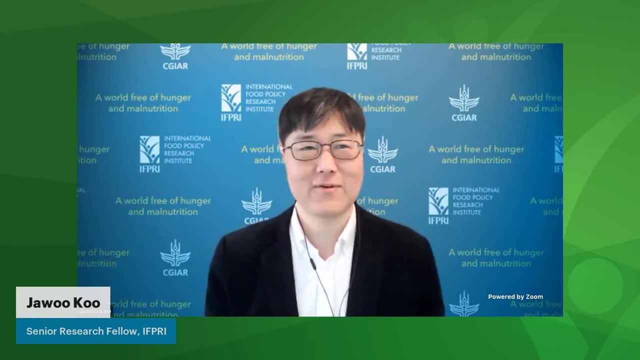 feedback back to the researchers. so yeah, it's a really difficult question. uh, in a way there are so many different types of farmers and different types of farming system for really low input system are very remote to the village. i think uh probably the easiest, the quickest way. 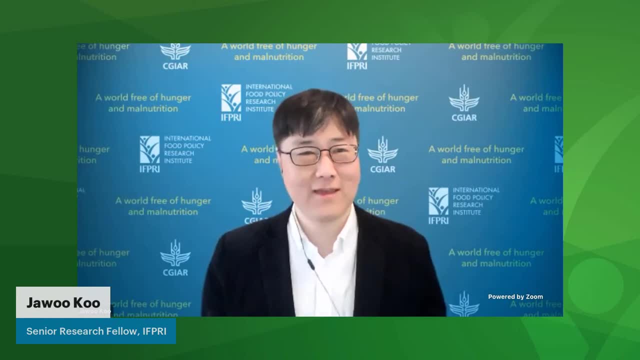 to get benefit from digital tourist weather uh and some kind of decision support tool in simplistic uh. but yeah, i mean it will be quite challenging to benefit all the remote villages uh using these digital technologies uh, especially specifically for the soil data quality issue. i briefly mentioned in my uh speech earlier on that there are like only limited fundamental data sets. 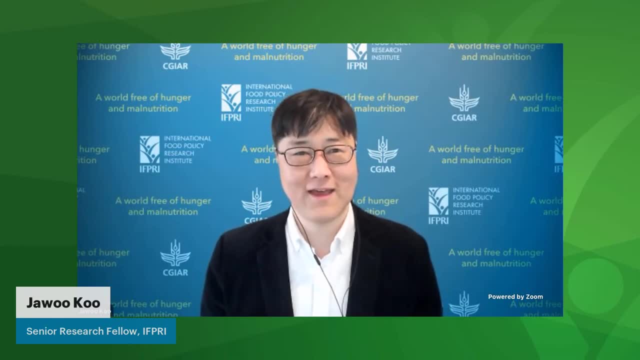 available and there are lots of ai and machine learning techniques to interpolate those data. but if those data sets are not really representative of where farmers are farming, the recommendations the researchers are giving might not be the right. um you know, advice that the most effective way to manage the story. so i think we have to be really cognizant of where. 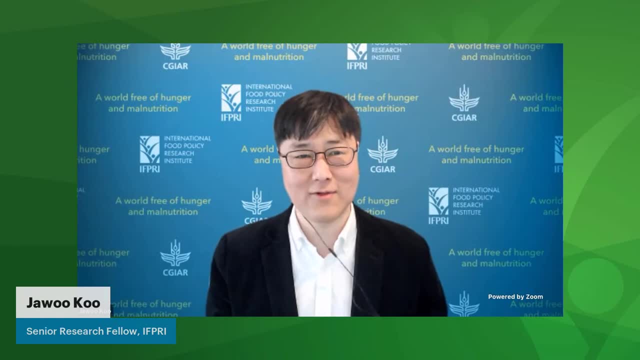 we have more uncertainties and we might even have biases the data, and that's where more research is really needed, uh, how we can best benefit from smaller farmers. thank you, java. very thoughtful reply. martin, would you like to come in also from world bank experience? yes, yes, definitely. 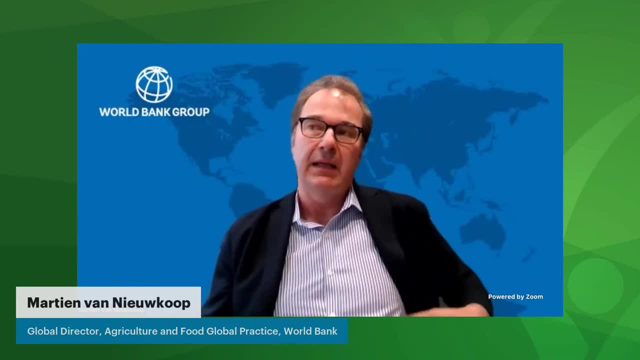 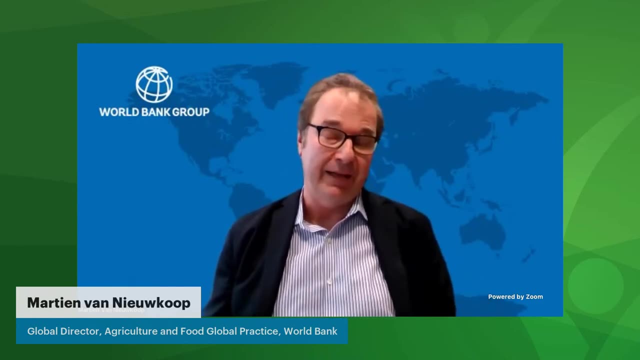 thanks for the question and thanks for julia. i mentioned in kind of my response to your first question. i mean, um, that, um, um, we came out with a reflection board on digital technologies and this is slightly culture, so and i think they're very powerful because you know, 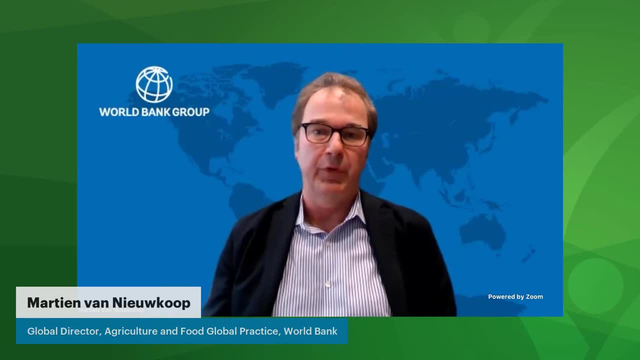 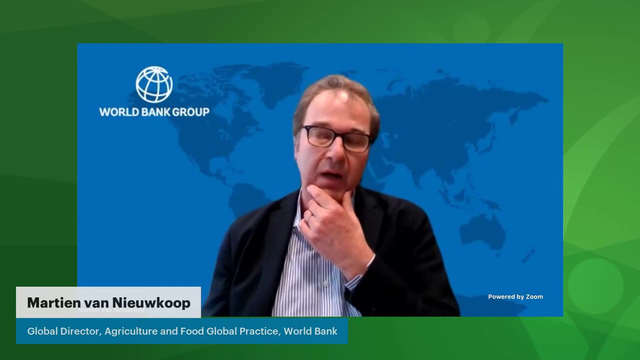 they're affecting production systems, you know, in multiple dimension and kind of simultaneous fashion. so so let me put a few considerations on the table here. one is that we think i mean, uh, in a national way related to small, far smallholder farmers. i mean we think that digital technologies 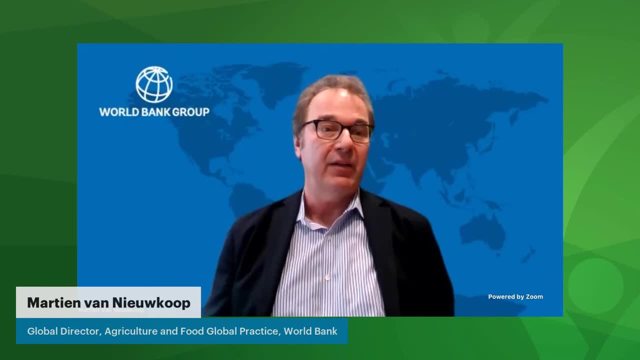 are directly actually affecting economies of scale and actually are providing opportunities for scale, i mean to smallholder farmers. i mean think about, i mean the sharing economy. i mean hello tractor, i mean that actually farmers get access to machinery that they don't know, that they don't own, but actually by taking advantage of of services, and i think that is very relevant. 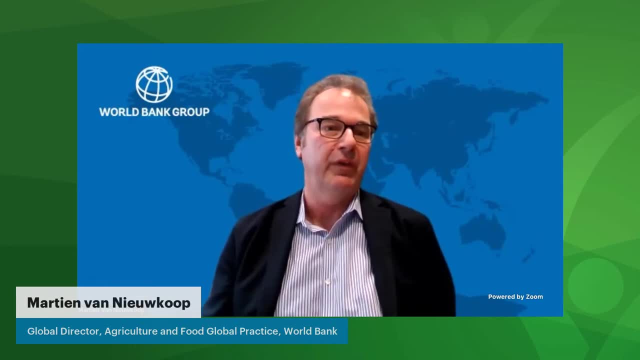 also for dr uh lal said you know, on the adoption of no tillage. you know, activities that we've been requires- I mean sometimes specialized machinery, Digital technologies, I mean- are key for precision farming, increasing input use efficiency and that. 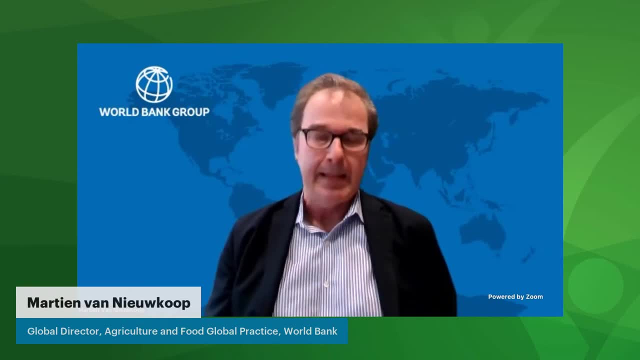 reduces the cost of farmers and improve directly the bottom line. It's very key for access to markets. I mean- think about e-markets- cutting out middlemen. I mean directly actually marketing their produce, I mean to consumers. it's a two-dimension. 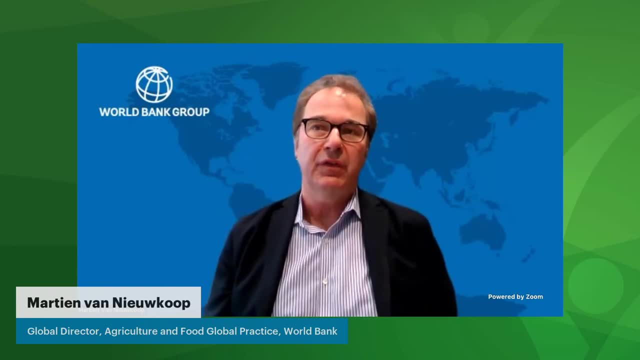 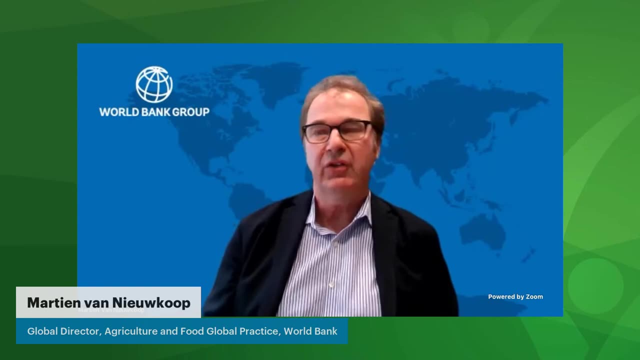 And fourth, of course, I mean the efficiency of services. I mean when it comes to the adoption of climate-smart agriculture, conservation agriculture, agroecology, whatever label you want to put on it, and Professor Lau provided quite a few examples. 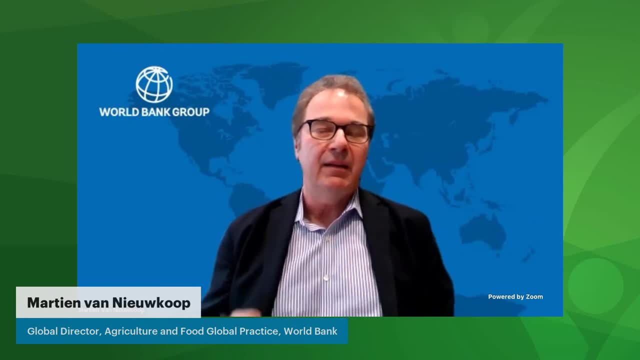 of the technologies that are available. I mean there is no silver bullet. I mean probably farmers need to adopt a consumer-friendly system. It's kind of a package of solutions. There are also no blueprints. I mean the solutions need to be tailored. 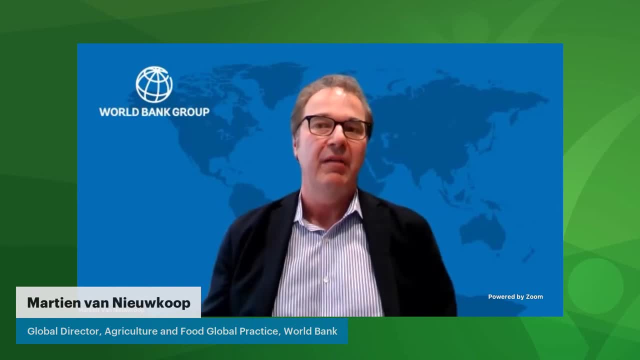 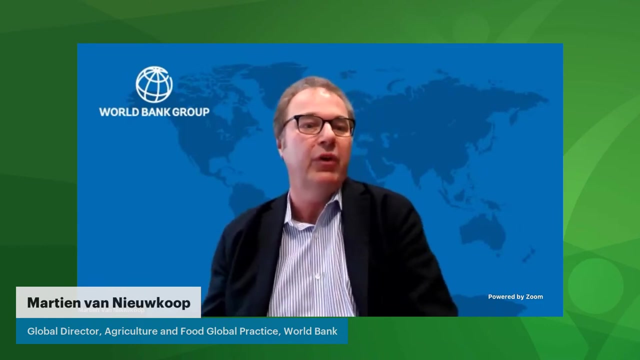 I mean to the existing local agroecological conditions. This means that there's kind of a knowledge gap that needs to be resolved, And we know that extension services in many countries are not very effective, So digital could actually play a very important role. 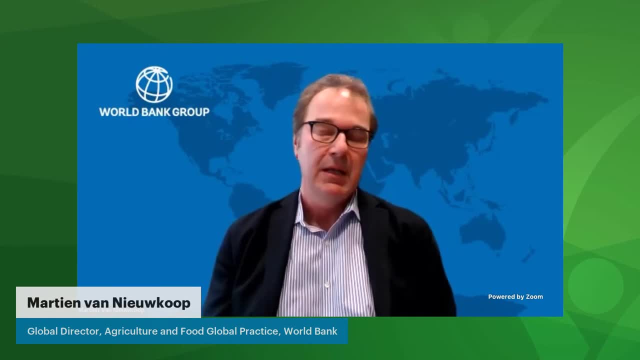 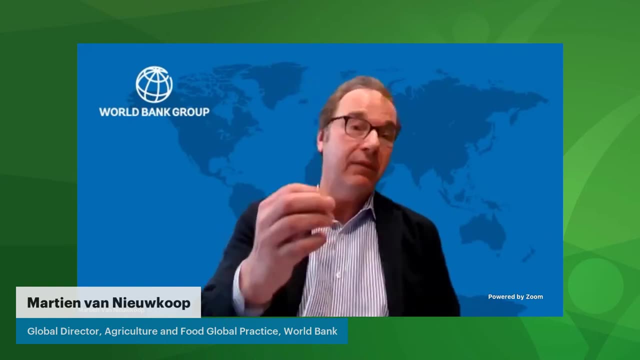 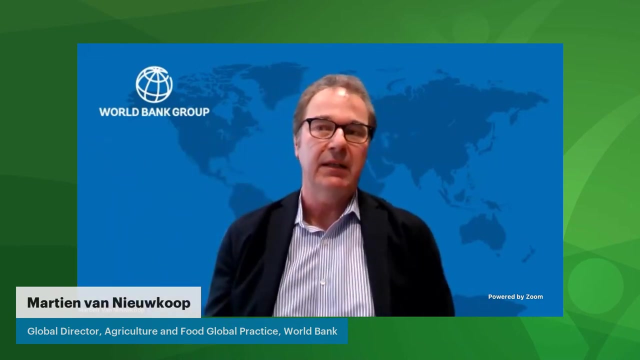 to put those type of technologies in the hands of farmers. There's a big upside on the digital revolution in agriculture. There's also a big risk, I mean we need to avoid actually that small farmers end up on the wrong side of the digital divide, because actually 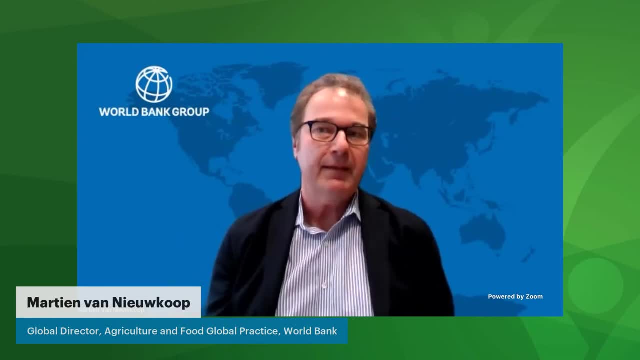 that would put them further back. And for that reason, I mean in the bank, I mean this is a high priority for us. I mean basically to capture these upsides and avoid these downsides. Back to you, Razul. 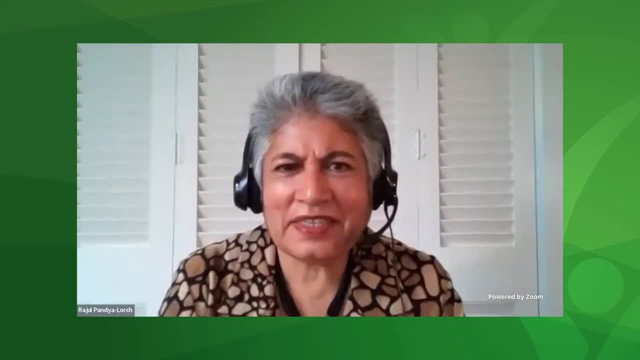 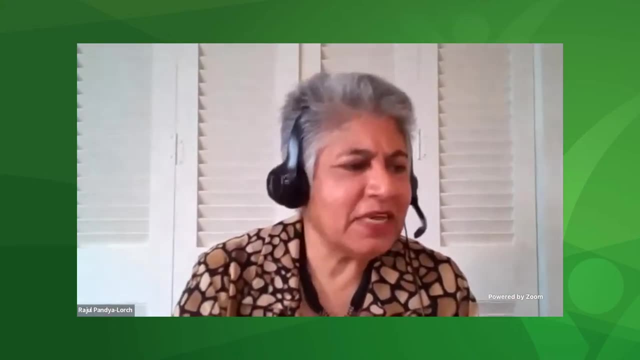 Thank you. I see Jawu nodding his head also on this one: the big, the upsides and the big risks. Let me move over to the next question. if anybody else, yeah, Katrine, I'd like to come over to you. 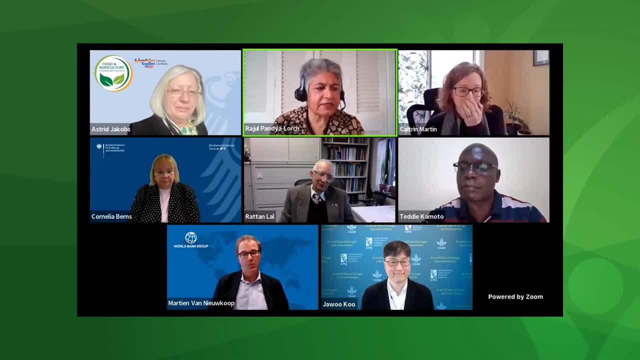 and pick up on something you had mentioned at the end of your remarks, And this is about the global solutions, the importance of global coordination, global working together, international coordination. Can you say a few words about what some of the USDA's multilateral efforts are? 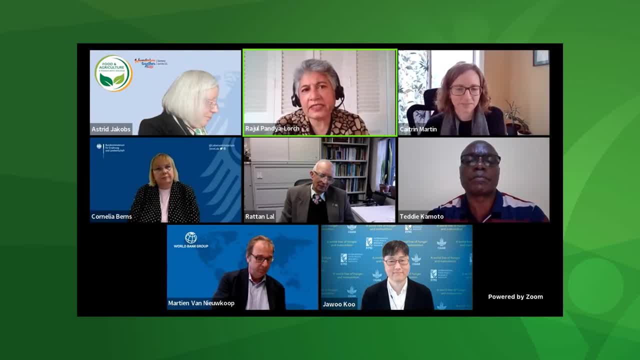 You gave us a great picture of domestic, But how is USDA looking to work with partners? And then I will come to Cornelia Burns after that on a similar question Over to you, Katrine first. Sure, Thanks a lot, And before I address that, I want 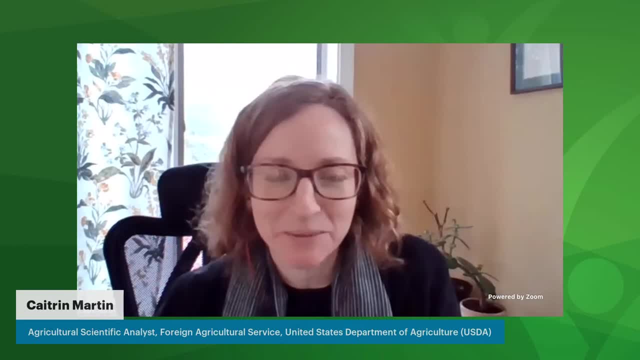 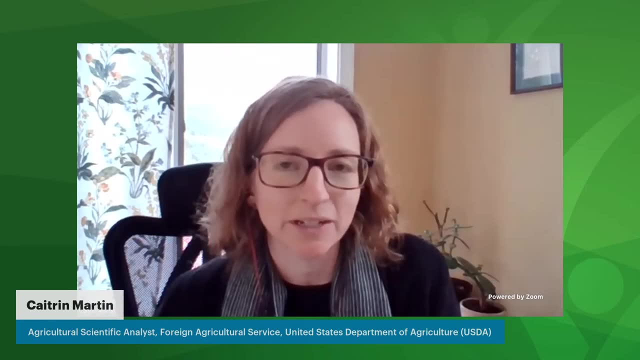 to say thanks a lot to Martian for mentioning the very same thing. we're saying often is that there's no silver bullet, And we're in the unfortunate position of a lot of times just kind of getting into these entrenched debates about how we label different production systems. 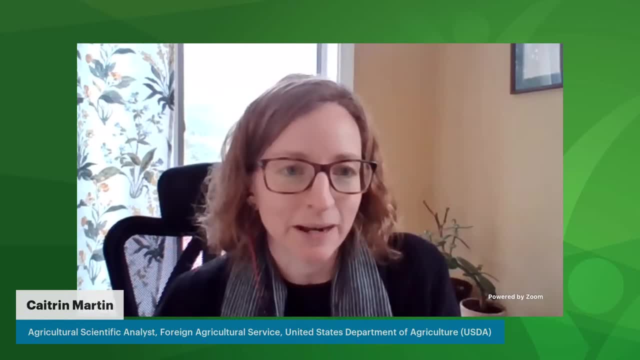 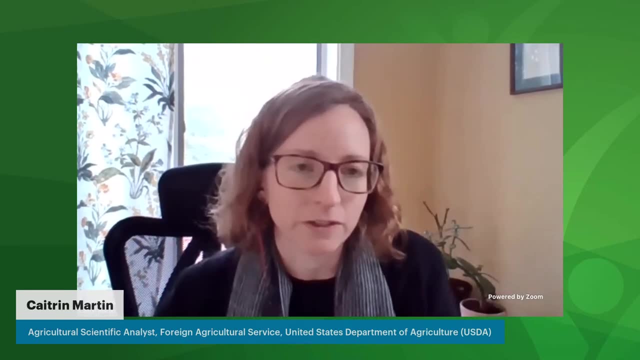 and approaches And I certainly agree with you wholeheartedly there. So yeah, on USDA's multilateral efforts, I'll note we're very engaged in all of the international organizations. UNEA 5.2 is starting next week. 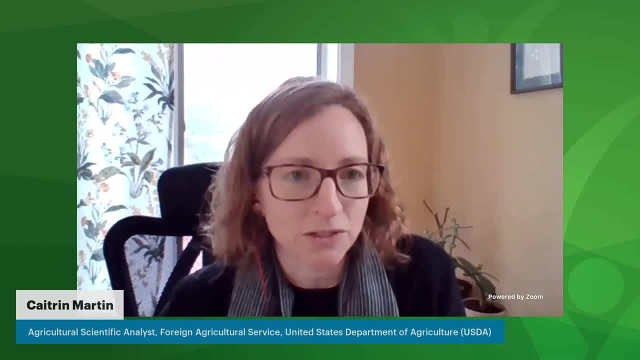 And the US is going to be promoting nature-based solutions and a transition to more circular approaches as opposed to extractive. We're engaged in the Global Soils Partnership, all the initiatives that were mentioned in the communique, The Global Research Alliance on Agricultural Greenhouse Gases. 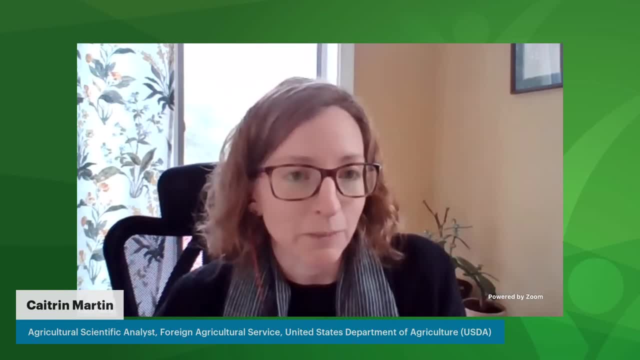 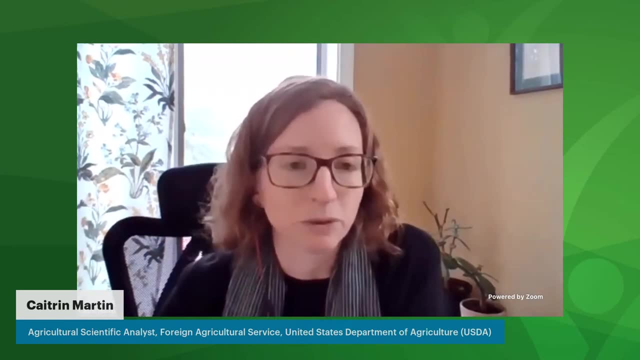 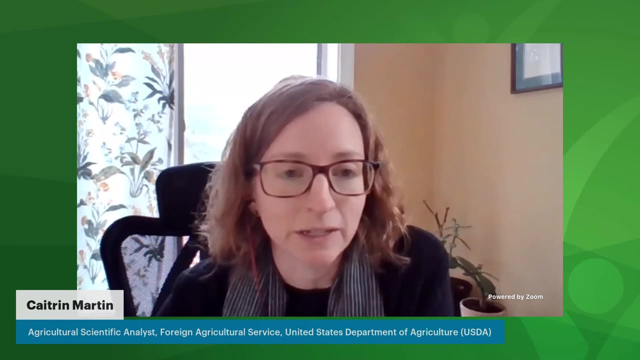 and the UNCCD, And then, in the lead up to COP26, the US launched a number of climate initiatives to advance the overarching objectives of building resilience and leveraging innovation to enhance agricultural and food system sustainability. And I'll mention just a few of those there. 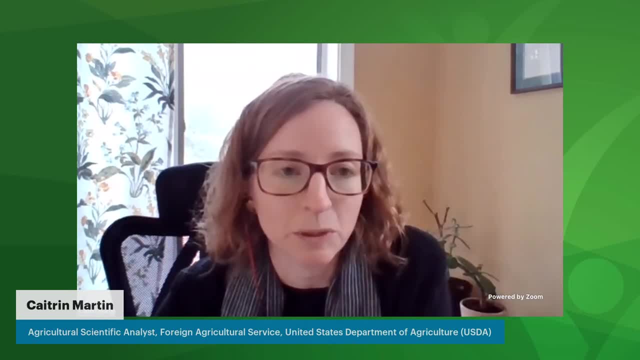 The AIM for Climate- the Agriculture Innovation Mission for Climate. It's a It's a joint initiative of the US and the UAE. Its intent is to catalyze greater investment in climate-smart agriculture and food systems innovation over the next five years. 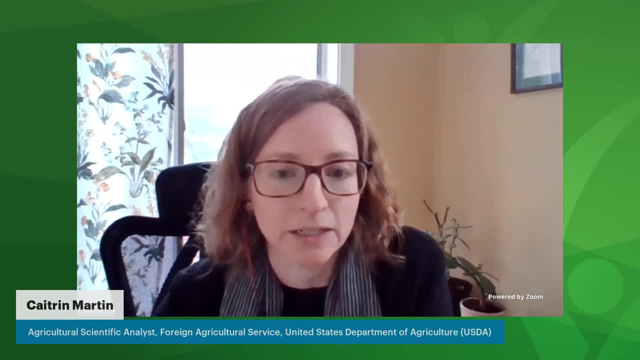 There's about 40 country partners and over 100 non-governmental partners, including CGIAR, And actually the first ministerial meeting is taking place next Monday in Dubai. And then the US was very active in the UN food system Summit. 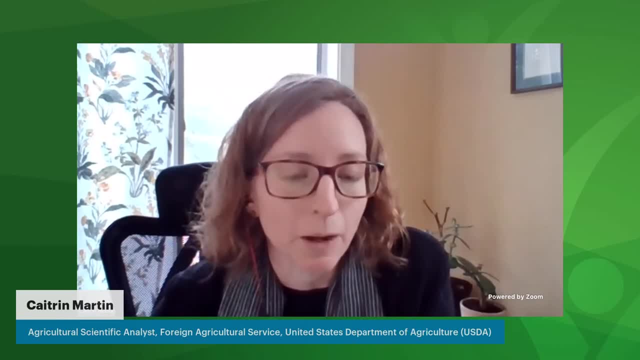 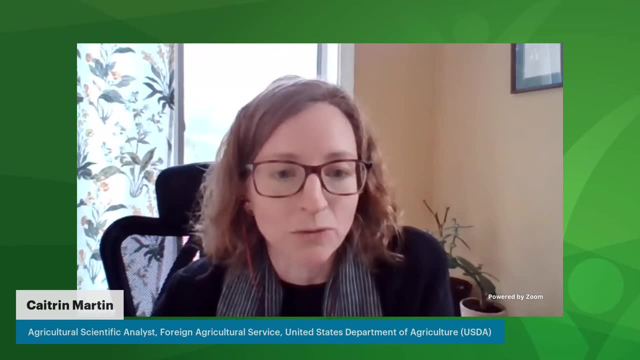 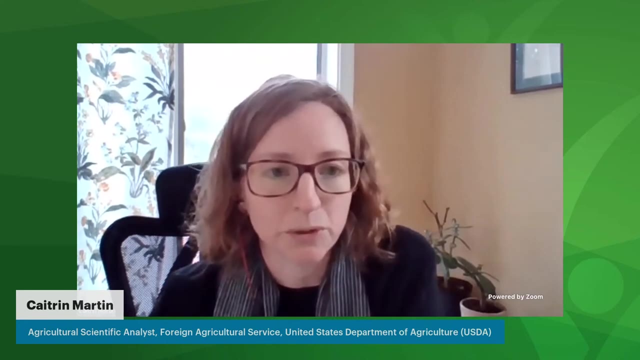 And as an outcome of that we initiated a coalition on sustainable productivity growth for research, conservation and food security, And this is sort of an effort to accelerate the transition to more sustainable food systems through agricultural productivity growth. that hits all the outcomes across all the three dimensions. 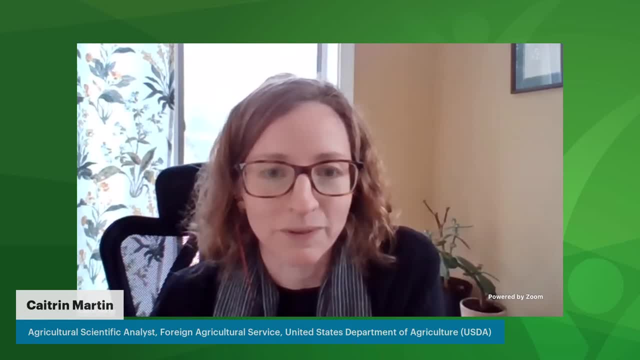 And IFPRI is a member of that. We certainly welcome Jeremy And Malawi to join us in these efforts But, recognizing that there's been a bit of sentiment of initiative fatigue, so we're certainly trying to expand synergies and make the most out. 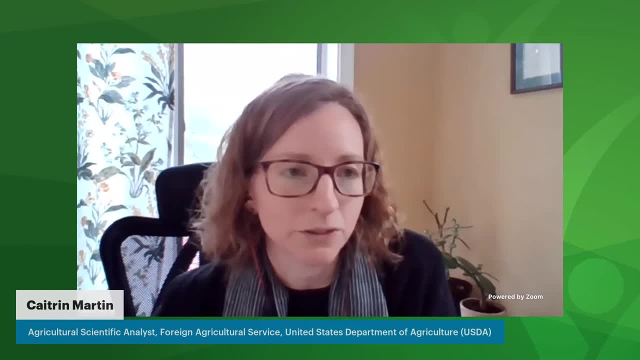 of existing efforts, Because we certainly understand that coordination and collaboration on these efforts can certainly be a full-time job, But it's important. So, yeah, we'll stop there, Thank you. Thank you, Katrin. Thank you for sharing that. 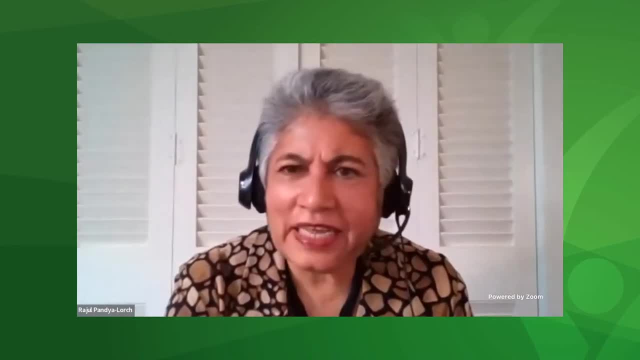 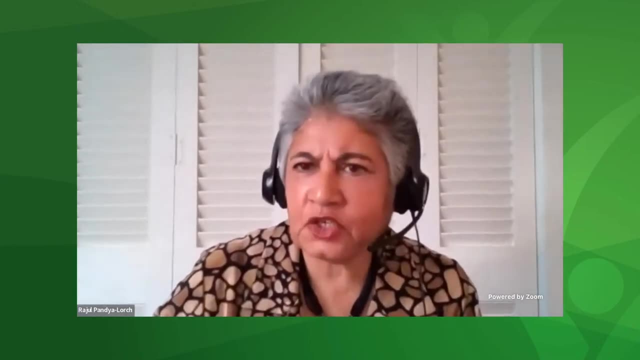 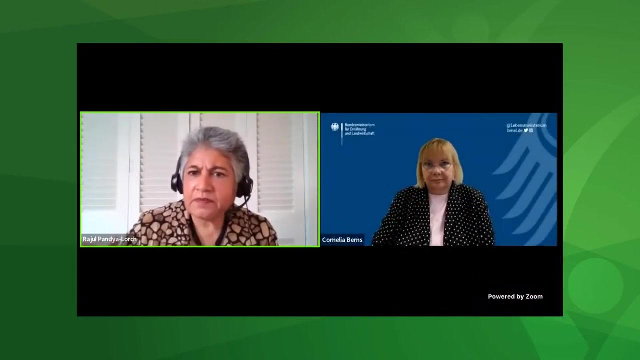 I'd like to move on the similar way. OK, So I'm going to turn it over to you, Cornelia And Cornelia, there are two questions coming in for you. One question is picking up on multilateral international cooperation. How is Germany helping countries to advance the actions that 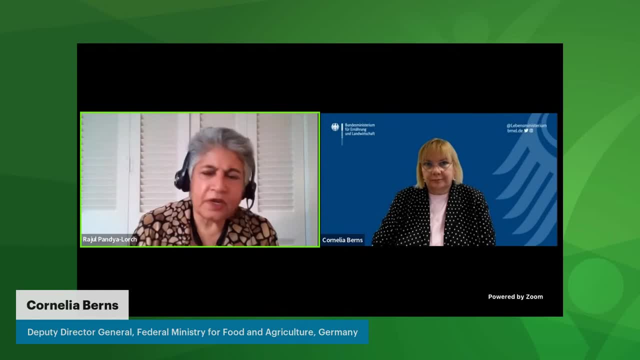 have been suggested in the communique. And then a different question, also on the GFFA, is: what were some of the key contentious issues that emerged during the GFFA that deserve attention in terms of unfinished work, And what are some of the key things? 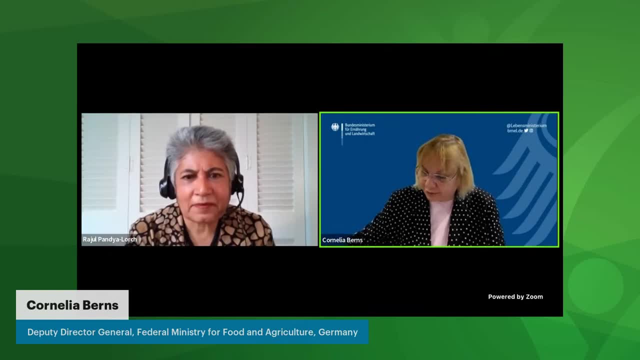 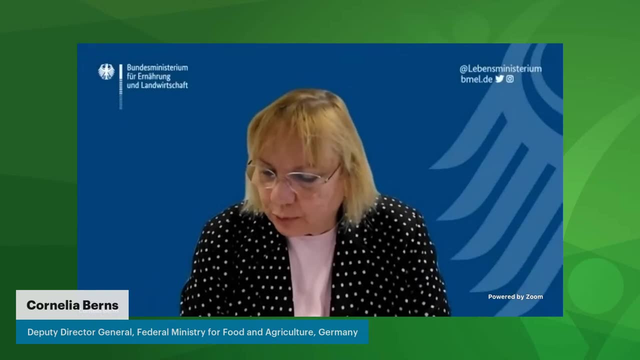 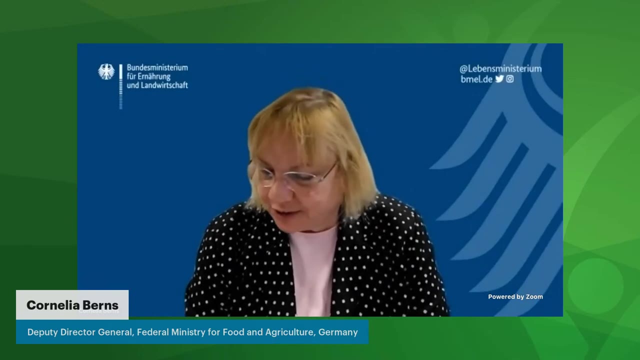 that we should be doing in order to ensure that we are able to continue to be a fully-fledged and fully-fledged business. OK, Thank you very much for your questions. I think I could just add to what the US said that we are part of most of the mentioned international 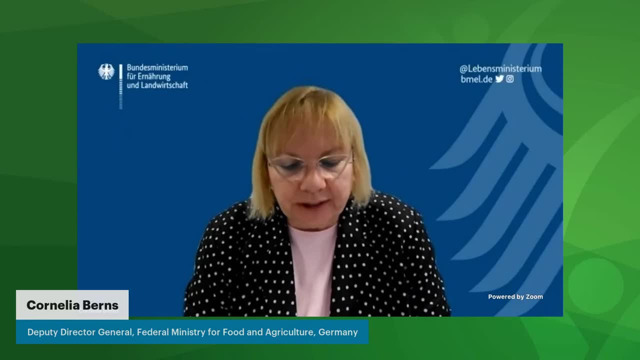 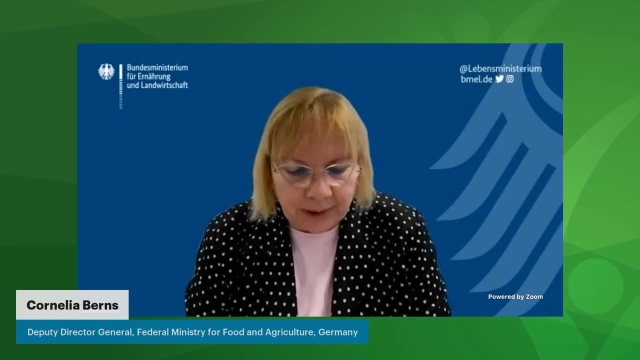 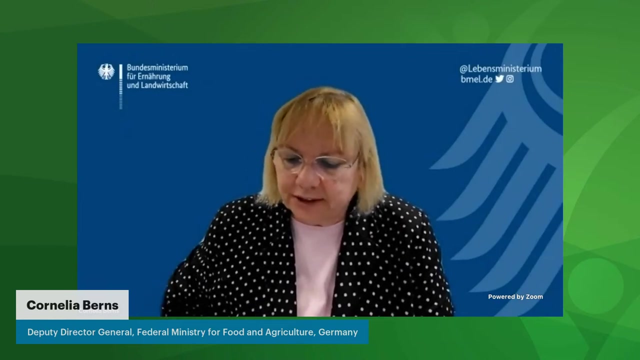 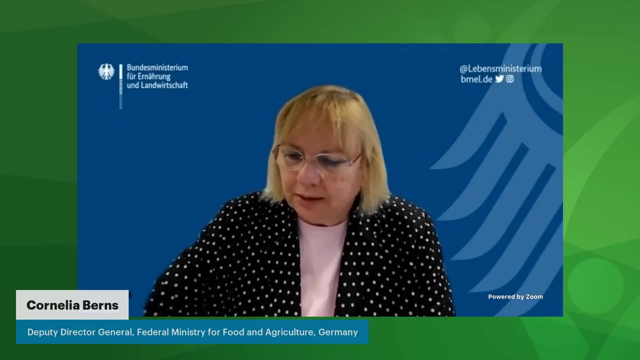 movements and organizations the US already mentioned. I want to mention especially the Committee on Food Security, because part of the GFFA was the discussion of their 10-year anniversary of the- how is it called? the guidance for land, forest and fishery land management. 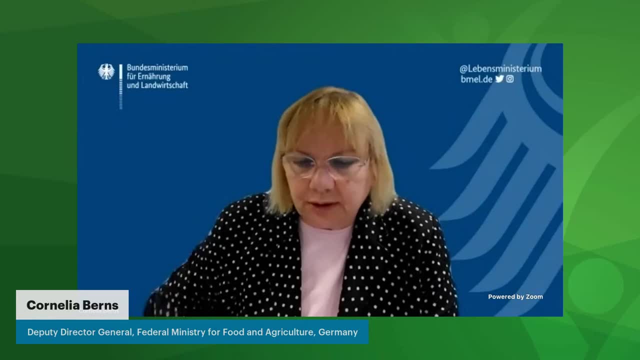 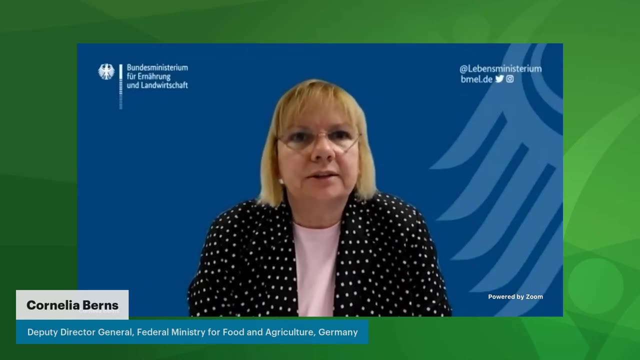 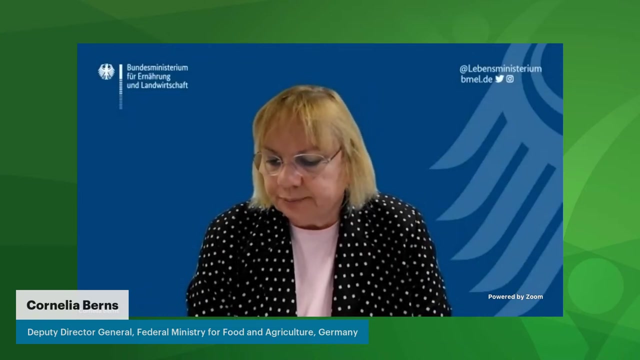 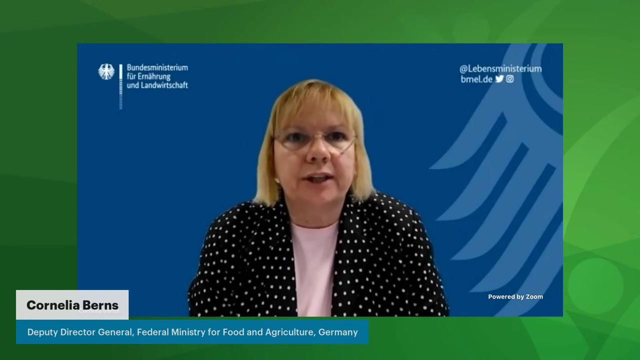 of forest and fishery, And this was developed with in close cooperation also with with Germany, And we are still working very closely with the Committee on Food Security. The last paper they finalized was on agroecology and other innovative approaches. 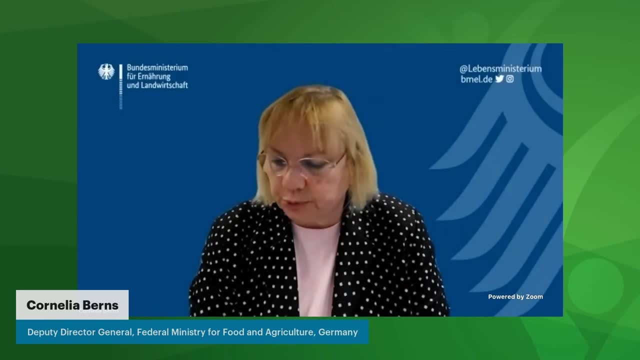 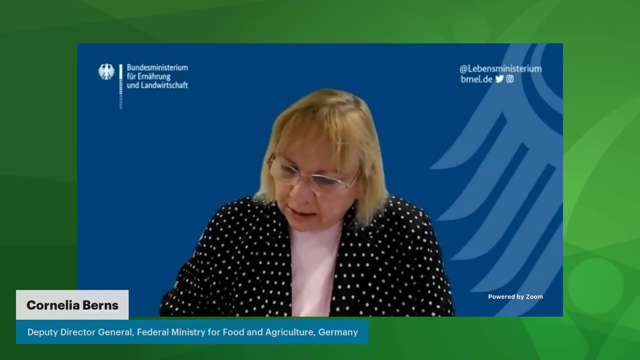 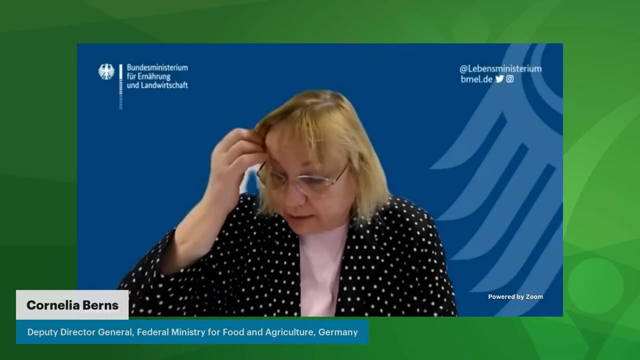 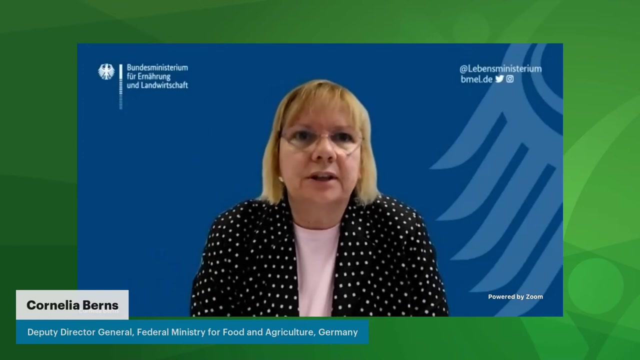 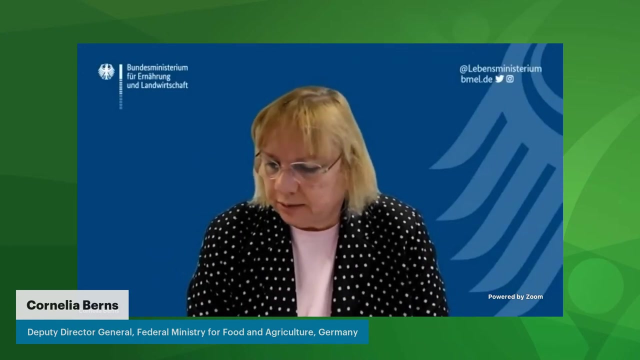 And I feel that we feel that these approaches also contribute to soil health, especially. Then there's the question: Yeah, this is on the multilateral side. I think the other question was: what are the most contentious points in the paper? I think most of the points were really very consensual. 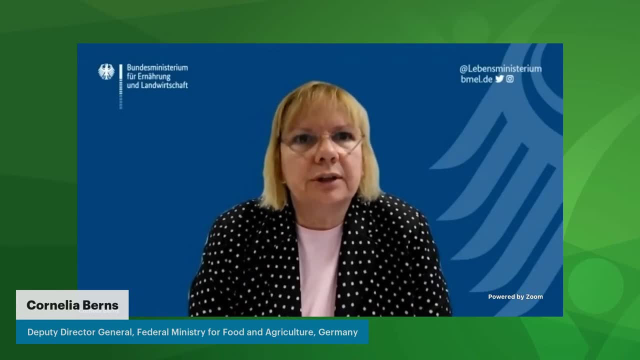 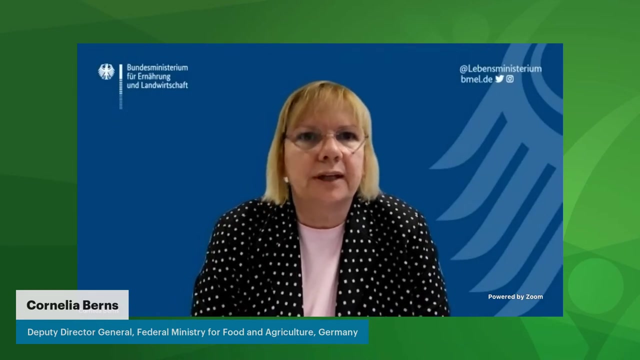 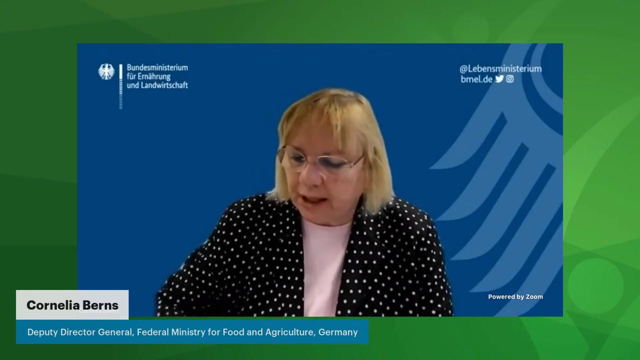 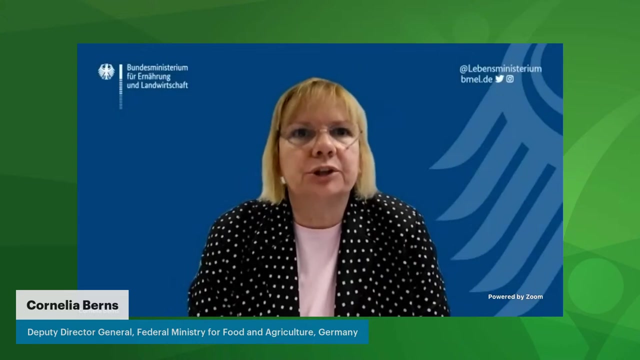 I think issues of land rights are the most difficult for countries Because they have their own, also a lot of legal issues around this point. So I think there it is always difficult to find some global language on that. But the idea which is behind the CFS guidance on land 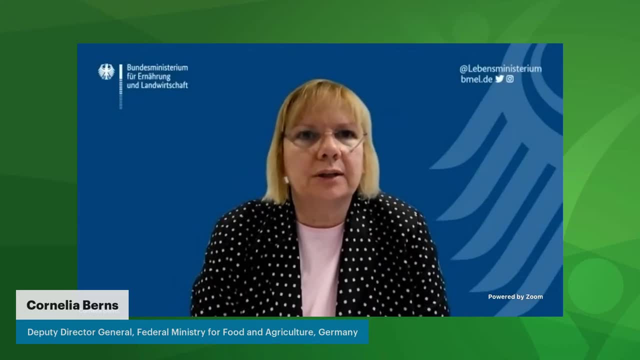 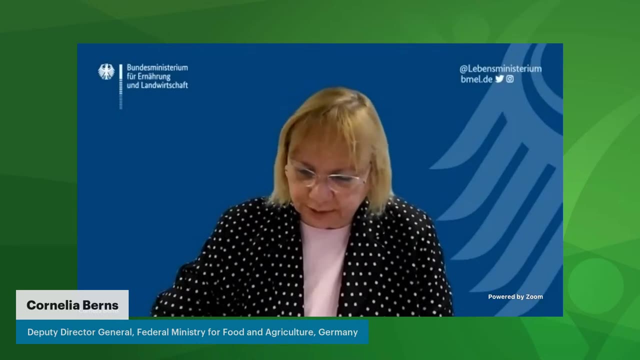 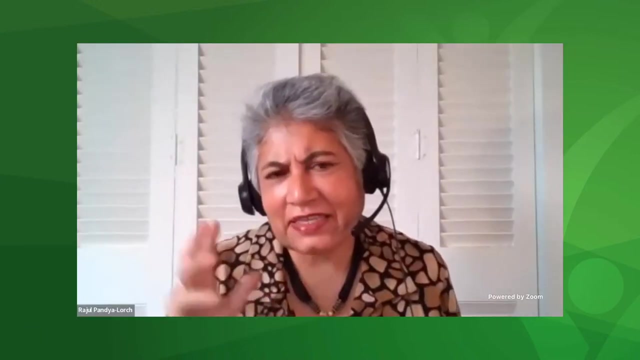 was shared by anyone, By everyone, Yeah, So it is not really contentious, if you mean so, Thank you. Thank you, Cornelia. Thank you for sharing with us, giving us a flavor of some of the discussions. My next question is for Teddy. 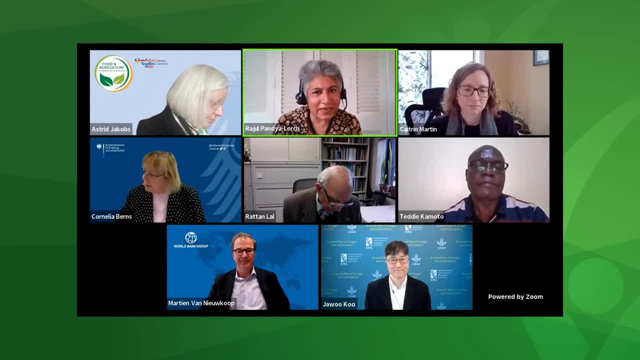 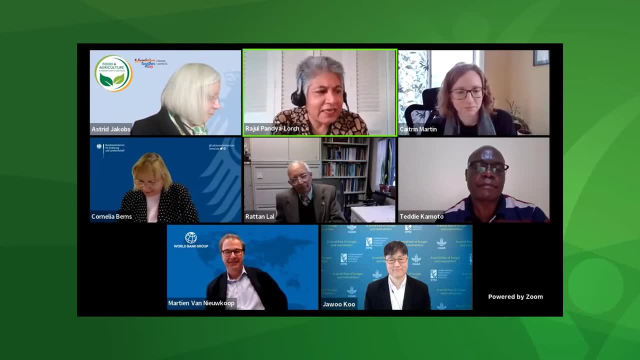 And then a heads up to Martin that he has a question for Professor Lal. So, Professor Lal, in a few moments we'll come to you with Martin's question, But before that a question for you, Teddy. Teddy, you talked at the end of your remarks. 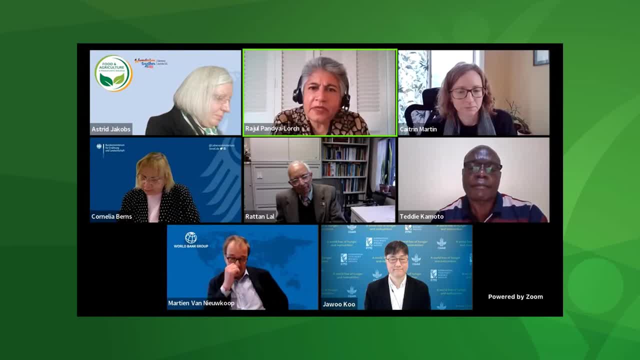 about forests, the importance of forests. Can you comment more specifically on how holding deforestation will contribute to healthy soils and to sustainable land use? And if you want to also say a few words on water management, that would also be welcome. Over to you, Teddy. 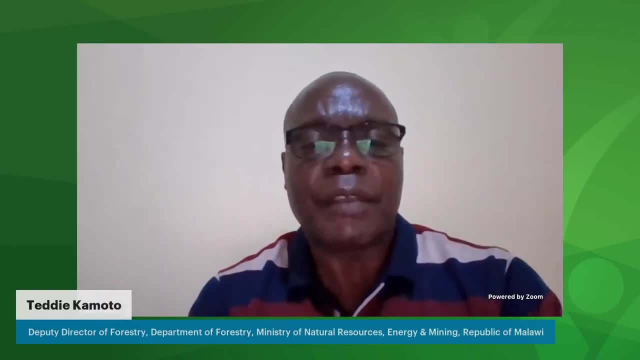 Thank you so very much. Indeed, Maybe let me start by saying that in Malawi, as a country, we already have to get rid of deforestation. we, our forest landscape restoration movement, is driven by what we call three special purpose vehicles, and this is uh uh. the first one is to do with the bond challenge where we have committed. 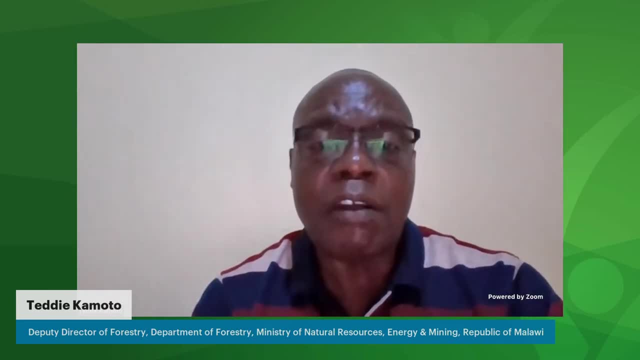 to restore over 4.5 million hectares of land by 2030. the second one is the ending deforestation by 2030. this was an outcome of the cop26. i think we've signed to that declaration and again within our policy, we've indicated that our forest policy, we've indicated that we want to achieve. 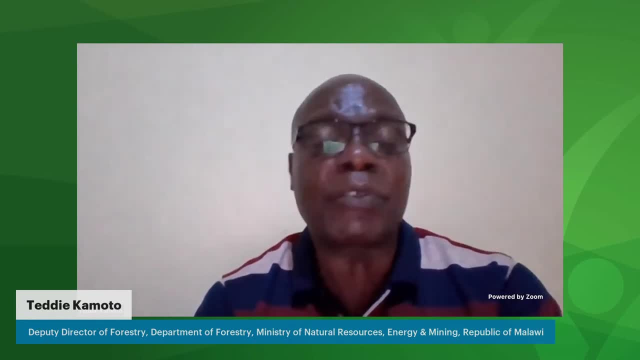 a two percent increase in forest cover, uh, by 2025.. but again, when you look at, uh, the, the ldn and the unc city, what we've declared in there is that we want to make sure that by 20 there is no, no net loss on land anymore. so these are key milestones that we've set. 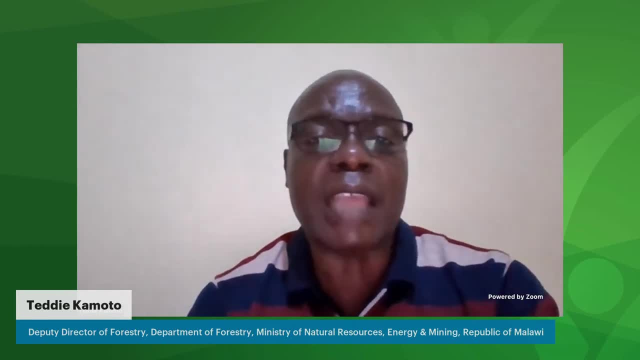 and and therefore, uh, all our efforts, uh, geared towards making sure that we, we achieve, we achieve this, and for us to, to, to, to do this. basically, we, we've, we're using a number of strategies. the first one is to make sure that we, we have on board all the communities, because 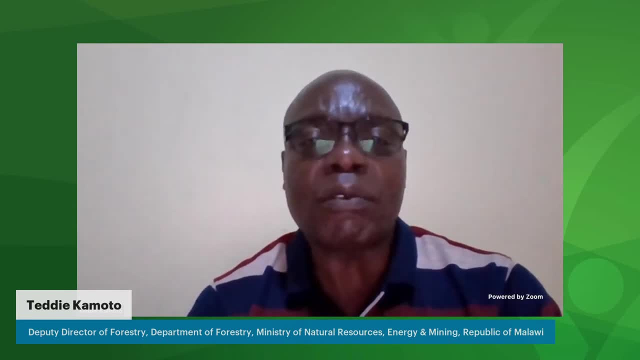 the second one is to make sure that we we have on board all the communities, because when you talk of land degradation, it normally happens in the communities, because that's where farming activities are happening. so if you have poor land use systems there, if you don't have 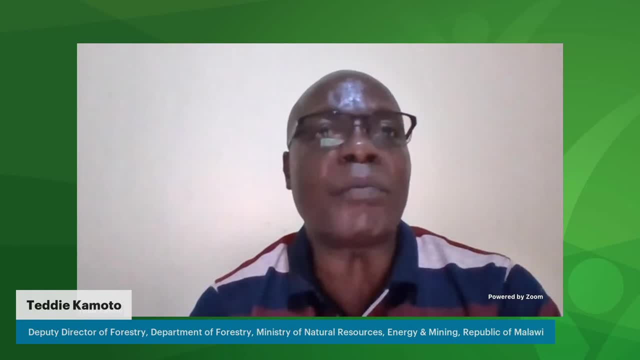 sustainable land use management plans. there you're likely going to have more lands, more land being degraded. the second one is we want to make sure that we bring in the element of the private sector, because we know that if we are to improve land, then there has to be a real land degradation. 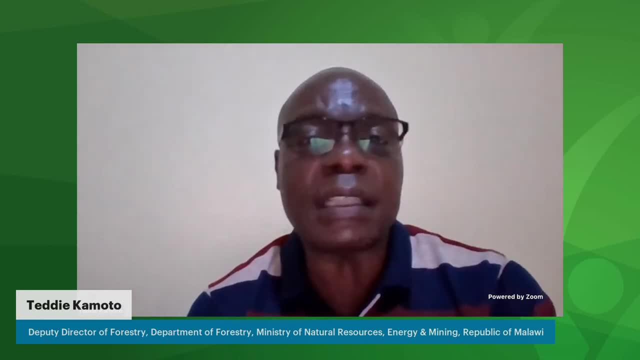 there is a reasonable amount of investment and it's usually the the private sector that can bring that investment. so we're trying to make sure that we bring the private sector and recently we had um a forum, uh, with the ceos of private sectors in the country. just. 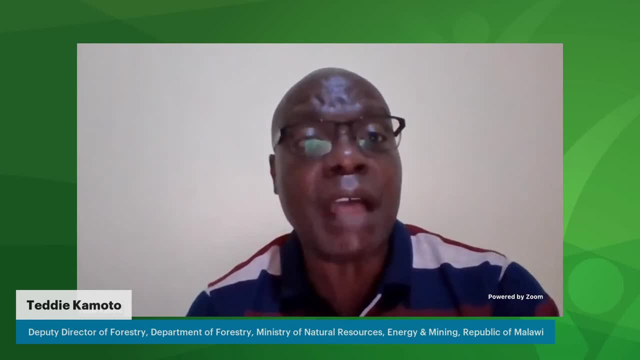 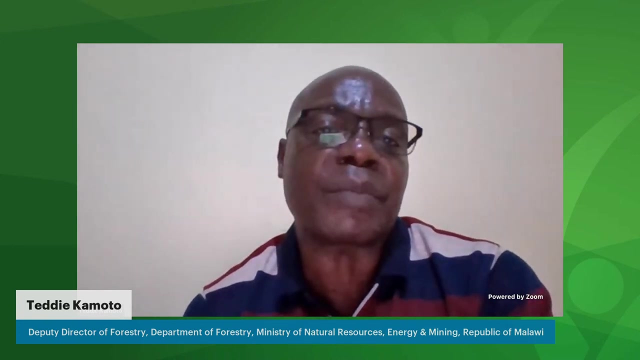 trying to to introduce to them in terms of how, how bad the degradation is in the country and the opportunities that exist for them to come in to invest, either as a business model- uh, through concessions, or or probably as a corporate social responsibility- uh, through mous and other forms of agreement. and that was successful. and the next meeting that we 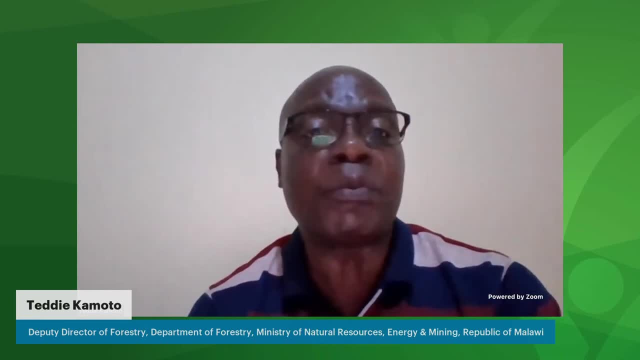 want to hold now is to do with the traditional leaders. we want to bring them on board so that again we make them understand that land. we won't have one land in this country and it will not have any other land from anywhere. so if we can't invest, if you can't protect, 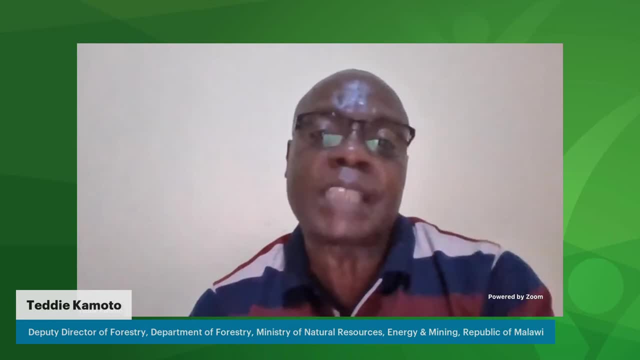 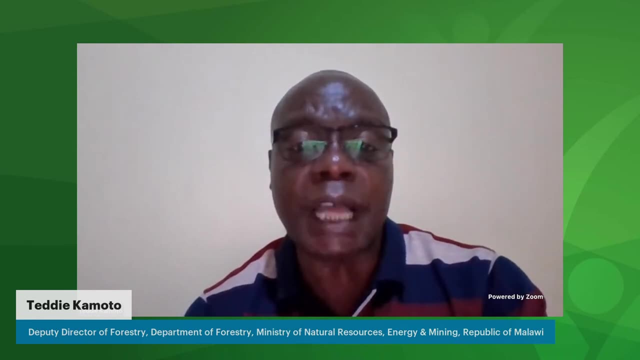 it, then it, it won't, it won't. we want to increase productivity, so these are some of the initiatives that that we are doing in order to make sure that um land is is rehabilitated and our forests are rehabilitated. you know, for us forests are key because, malawi, we only enjoy one rainy. 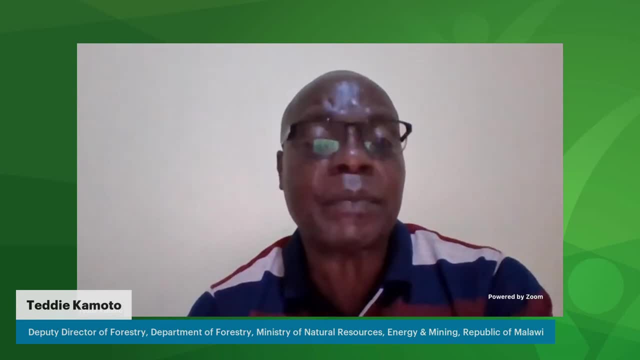 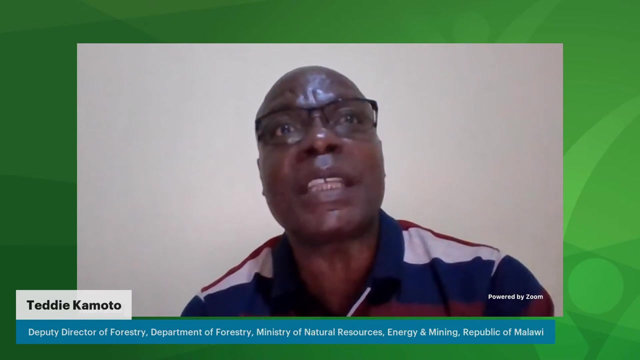 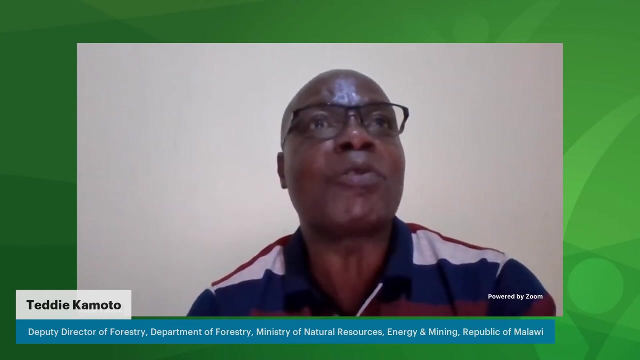 season, um, and basically, such being the case, uh, it means we produce crops, probably during the season, now the extra food that we are able to produce through irrigation. now, if we deplete all the forests- and most of our forests are catchment areas- and if we deplete them, that means we'll have no water, and if, in terms of the water that we use for, 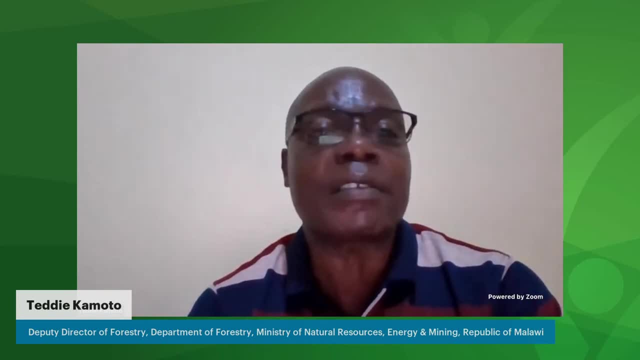 domestic use. basically, it's coming out from this forest. so for us, the relationship between forests, soil and water, uh, it's, it's, it's, it's just too strong. you can't separate them and and and, for us, is the basis for our survival. labor can stop there, thank you. thank you, teddy, very powerful the. you know the. 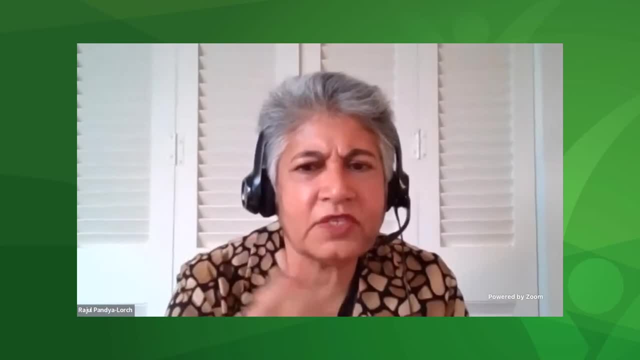 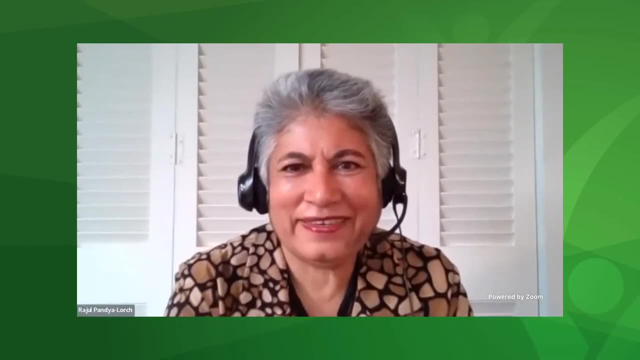 relationship between forest, soil and land is so into and water is so intertwined. thank you for that, martin. you have a question for professor louse over to you. yes, very good, uh, thank you very much. uh, yes, my question, professor lull, is: you know, and i'm very intrigued by what you said. 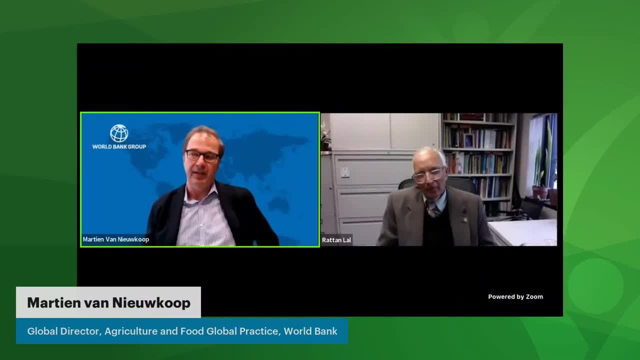 i mean that farmers, I mean, should be compensated. I mean for providing the service of sequestering uh, carbon, um, and, you know, given that soil carbon sequestration, you know, is a public good, I mean that clearly is a sound economic case and rationale. I mean that farmers should be compensated for that. because if farmers are not compensated for that, they actually will be subsidizing. you know society at large and of course, we know that most more, most farmers are smallholder farmers, poor farmers, Etc. so it's not, it's not just right. I mean that this would be the case. I mean that poor, small farmers. 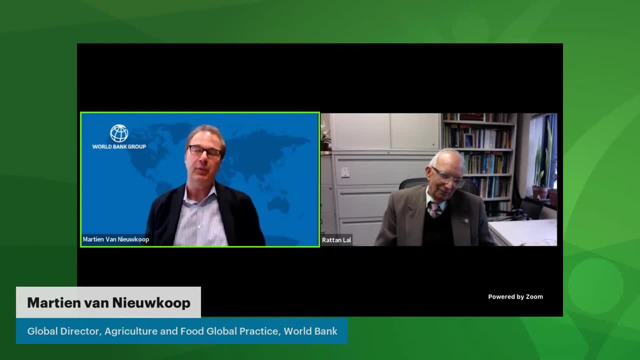 will be subsidizing society at large. the question then is, Professor law, what is the right price and the right compensation? you know, I would also agree with you that current market prices for carbon, which are you know what is it ten dollars or even less, I mean do not reflect, I mean the uh. 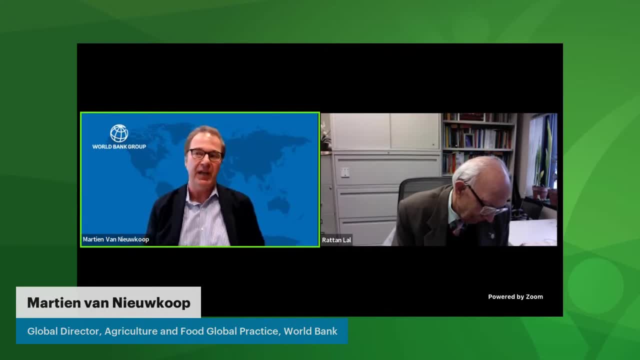 economic value at the World Bank. you know, uh, we use a shadow price of carbon in our economic cost benefit analysis of projects of forty dollars a ton. the IMF has done calculations and they come up with a figure of 75 dollars per ton as the opportunity cost of carbon. now I'm very intrigued. 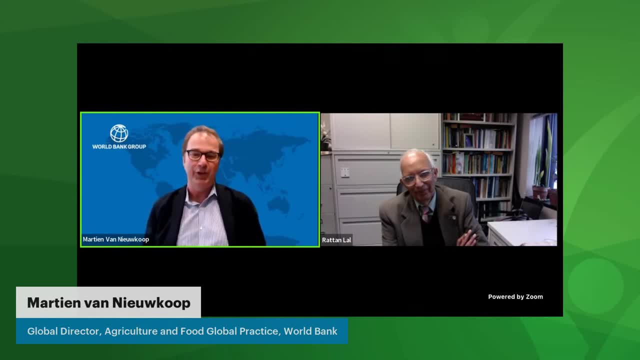 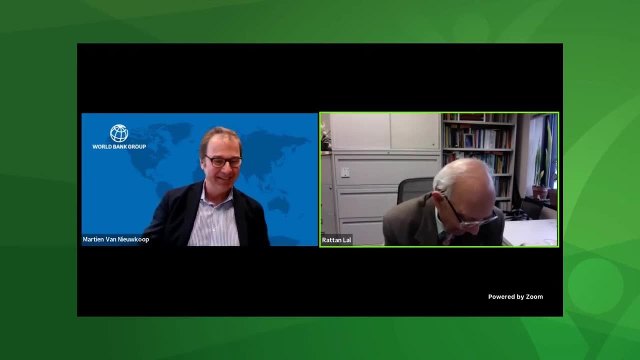 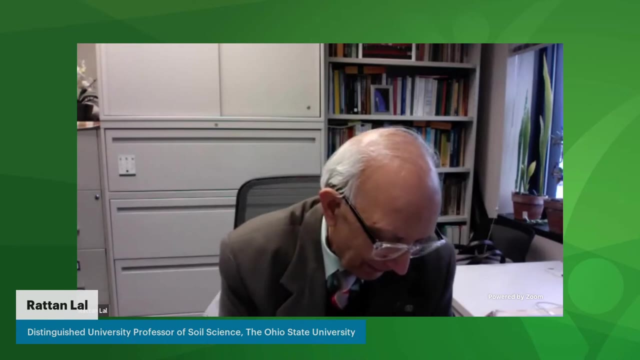 because you said the number is should be about 110 or 130 dollars per ton. so I'm wondering how you arrive at that number. yeah, thank you very much. um, very good question. I'll try to answer in two, three minutes. and especially, you mentioned small holder and Malawi colleague Teddy kamato also mentioned 0.5 acre and serious problem for. 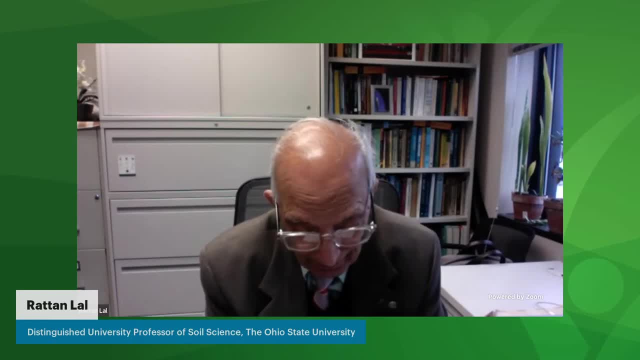 degradation and drought. in fact, the latest estimated there are 570 million small land holders throughout the world that cultivate less than two hectares. they feed three billion people and 60 to 70 percent of those 570 million of women. so this is something we can't ignore. 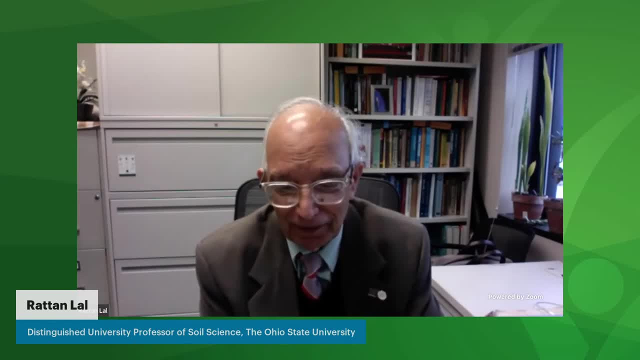 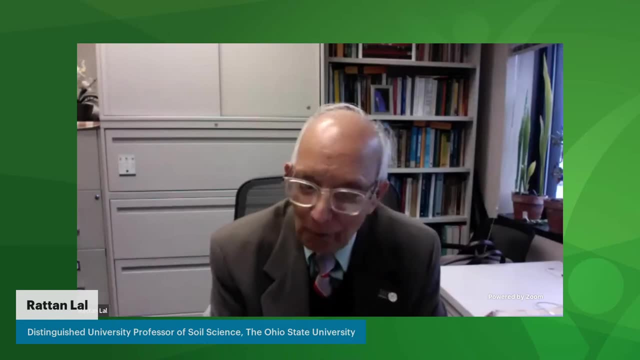 uh, World Bank, USDA, other development organization, GTZ, everybody. this is a very important part that we can't ignore. the question is how much they should be paid. you know, Chicago climate exchange started: uh, one dollar ton of CO2. sometimes there's a confusion: ton of CO2 or ton of carbon. you know? 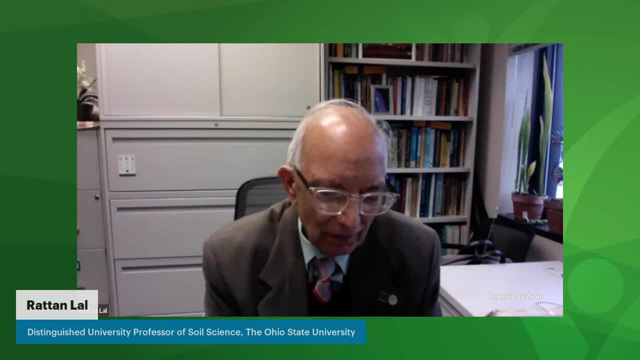 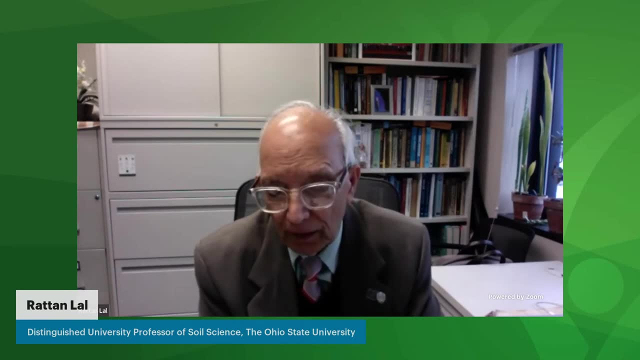 related, but not the same. uh, CO2 is uh 12 or 44, so that's where we compare them. and uh, they went up to six dollars a ton and then collapsed to 20 cents because the US did not have a cap on how much fossil fuel could be burned. uh, then came the geologic sequestration, and even yesterday there 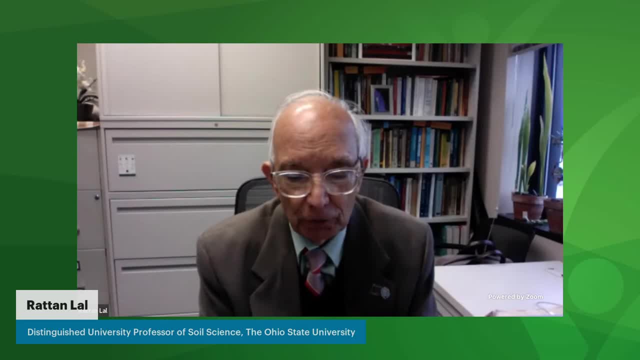 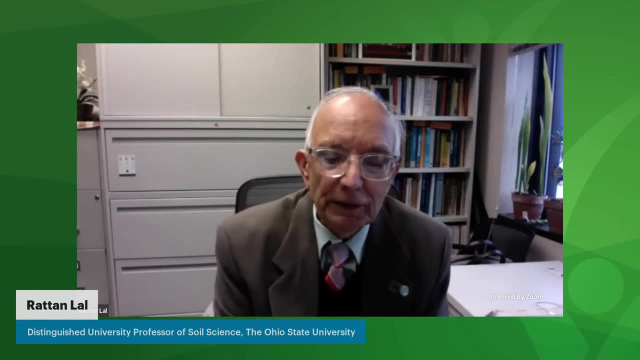 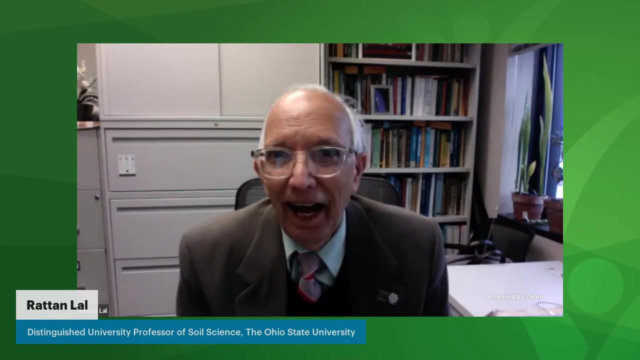 was a statement that those people who take geologic carbon from chimney of a power plant, from ethanol plant, and inject a mile or two mile deep, should be paid 50 ton of CO2. and yet farmers are being paid, as you know, less than ten dollars. I am concerned why that's disparity? fifty dollar. ton when you inject two mile deep and five dollar ton when you are putting 20 centimeter deep. and the five dollar ton has many ecosystem services. so what is it? just and fair price. and that is not demand and supply, because when your government does not put a cap on, 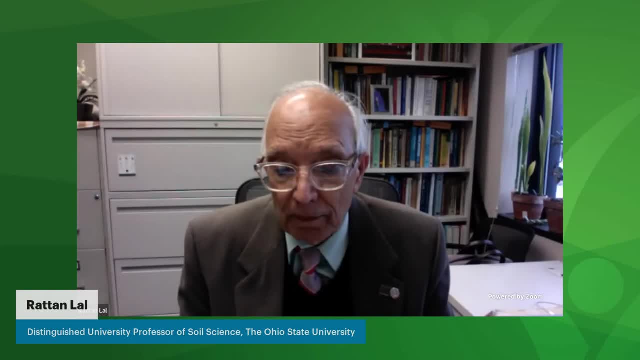 fossil fuel emission emission. you can burn as much as you want. there is no demand because you're burning whatever you like. supply. there are many farmers willing to do it. so, uh, the real price. I published and I'll send you, Martin, a copy, and I'll send it to our host a copy in 2013.. I took the price. 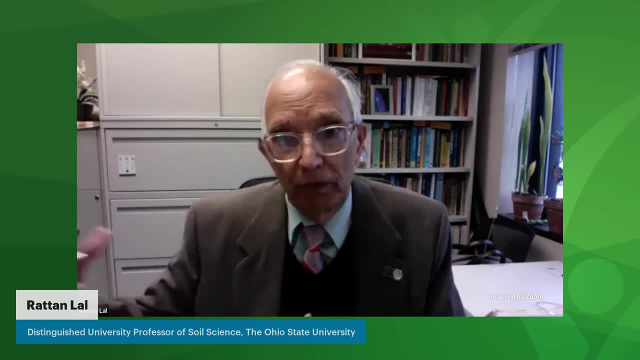 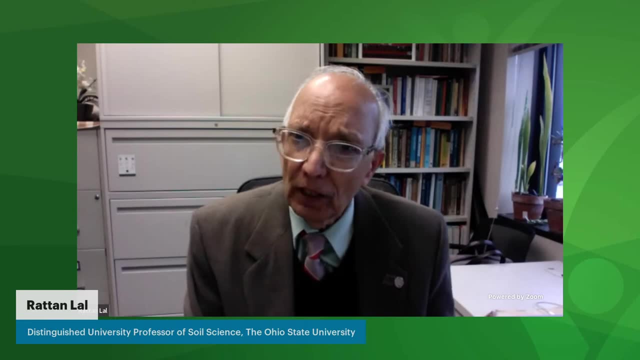 of crop residue. if you want to sell it, what would they get? I took the price of fertilizer because c and p? k ratio in residue is 100 to 1, maybe 500 upon my father in humus is 10 or 50. so farmers are knowingly or unknowingly putting nitrogen and phosphorus into the humus and the other factors and the 2013 price, I came to 123 dollar ton of C. that comes to about $50 per ton of CO2. I think the prices have changed, but I think if we pay Farmer five dollar, we are undervaluing a. 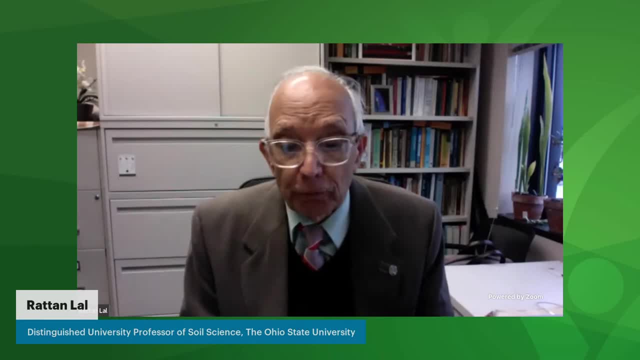 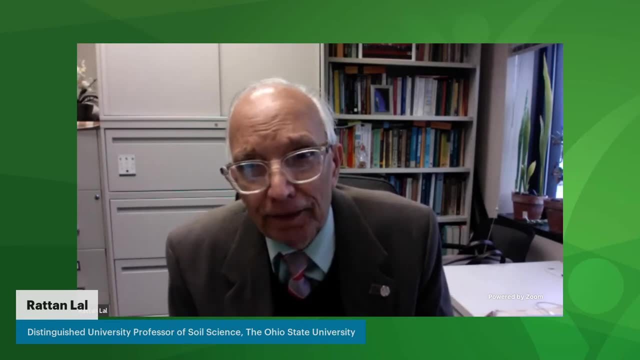 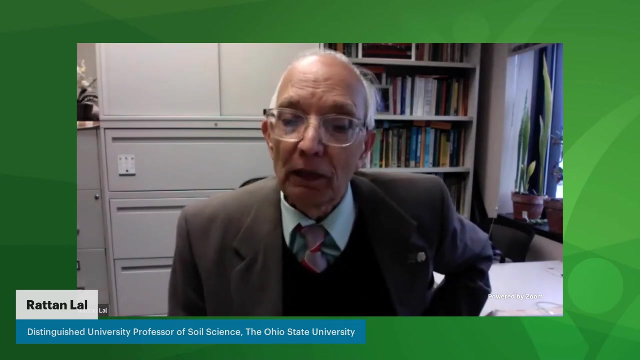 resource and it's going to suffer from the entirety of common. so you give five dollar to a half an acre Farmer and they get a two dollar. what will they do with it? a cup of coffee. if we do not pay them properly, transparently, fairly and justly, we should not be demanding from them. 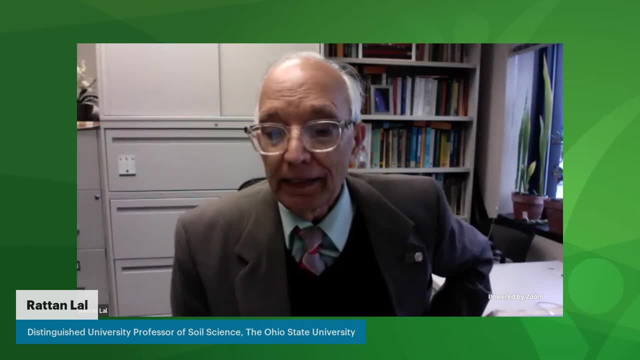 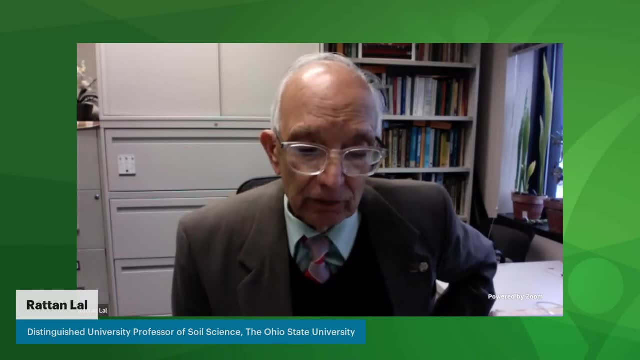 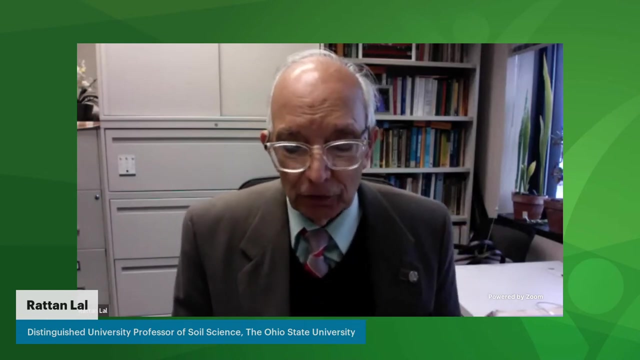 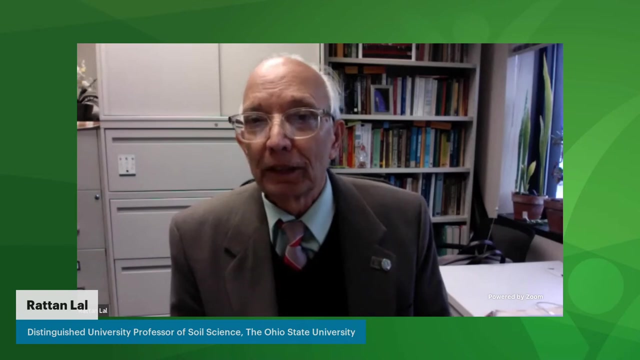 do this and the society has to realize. I was very glad when cop 21 in Paris suggested 100 billion dollar and I immediately suggested to Dr Mr Stephan LaFolle, who was the minister of agriculture at that time. I hope 60 of that goes to Farmer or payment for them to do something good. we cannot. 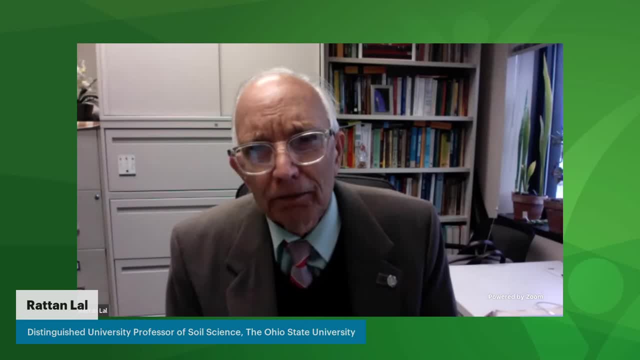 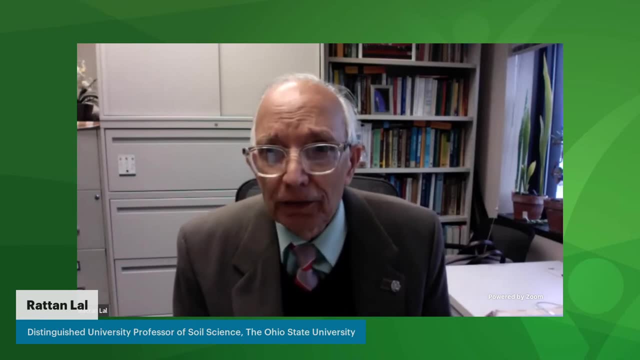 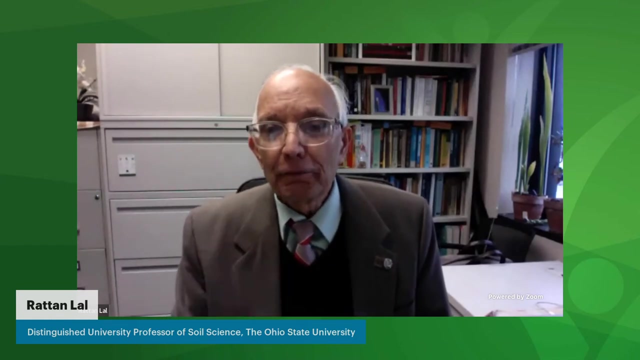 expect them to do it, especially the source per Farmer, but even the bigger one we could not. and when you undervalue is such a precious resource, then the tragedy of the common. we are very fun for me. so World Bank Martin must set the standard high. we will pay the Farmer what they really deserve, what the real, what the societal value of that is. 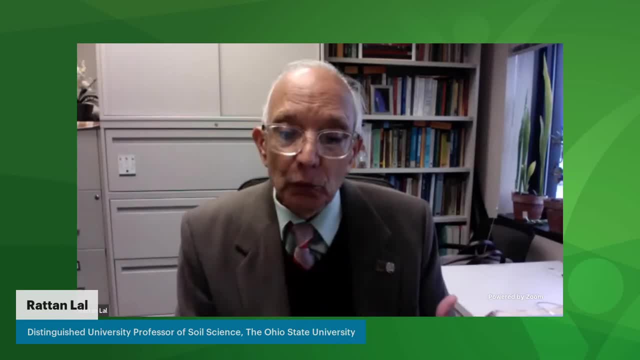 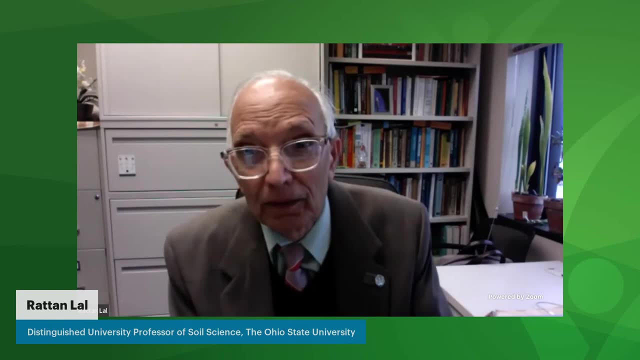 when one ton of carbon goes into the soil, what does it do to climate, to water, to biodiversity, to food, quality, foods, everything, and not demand and supply. and I salute you for asking that question, but not the 121 to ask it in public. that debate is, thank you. thank you, Professor Martin. the challenge is on you to go beyond asking. 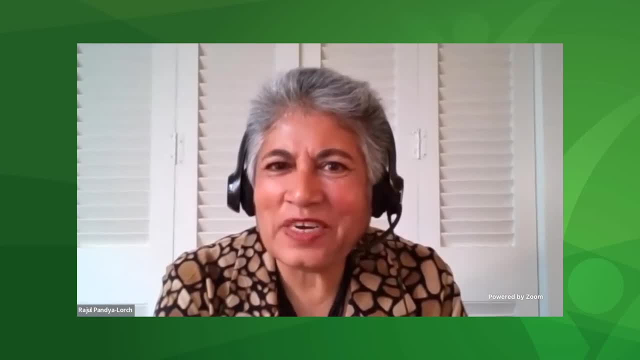 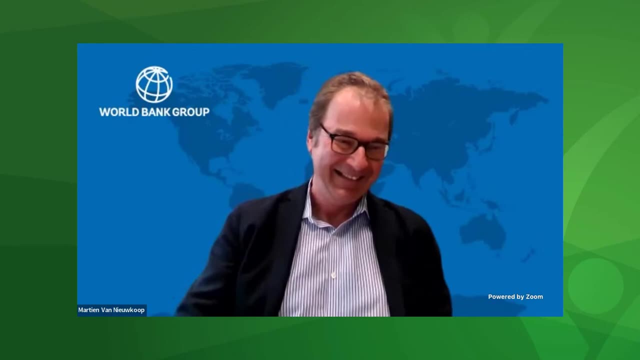 the question I hear. so I think, uh, we will look for further discourse on this. that's exactly what we're working on. but you know, I mean, for that reason I want to make sure we get the price right, so we keep our ears tuned to see something coming out from the World Bank that will help to share. 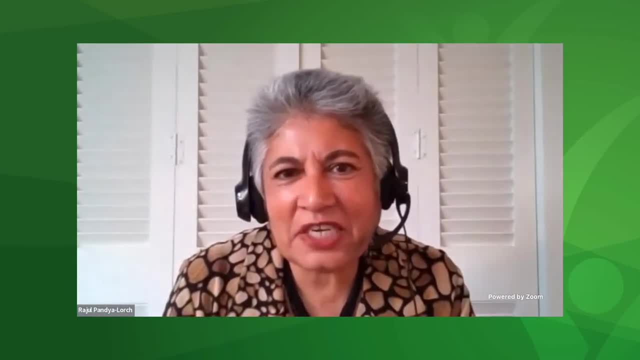 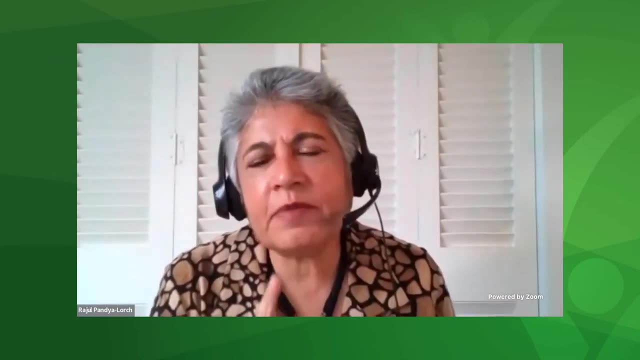 that light on this. colleagues, like we are running close to the end of our Q&A period, I will have two more questions. uh, next question is for you, java and Java. this and then the last question would be for Professor Lal. again, a lot of questions coming in Java. quick question for you is on soil. 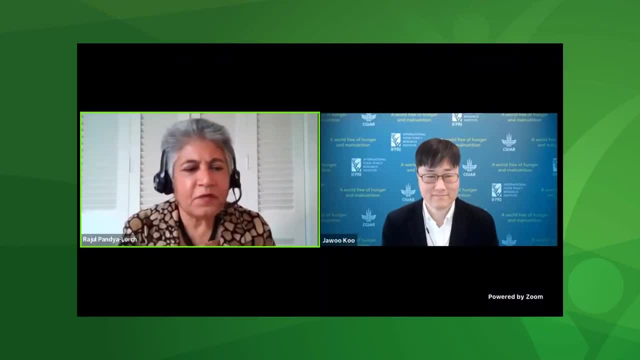 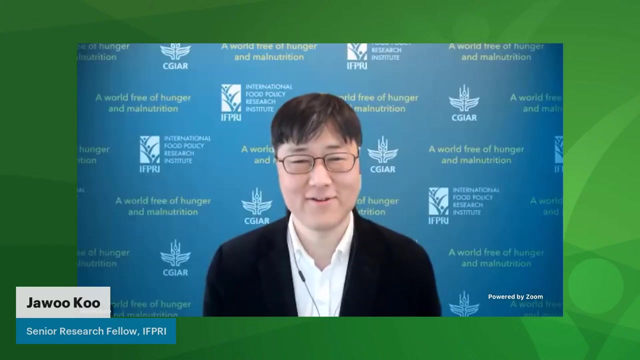 data. so time is of the essence. if we have uh low hanging fruits available, that will help us to advance the soil data issue. where should we invest in the next three years or so? over to you, uh, Joe, okay, great, um. so if, if we are looking at next three years, I would launch a global campaign to 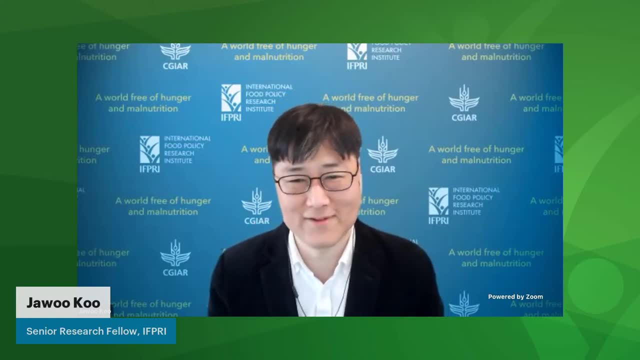 scale the collection of soil sampling data across low input farming system around the world and also collect farmers management practice information in recent years so that we can understand the trend of changes of those soil, carbon and nitrogen and many things with properties over time and this information can really significantly improve the quality and reliability. 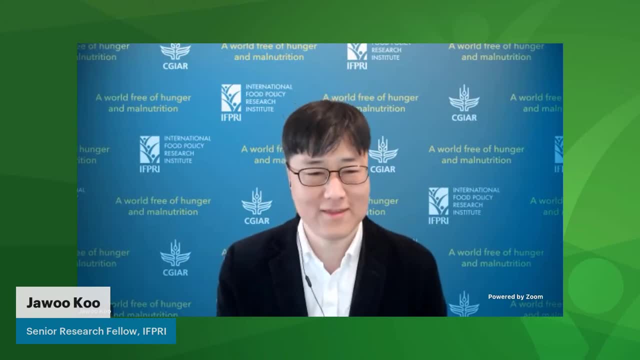 of digital soil mapping processes and the prediction data and I think other sources spare some of the money, some of the research, to improve how we communicate so information to farmers. uh, in the India example I mentioned before, when the full information card, the information design of the information card, was improved and they saw the huge takeoff of how farmers understand the information. 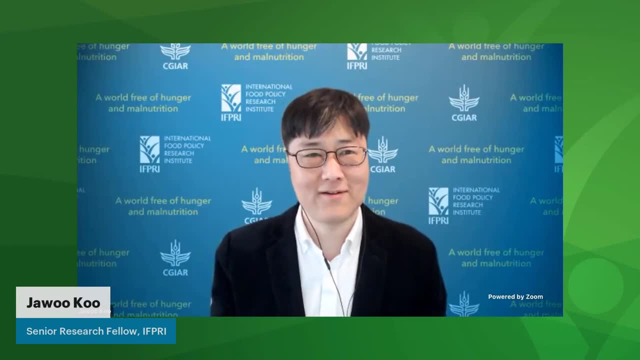 and what to do and how they uh better understand their fertilizer recommendation, where it's coming from and what I should do better. so, yeah, I think that we can really benefit from like human-centered design and better design approaches to deliver this nuanced, very complicated for information and also uncertainties around the 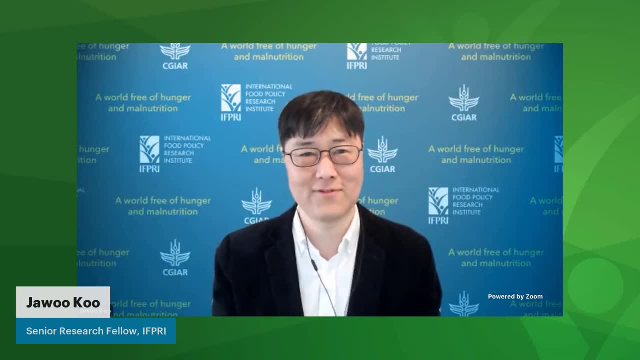 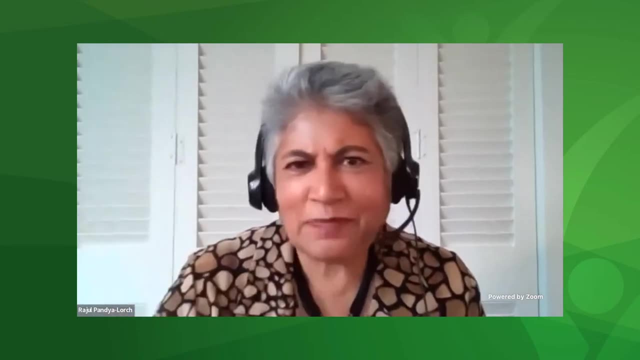 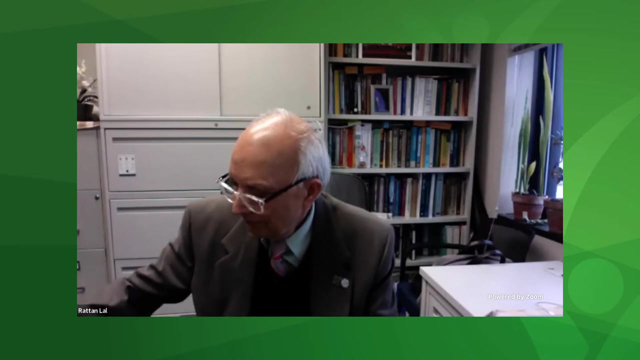 soil data to farmers and who can really use and benefit the most. thank you, Joe. Professor, I'm combining several questions to ask you. you have demonstrated you can respond to multiple questions in a very succinct way, but I'm combining several questions that have come in. uh, question number one. 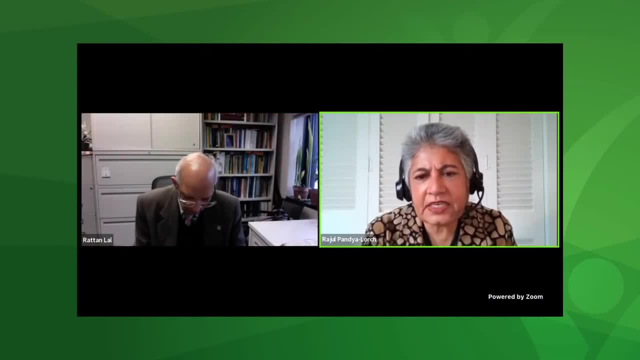 is: what is your view of chemical fertilizers used in Africa, where low input output, uh, low input, low output in cultures- practiced abandon or reduce? and then second question, uh is around organic agriculture: is it possible to feed any nation with a hundred percent organic cultivation, giving consideration to sustainable land use? 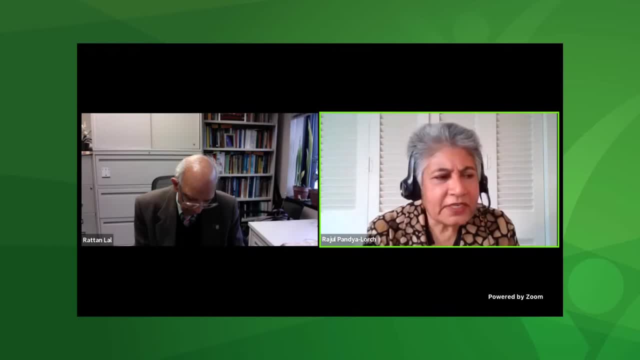 and then the third question is: what are some of the big research and Innovations opportunities open to us, um that we should be considering to accelerate our efforts to achieve healthy soils? where do we, where is the new science for uh research and Innovation opportunities? over to you, Professor. 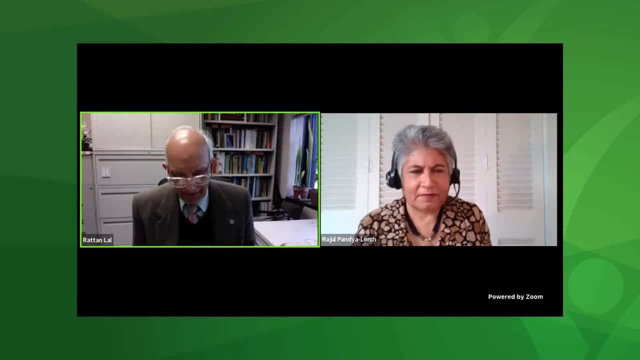 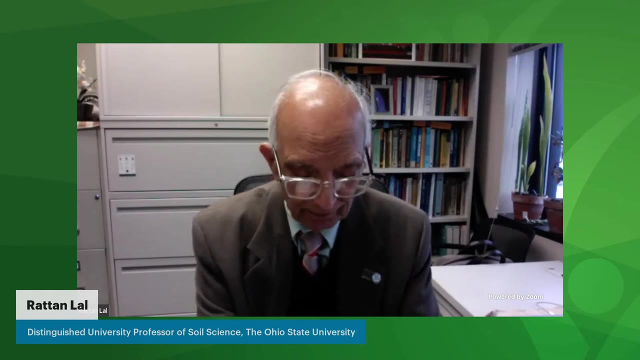 thank you. chemical fertilizer really very um kind of a hard topic. we are using about 200 million tons of fertilizer right now globally. uh, India, China are on the top of the list of fertilizer consumption. I was surprised. Punjab is using 240 kilograms per hectare of fertilizer, United States on the average. 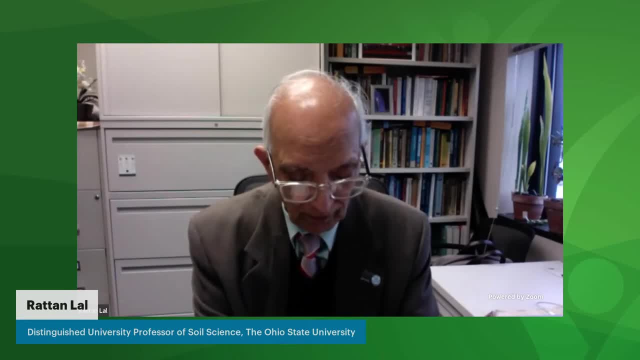 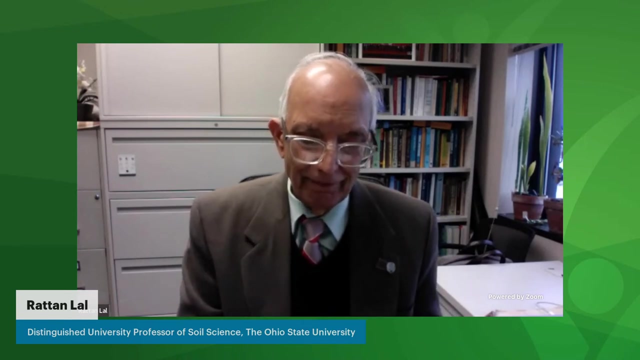 less than 100 kilograms per hectare. so uh, China, someplace is 500 kilograms per hectare. uh, use efficiency fertilizer. uh can be twenty percent, thirty percent, fifty percent would be very, very good uh. so rather than focus on rate of fertilizer, the focus should be on efficiency of fertilizer can. 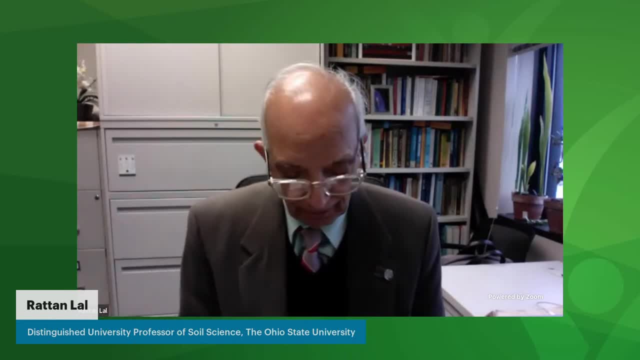 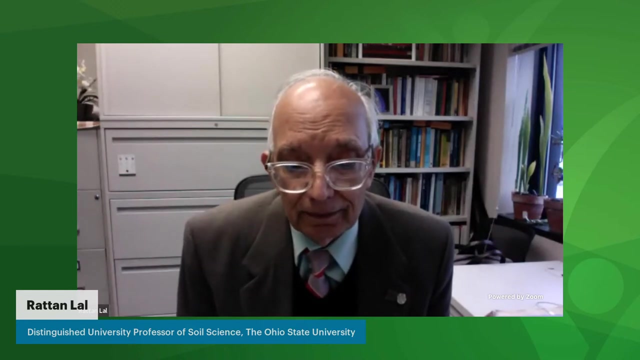 we improve the efficiency from twenty percent to seventy eighty percent and, if so, how soil health becomes very important. the answer whether we can feed the world without fertilizer- nine billion people almost now, 7.9 billion now and coming to uh 10 billion by 2050- the answer is no, we cannot. 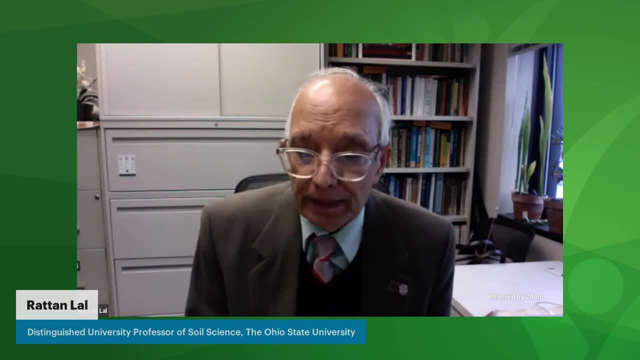 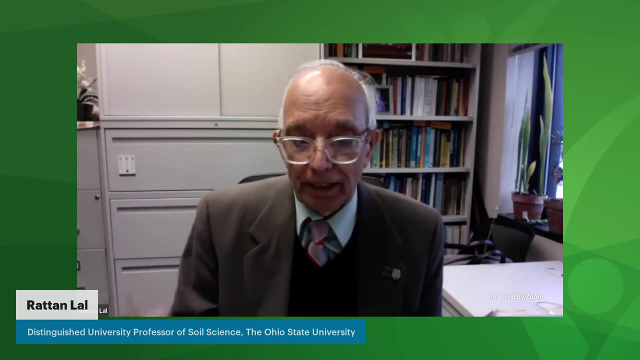 feed, uh. therefore, feeding the world is a priority number one. 820 million people hungry and covered 19 has added another 130 million. 2 billion people suffering from malnutrition. so to say thou shall never use fertilizer? I will not accept that statement. yes, minimize the use, increase the. 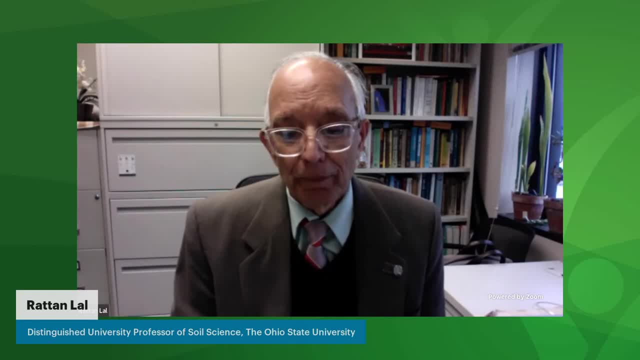 use efficiency, use it judiciously, prudently. please remember the difference between poison and medicine is the dose and the time it is taken, and that's very important. when you use indiscriminately, even the medicine becomes poison. aspirin is a very good example, so using that's where digital agriculture precision. 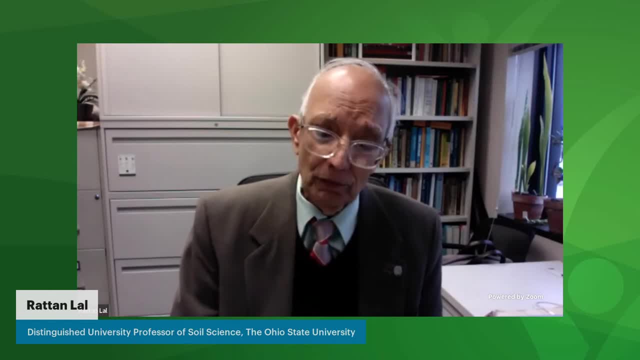 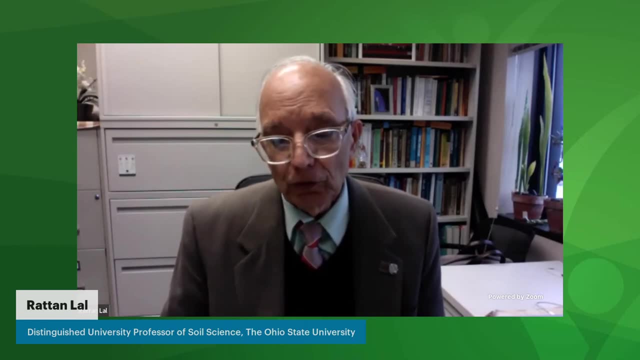 agriculture. soil test values, soil health card are very important. integrated soil fertility management, combination of biological fertilizer, combination of recycling and whatever is needed more. because we cannot get the yield required, we should not hold back chemical. use it judiciously, prudently, sparingly, properly, scientifically can organic agriculture fees. 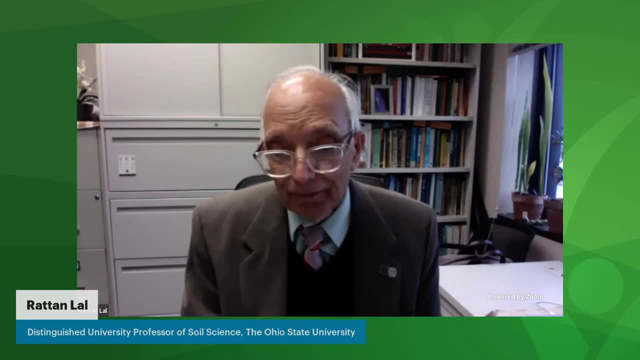 100 percent of people. if our population was 2 billion, 3 billion, I think organic agriculture would be ideal and I think organic agriculture has a niche, uh, where certain things can be grown with organic agriculture. but the way our population trend is now, some people have will have to go. 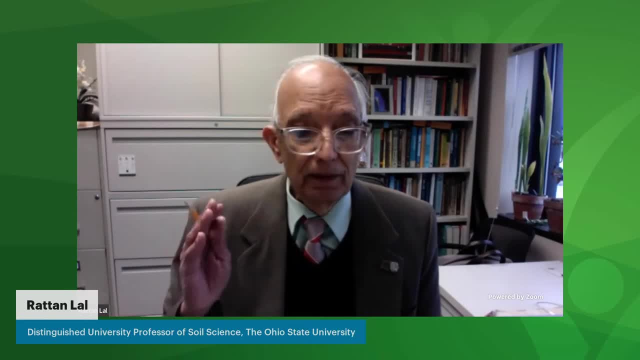 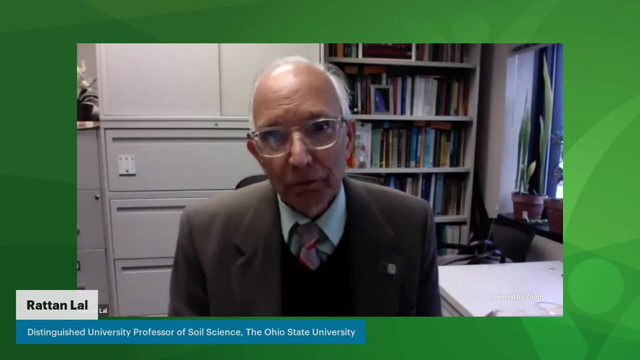 hungry and therefore organic is in terms of soil health, in terms of soil qualities, organic increasing is absolutely essential. there is no question but to go and say that we will not put any chemical at all. I'm worried whether we can feed 10 billion people. so that is the part. let's. 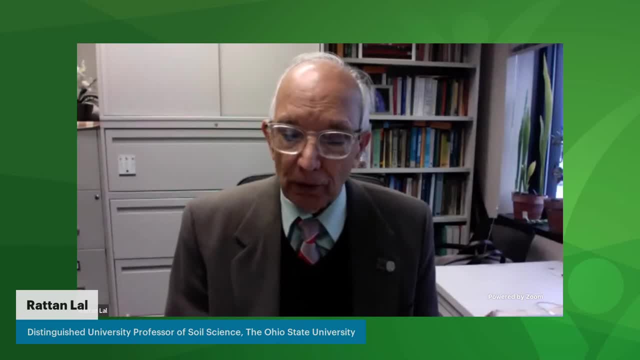 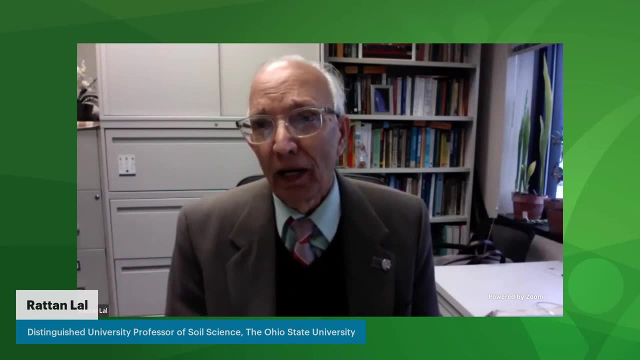 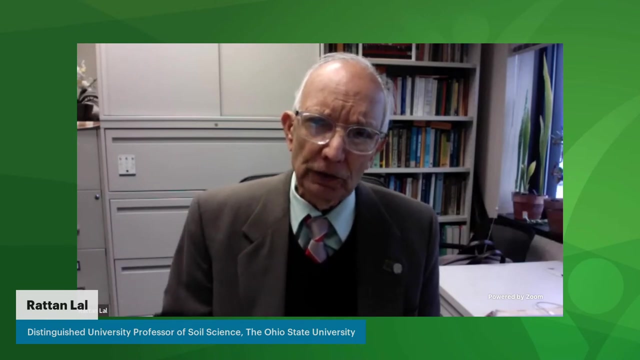 use organic wherever it's feasible and as judicial as possible. some farmer can get extra price for it. yes, let's support it, but let's not make it a divine rule that this is the only option. we have such a humongous problem at the moment of food insecurity, of water quality, of climate change. putting these 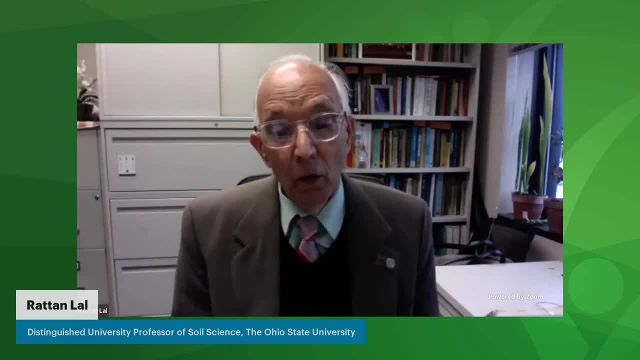 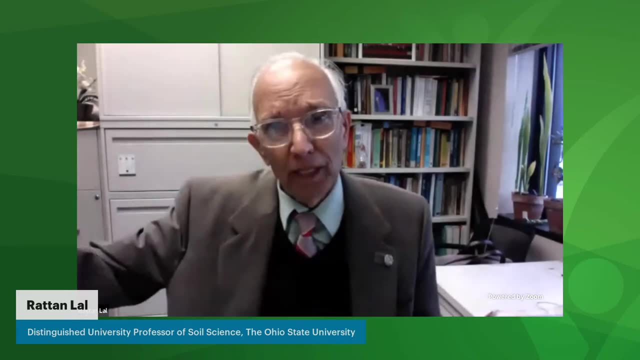 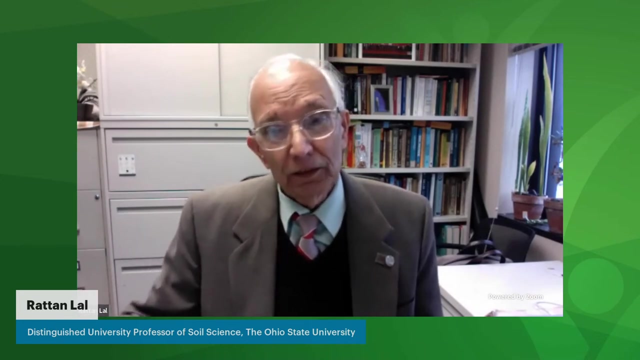 very strict. do's and don'ts may not be, hopefully, with education of the women, especially in developing country. population train may not go to 11 billion. there are data that if the women have a power, they are empowered, they have education, they have their own destiny in their hand. maybe will stabilize at 8. billion. well, there, that's a bright side, but that has to happen. the last part: what are the innovation? please remember, soil is a living thing and a living soil dumping chemicals inappropriately, ad-hocly, flowing, inappropriately flooding. you are dealing with a living entity and just like any other. 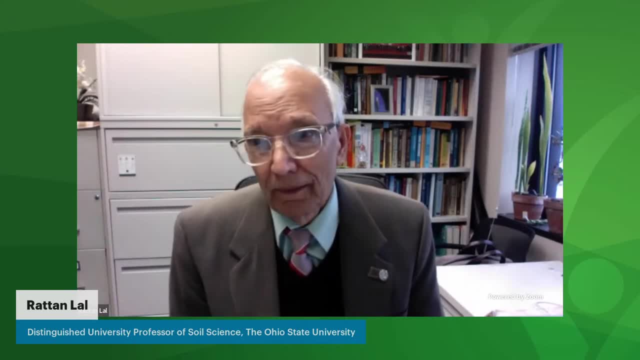 living entity. I think soil must also have rights: rise to be protected, rise to be restored, rise to thrive, rise to manage properly. simply because you own it doesn't mean you can do anything with it as you wish. we have in this country a very good example of a clean air act. we have an example of 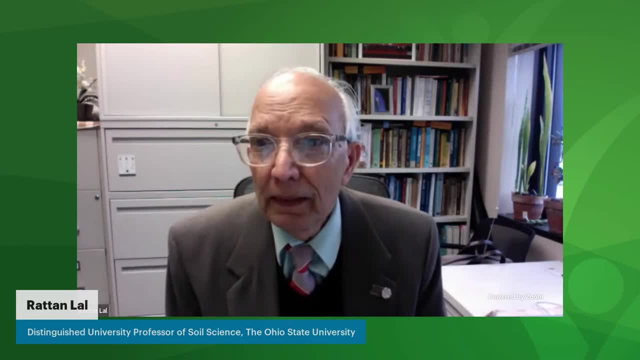 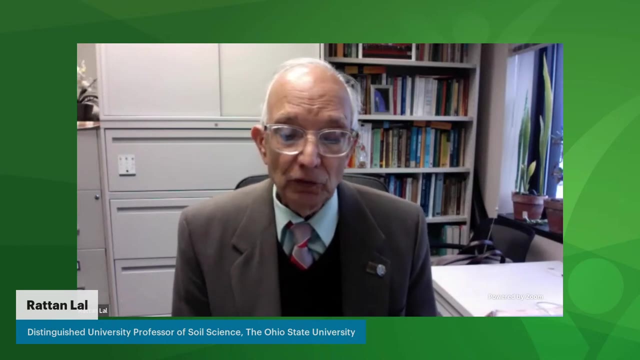 clean water act. there is no healthy soil act. is it ever possible to have clean air and clean water without healthy soil? it's rather being naive, and this is a time where Germany and US and France and other countries set up a model soil health Act. that doesn't mean you are going to punish those who do not do it properly. 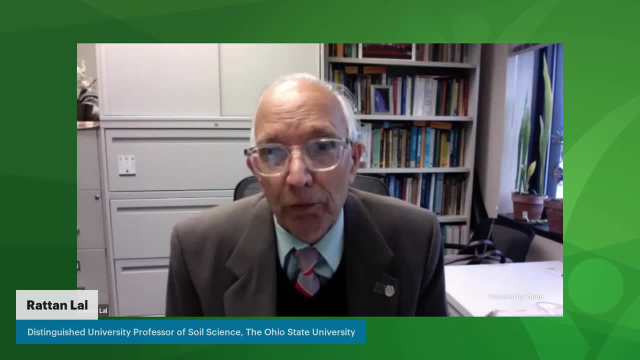 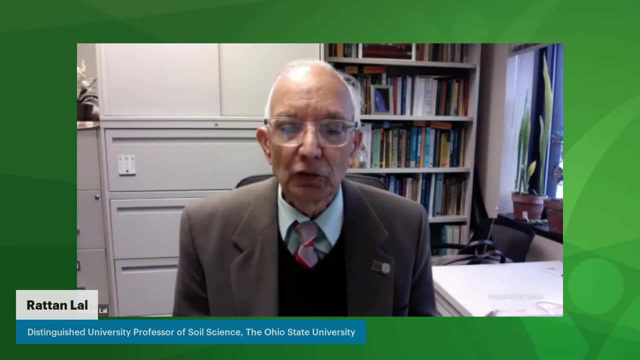 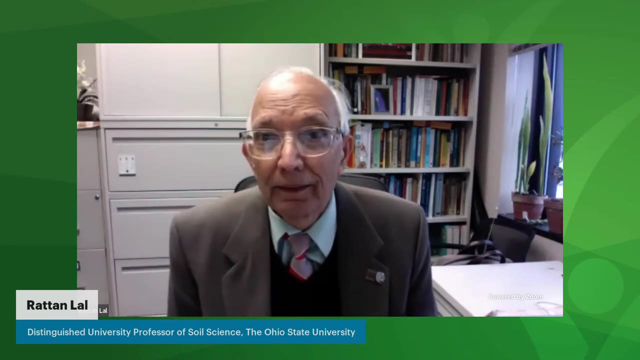 that means you are going to reward those who restore and protect soil health. so I think the I'm surprised that at the kindergarten level, nursery level, We do not have alphabet books which are based on agriculture and soil health and other things. I don't know why not. 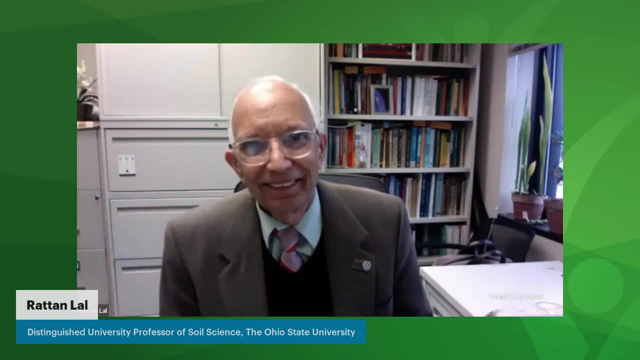 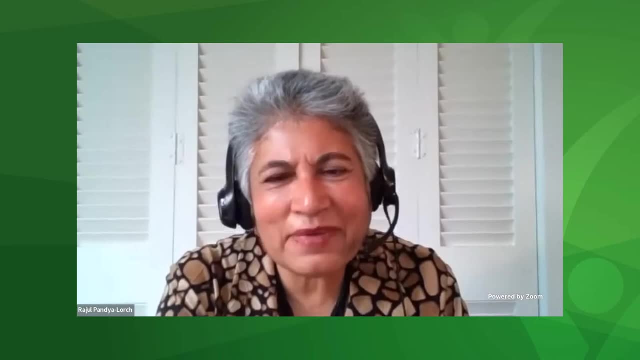 It's for you to write that book. Look forward to Thank you. Incredible Thank you, panelists. I would love for us to continue this conversation, but we are running out of time. to the audience I say thank you for sharing with us your questions And I'm so sorry we could not take all of them. 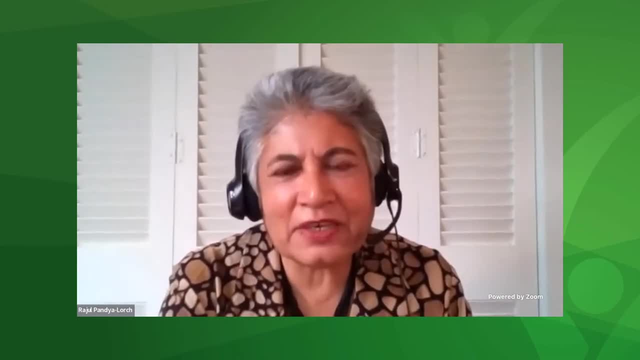 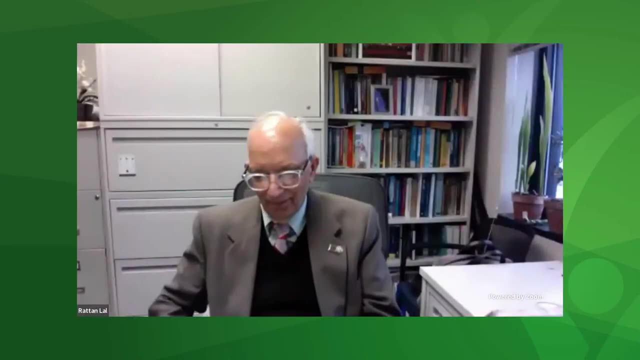 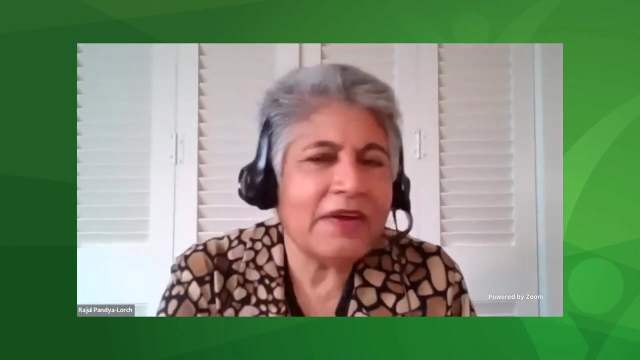 But it is a very lively engagement and a very lively conversation. I would like to give each panelist a chance for 20 second final, final tweetable message. What do you want the audience to take away in these 20 seconds? And then I will give Astrid the closing remarks. I will go in reverse order. 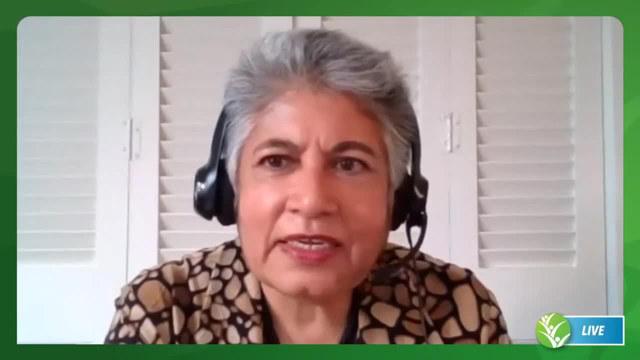 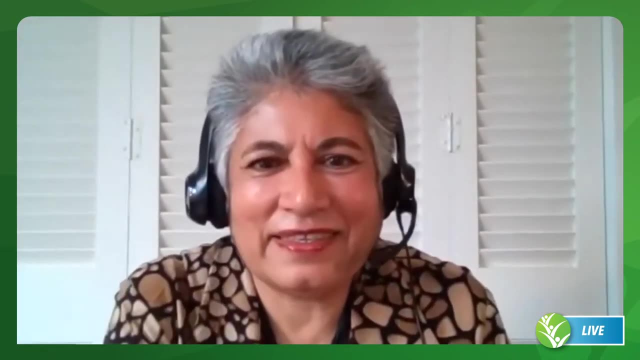 And that will be then Martin, followed by Katrine, Teddy, Jawu, Ratan and Cornelia. Please, Martin, kick us off. For me, I mean, I think the takeaway is the confirmation that providing the right incentives and defining the right values is the right thing to do. 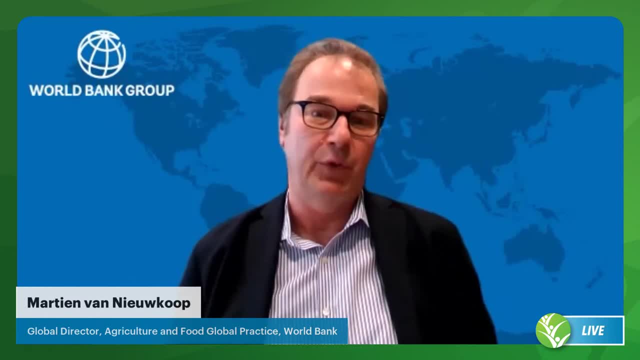 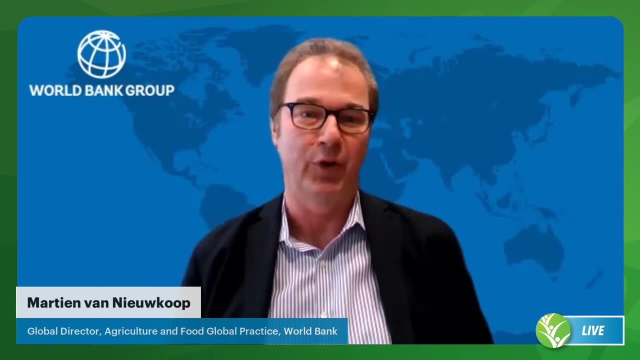 I think the fact that we have over 570 million farmers to invest in healthy soil, I mean, will be a very powerful force, I mean, to transform the food system in support of healthy people, planet and economy. Thank you, Katrine, Thank you. 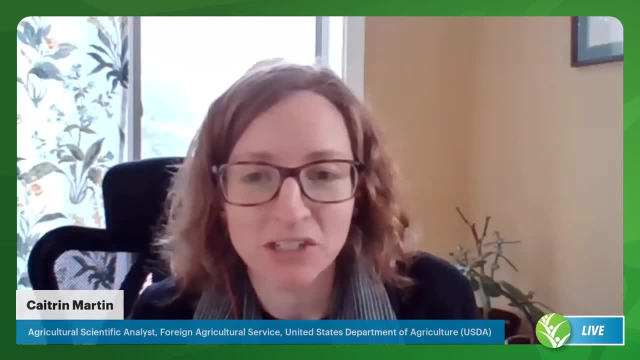 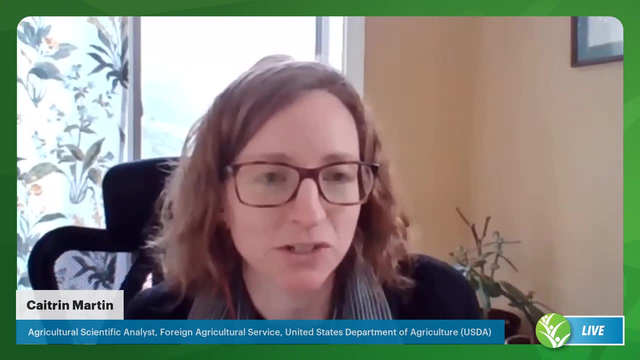 Yes, And thanks to all the panelists, I learned so much today. I'm going to cheat a little bit and give a quote by Secretary Tom Vilsack. This was for a domestic audience, So I'll shift it just a little bit. 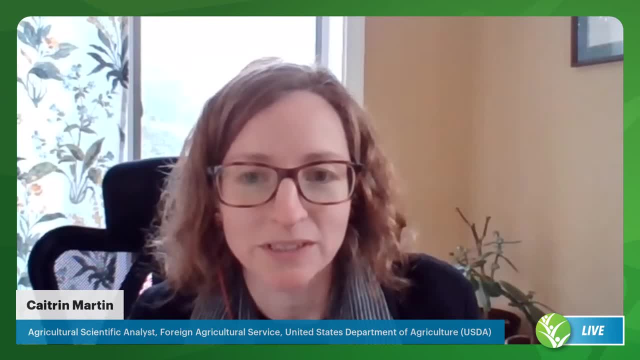 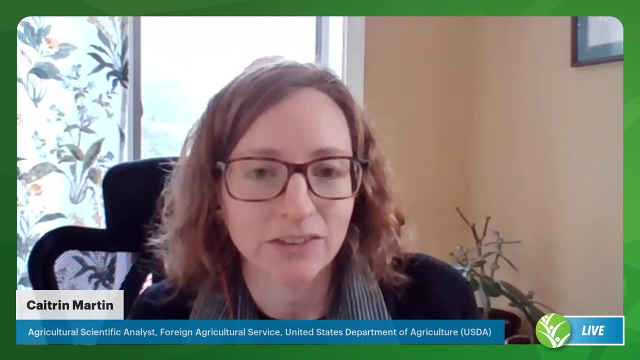 to combat climate change cannot be done alone. to be truly successful, we must creatively examine our partnerships with state, local, tribal, private and non-sector partners, and i would add here international partners- to tap into their expertise, leverage shared resources and seek out new ways to work together to tackle these problems across a landscape that we all share. thanks, thank you. 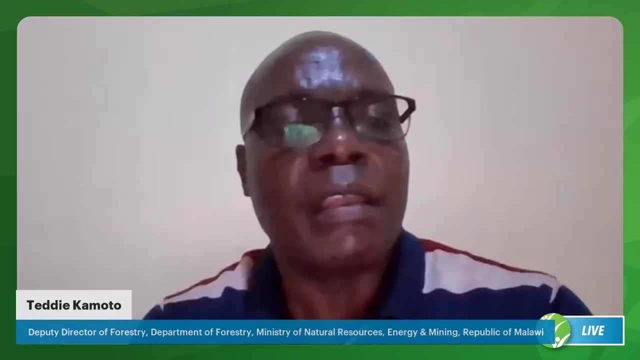 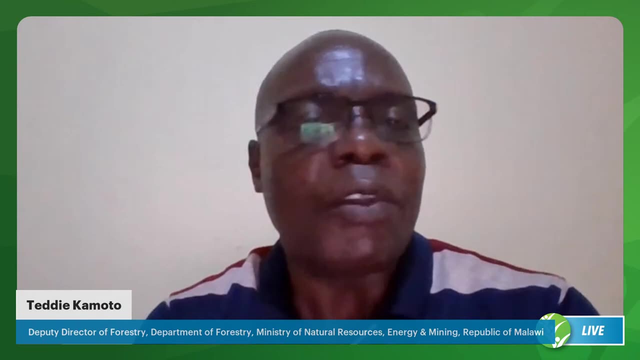 teddy. uh, thank you so very much. i think for me, um, my interpretation of all what we've discussed is that, um, all these technologies that we are talking about, whether it's digital, all these interventions that we, we we're trying to research on, what we should know is, by the end of the day, 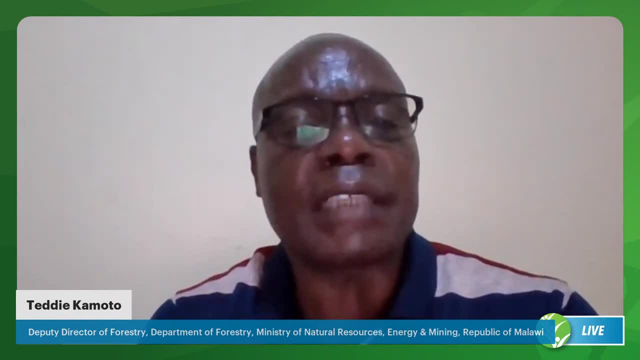 the most important person is the farmer who is going to utilize those, and i think we should make an effort to make sure that we listen to what the farmer is saying, because in some case, the farmer is the one who is going to utilize those. and i think we should make an effort to make sure that we listen to what the farmer is saying, because in some cases, 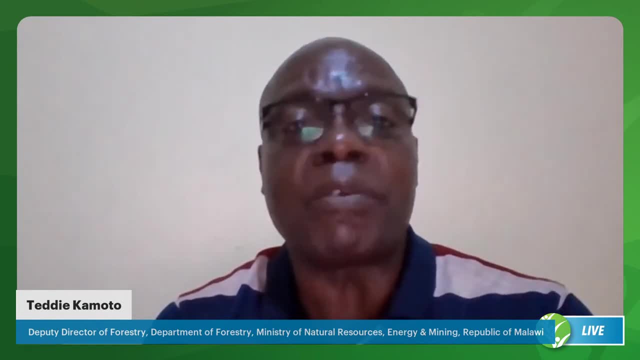 the farmer is the one who is going to utilize those, and i think we should make an effort to make sure that we listen to what the farmer is saying, because in some cases, they do come with brilliant ideas. so that's, that would be my, my way, thank you. 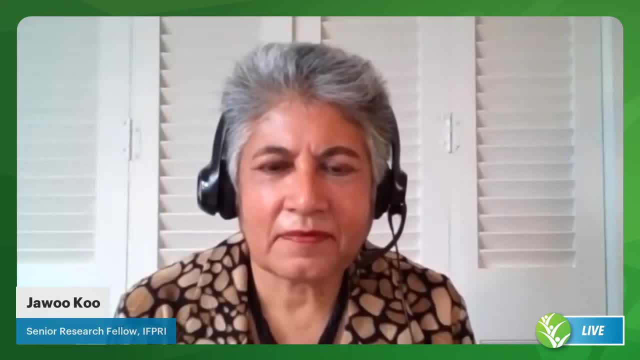 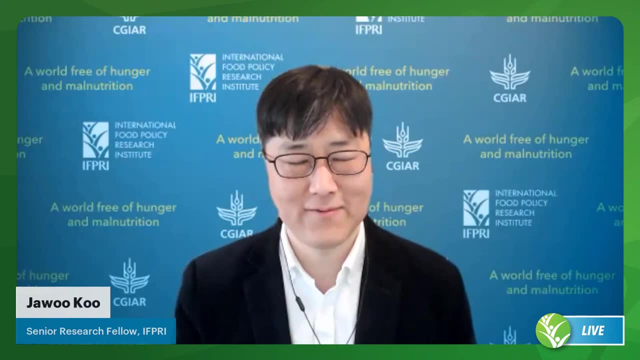 thank you. yes, uh, so we already have very strong source scientific knowledge and how to manage stories better and either get even stronger with more data, uh becoming available on, also utilizing super tools. so, yeah, i think this is time to act. uh, and yeah, i also had a sensation. 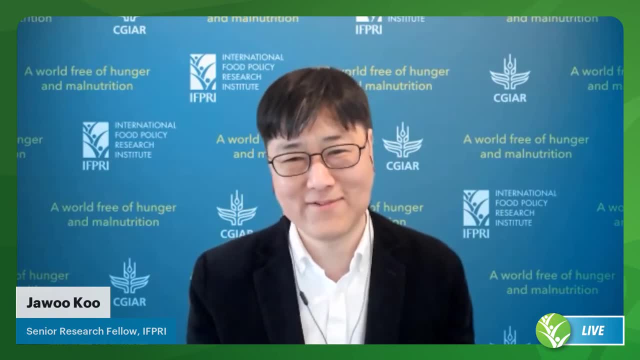 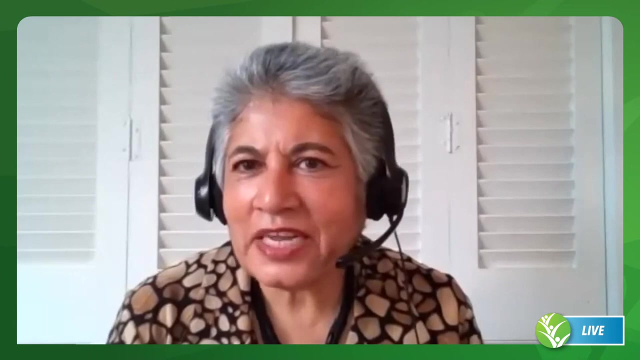 today that professor larry is our generation, the leonardo dicaprio we just don't look up and i think we should uh continue his journey and story, um to really uh bring the audience and make this global action happen. yeah thanks, thank you, professor lal, or the new leonardo dicaprio. 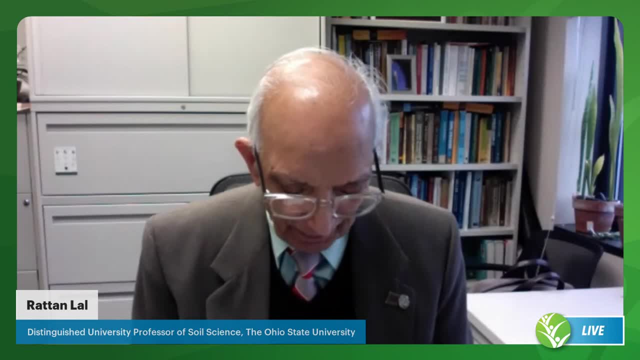 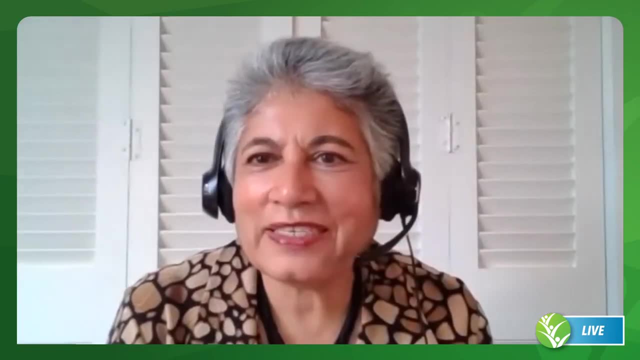 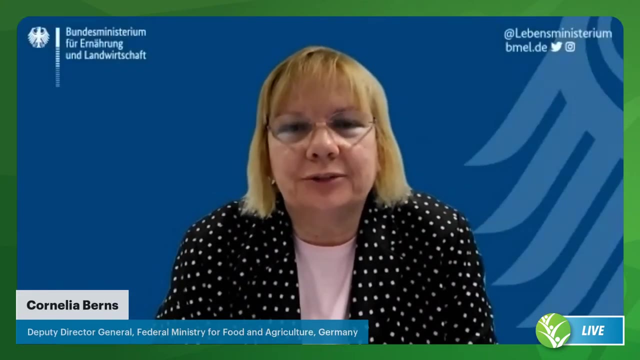 thank you. our policy should be pro-nature, pro-agriculture, pro-farmer and pro-soil. thank you, thank you, thank you, and cornelia, you have the final word. yes, thank you very much. yeah, we all have to take the torch forward and move on to really transformation, uh, of food systems and uh, i just want to mention that. 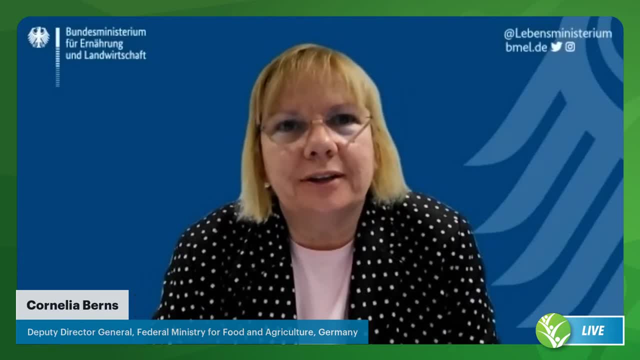 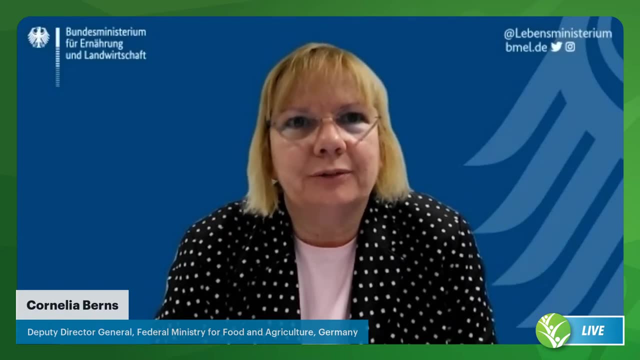 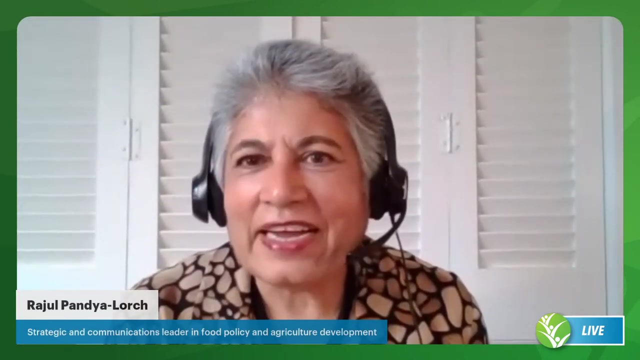 germany is going to pick some of the topics up in the in our g7 presidency, looking at sustainable supply chains and carbon farming. thank you very much. thank you, cornelia. colleagues, this was a remarkable, remarkable session and i echo catherine. i learned so much i will not dare. 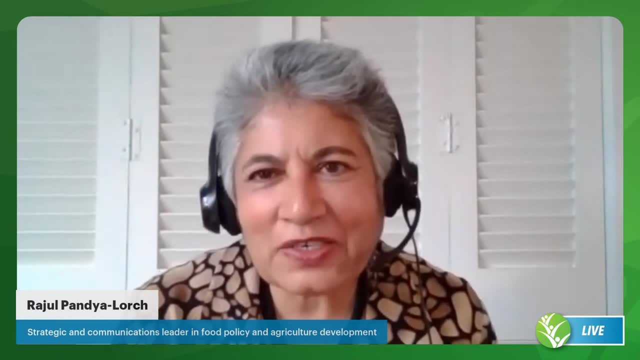 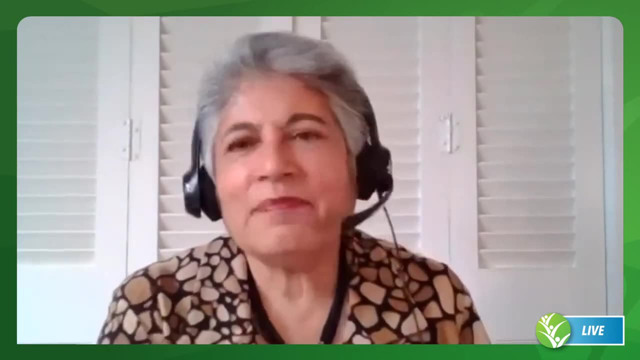 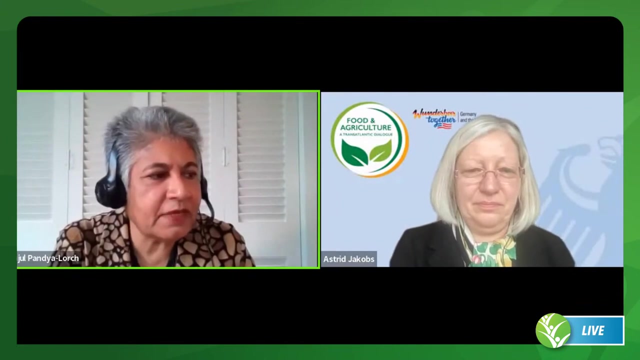 think i will pass that uh back over to astrid. i know i probably you will not summarize but share some reflections. but, astrid, over to you and this is, um, uh, let me introduce you formally. uh, we are turning to astrid jacobs de padua, the minister, counselor and head of department for 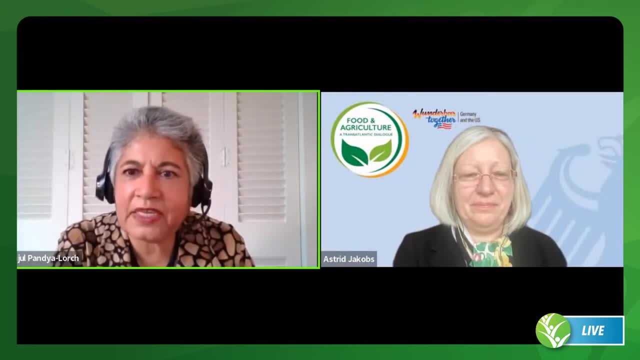 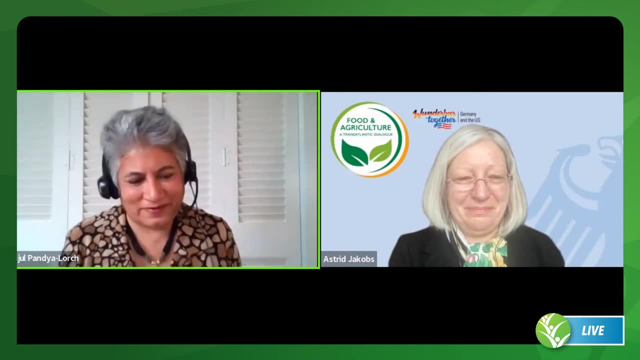 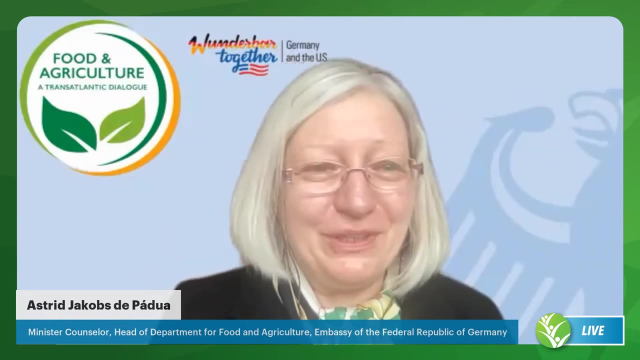 food and agriculture at the embassy of the federal republic of germany in washington dc, and really the lead organizer for this remarkable event. astrid, over to you. thank you very much. it's really difficult to uh to find better words than these. we just have heard, and i think we've really identified our champion, which is professor ratan dal. so um, i would first of all, 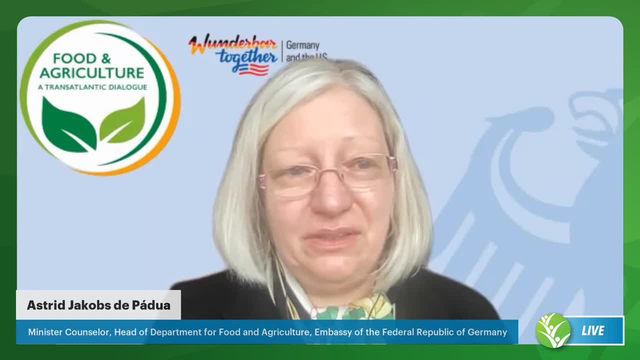 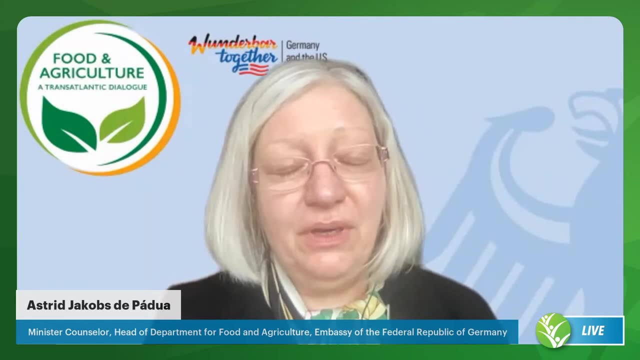 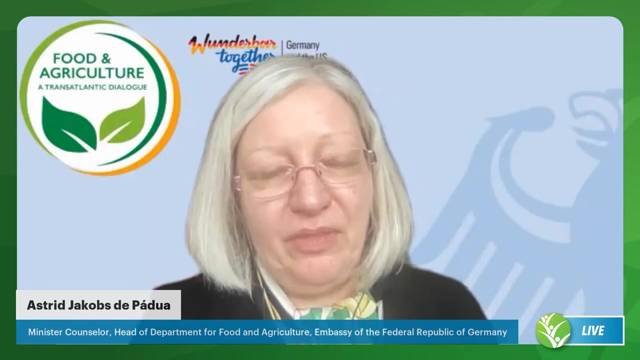 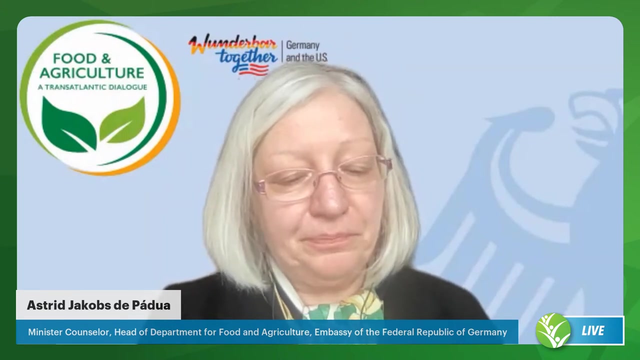 like to thank all speakers for this great uh exchange and event. i would like to thank uh ifpre to facilitate this because, with your support and um helping us with bringing people together and these uh wonderful platform you have, uh would, it would be. not, it wouldn't be possible. i would like to you, uh rajul, that you gave us. 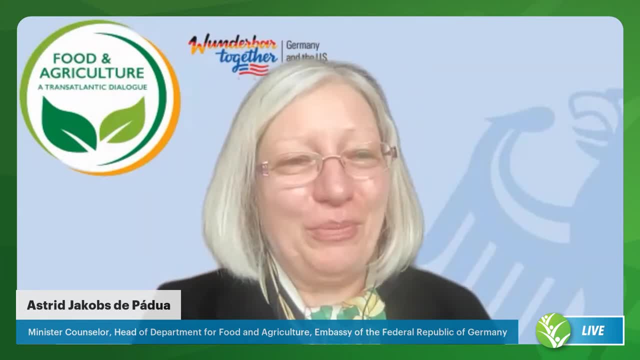 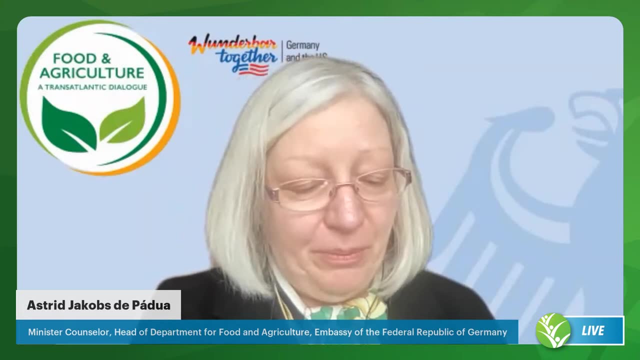 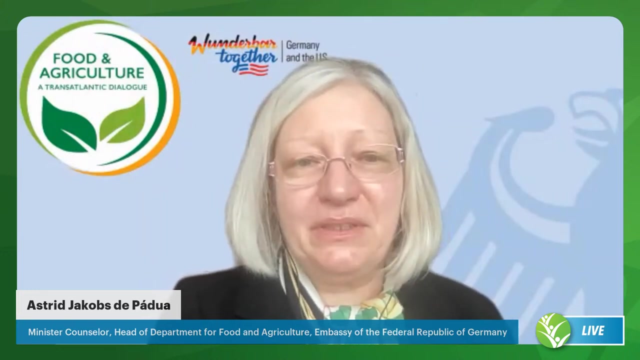 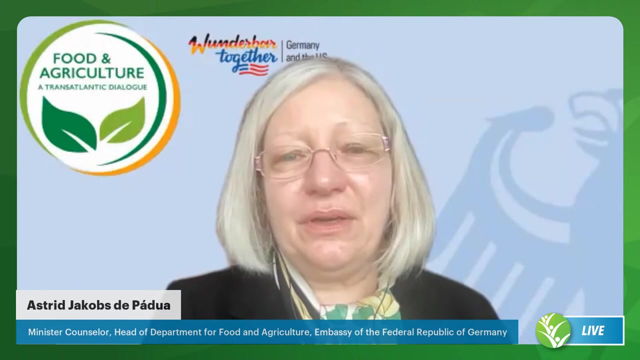 really a wonderful uh moderation through the topic and teasing everybody with the questions. um, for me, connie already mentioned, g7 offers a lot of more topics. um, therefore, here at the embassy, we decided to start a platform. you can see our new uh logo up there: food and agriculture, transatlantic dialogue, so you can. 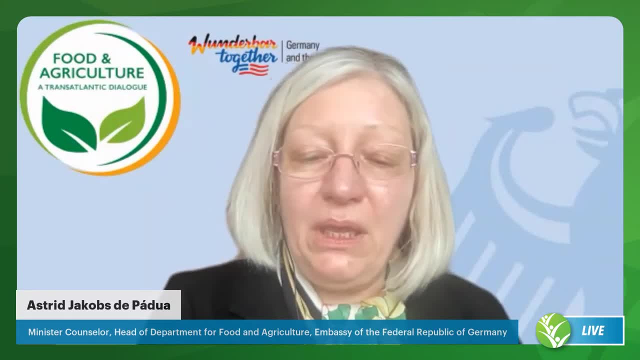 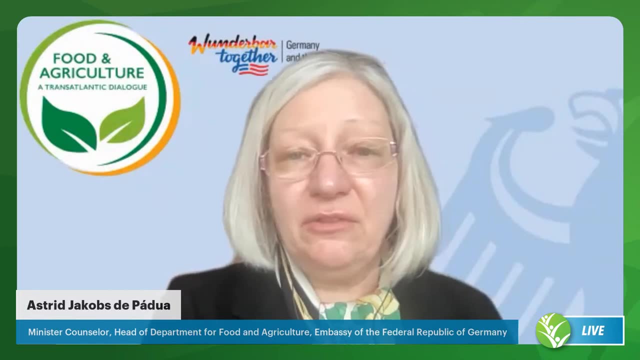 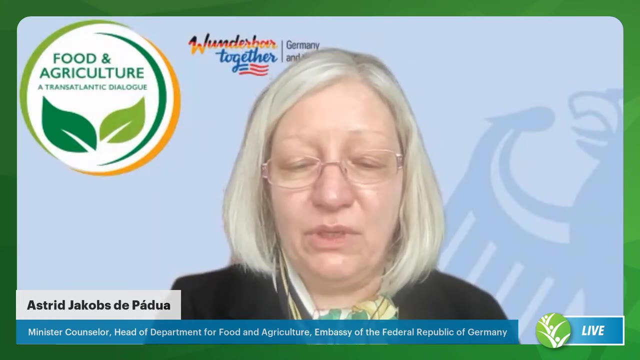 expect more of us. um, we- i i heard you know the challenges are huge. we have on the one side the individuals which we need to give access to healthy food. it's not just about quantity, but also about qualities. so how can, are we able to feed the world, whether it's 7 billion or 9 billion? 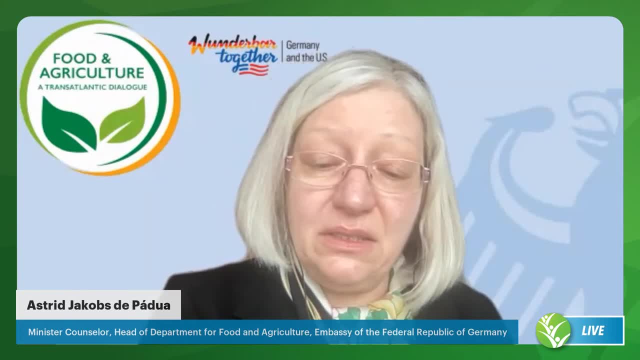 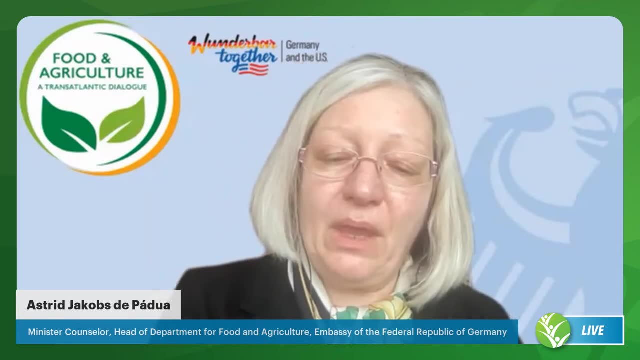 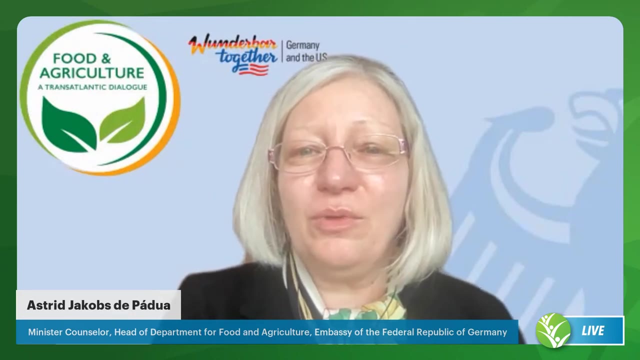 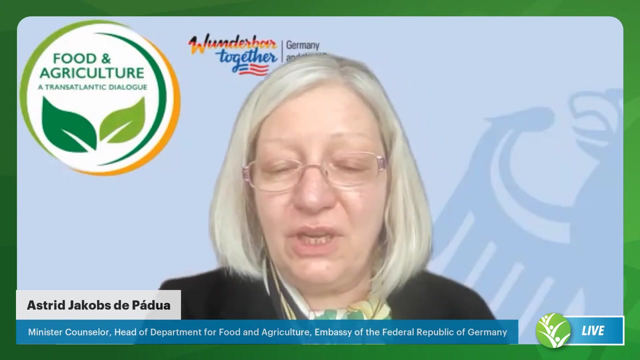 who knows? we learned that there is technology and innovation out there. there are old um techniques, there are old um practices, which we shouldn't discard but take into account. katrin, you mentioned the one yearbook, from 1938, so that's impressive. but we have also the opportunity to take char, to take new technologies. 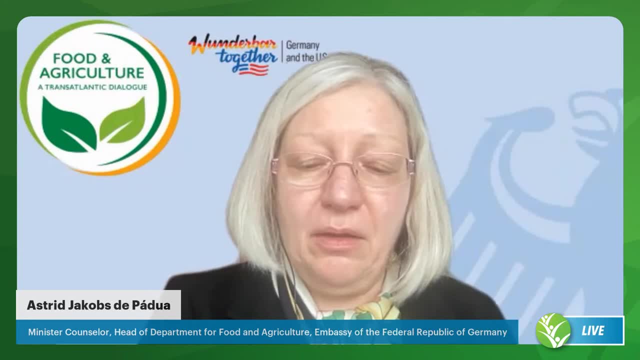 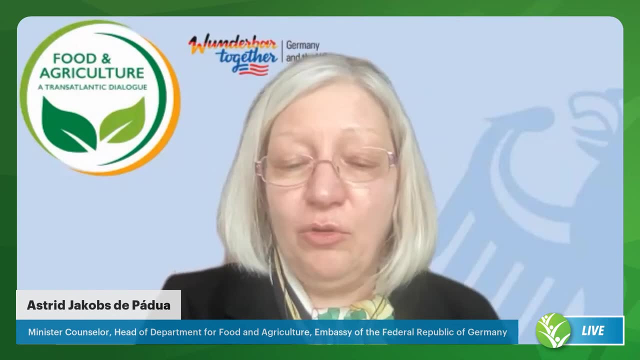 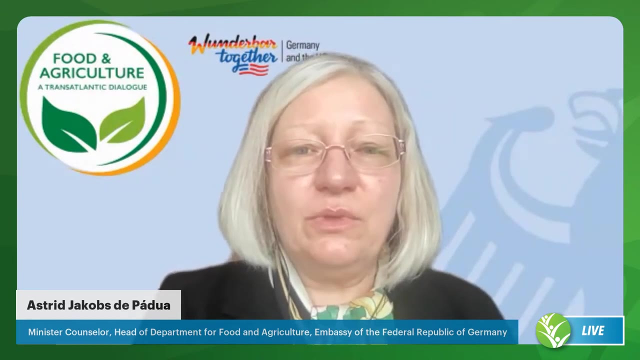 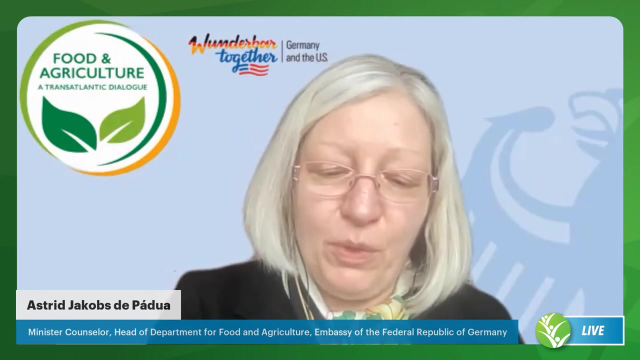 and to advance and to to grow. on this, we learned from governments that, uh, they're on top of it, they're working in it. there are no silver bullets and i- uh, teddy, i really heard you farmers. we need to learn to listen to farmers, and there will be another part of this discussion where we will bring in farmers. 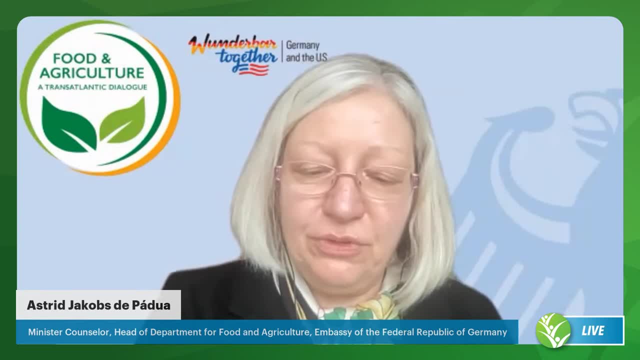 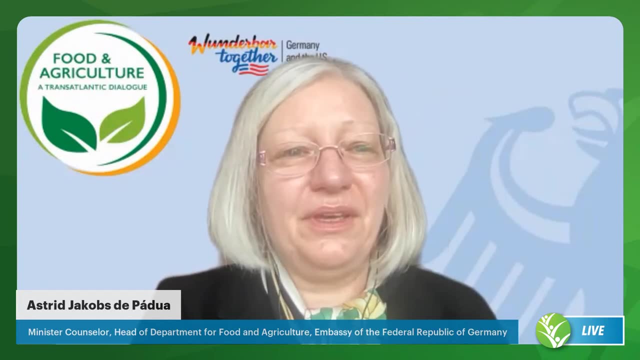 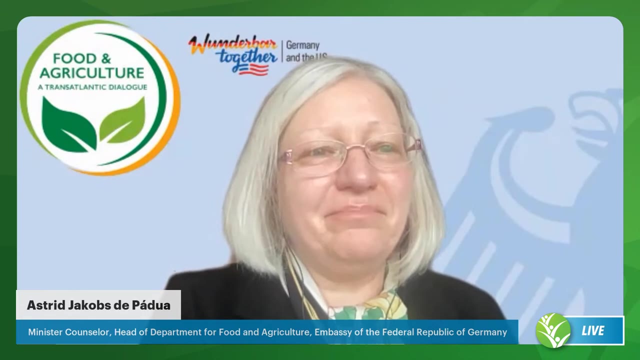 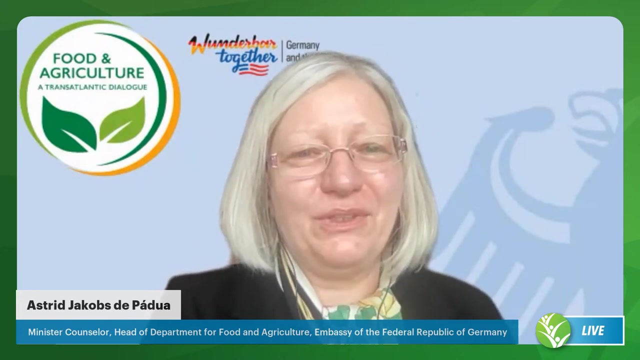 and i think there is no better way to to bring everything together. and in saying, soils are the essence of life, i think that is the one which sticks with me as my new motto for the upcoming events: work, everything will be around this aspect. thank you very much. 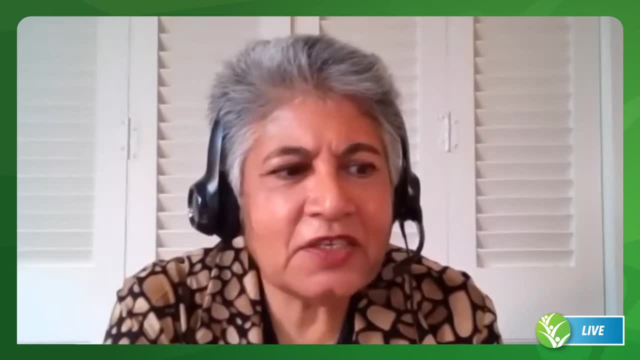 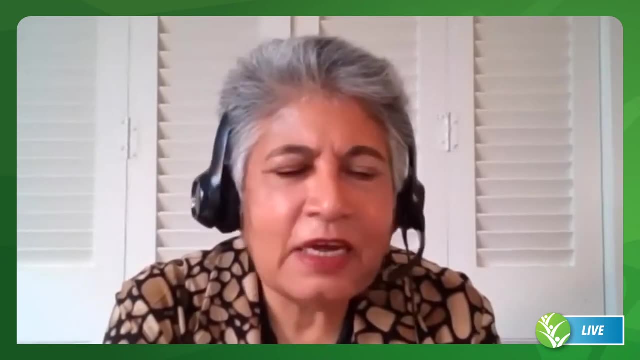 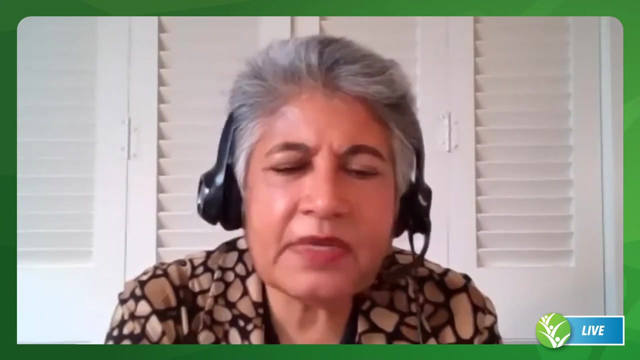 thank you, astrid. before we adjourn, i would like to invite all of you to please join IfPri on february 23 at 9: 30 am est for the next policy seminar, which is an advancing food systems transformation, a dialogue between german development cooperation and cgir co-organized. 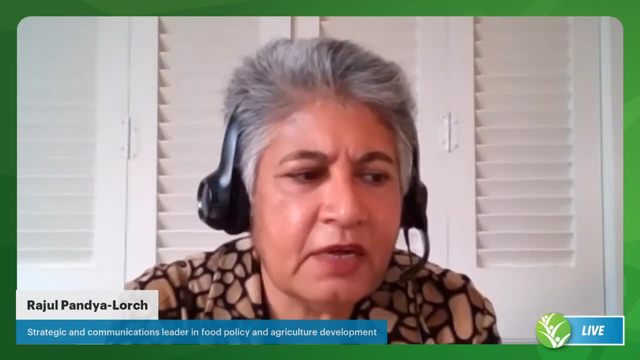 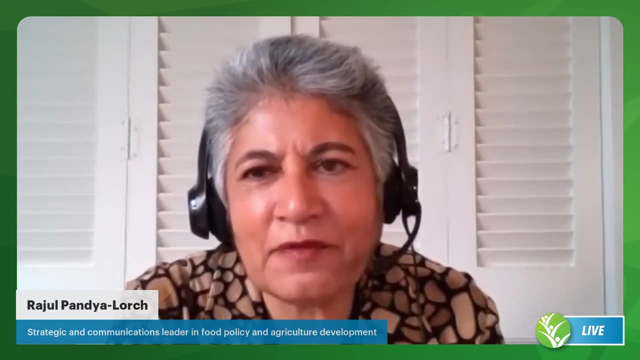 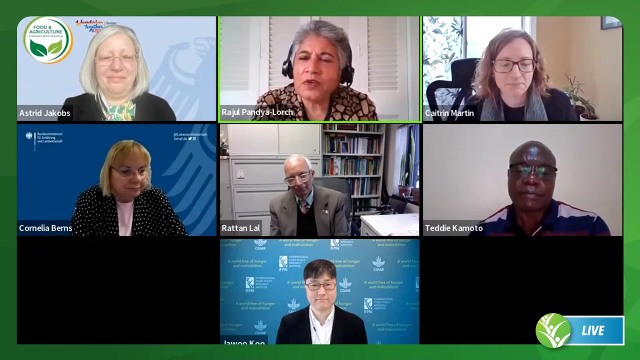 by the cgir if free and the german federal ministry for economic cooperation and development. a big thank you to all the speakers today for your inspirational and informative remarks. a big thank you to all the participants for taking the time to join us and a big thank you to all of those who